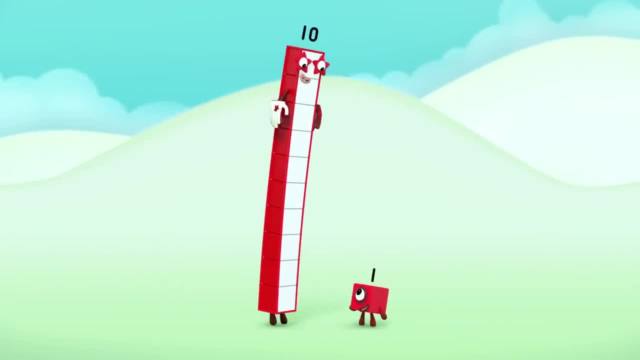 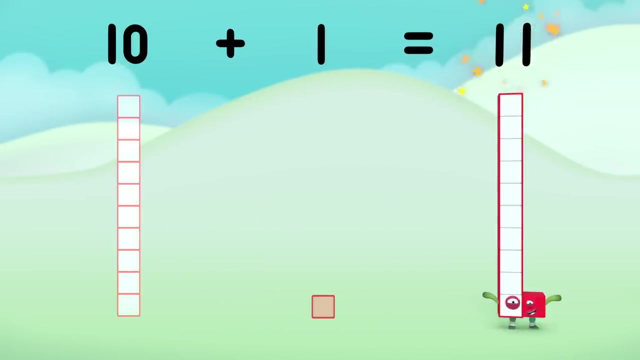 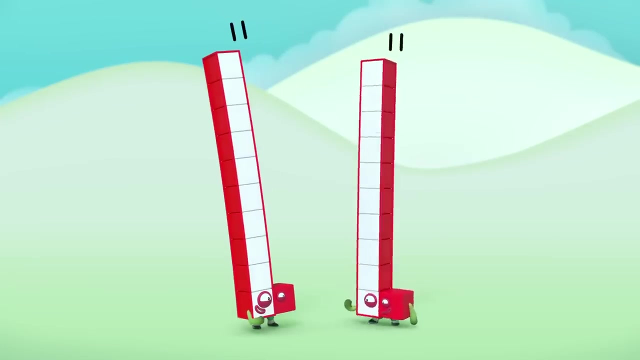 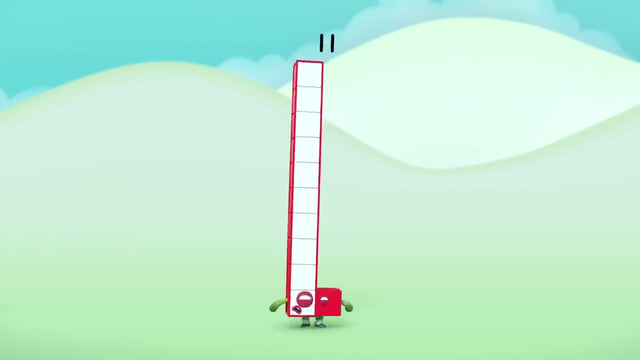 Hello ten, Hello one. What shall we play today? What was that? Who was that? A new number. block Ten plus one equals eleven. Hello, I'm eleven. So am I, And I'm ten and one. That's better. 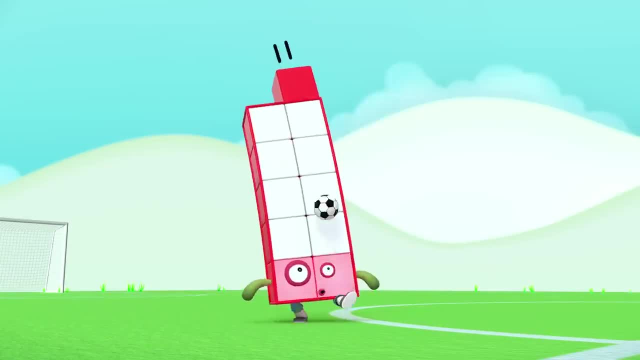 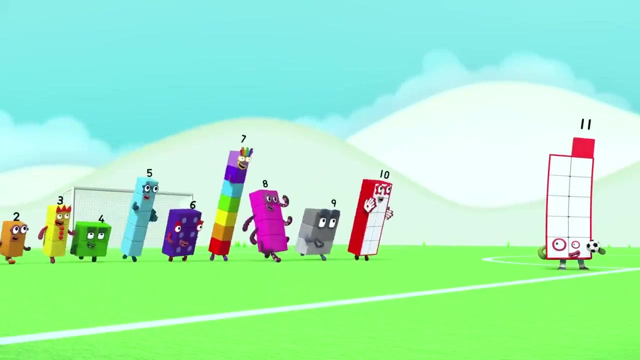 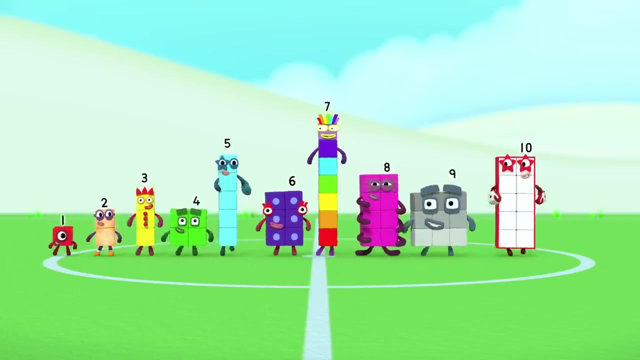 Whoa. One, two, three, four, five, six, seven, eight, nine and ten, And one more is eleven. I am eleven and I love football. Wow, Let's play football, Hooray. One, two, three, four, five, six, seven, eight, nine and ten. 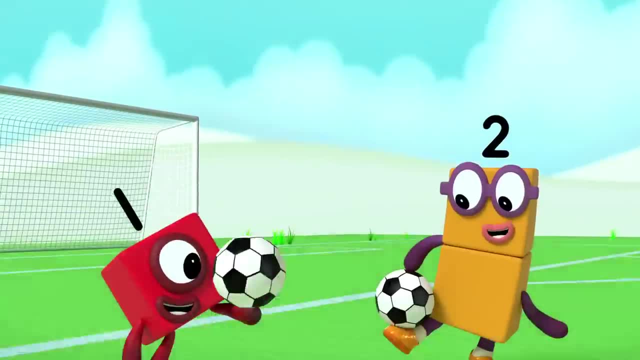 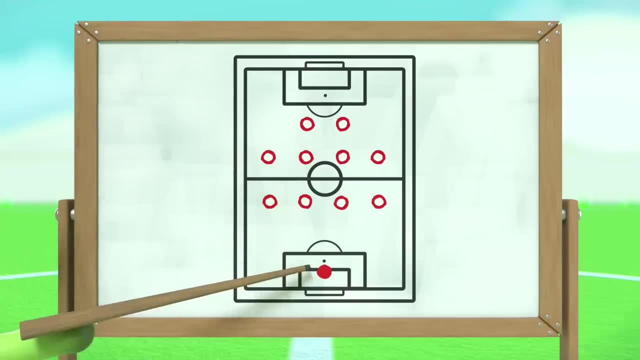 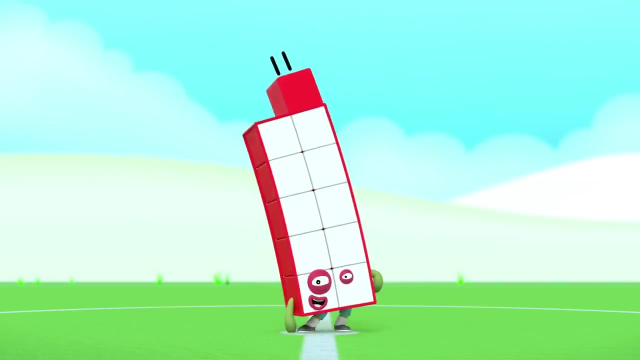 One more is eleven. We're on our way to victory. We're on a roll, We're ten and on the pitch, And one in gold. We will never be denied. We'll take it in our pride With ten and one. ten and one, eleven on our side. 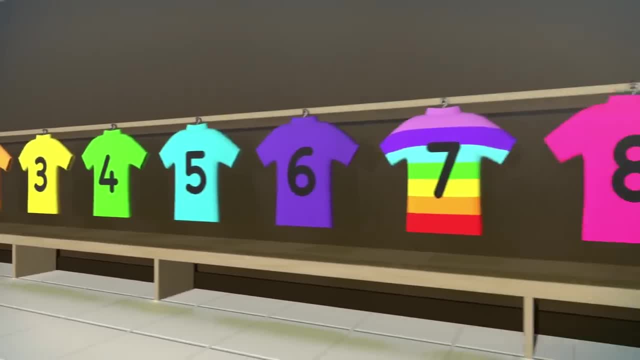 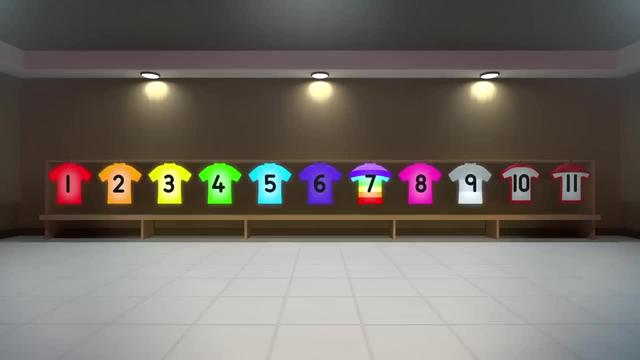 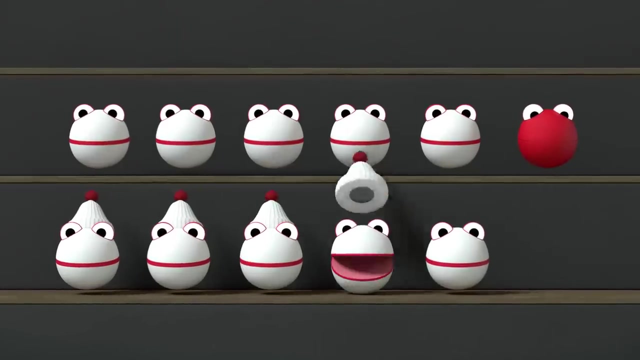 Football shirts. Football shirts, One for every number. block Football shirts: One, two, three, four, five, six, seven, eight, nine and ten, And one more is eleven. Hooray Bubble hats. Bubble hats. 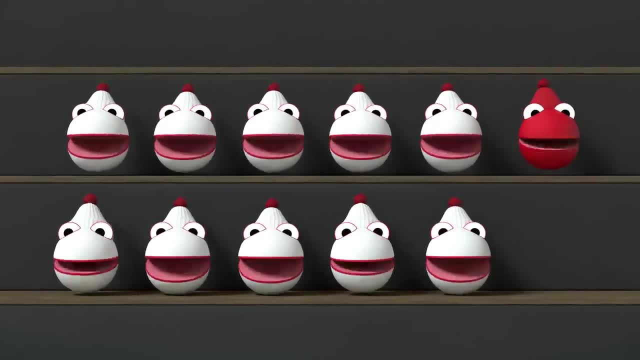 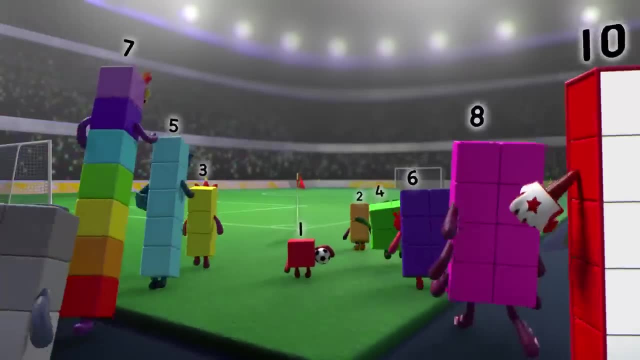 One for every number: block Bubble hats: One, two, three, four, five, six, seven, eight, nine and ten, And one more is eleven. Hooray, We're on our way to victory. We're on a roll. 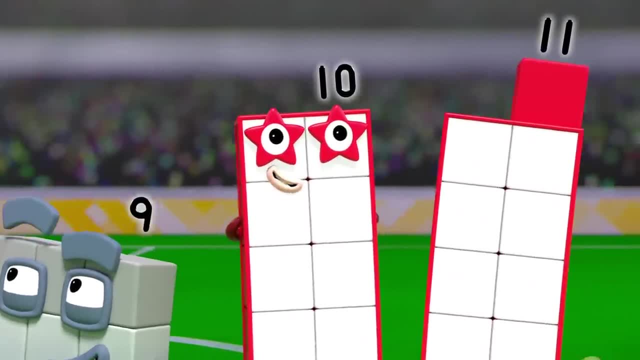 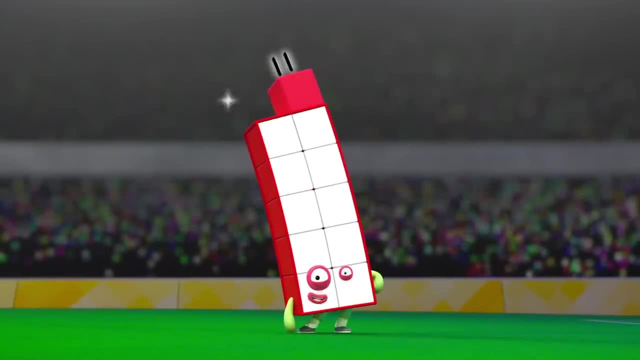 We're ten on the pitch And one in gold. We will never be denied. We'll take it in our pride With ten and one, ten and one, eleven on our side. We're ten One one, Ten And one. 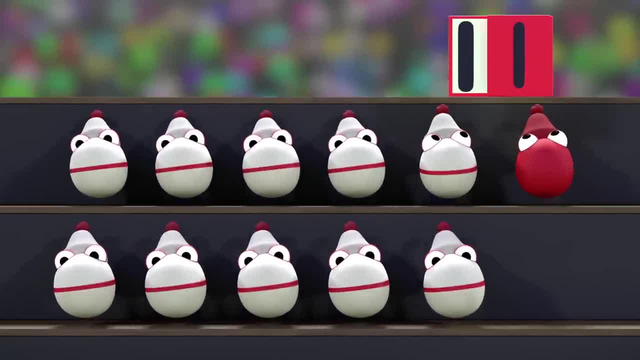 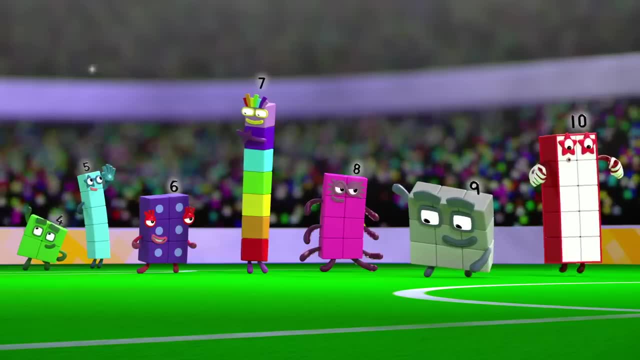 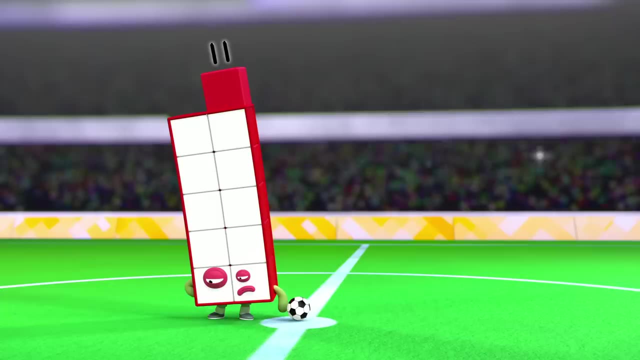 Eleven, One, one, Ten And one Seven- The number blocks- are out on the pitch for the big match And their captain, Eleven, looks ready to lead the team to victory. Something's wrong. What can it be? I've forgotten something. 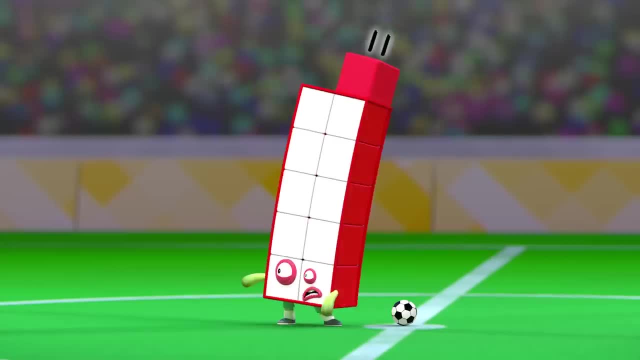 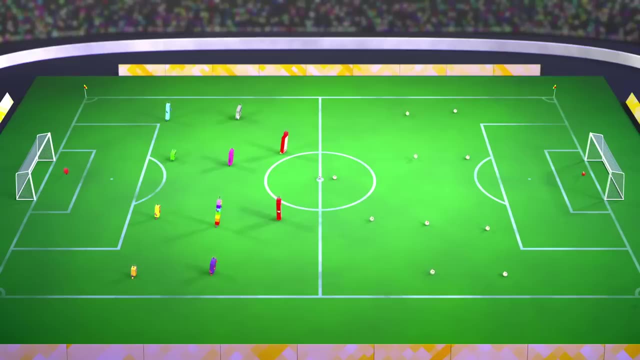 The other team. We need eleven more players. Number blocks: Game on And the number blocks have kicked off. It goes high towards the goal And saved by one. Take a bow one. One throws it down to two. Who passes it? 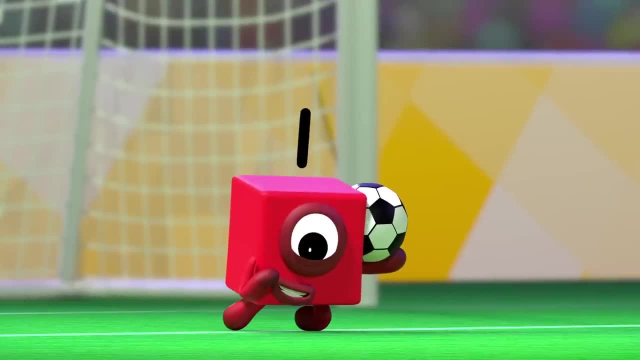 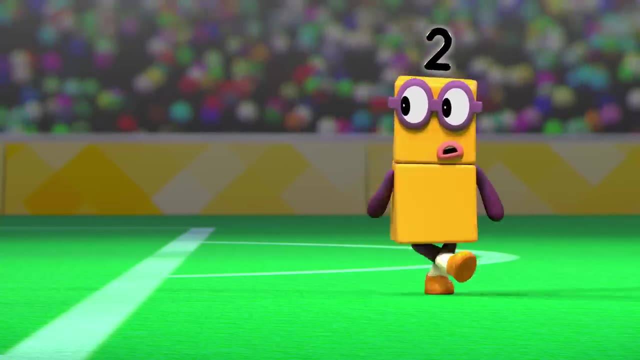 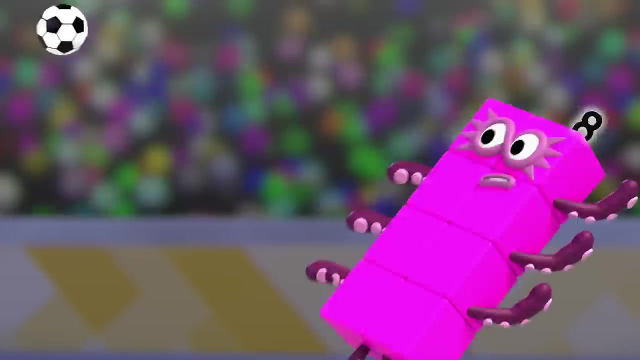 That's right To three, Four, Five, Six, Seven, Eight, Nine And ten. Now pause it to eleven, Seven, Eight, Nine And ten. Now pause it to eleven, Seven, Eight, Nine And ten. 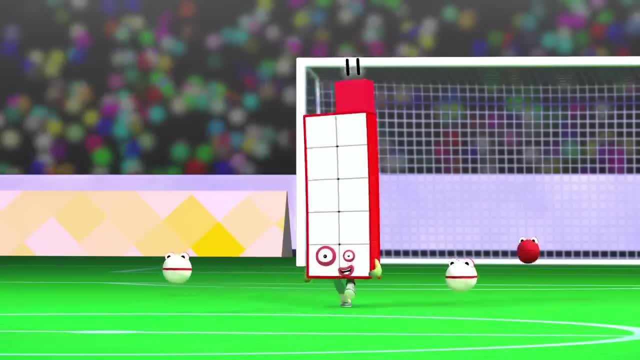 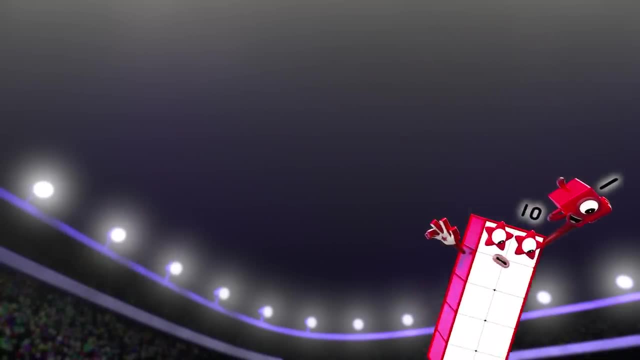 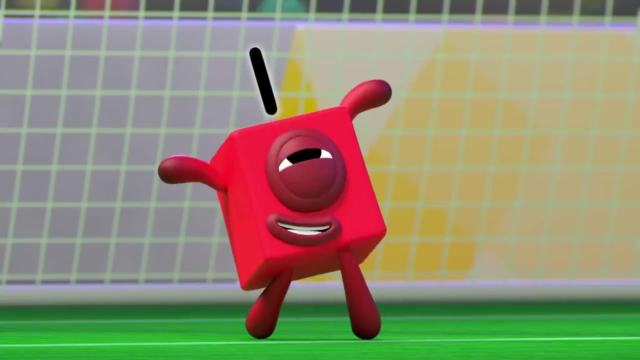 And ten. Now pause it to eleven, Seven, Nine, Ten passes, Eleven bleeps for the header and, oh my, Splits into ten and one to reach the ball. Incredible, And It's a save. What a save. 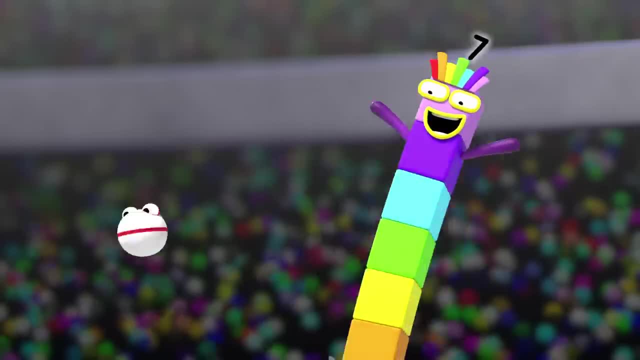 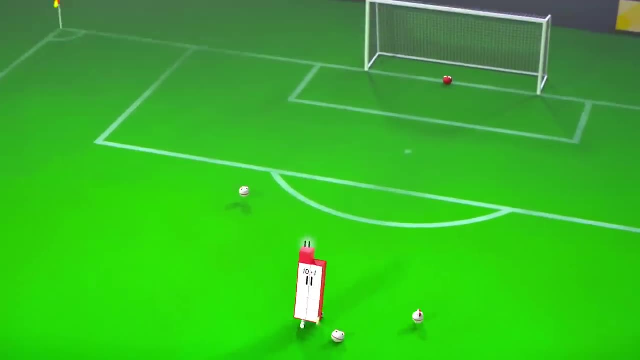 Number block passes to number block, The fine's number block. We'll find Number Blob and a lovely header there to Number Blob. Look, 11!. He heads it to 11.. And it's 11!, 11!, 11!. 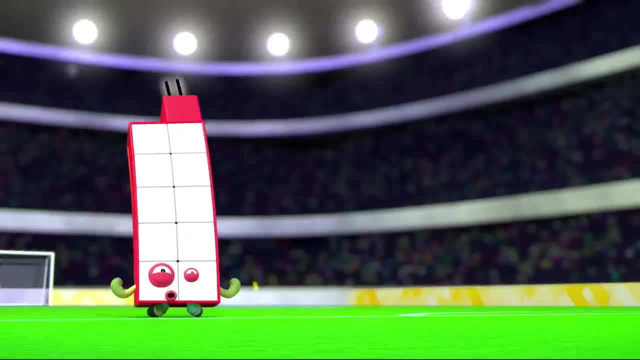 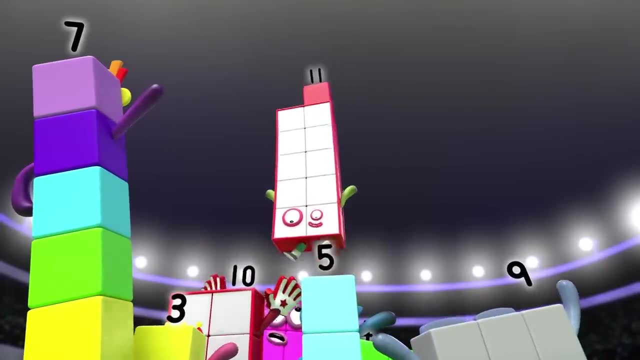 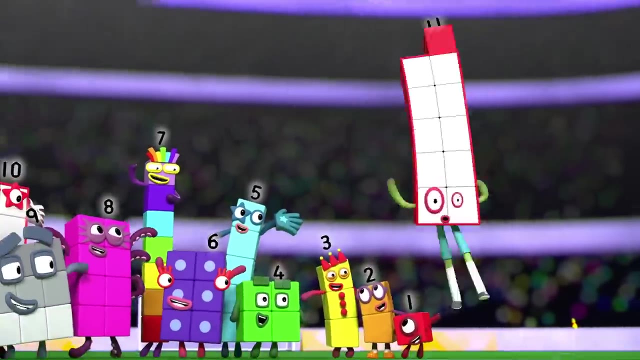 Whoa, Yeah, Whoa, Whoa. We're on our way to victory. we're on a roll With 10 on the pitch and one in goal. We will never be denied. we'll take it in our stride With 10 and 1, 10 and 1, 11 on our side. 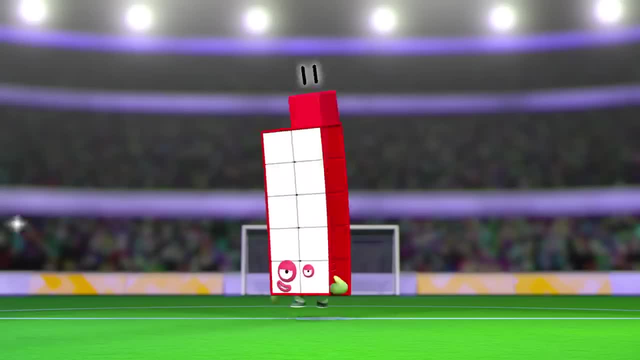 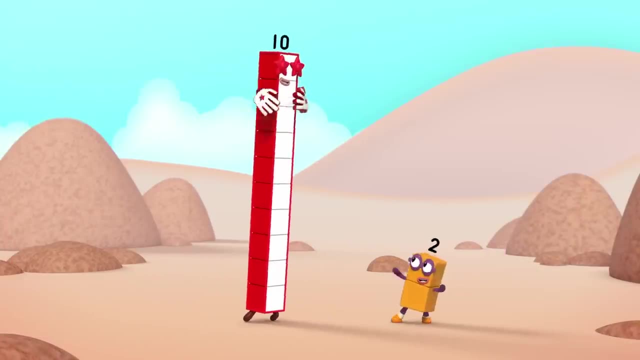 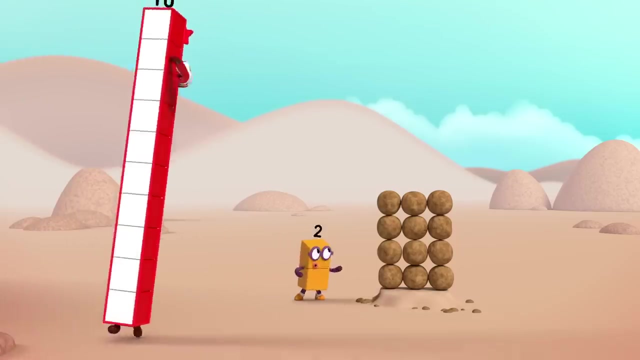 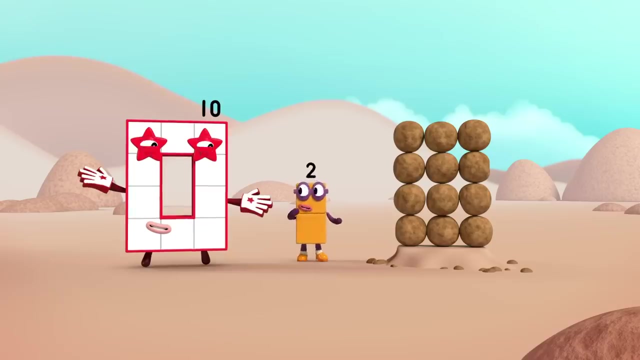 10 and 1, 10 and 1,, 11 on our side, Yeah, 10! And 2!, 10!. And ooh, Look at that, Hey, What am I? Oh, um A rectangle. 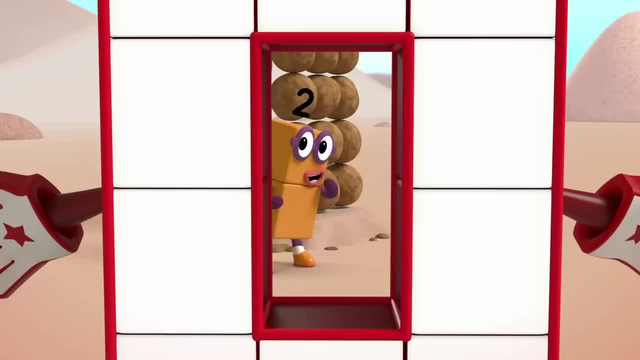 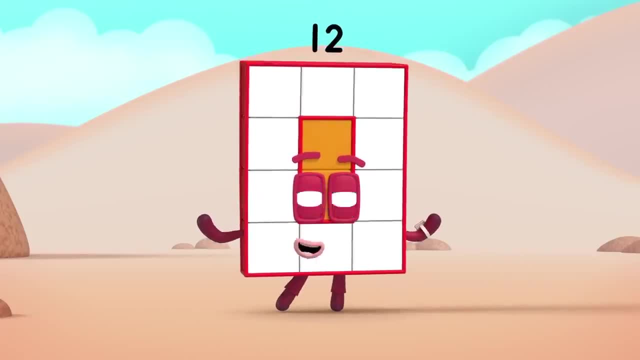 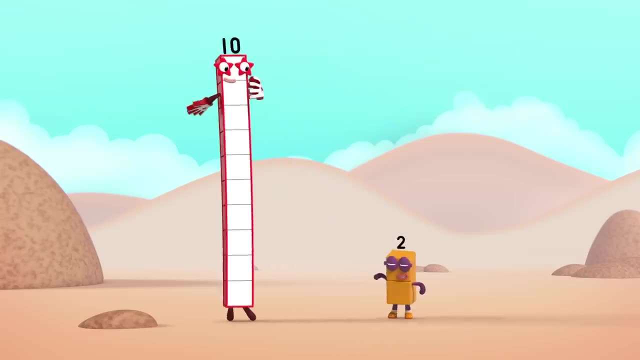 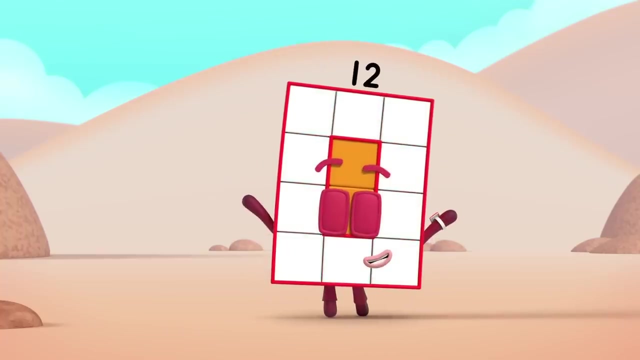 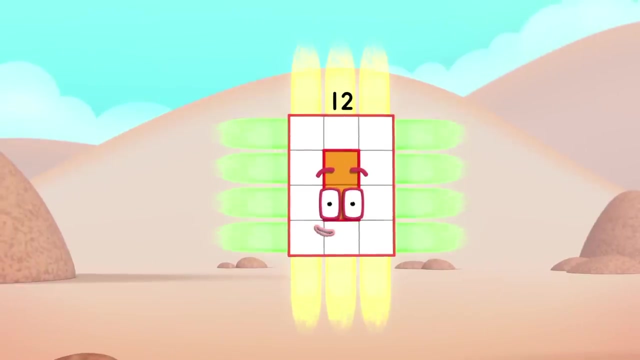 With a hole. Come on then, Ooh, A whole new rectangle. I'm new, I'm 12!, I'm 10 and 2!. 12!, Yes, I am 12! And I am a Super rectangle. 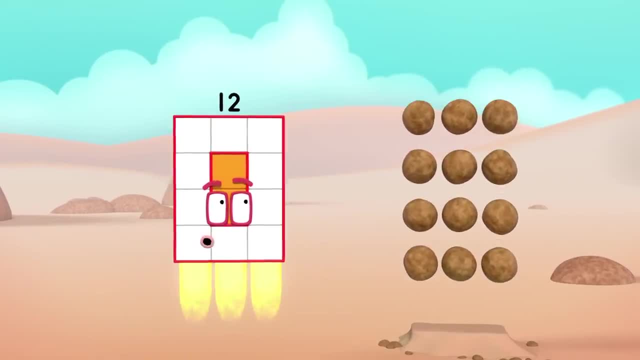 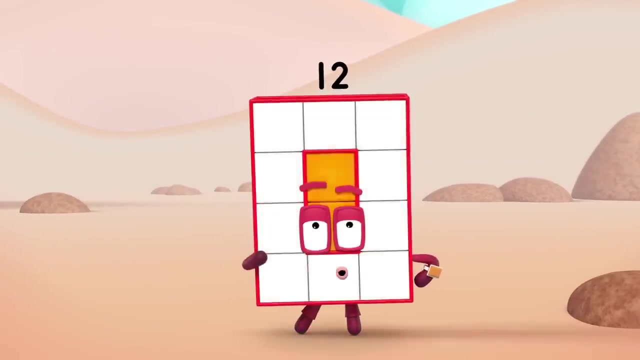 The rocks are in columns and rows, My blocks are in columns and rows And that's called an array- Array. Hey, I'm Rectangular 12!. I'm 10 and 2. I make arrays. that's what I do. 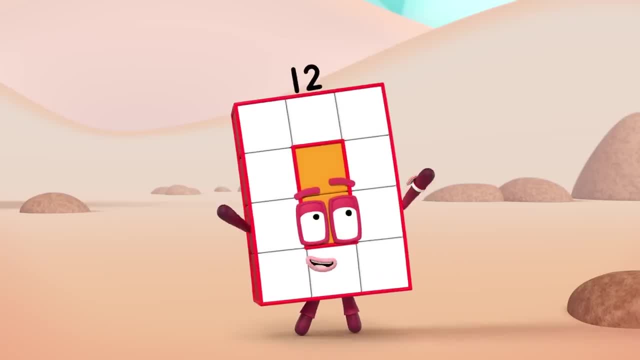 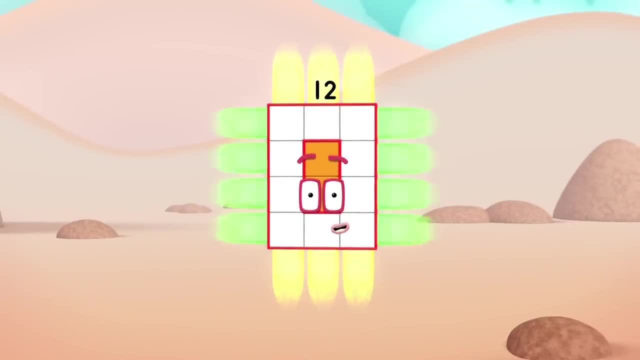 I'm 10 and 2, I make arrays. that's what I do When I put my blocks in columns and rows, I make an array and my rectangle goes like this: Three by four. Today's the day for an array display. 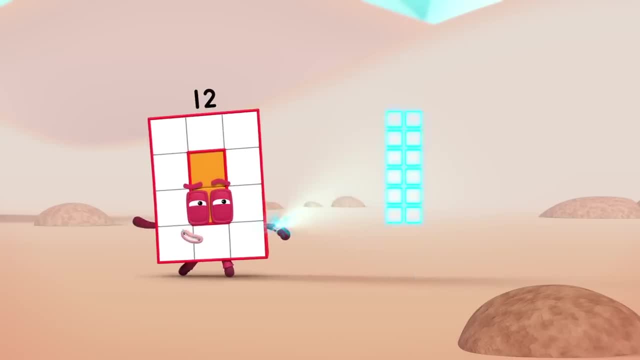 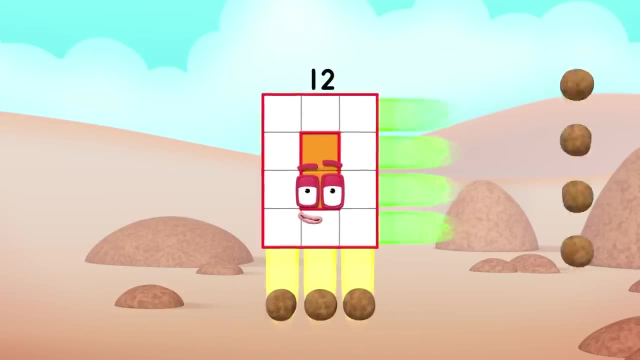 I can make arrays all day. I make arrays in many ways. Stand back, let's play arrays away. Three by four is my first array. Three, lots of four- you could put it that way, And if you're not following what I say, 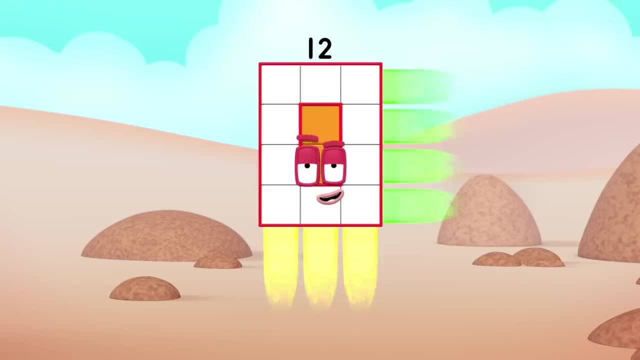 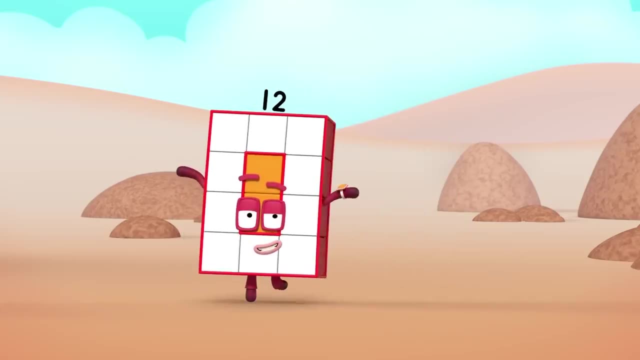 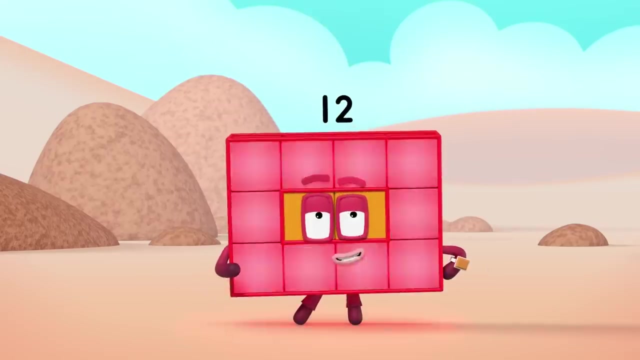 I'll rectify that right away. Break away Three fours, A four and a four and a four. Rectangle rise Time: I'm rectangular 12, I'm 10 and 2.. I make arrays. that's what I do. 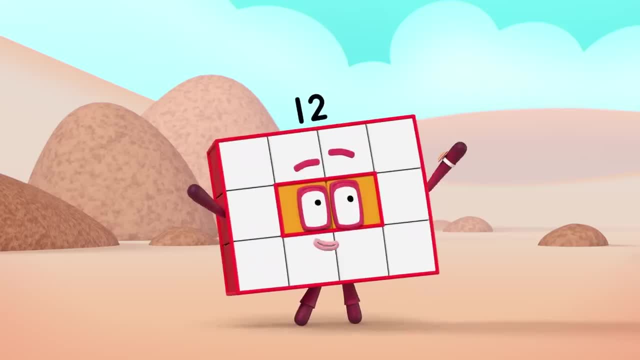 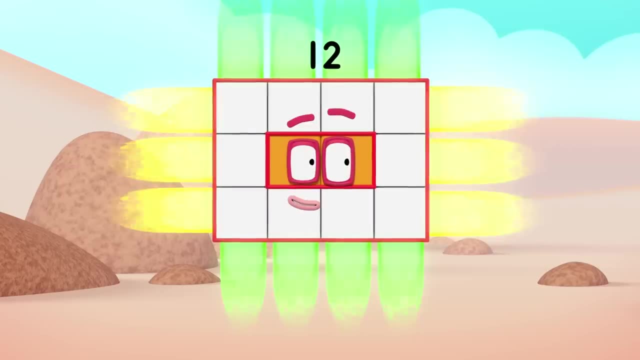 When I put my blocks in columns and rows, I make an array and my rectangle goes like this: Four, Five, Three, Four by three's. my next array: Four, lots of three, you could put it that way- And this rectangular display is about to show you how it's made. 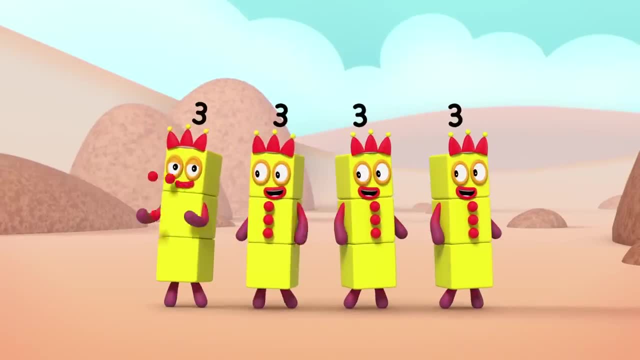 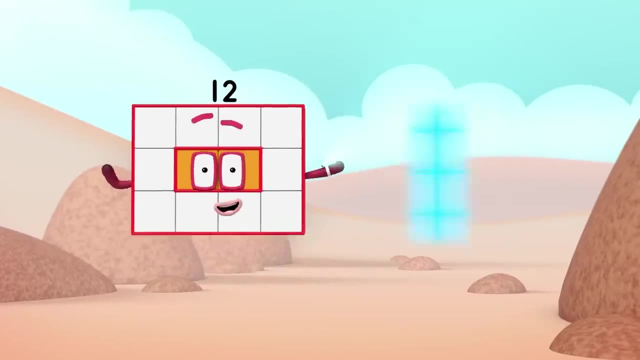 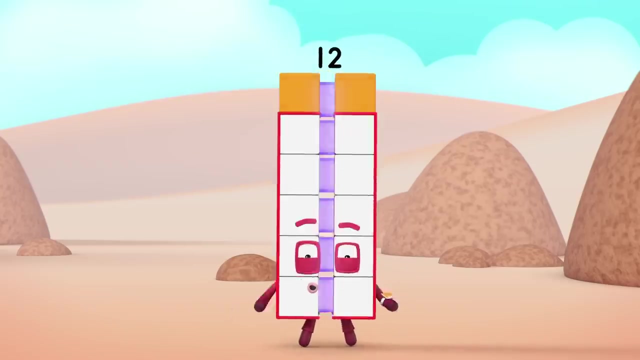 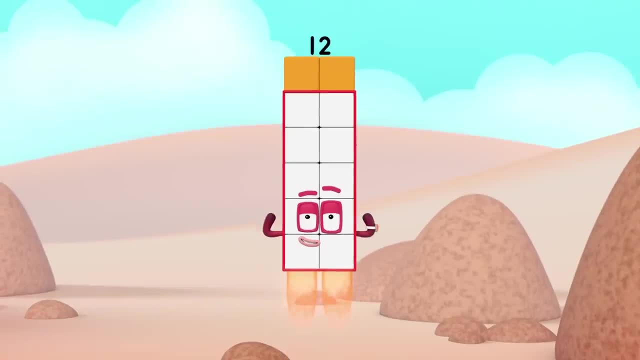 I make an array and my rectangle goes like this: Two By six. Two by six is another way. Two, lots of six. do you hear what I say? Another rectangular array. So let's split Without delay, Break away Two sixes. 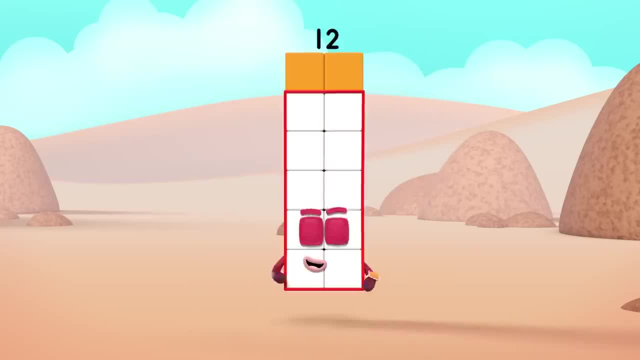 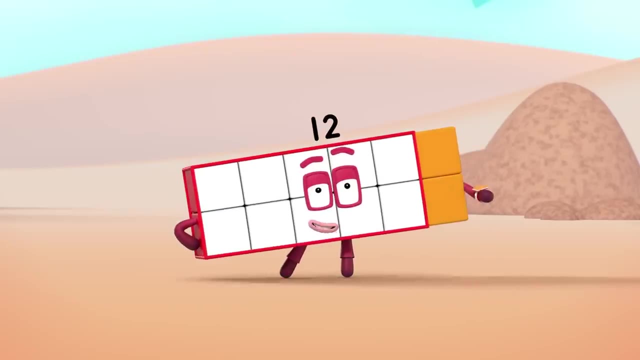 Let's roll Double six Time Time. I'm rectangular 12,, I'm 10 and 2. I make arrays. that's what I do When I put my blocks in columns and rows. I make an array and my rectangle goes like this: 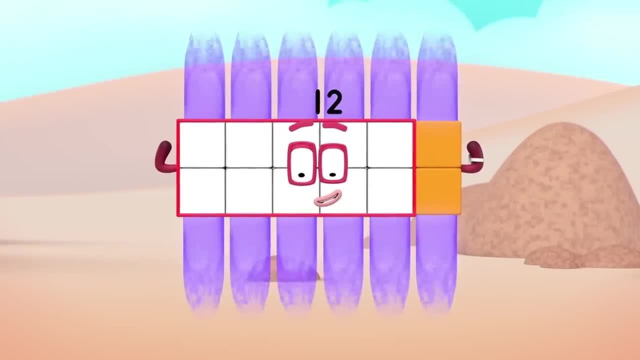 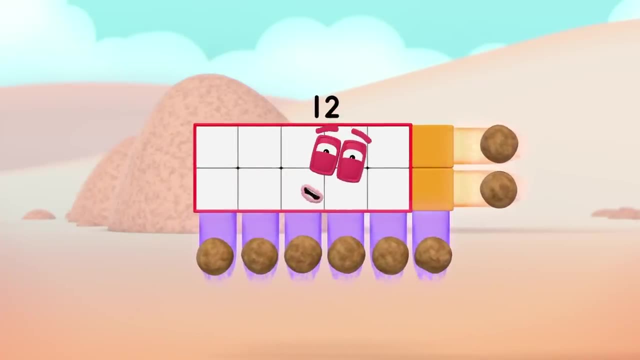 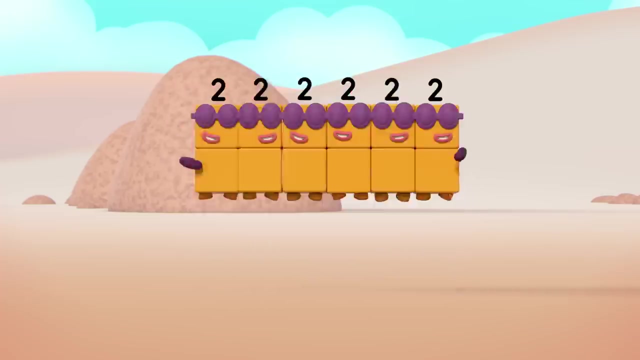 Six By two. Six by two is next in line. Six, lots of two. it's a clever design And if you want to see how all this fits, I can break it all to bits. Break away Six, two, Two. 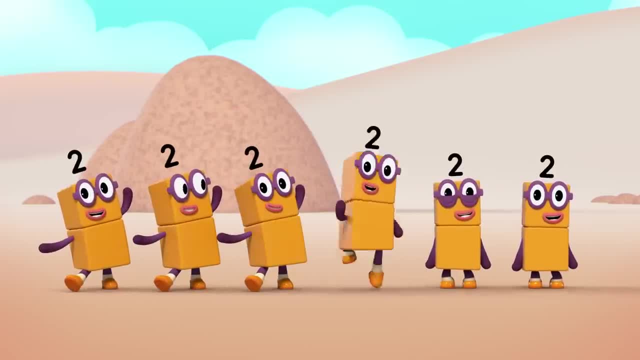 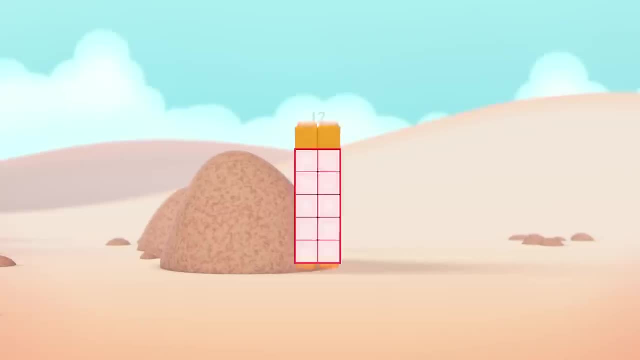 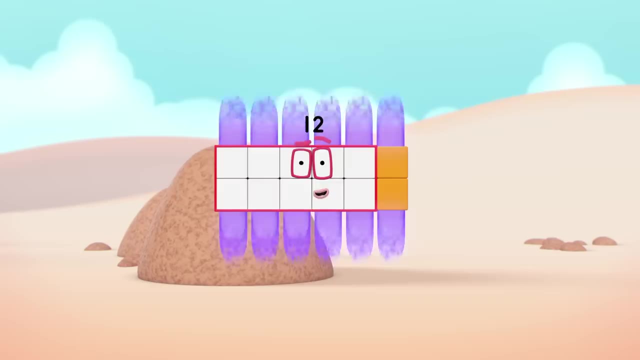 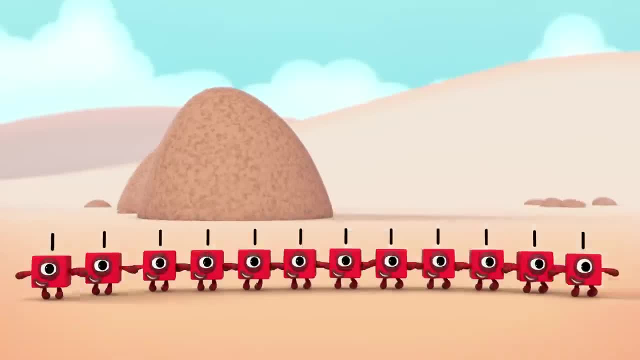 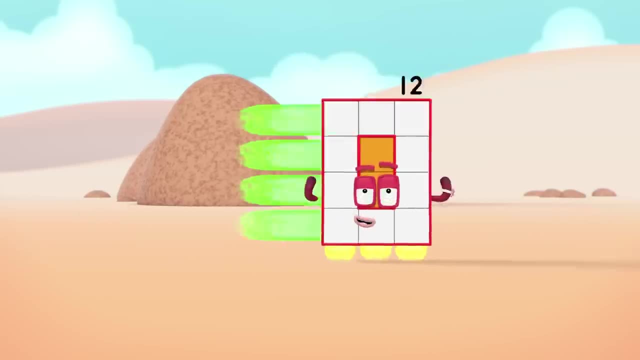 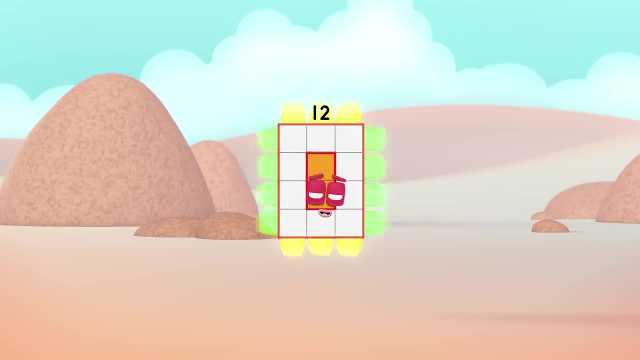 Six By two, Switch Twelve By one, Break away One, Two, Three, Four, Five. It's a new crease. to coin a phrase, You'll be in a daze when you fix your gaze on my amazing array displays. 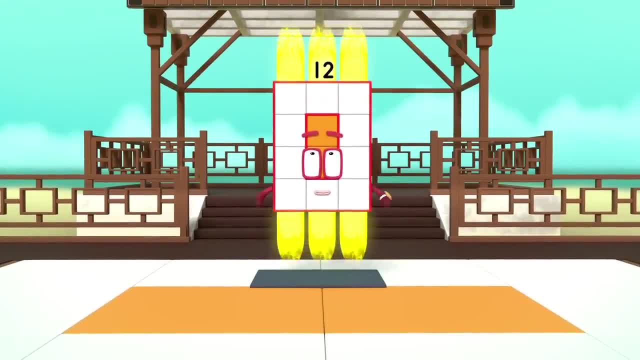 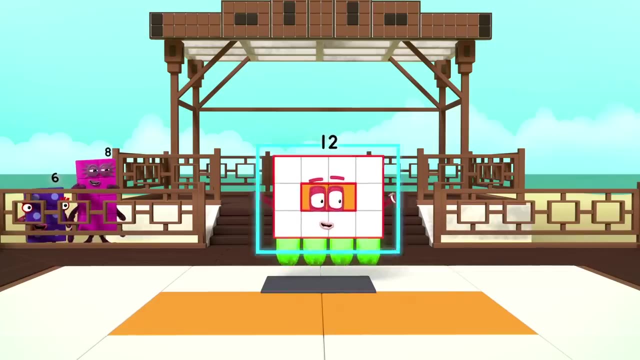 I am twelve. I am three by four. I am a rectangle Turn. I am also four by three, Ooh, Oh, And I am a super rectangle. I can take many forms, Switch. I am six by two Turn. 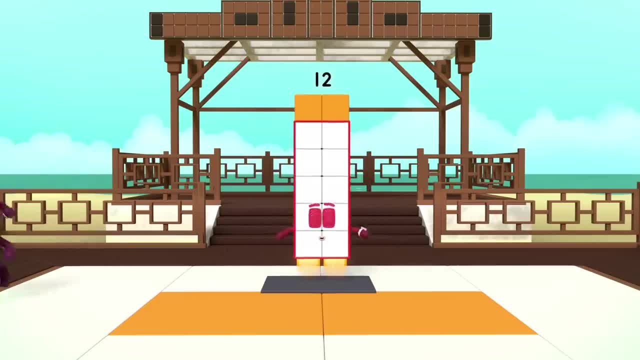 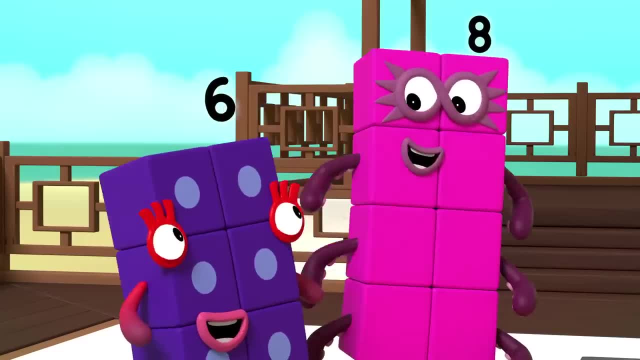 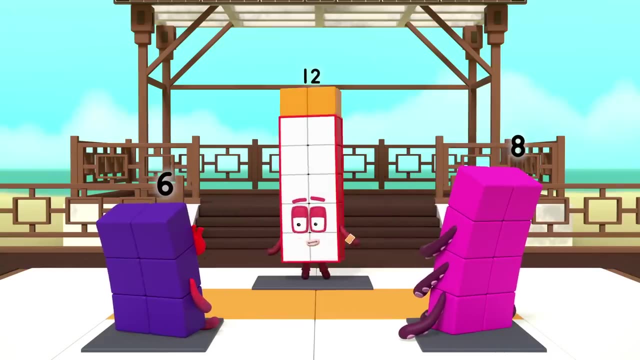 I am two by six. I am a rectangle. Welcome, my friends. Would you like to master the way of the rectangle? Oh, First you need to stand, so your front makes a rectangle shape. Watch, Tell me when I'm making a rectangle. 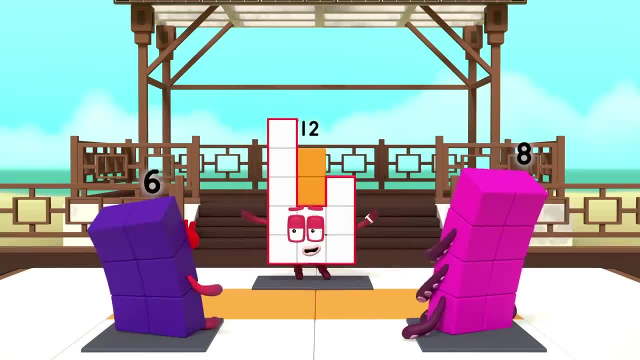 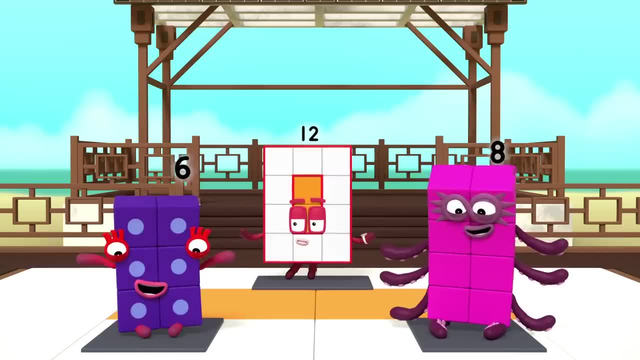 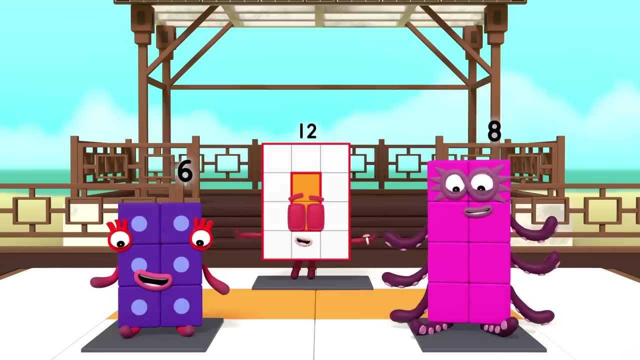 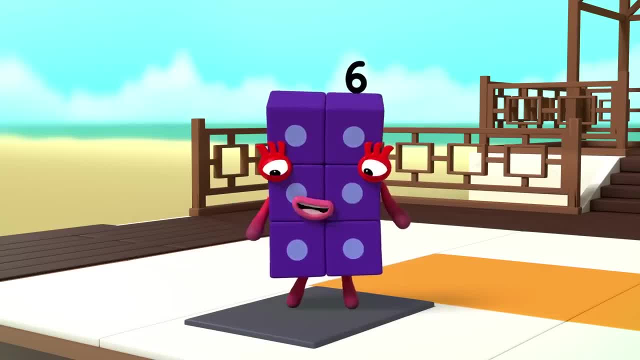 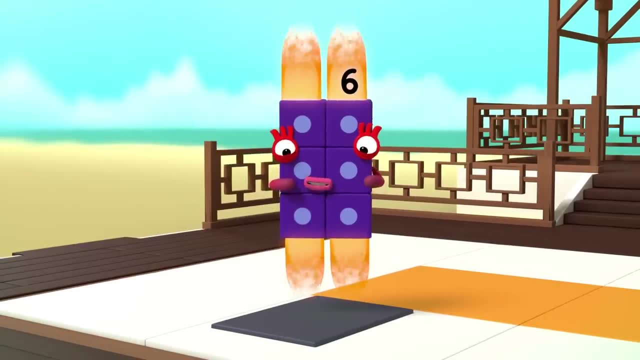 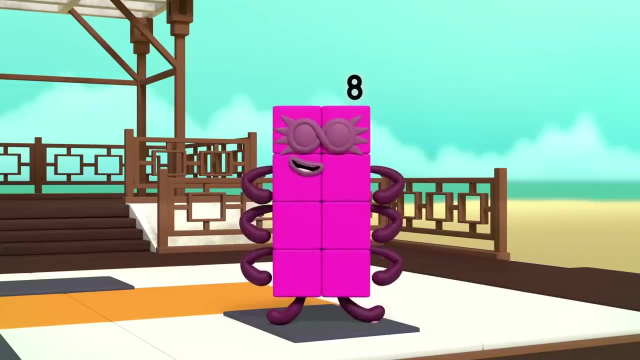 Your blocks are arranged in neat columns and rows. Now concentrate on how wide you are: Wide by three blocks tall. I am two by three. I am a rectangle. Hee-hee-hee Ugh, I am eight. I am two blocks wide by four blocks tall. 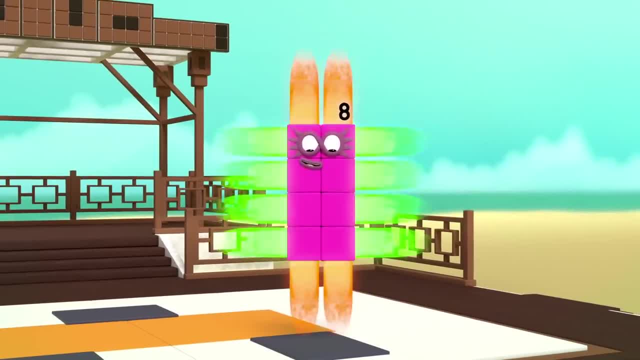 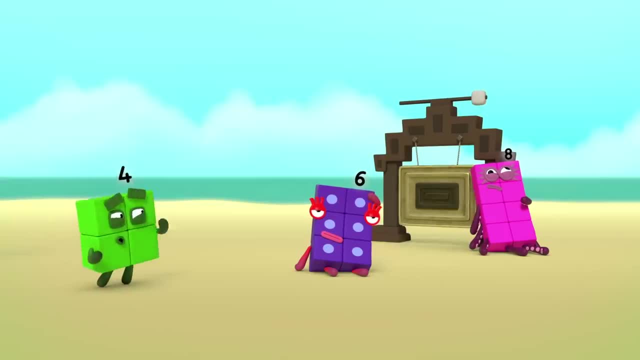 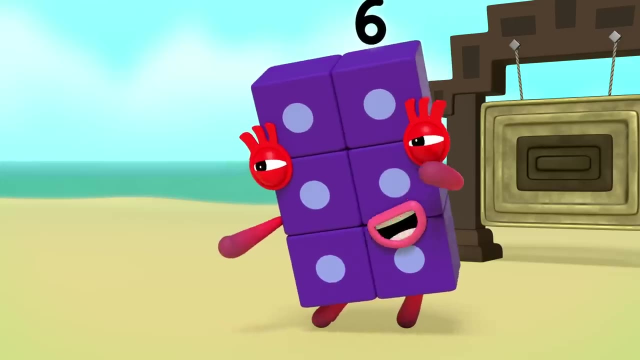 I am two by four. I am a rectangle Up, up and away. Whoa, Oh, Oh, Oh, Oh, Oh, my goodness, Have you heard a band? Are you okay? Six, I'm more than okay. 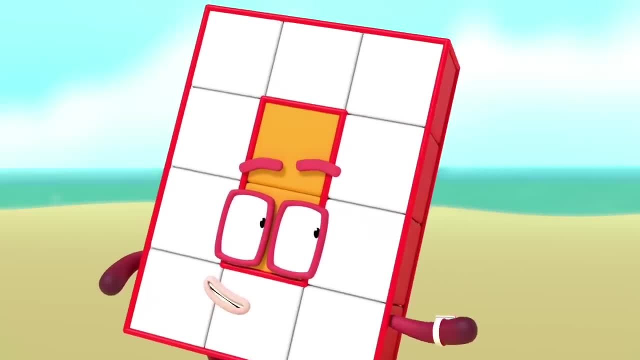 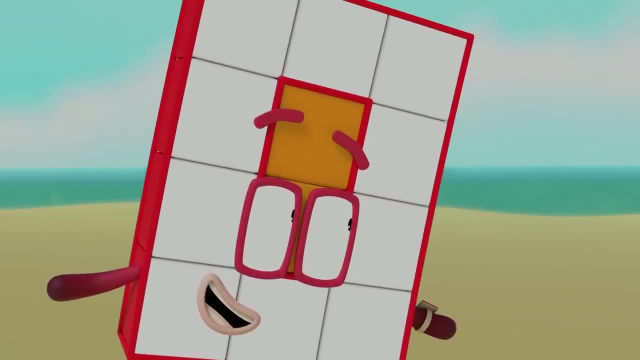 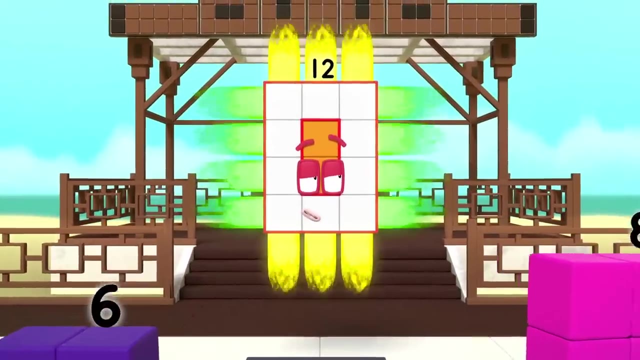 I've mastered the way. Hey, where are my rays? You need to concentrate. It gets easier with practice, So let's practice. It's time for the turn. I am 12.. I am three by four. I am also four by three. 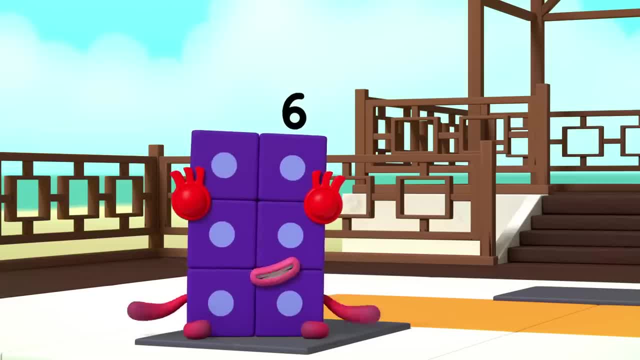 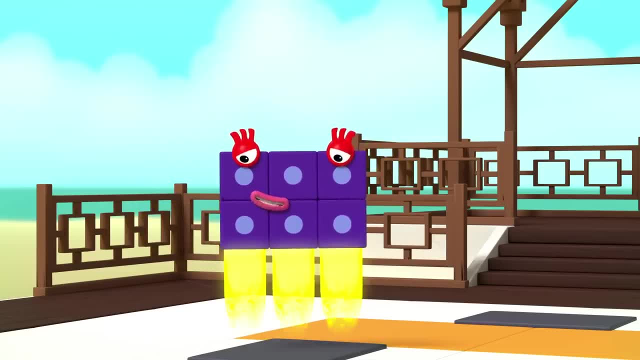 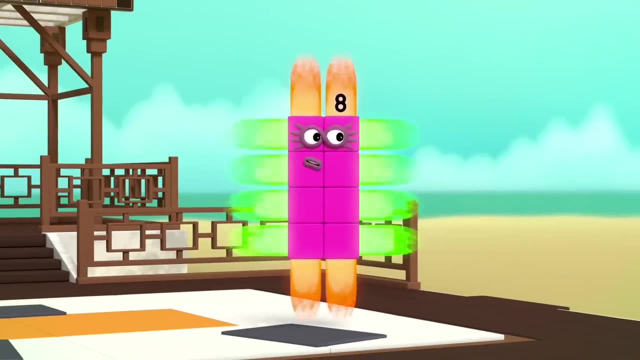 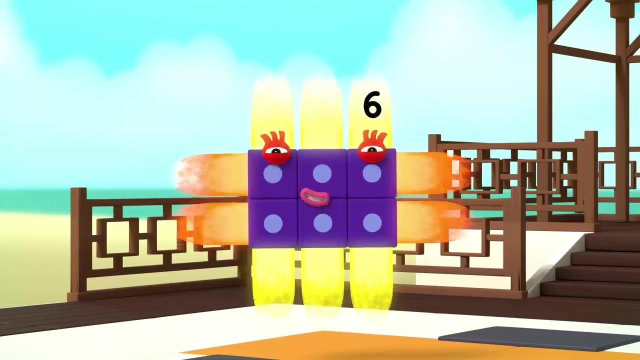 See, I am six. I am two by three, which means ten. I am also three by two. I am eight, I am two by four, which means octoblock turn. I am also four by two Turn. two by three. 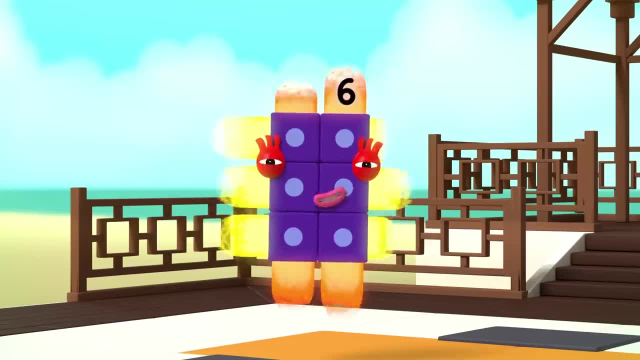 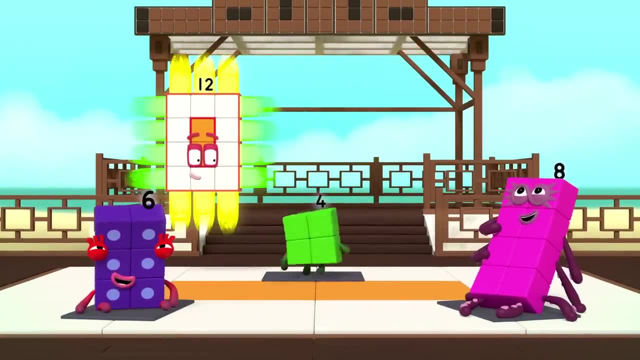 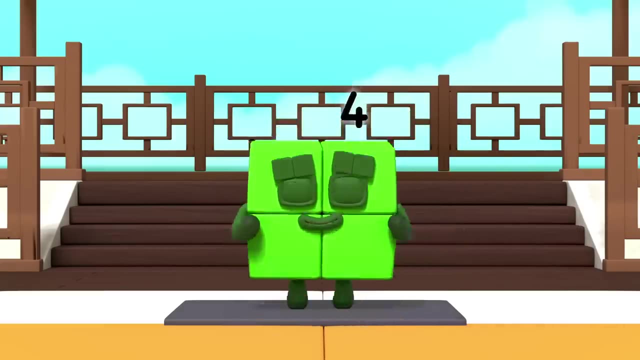 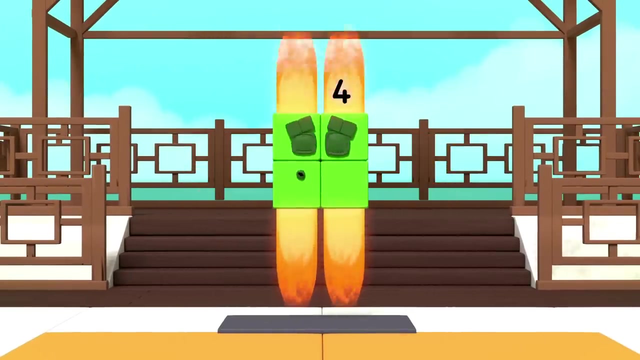 Turn three by two. Turn, turn, turn. Let me try that. I am four. I am two blocks wide by two blocks tall. I am two by two. Yay, And I am also turn Two by two. That's it. 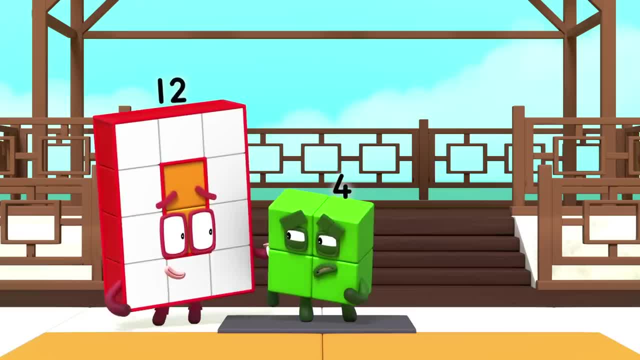 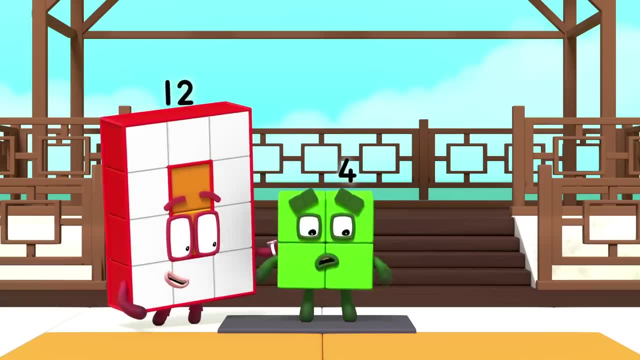 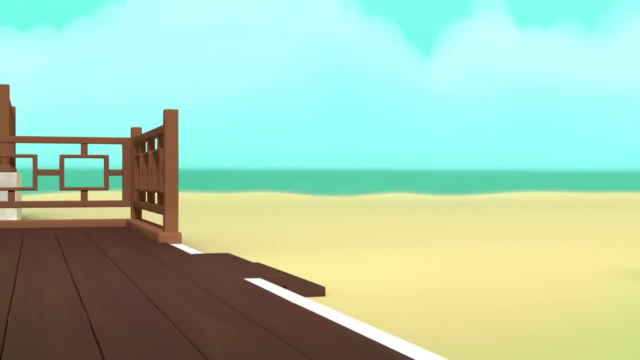 That's it. That's the same again. Did I go wrong? No Four, You're a special kind of rectangle that is the same number of blocks wide as tall A square, A square. Hey, hey, hey. What's all this? 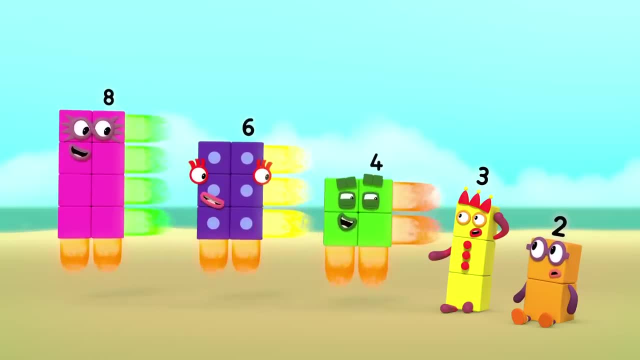 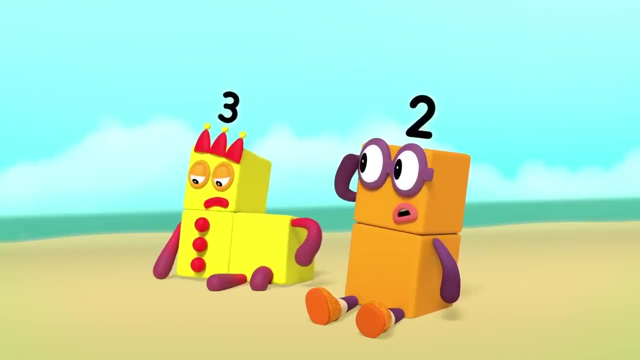 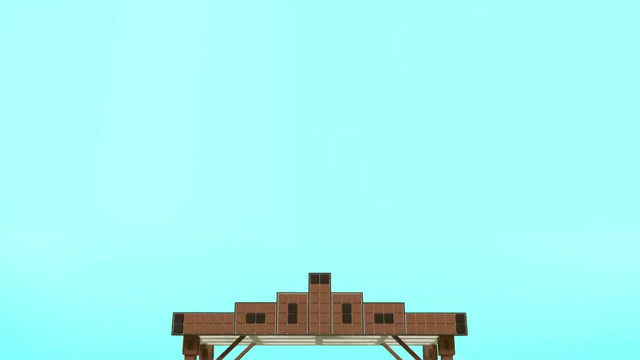 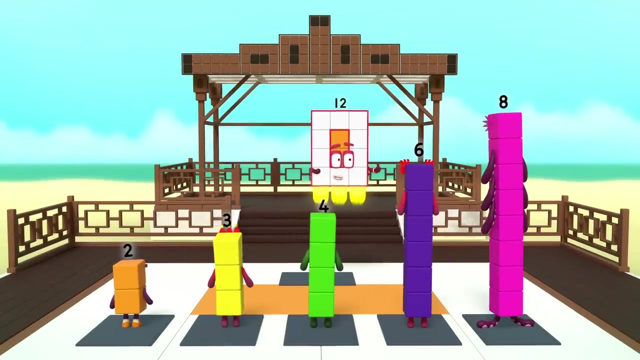 Look at us and be amazed. We all have rectangle rays. It's all right for some. I can. We can't make big, wide rectangles. Whoever said rectangles had to be wide? Oh, Number blocks stand tall. Now what shape are you making? 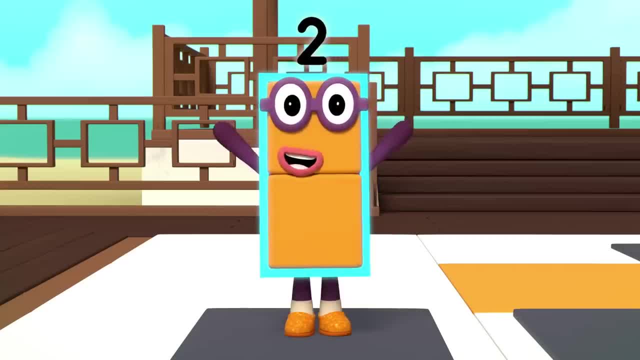 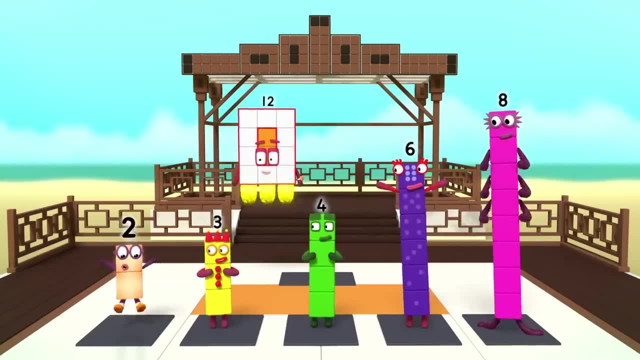 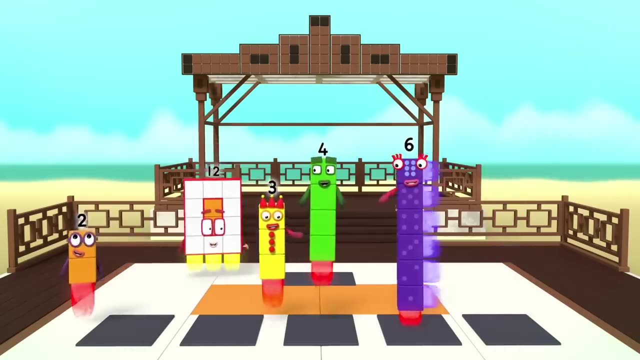 Oh uh, A rectangle, A tall, thin rectangle. I am one block wide And I am Two, Three, Four, Six, Eight Blocks tall. I am a rectangle- Three, Four, Six, Eight Blocks tall. 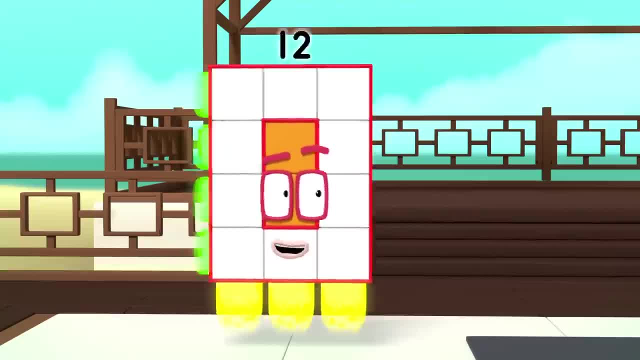 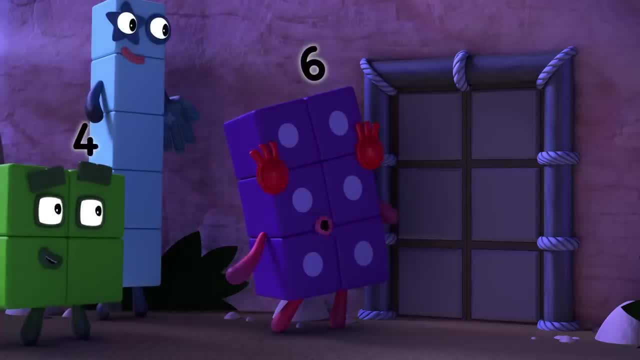 I am a rectangle. Maybe I shouldn't have told them Whee. Oh well, Too late. now Here it is, Right where Twelve told us The doors to Ray Canyon. I wonder why it's called Oh, Oh. 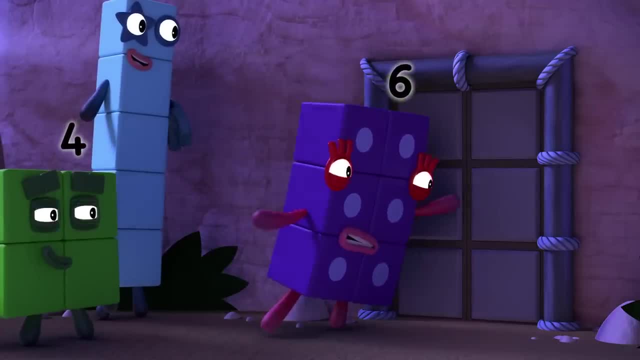 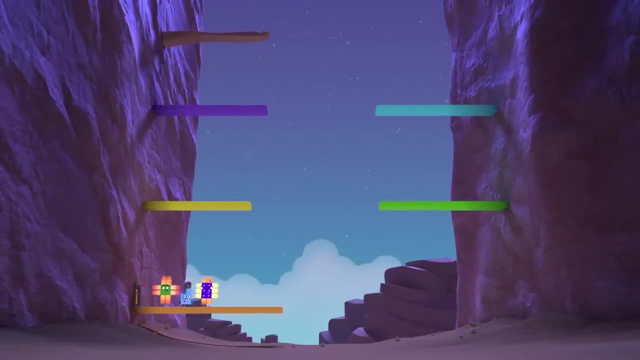 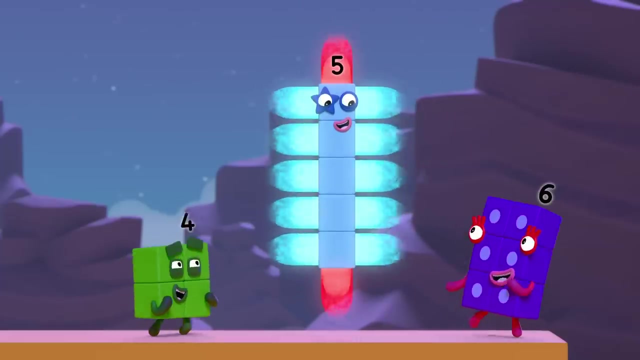 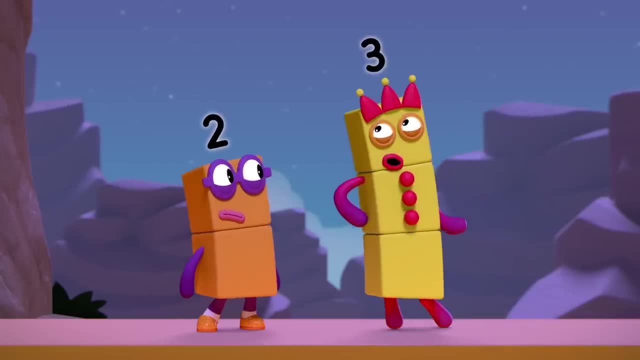 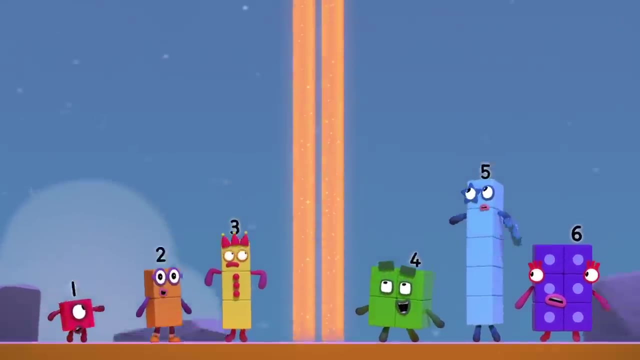 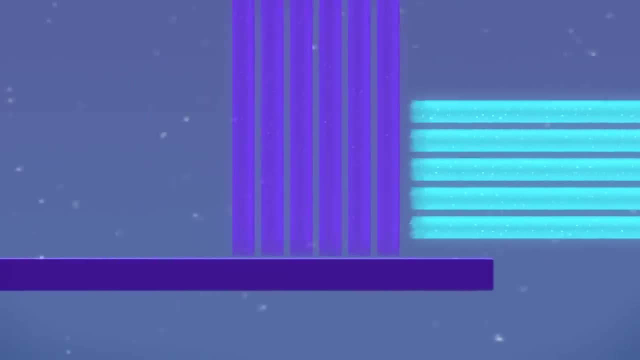 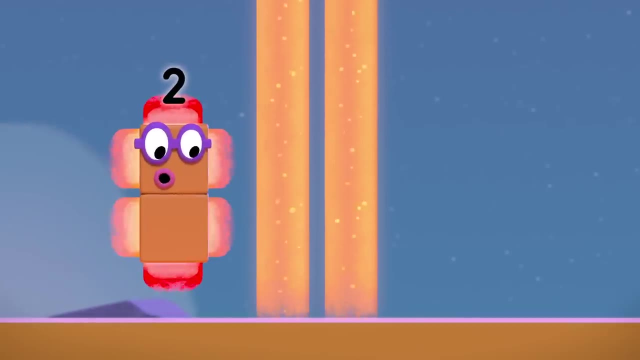 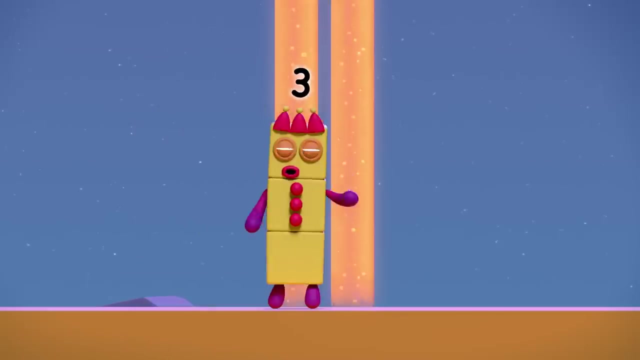 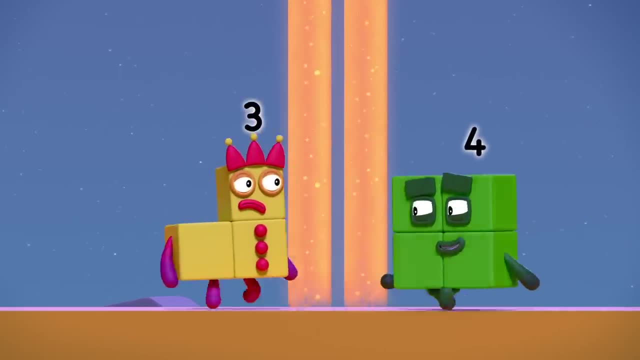 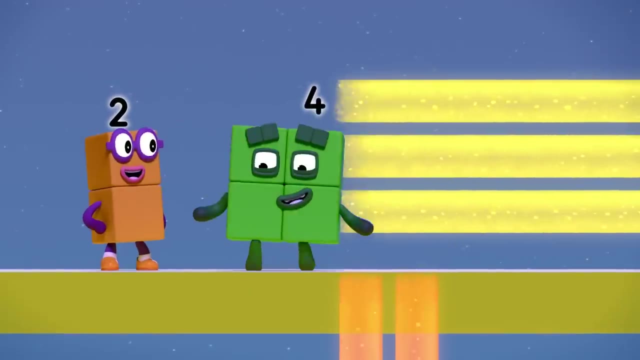 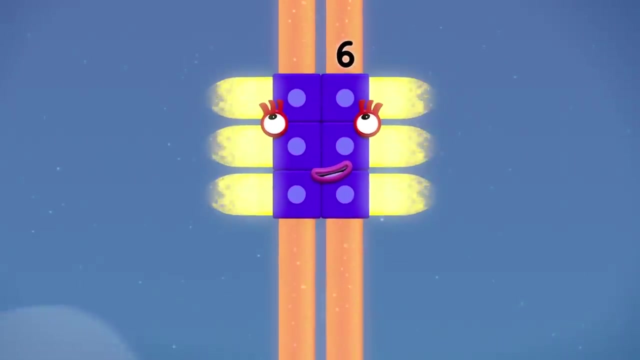 No, but I can. I'm a two-by-two square. If you think that ride is smooth, wait till you check out this move. Ooh Whoa, I'm two, lots of three. I've got two rays and three rays. 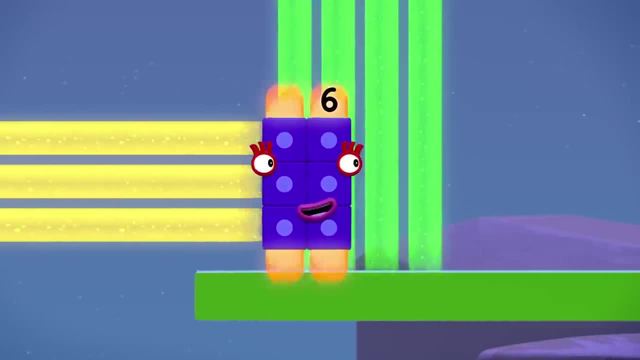 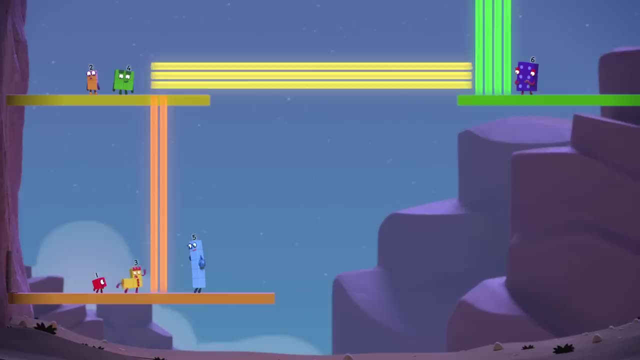 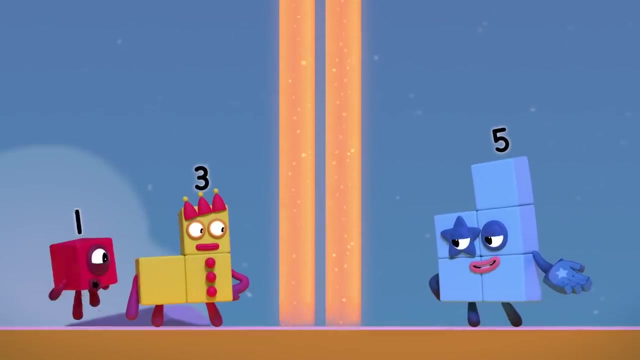 Ha-ha, I've got three rays too. you know, I could ride across just like Six if I could get up there. Hmm, Odd number, Oh, no, no, no, Numbers like us just can't make a rectangle. that's two blocks wide. 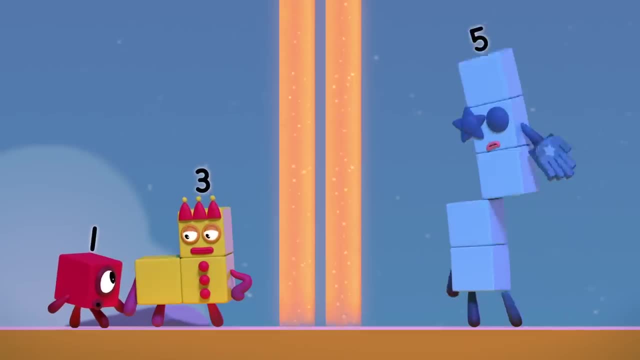 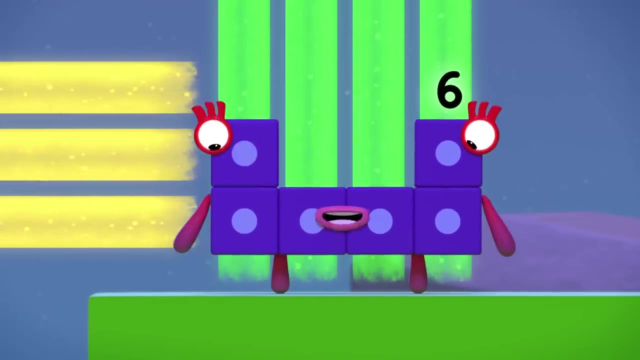 Twelve said only one of us had to get to the top. remember, We can all work together to find a way. I don't see how We're out of luck. I can't make four blocks wide. I'm stuck. I can, I can. 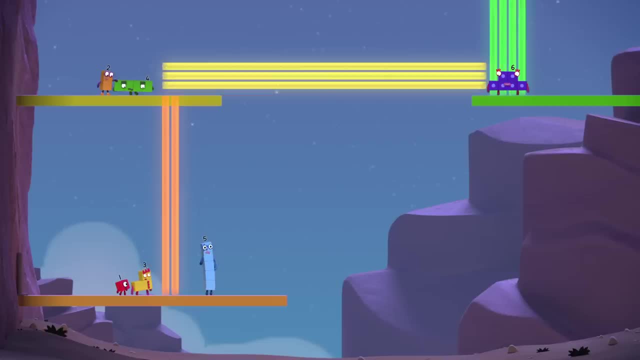 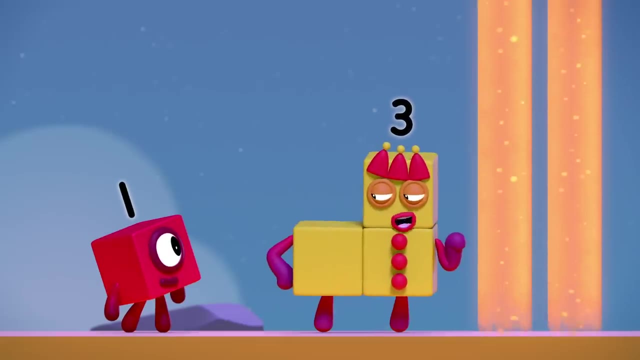 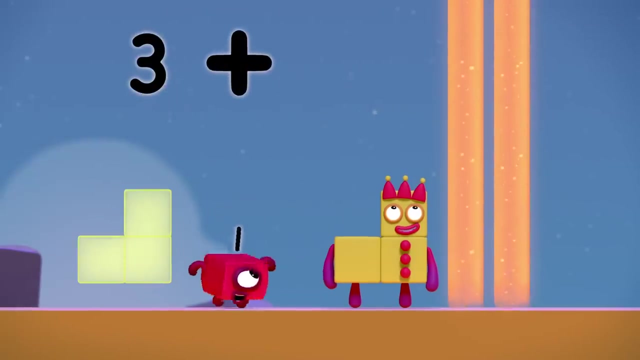 But I'm stuck here. We're all stuck. Twelve must have made a mistake. Wait a moment. Maybe there's more than one way to solve this problem. Sometimes you need to think round corners. Three plus one equals Four. Ooh. 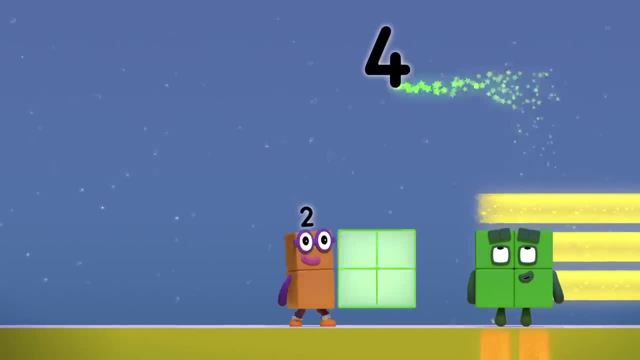 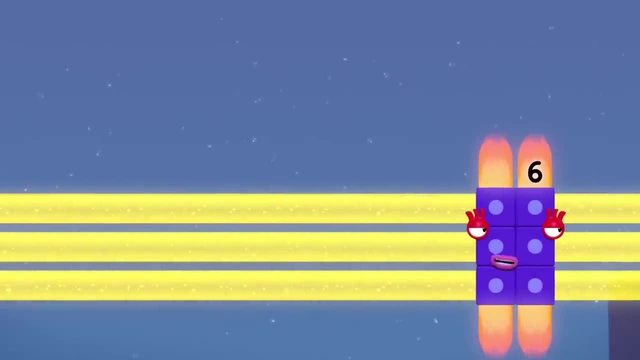 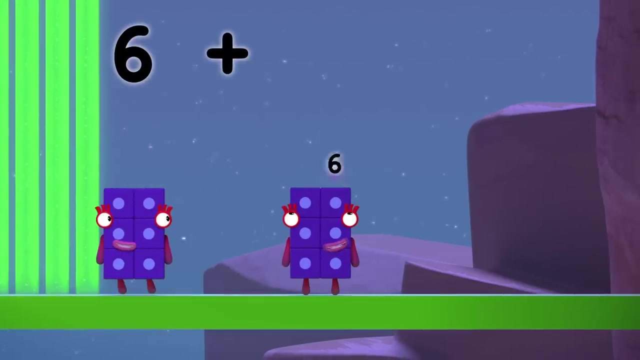 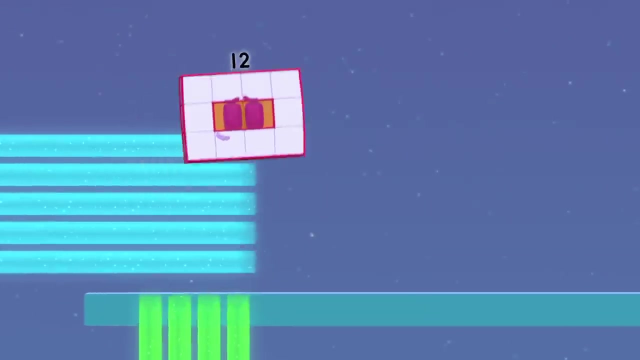 Ooh Ooh, Four plus two equals Six. I'm so glad I can reach this shelf, So happy I'm beside myself. Ooh, Six plus six equals Twelve. Oh, well done. Who came up with this idea? 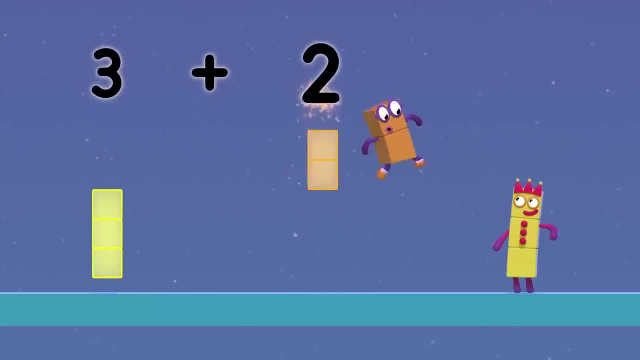 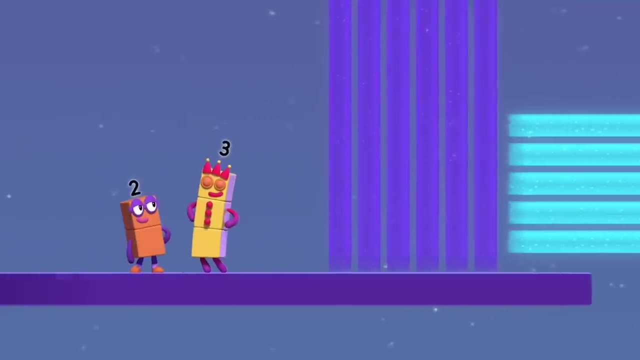 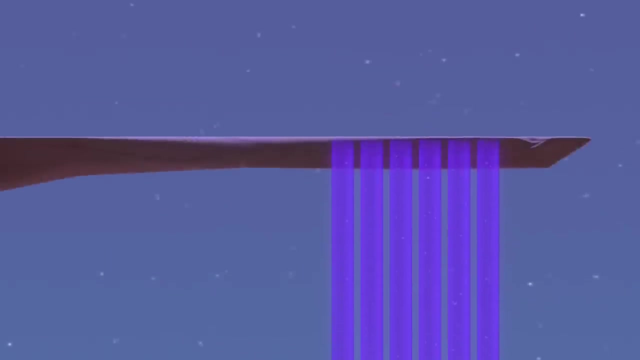 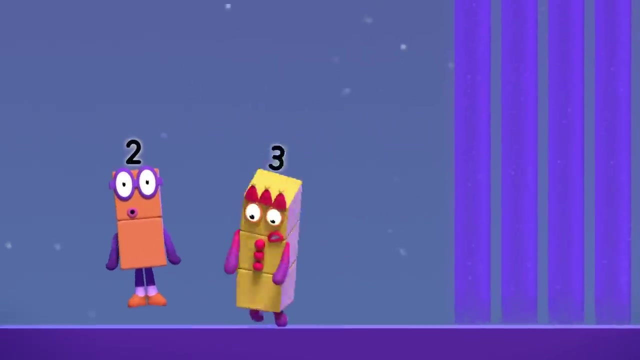 Me, me, me. Three plus two equals Five. Hooray, Yeah, Um, but how do we get up there? We can't make anything. that's six blocks wide. We've only got five blocks between us. Hello, my friends. 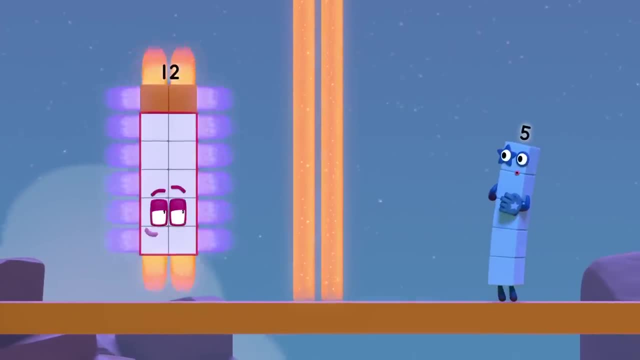 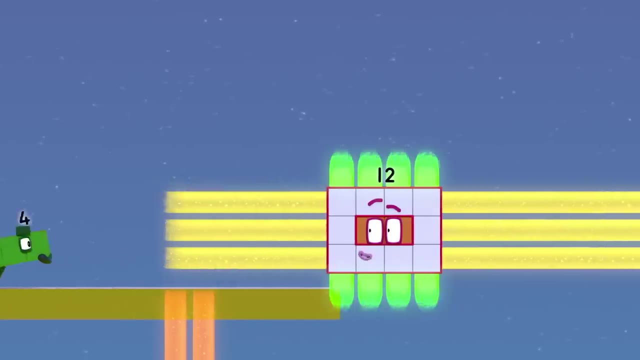 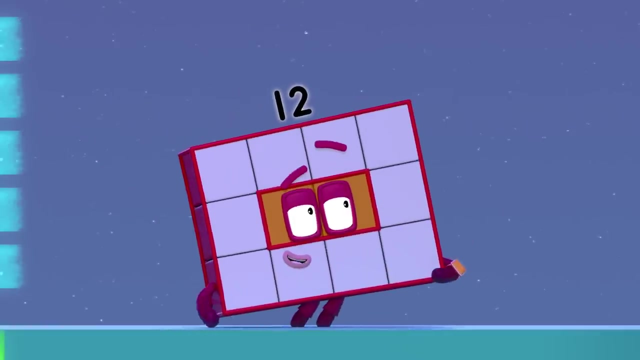 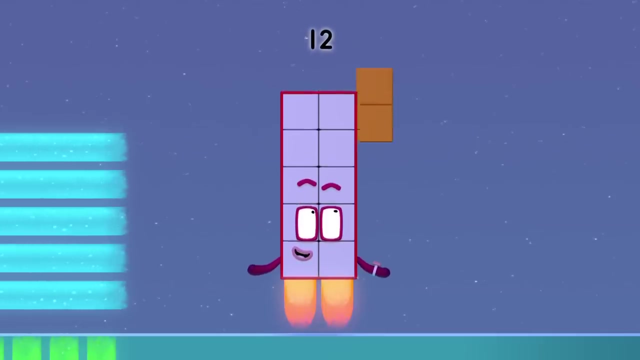 Twelve Switch. Congratulations on getting so far. Switch. By working together, you've nearly reached the top. What a super rectangle. But not even I can make every size of rectangle. I can't make a rectangle that's five blocks tall. see. 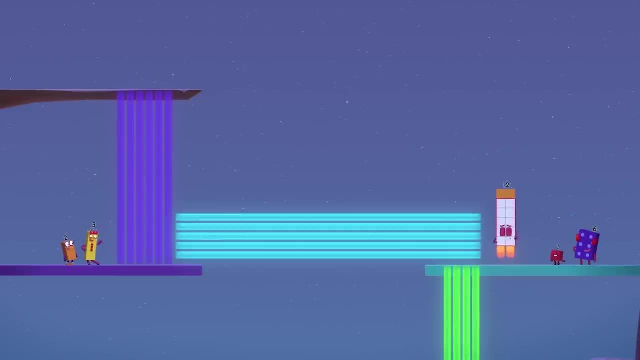 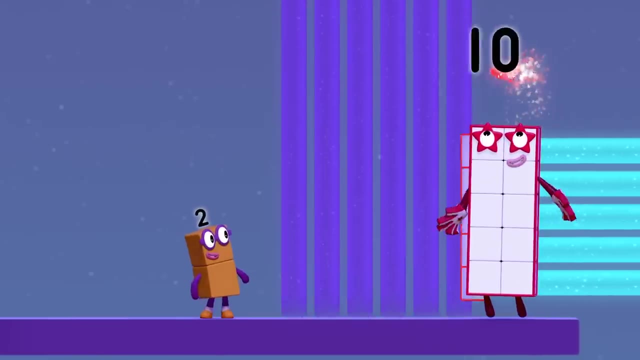 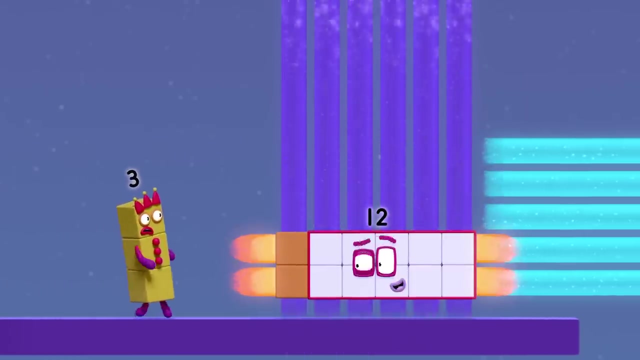 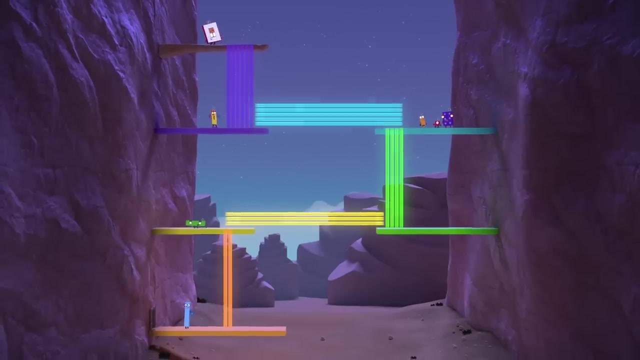 But, like you said, Three. sometimes there's more than one way to solve a problem. Twelve is ten plus two. Ten plus two equals Twelve Ten. I'll drop you a line. Hmm, What does that mean? Whoa. 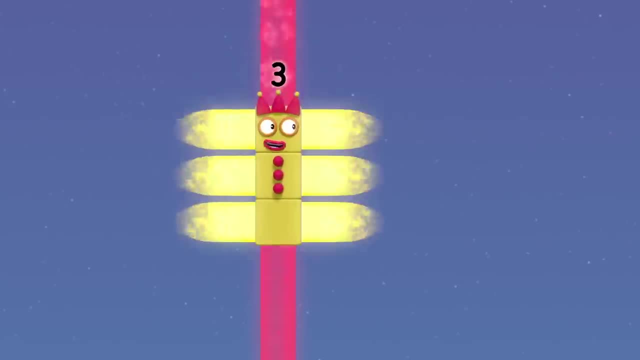 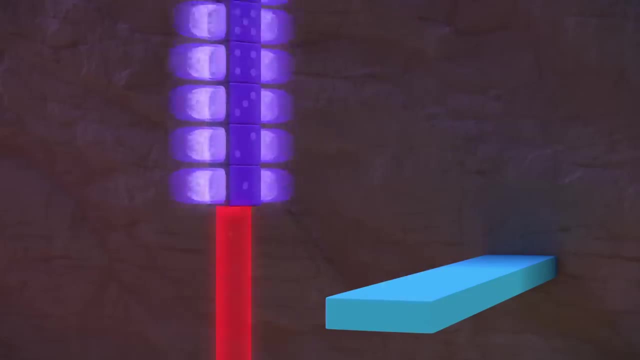 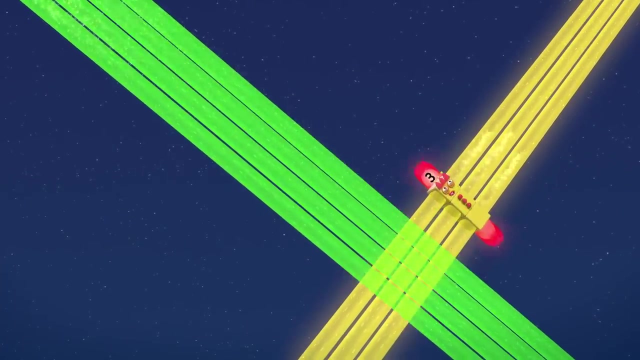 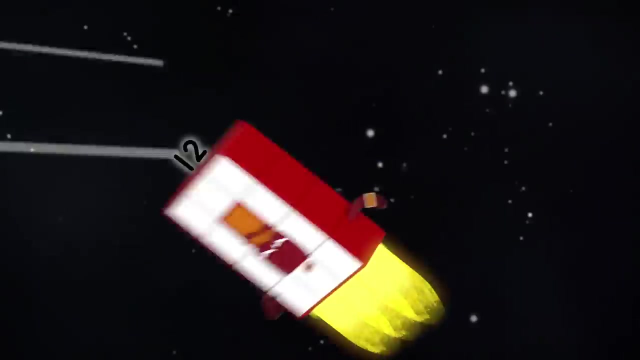 Ha-ha, Yeah, Whoa, Whoo-hoo, Woo-hoo-hoo, Woo-hoo-hoo, Whoa. Welcome to the race track. What do you think? I love it. MUSIC. Come in Number Base. 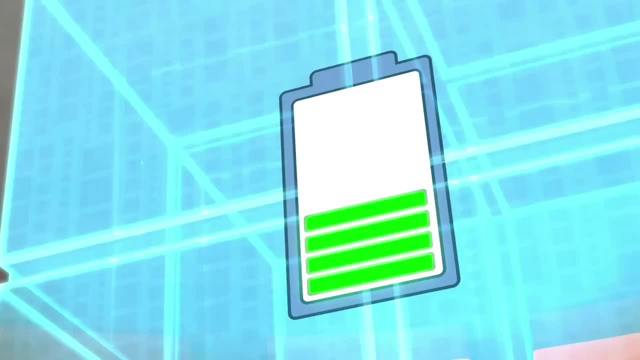 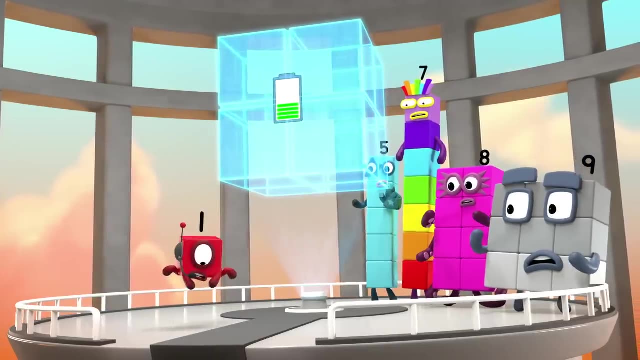 I'm in position, Careful 12.. The Blockstar's battery's running out. You need to change it before the whole thing drops out of the sky and smashes into Numberland. That block is no match for a super rectangle like me. 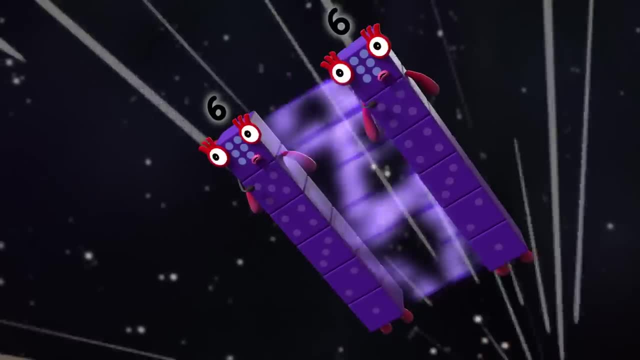 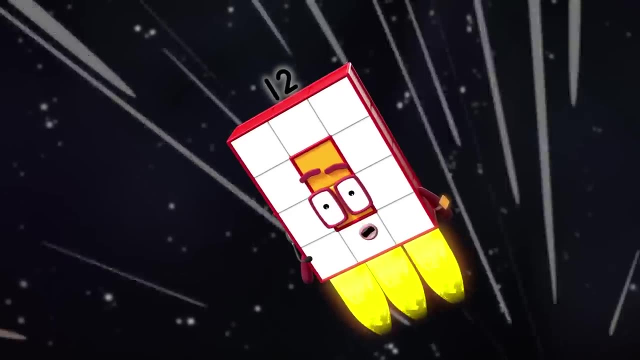 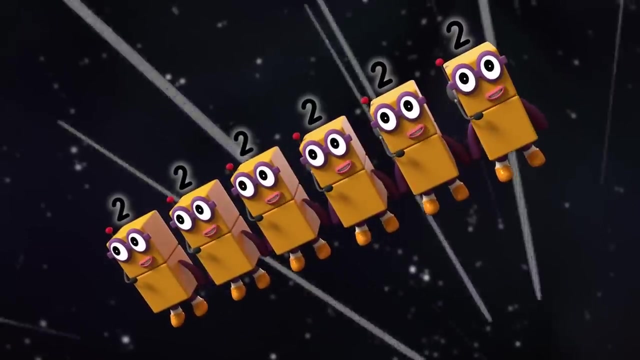 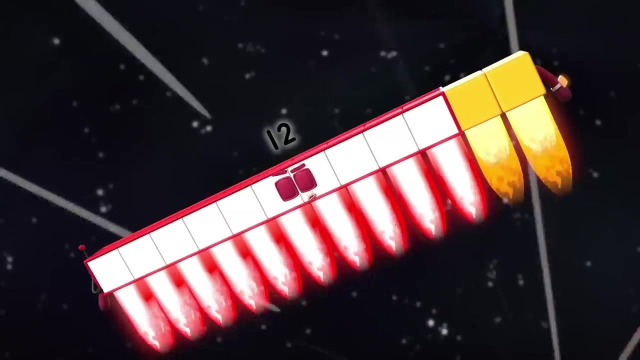 All teams report. in Switch. Two. sixes standing by Switch Three. fours standing by Turn Four. threes standing by Switch. Six. twos standing by Switch. Twelve ones standing by Switch. 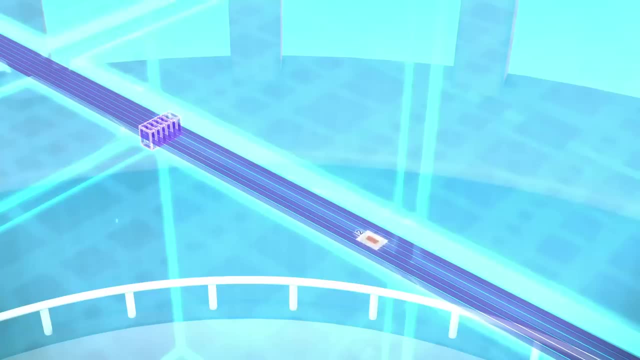 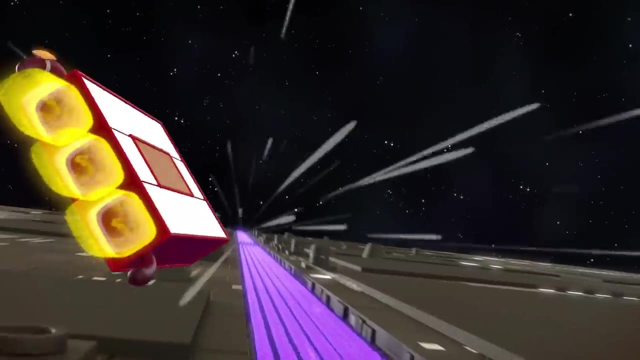 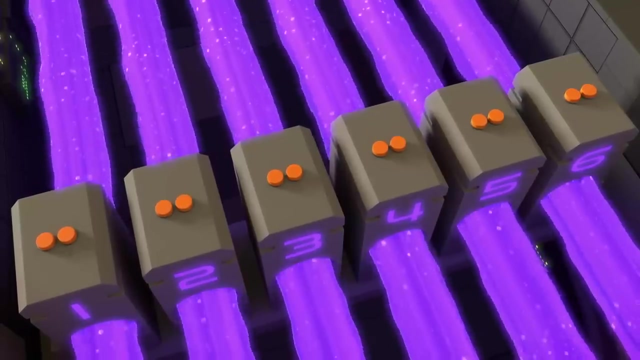 I'm going in. Hold on tight. You need to turn off the force field before you can get to the battery. Can you see a line of towers ahead? Yes, six of them. Each has two buttons on top. You need to press all the buttons. 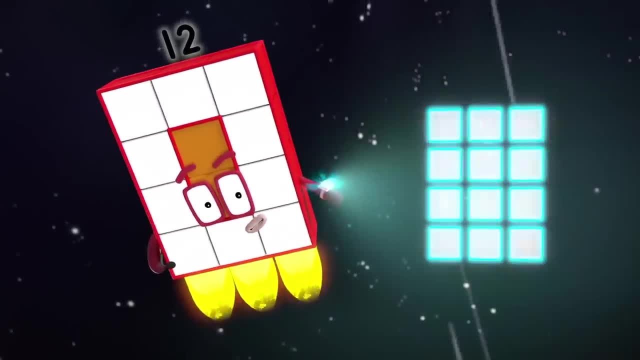 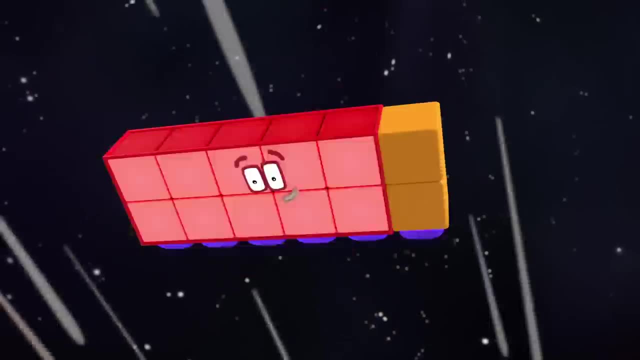 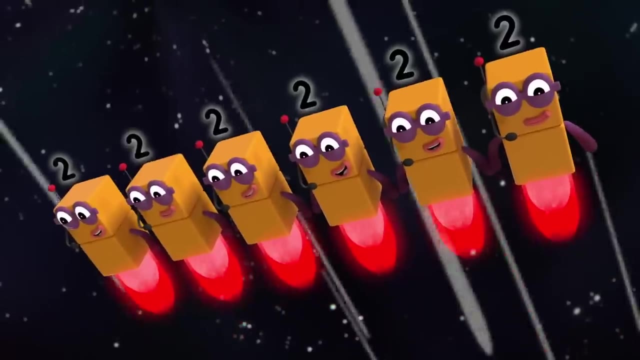 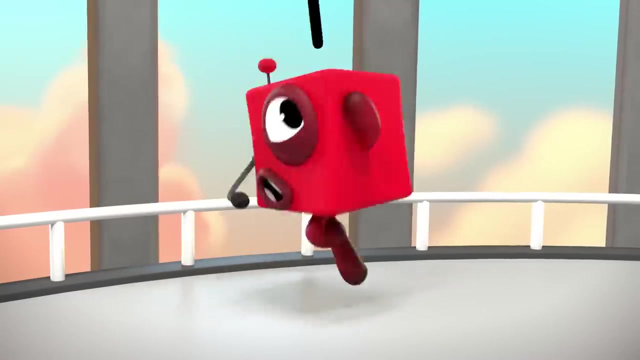 Together: Six towers, two buttons each Array display. This calls for switch Three sixes. Whoa Lucky, you've done it. 12.. Now head for that battery. There's no time to lose, I'm on it. 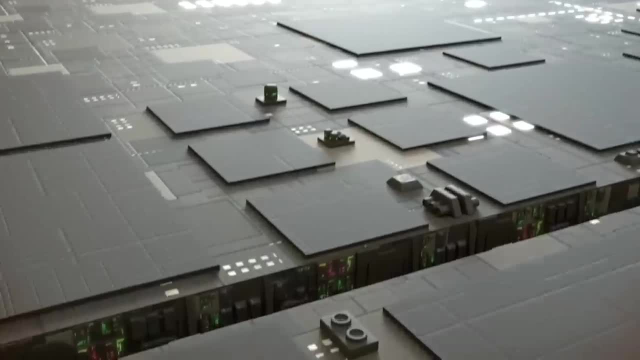 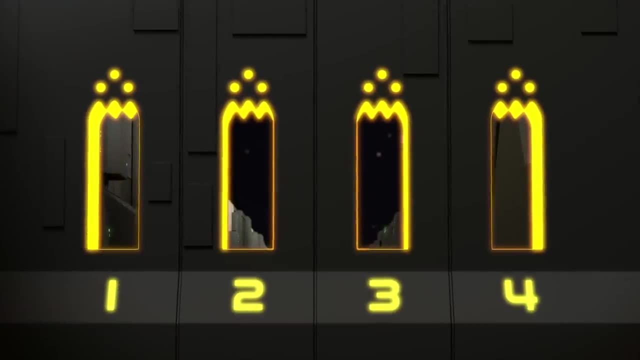 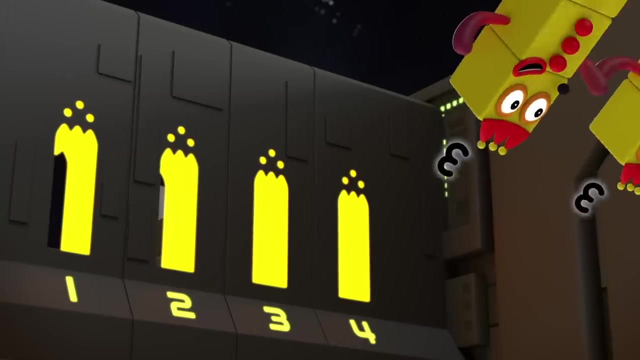 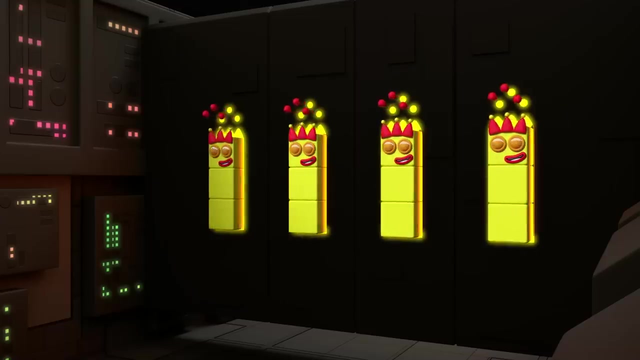 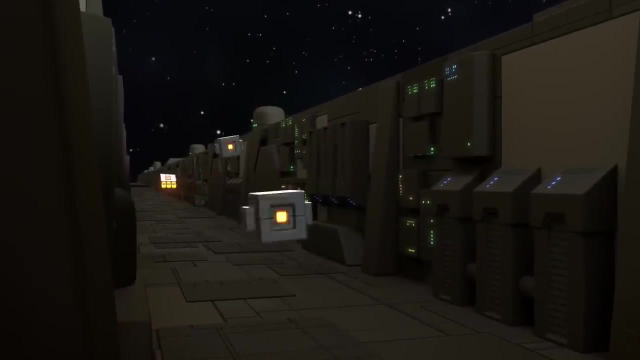 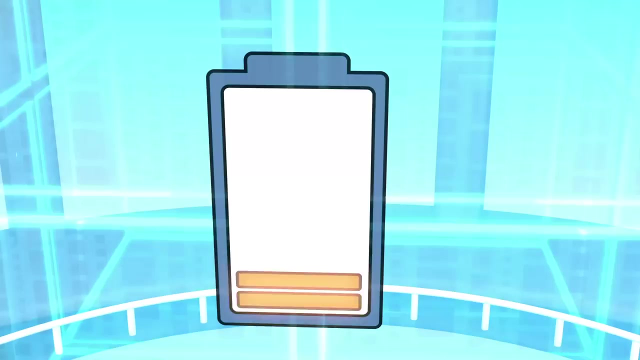 Switch, Indeed Roar, Pull up 12.. You are going to hit No time. Turn Four threes: Brrrrrr, Derp, brrrr, brrrrrrr. Woohoo, Those block ships have gone haywire. 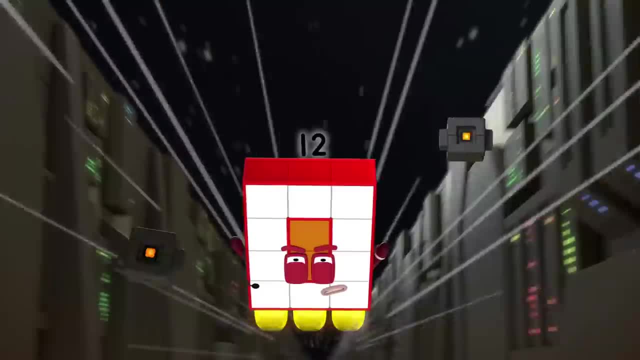 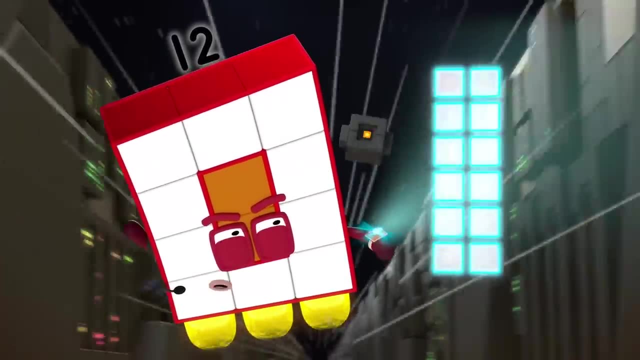 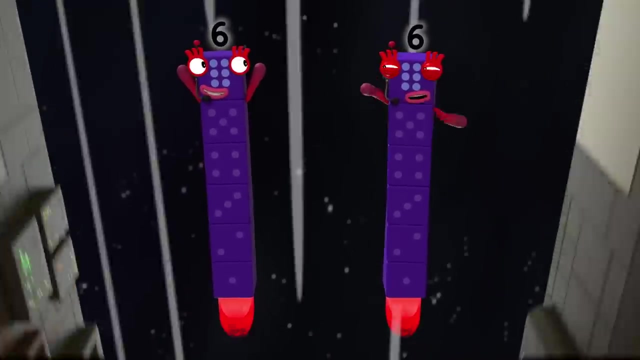 It must be the low battery. Don't let them slow you down. Woohoo, A latest play. I've got just the team Switch, Two sixes. We've got a great escape technique. Let's play a game of hide and seek. 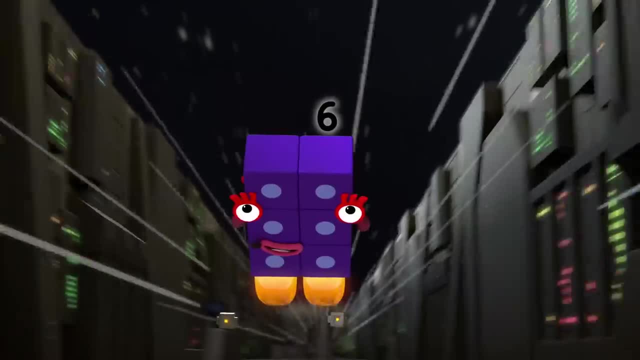 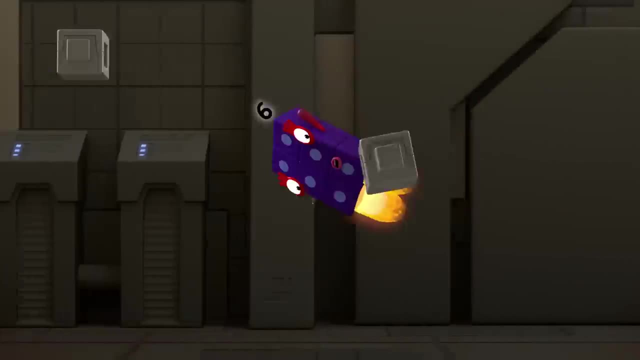 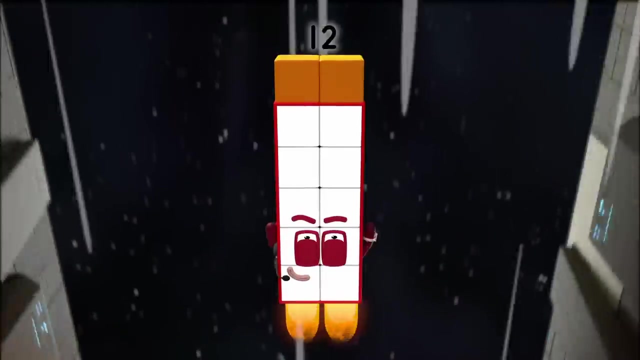 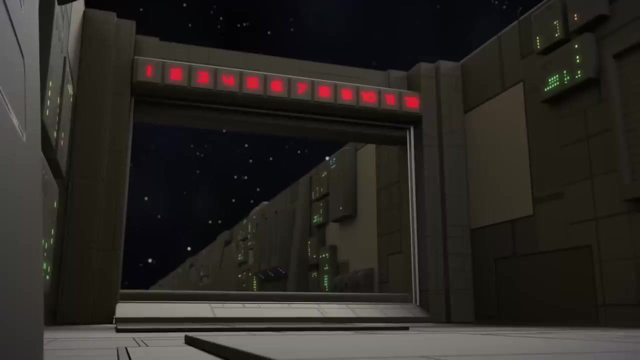 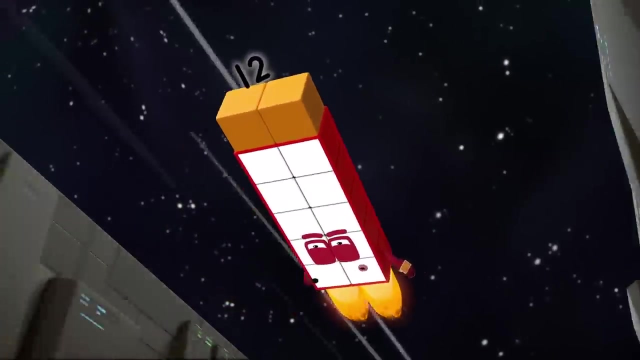 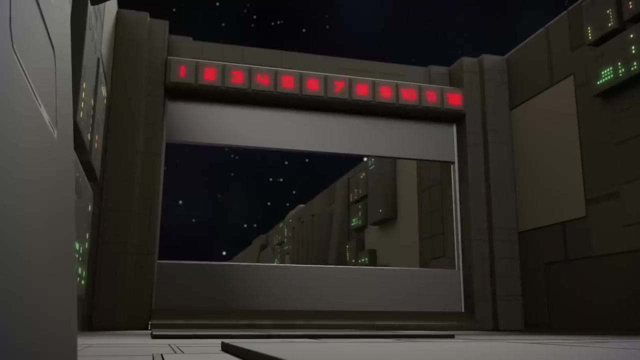 Switch. Catch me if you can. Ah, Whoa, I've got to lose them Through there. Oh, I've got a bad feeling about this. A razor's blade, Long and low Switch. Ah, Look out twelve. 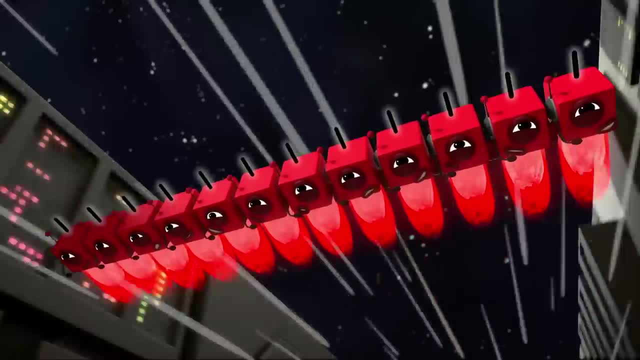 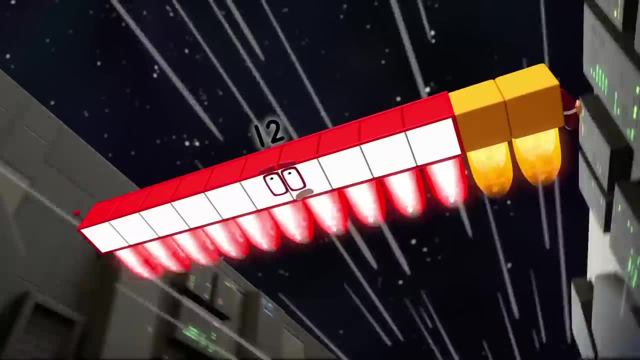 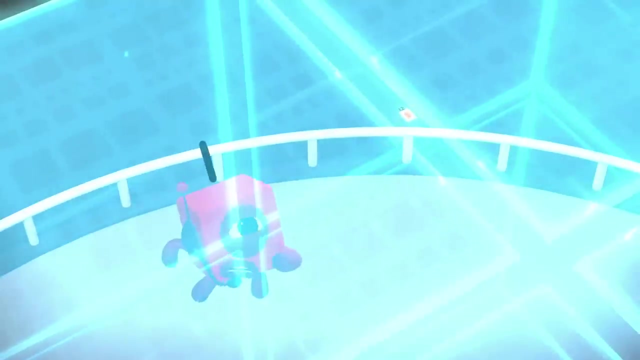 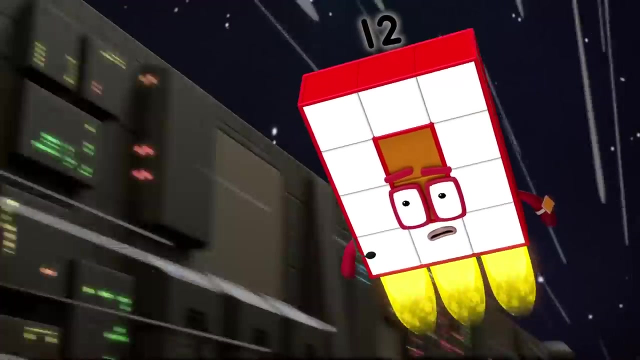 Twelve, what Phew. Wow, Battery level almost dead, but you're right on top of it. You need to open the cover, take out the old battery, then put in a new one as fast as you can, Phew. 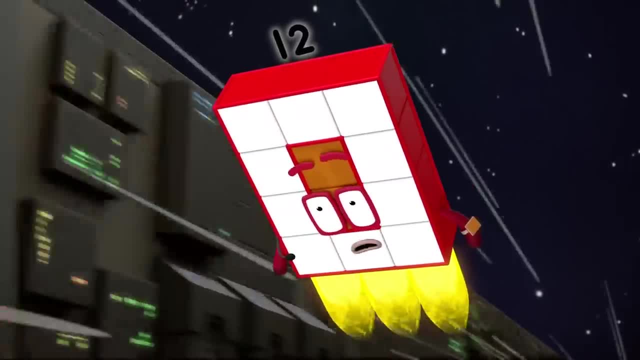 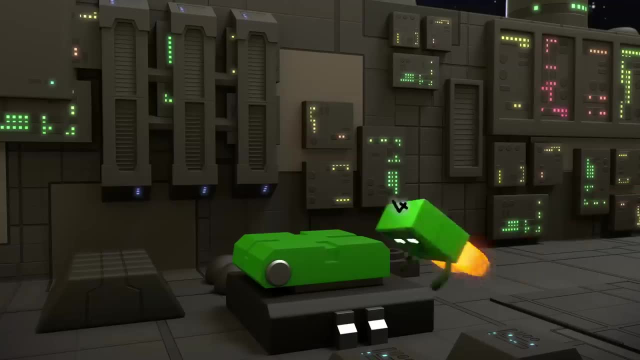 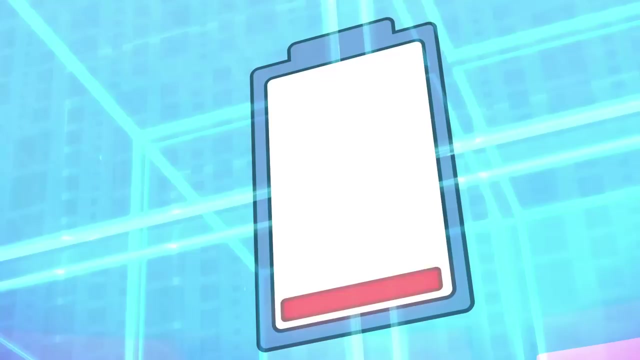 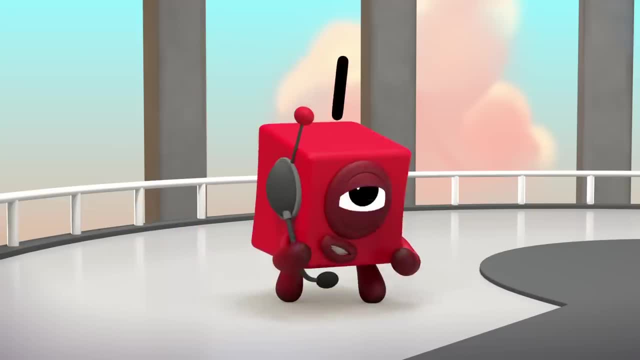 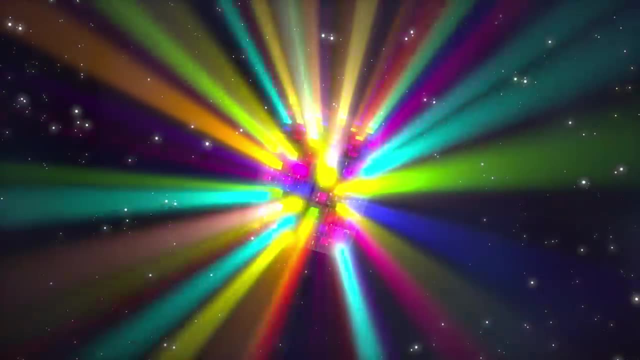 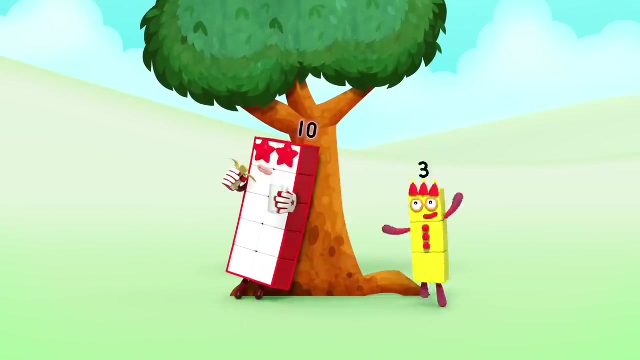 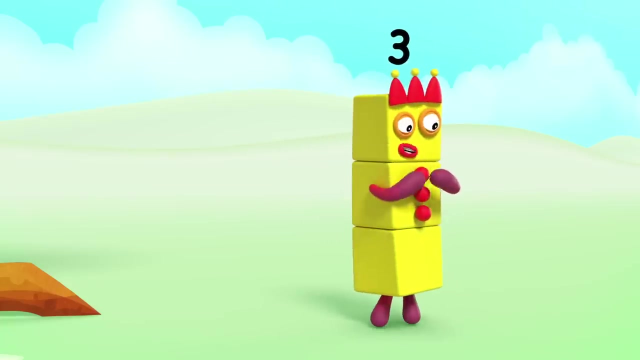 We did it, Oh, You did it. Now witness the power of this fully operational Disco Cube: Bum, bum, bum. Oh Three, Oh sorry Ten. I'm just so excited to show you my new trick. Ooh. 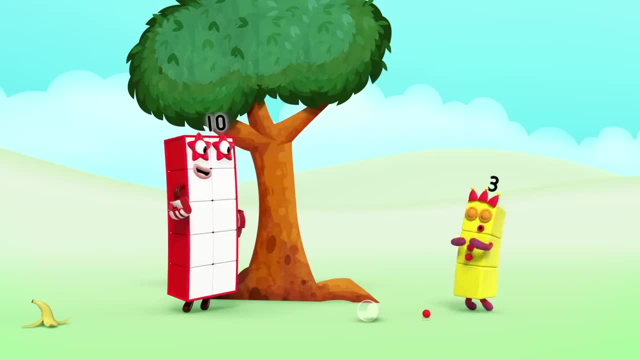 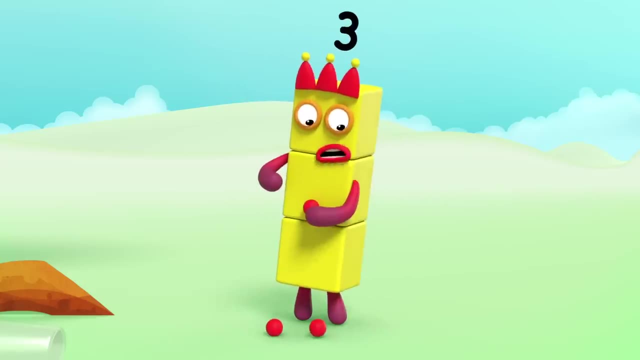 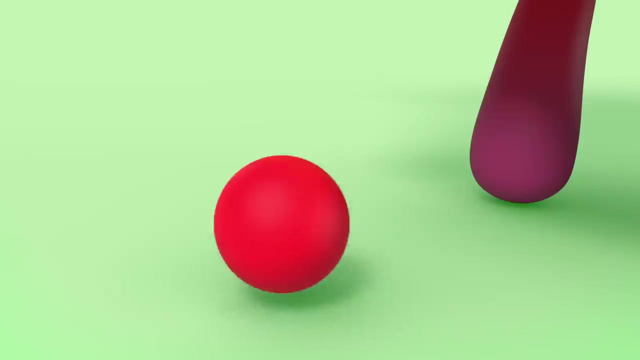 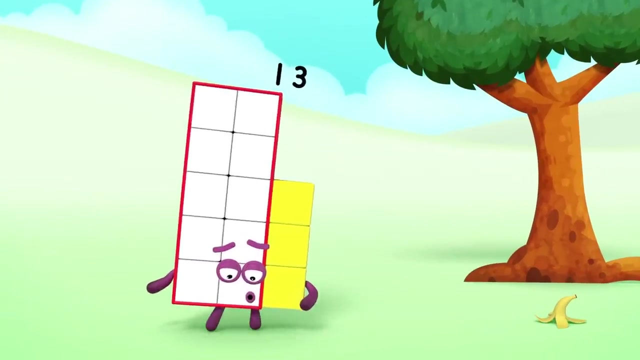 Oh, is that it? No wait, I'm not having much luck with my today. Oh no, My new trick: Ready, steady go, Oh unlucky. Oh hi, Who am I? What are you doing here? 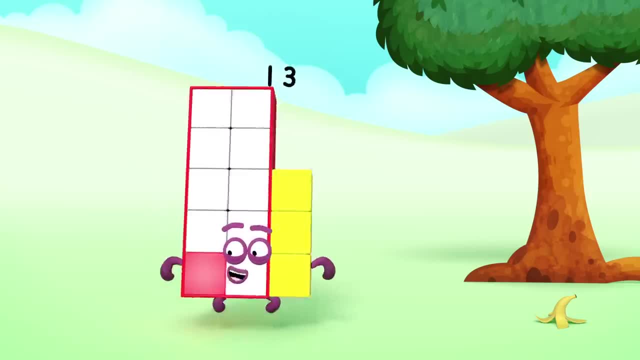 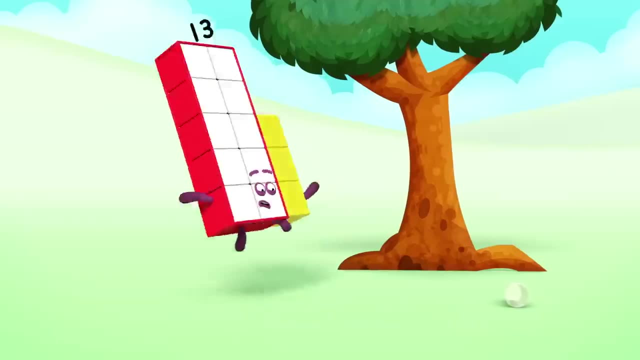 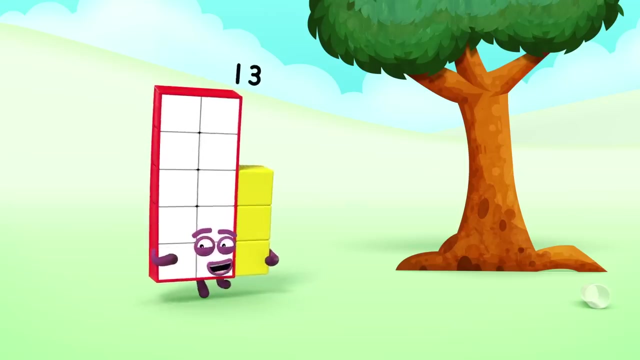 Hi, Who am I? I'm one, two, three, four, five, six, seven, eight, nine, 10,, 11,, 12, 13.. Whoa, Wow, Whoa, Oh, my three fell off. 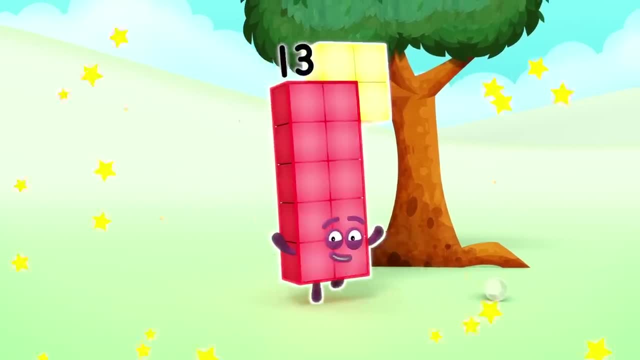 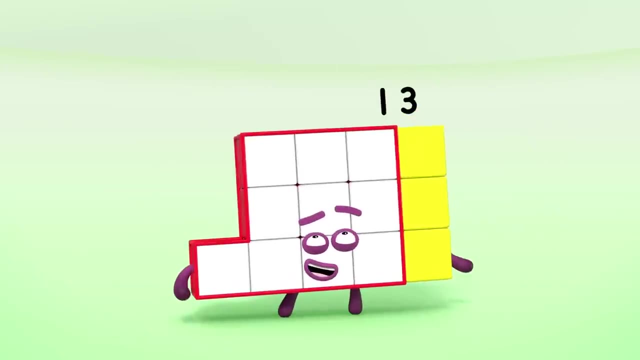 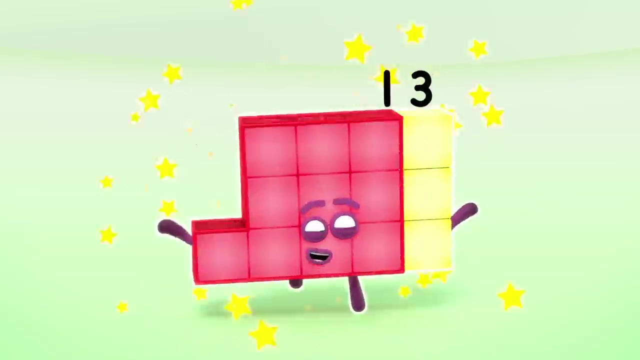 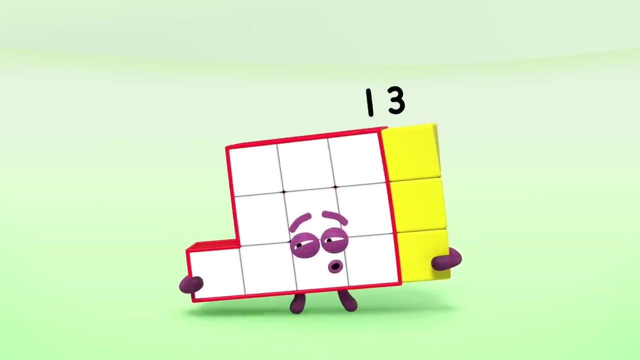 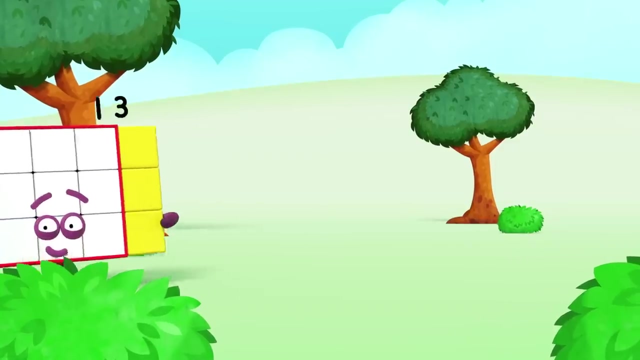 Never mind, I am 13.. Oh, whoa Unlucky. Try again, I am 13.. Hooray, Hooray, And I think I might be a little bit unlucky. This is me. ten and three. 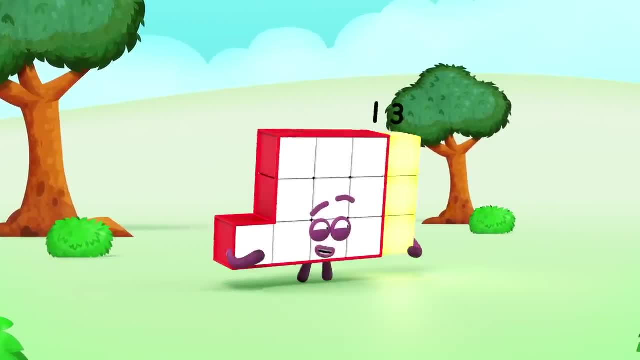 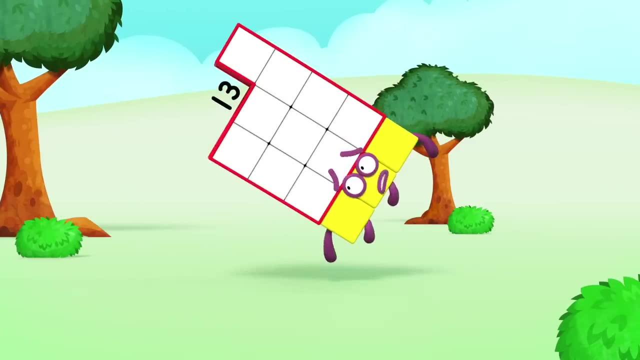 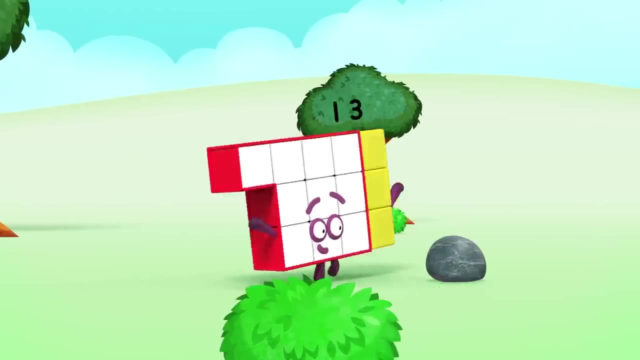 Expecting to run out of luck. Sorry, It's all jolly japes. when I'm out of luck, I'm so lucky. Sorry, When I get into scrapes I'm always coming unstuck. I'm the clumsiest number you've ever seen. 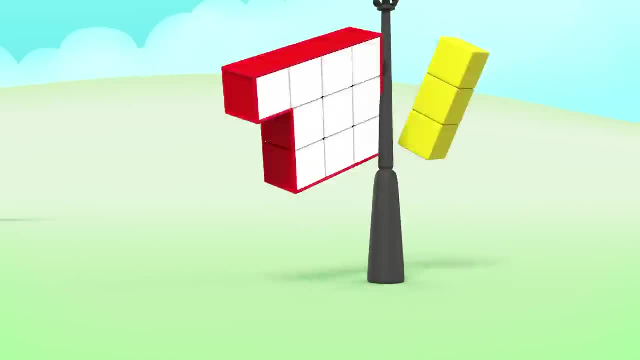 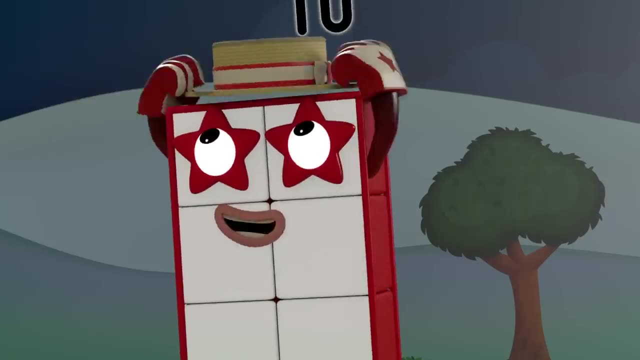 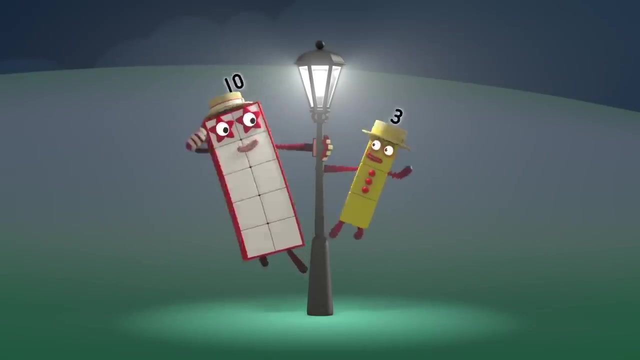 Unlucky number 13. Oh, It's happened again. A three and a ten. Somebody should tell. if not, it's happened again. I don't have the heart to be fussy or picky, But he's falling apart. He's a bit unsticky. It's happened again. 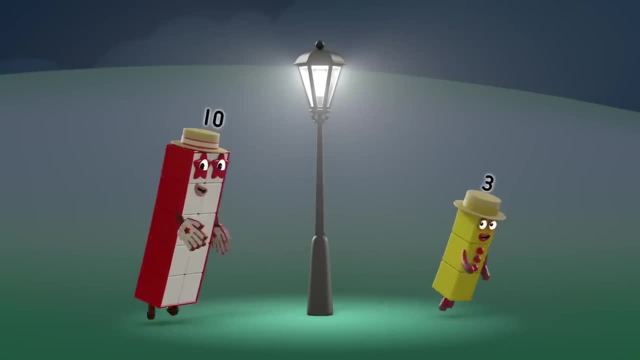 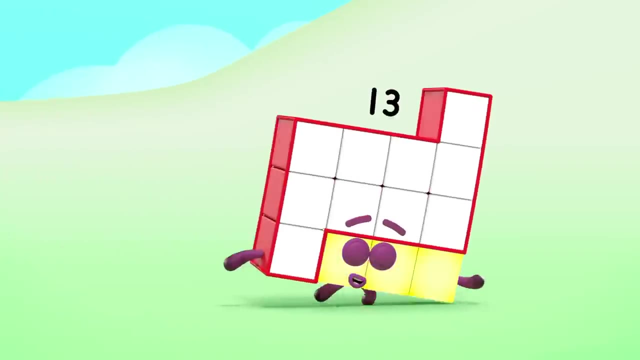 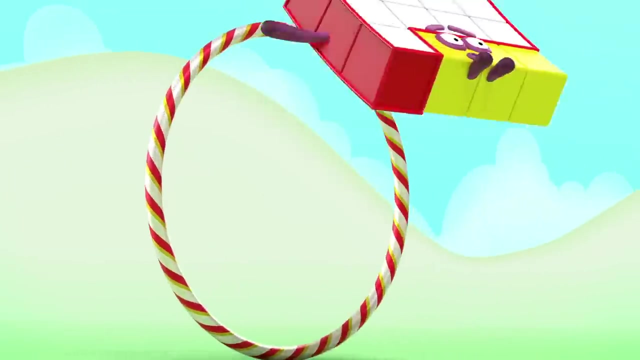 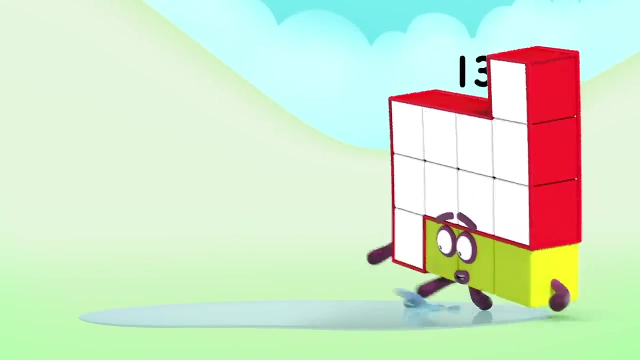 And no-one knows when. So far, we should tell him that it's happened again. Me again. Three and ten Expecting to fall down a hole. Ha, I jump through a hoop And step in the puddle. That seems to sum up my role, And wherever I end up, I might have seen. 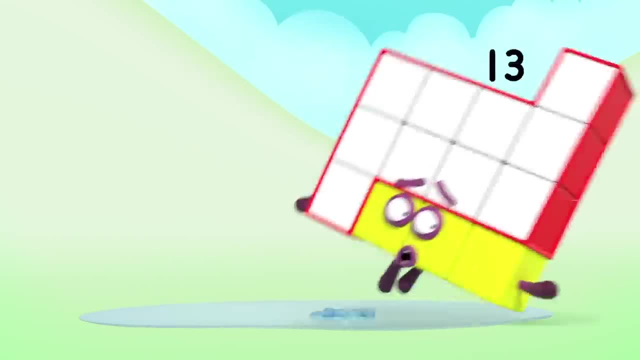 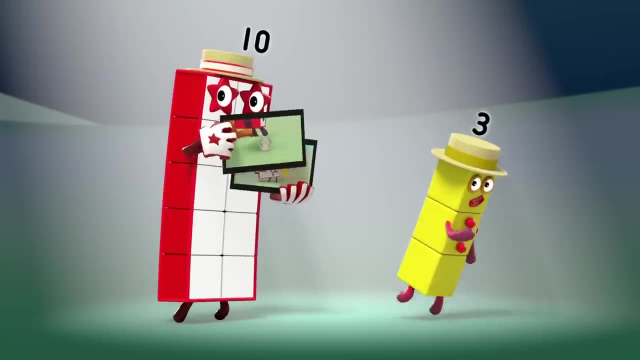 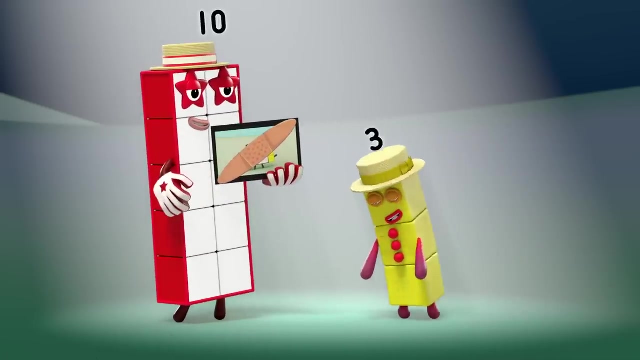 Unlucky Number 13. Oh, It's always the same When he says his name. Somebody should tell him that's the name of the game. It's happened before A total disaster, But he's going to need more than a sticking cluster. It's always the same. 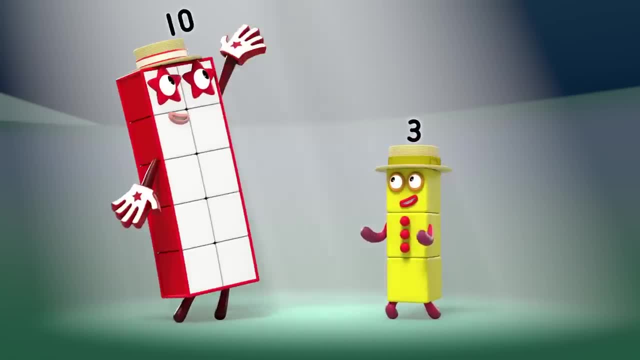 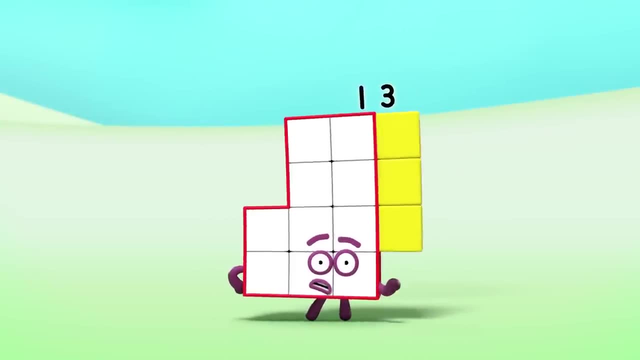 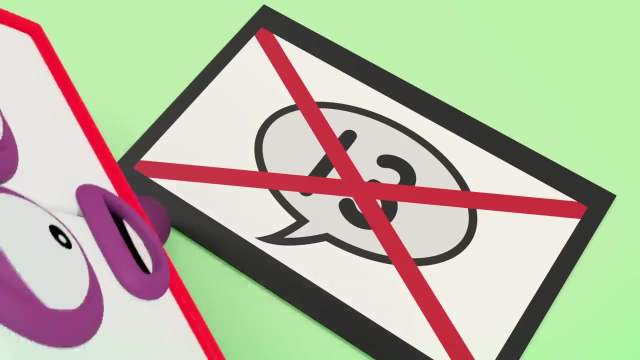 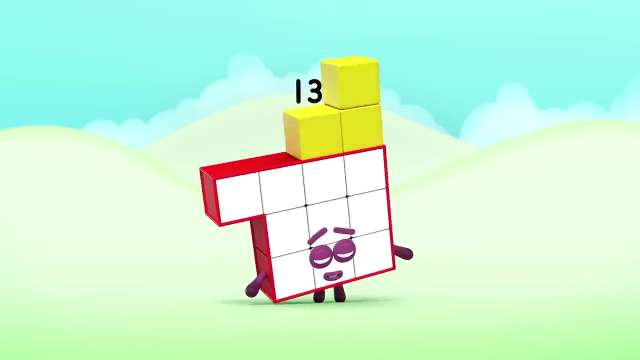 We know what to blame. Somebody should tell him not to mention his name. It's getting routine. I say I'm 13, Keep it together. This is absurd. You know what I mean? I say it's 13. End of my tether. Don't say that word. It's always the same. 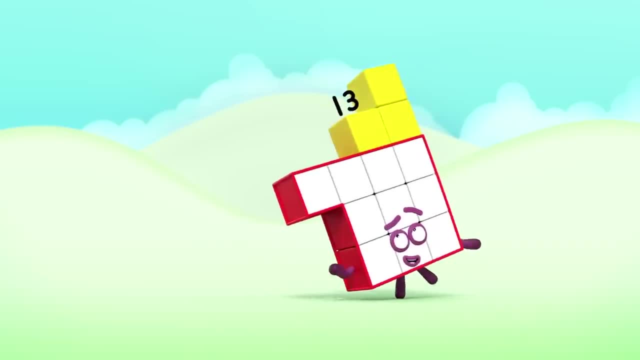 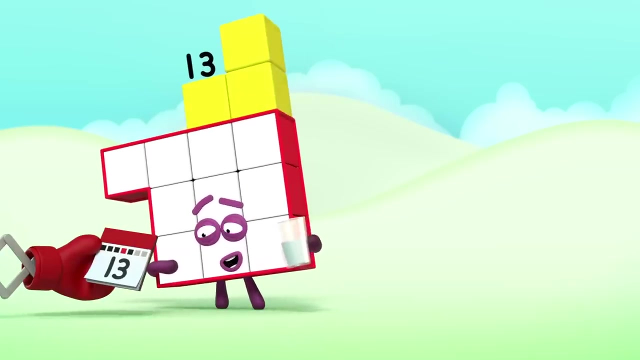 It's getting routine. They ask me my name. I say I'm thir Thirsty. I say I'm thirsty. They ask me my number- You know what I mean. And I always say it's thir Thirsty. I always say it's thursday. 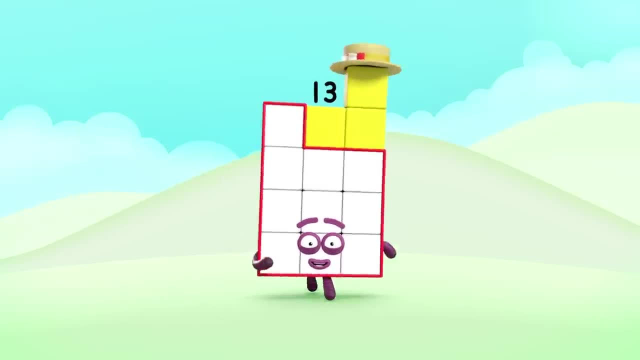 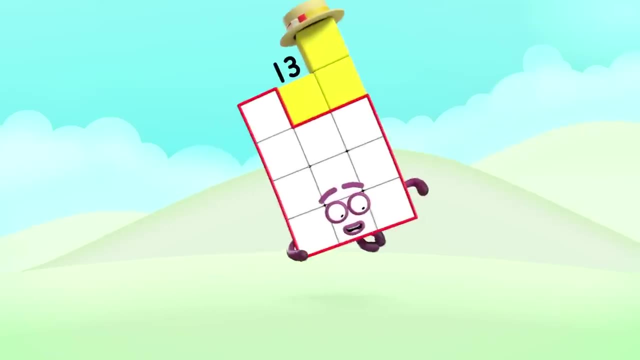 And he's jacking. it's thir-tay Whee. This is me, 10 and 3 Turning this into a game. I'm changing my luck. I won't come unstuck As long as they don't say my name. Call me one more than 12. 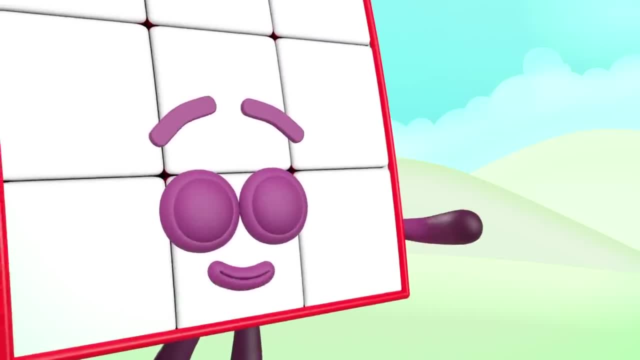 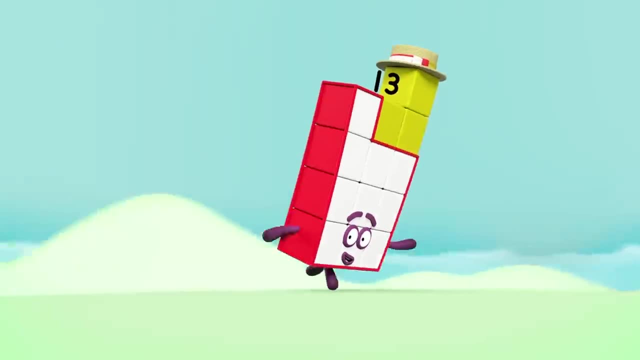 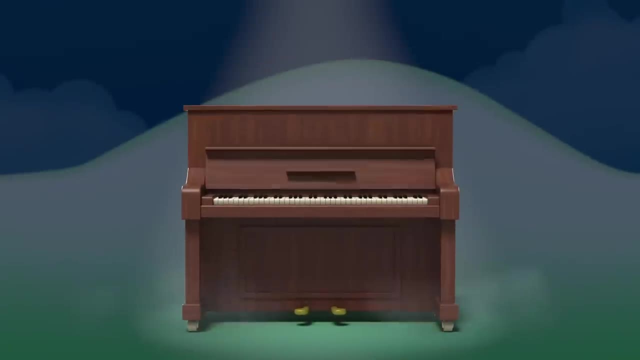 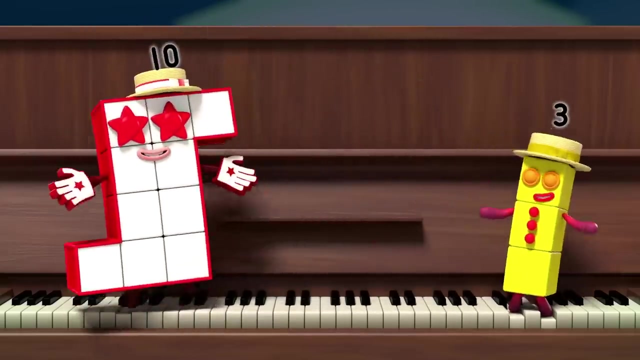 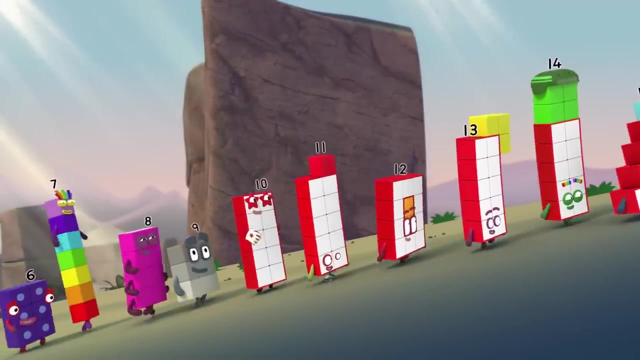 Or 10 and 3, Whatever you call me, I'm still me. I'm still me. The number you've ever seen So lucky To be unlucky Number 13, 13, 13, 13, 13, 13, 13. Unlucky me. I can't wait to visit the pattern palace. 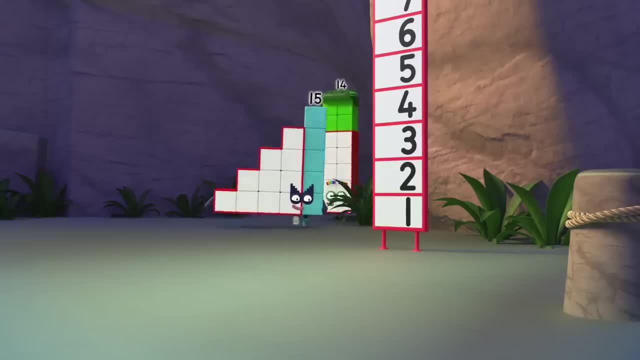 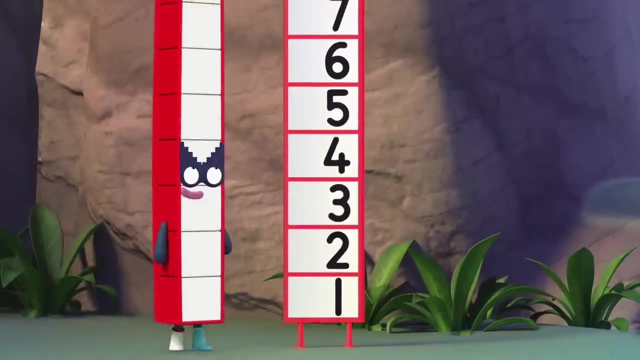 Is it far? There's a shortcut round this ridge. If you can cross the balancing bridge, It might take you to the name of the iron wall, But I've got to find the direction. Do I have to climb this? Where's the easy bike? I can't find it. 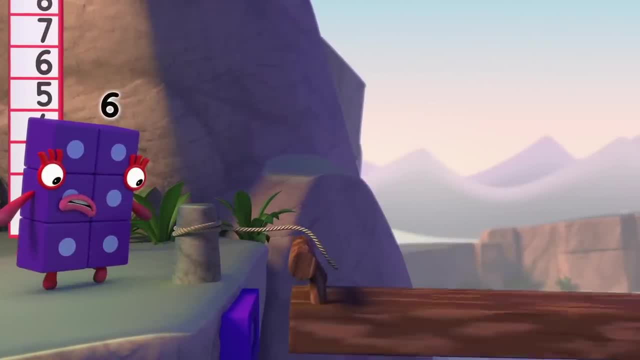 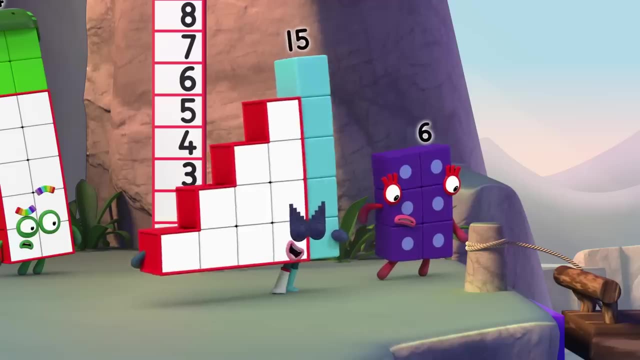 I'll go the other way. I'm going to give it a try. I think I'm gonna go the wrong way. Why, Yo? Oh, What's that? One, two, three, Oh, there it is. Ah, look at that, You're all stuck. 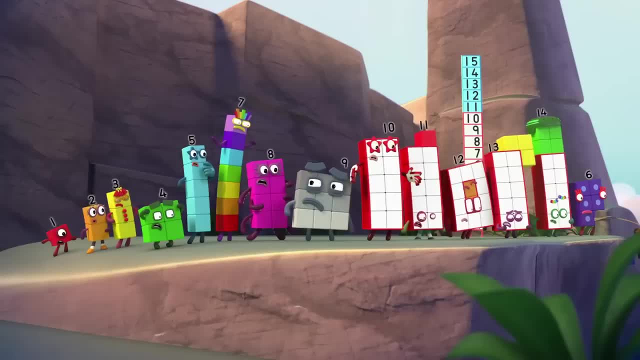 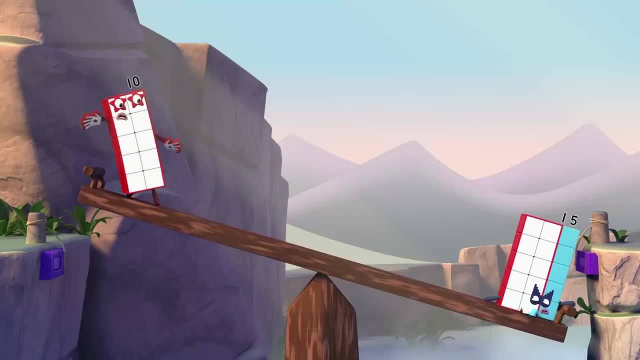 I've got my ring. You're all stuck. What do you think? Oh, it's a good thing. Oh, don't worry, It's nice out before 15 falls off, but I'm not big enough to do it alone. 10 is less than 15.. You need 15. 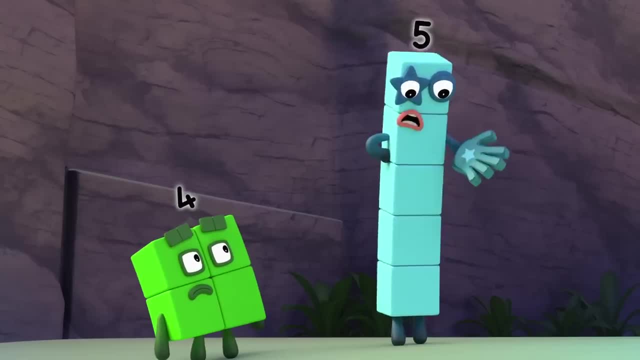 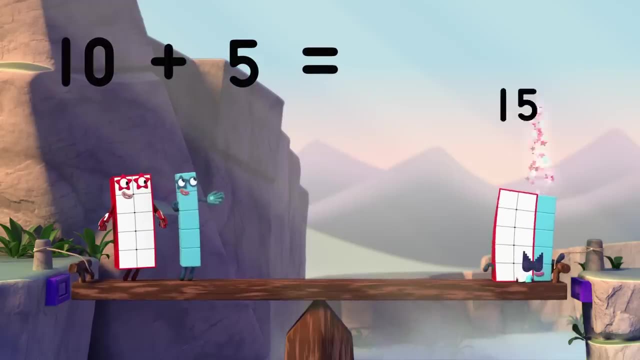 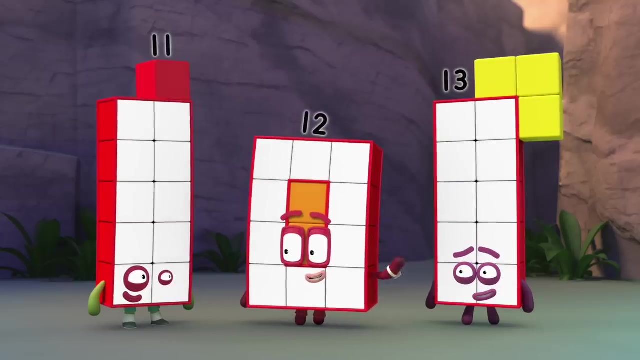 blocks to balance me out. But 15 is 10 and 5, so if I land a hand, 2 plus 5 equals 15.. Grib hold, We need to reach the far side so we can lock the bridge. I can do this, I am. 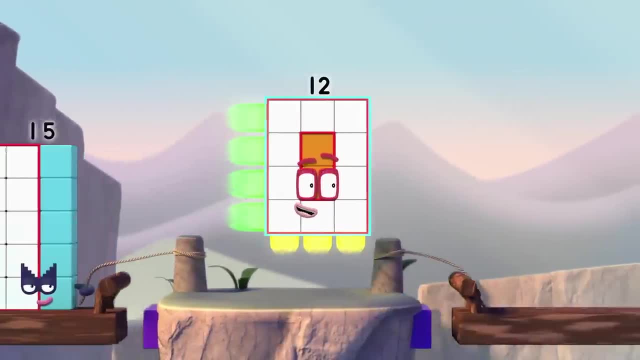 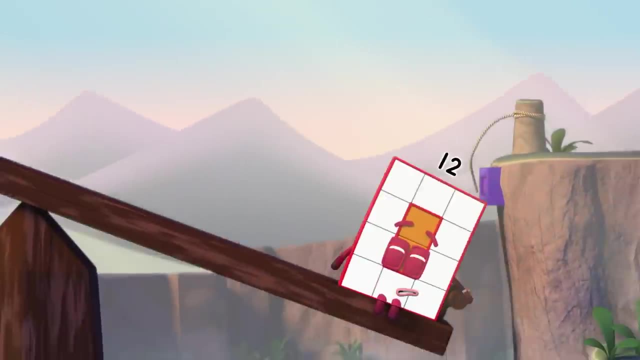 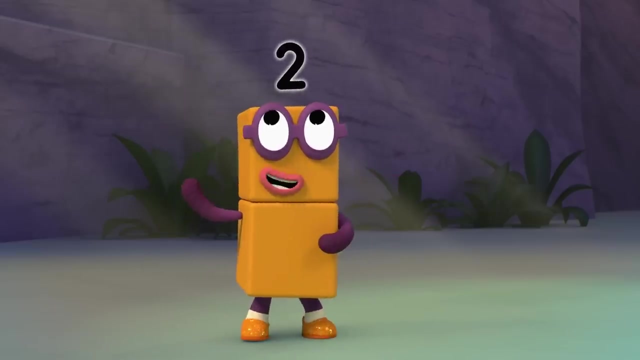 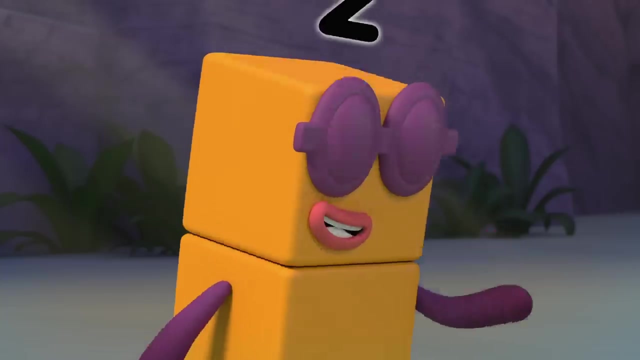 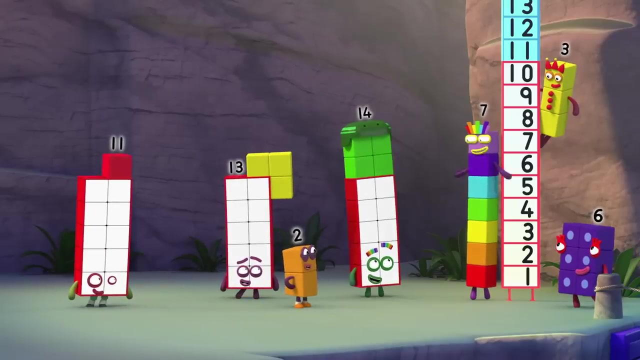 3 by 4.. I am a rectangle. Wow, that is so cool. Thanks, What's going on? 12 needs balancing and 12 is 10 plus 2.. Come on 10.. Wait, Where's 10?? A bit busy, Sorry. Then we need another 10.. 7, 3. You can make 10.. That's lucky. 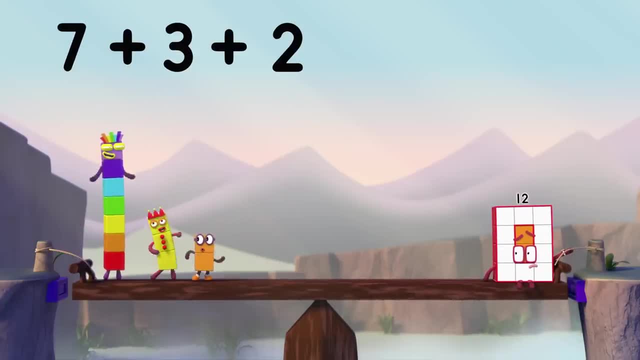 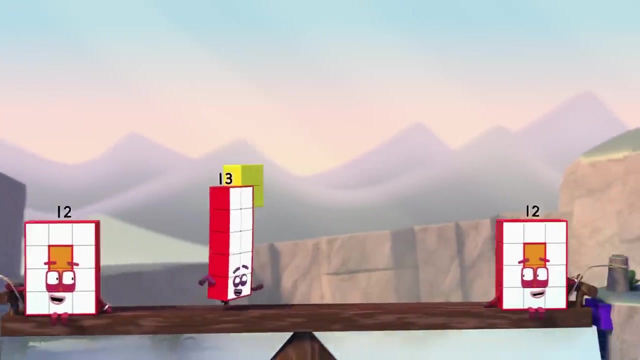 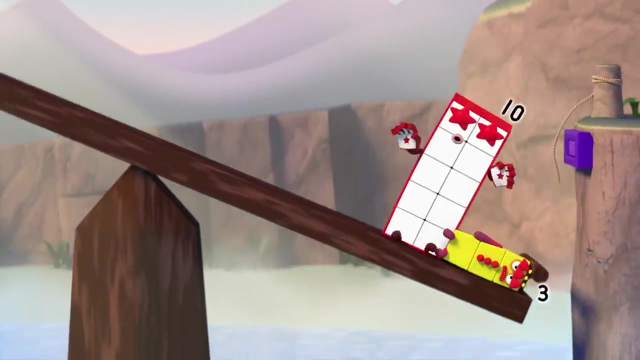 7 plus 3 plus 2 equals 10 plus 2 equals 12.. Grib hold, We're halfway there. What could possibly happen? Oh, look out 13.. Who said it? We need to balance 13,, but we haven't got a 3 or a 10.. 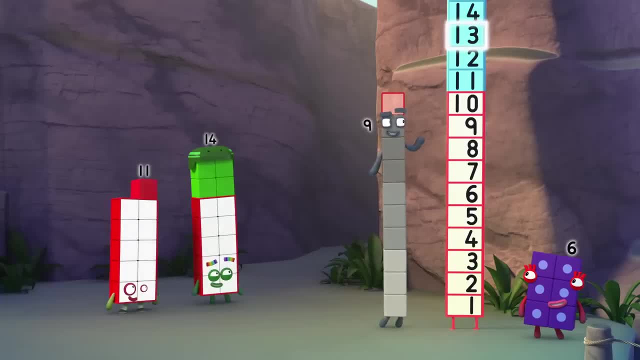 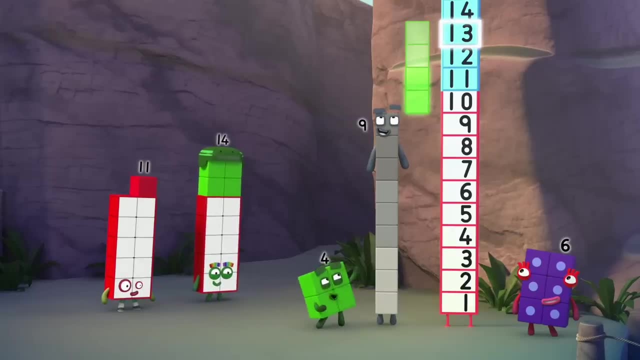 Maybe I can help. I'm only 1, less than 10.. That's close, And after that we need 3 more blocks, So that adds up to 1,, 2,, 3, 4. 4 blocks. 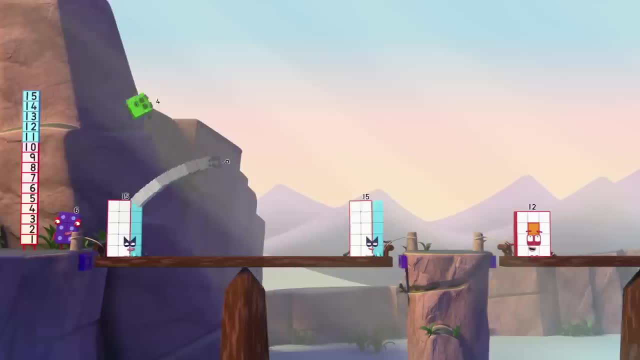 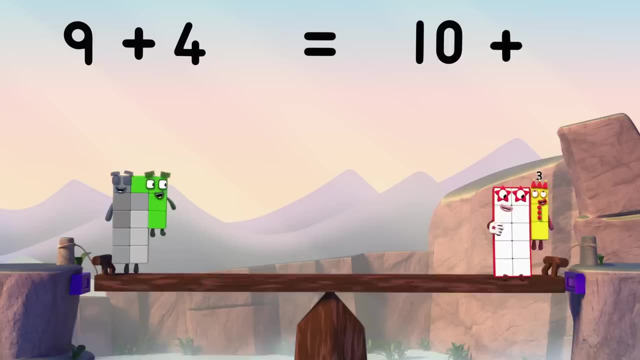 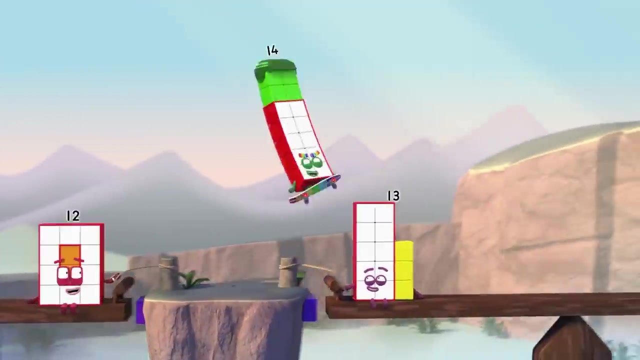 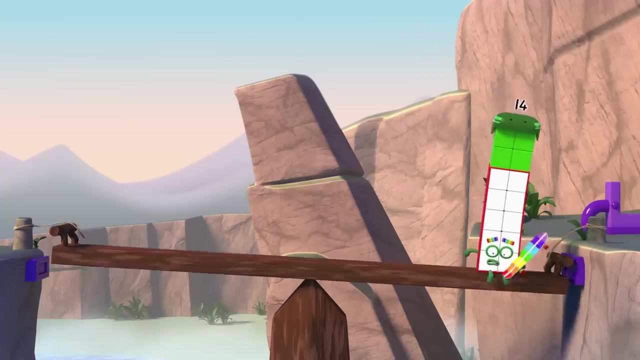 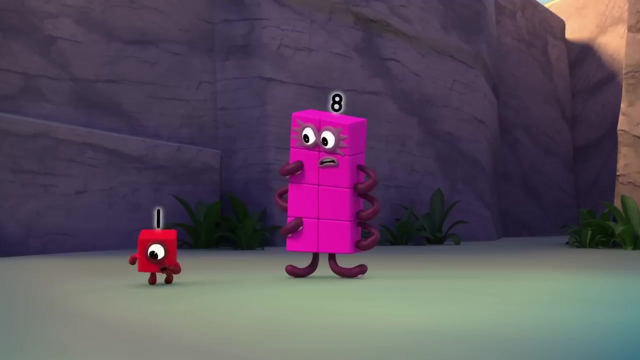 Oh, Square power. 9 plus 4 equals 10 plus 3. And both sides equal 13.. Woo-hoo, Grib, hold One more bridge to go. Woo-hoo, Hey, hello, We need to balance out 14. Somehow, 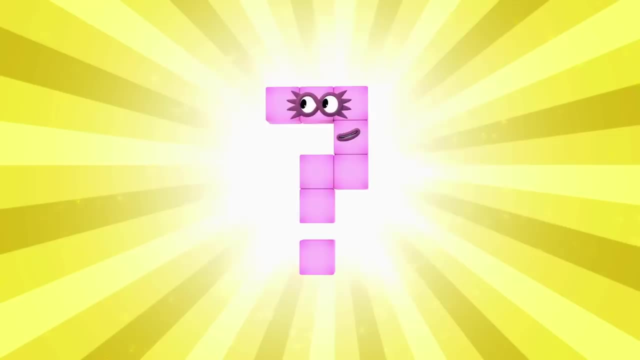 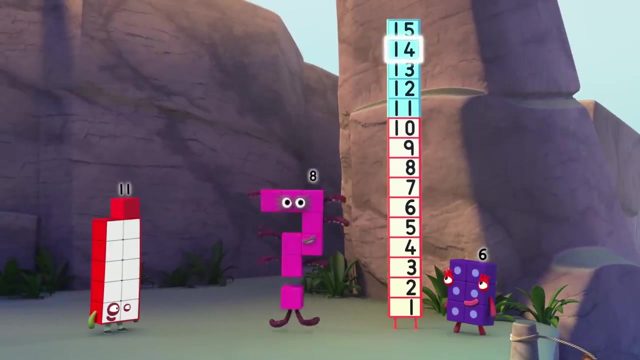 Octoblock. think 1,, 2,, 3,, 4,, 5,, 6,, 7,, 8.. Think: Hmm, How do I get from 8 to 14?? Ha, From 8 to 10 takes 2 blocks And 14 is 10 and 4.. So I need. 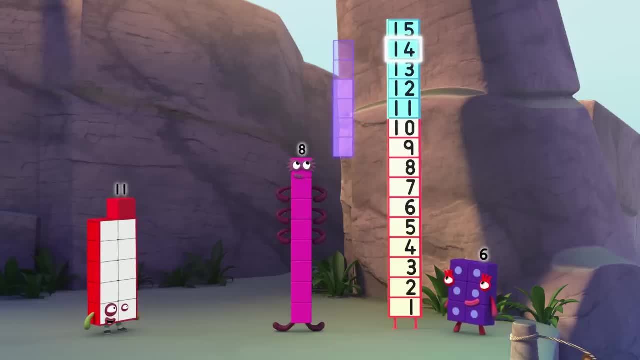 4 blocks more, which makes 1,, 2,, 3,, 4,, 5,, 6.. 1,, 2,, 3,, 4,, 5,, 6.. 3, 2, 1, 1.. 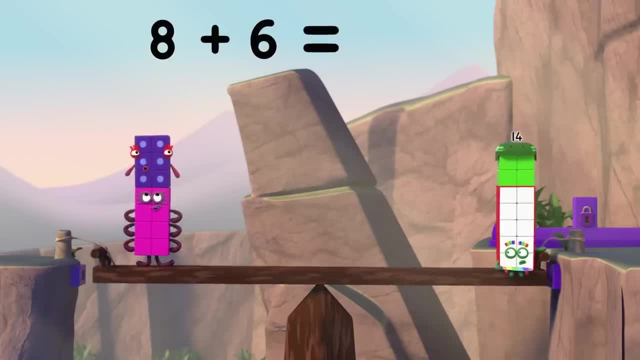 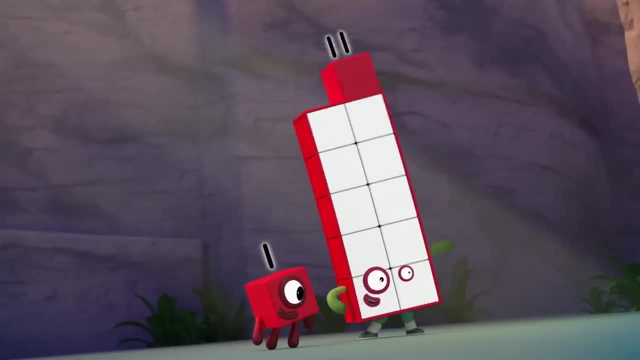 Plus 2. 8. Plus 6.. Equals 14.. Grab hold. Thanks to our team, we've got a clear run at goal And we've got the rest of the course. No, not yet, Not yet. 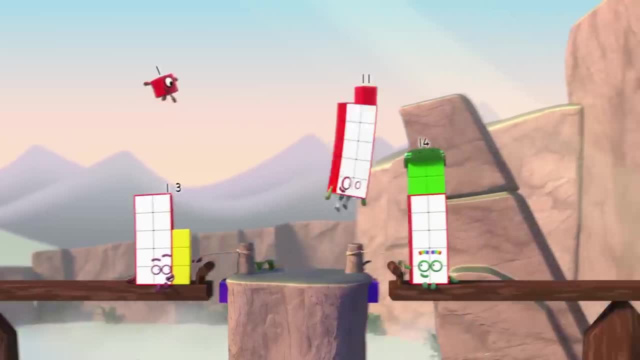 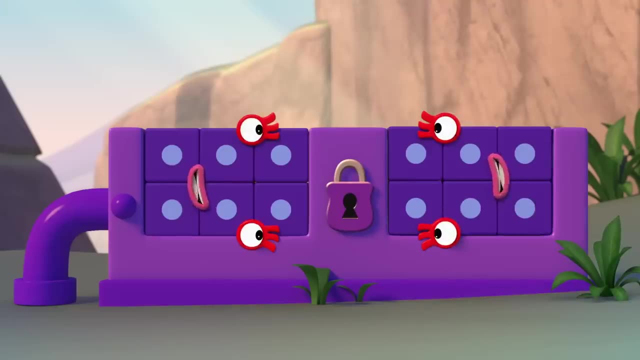 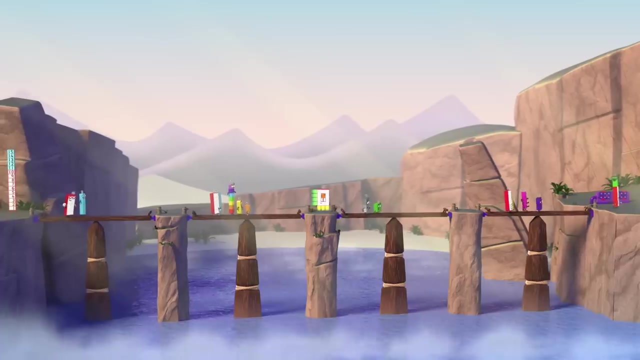 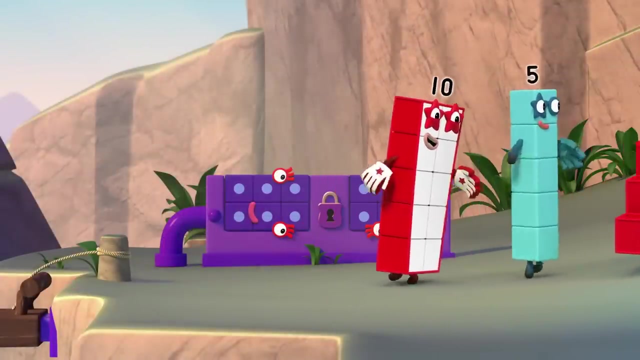 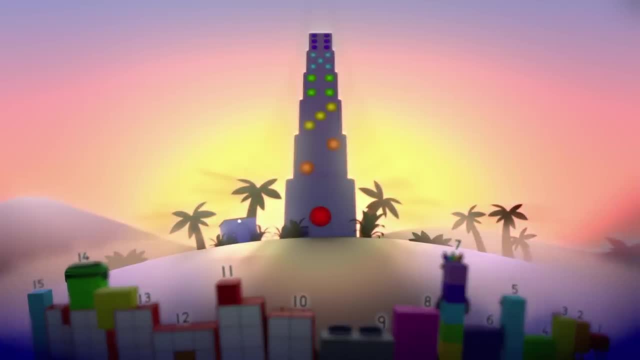 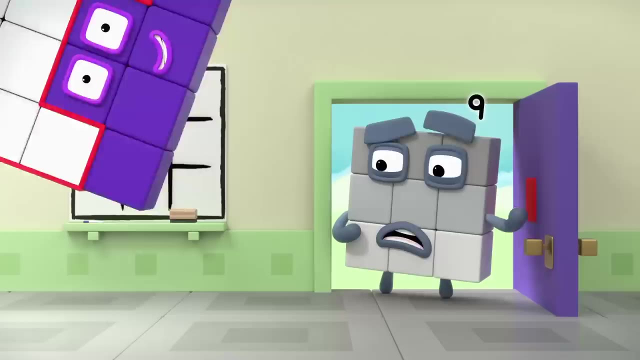 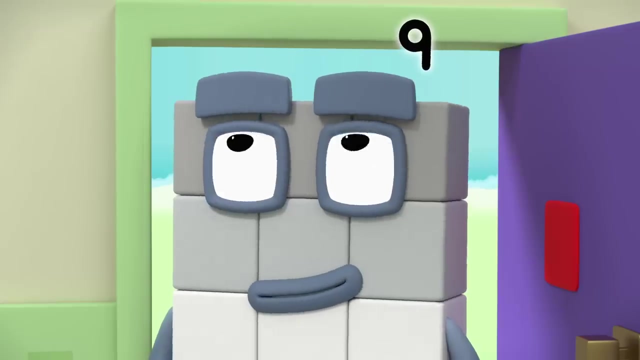 There's a lift. Oh, there's a lift, We can take the lift. There's a lift. Sick Um, is this Square Club? I'll be square with you. Yes, it is Square, Come in. come in, Let's play a game. 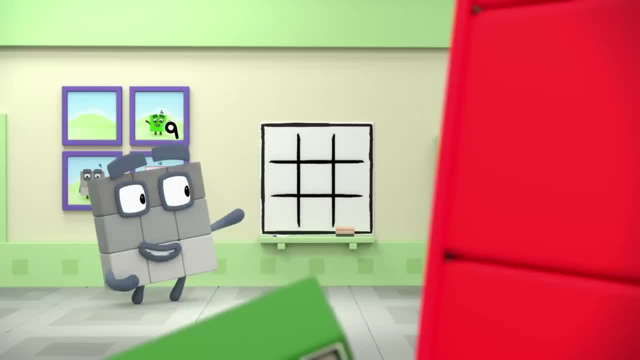 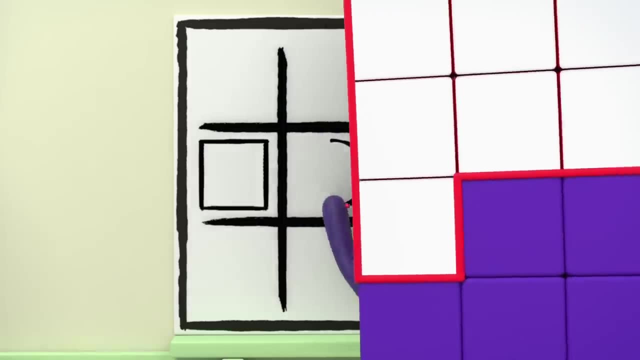 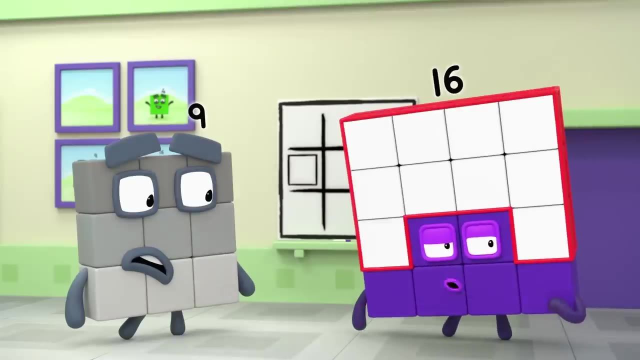 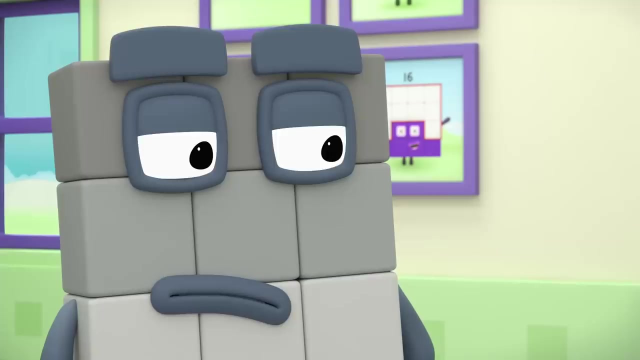 Rock paper squares, Tiddly squares. How about Norton squares? Good call, You start Oh round thing. Oh, I forgot, No round things at Square Club. You win fair and square Square. Sorry, I'm late. 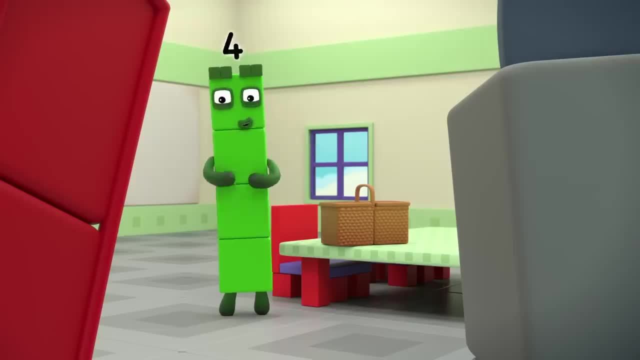 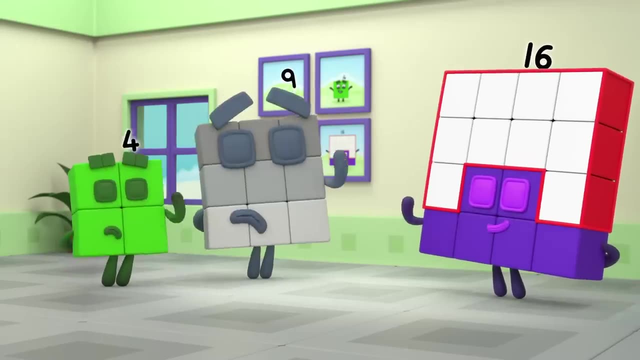 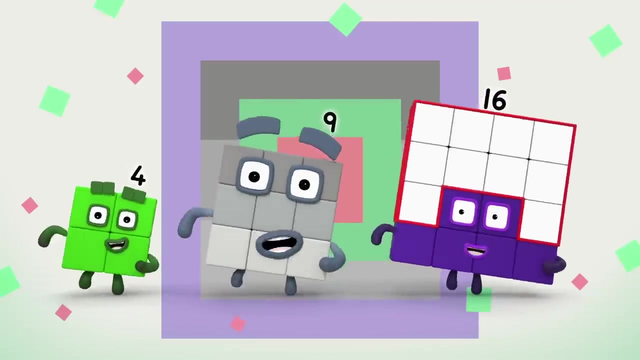 Oh, Oh, dear What? Oh, sorry You. now we're all here and square we can begin. What's the first rule of Square Club? No round things. Right, you are. And let me hear the motto: Even though we're different sizes, you can always recognise us. 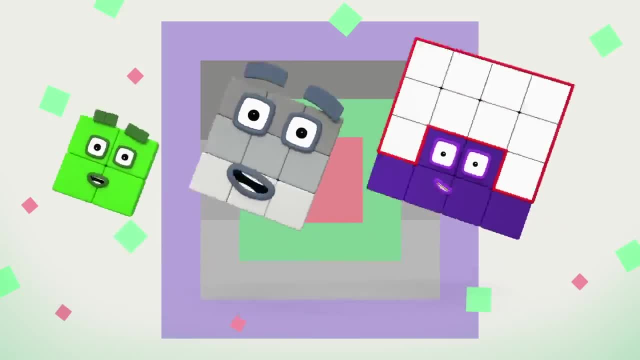 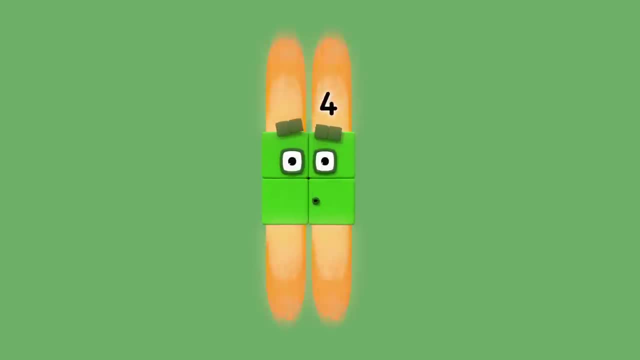 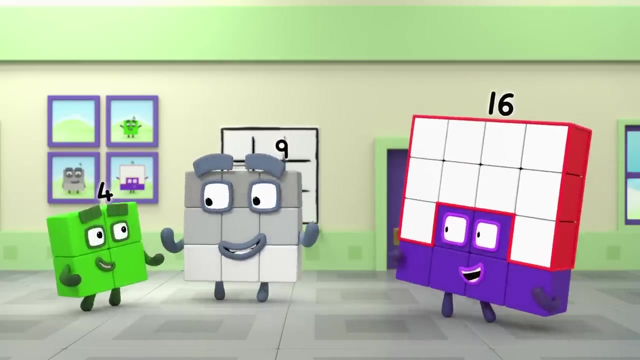 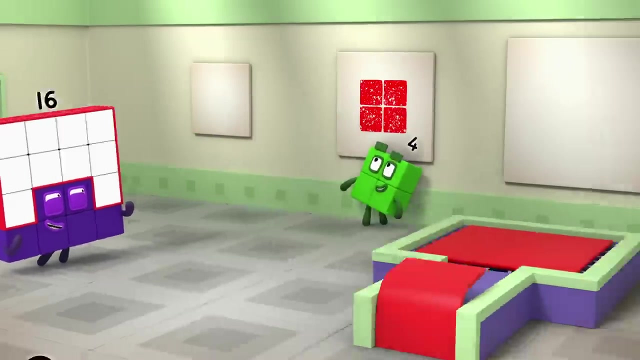 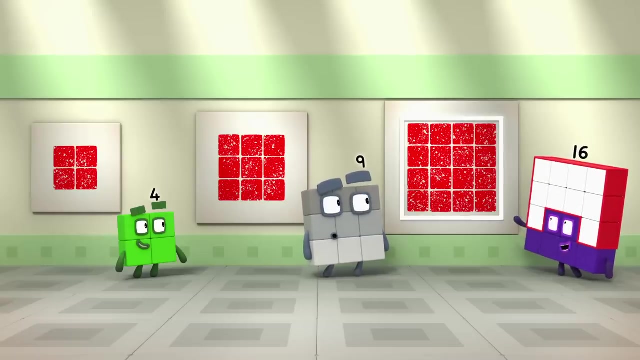 We're as tall as we are wide. We're the same, tall on each side, Four by four, Three by three, Two by two. Square Club Hooray: Time for some square art. My square has four sides all the same and four corners all the same. 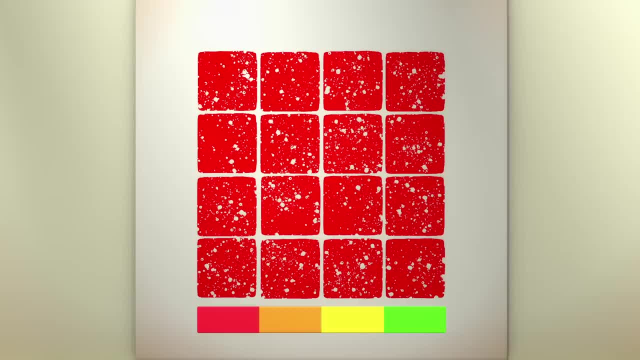 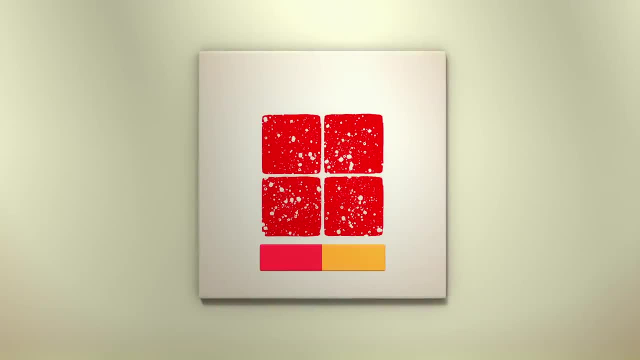 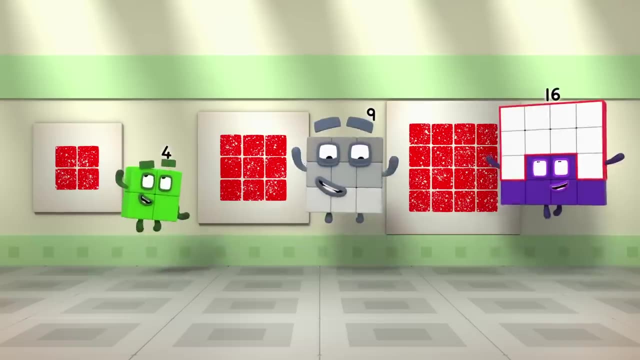 So does mine. Mine too. Mine's four across by four down, Mine's three across by three down, Mine's two across by two down. We're all square. Hooray again, Hooray, Woohoo, Ooh. time to eat. 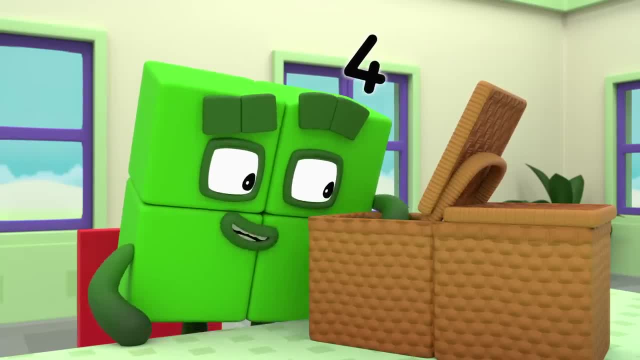 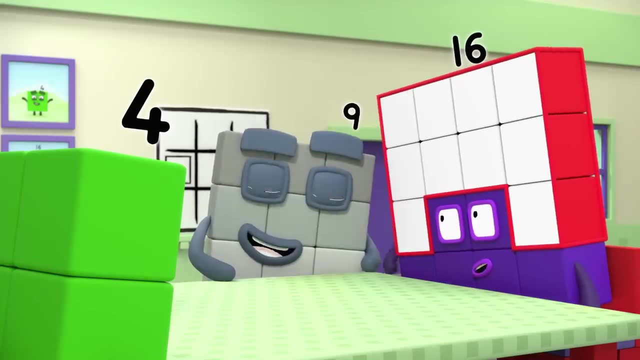 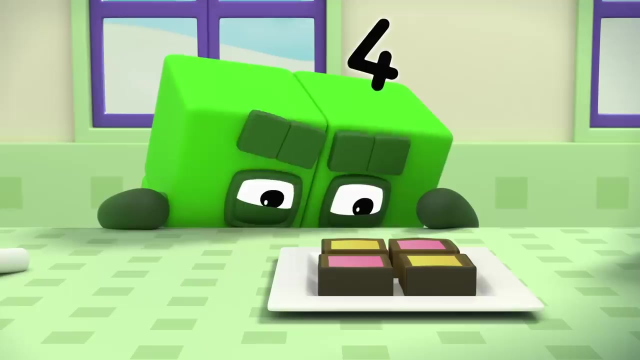 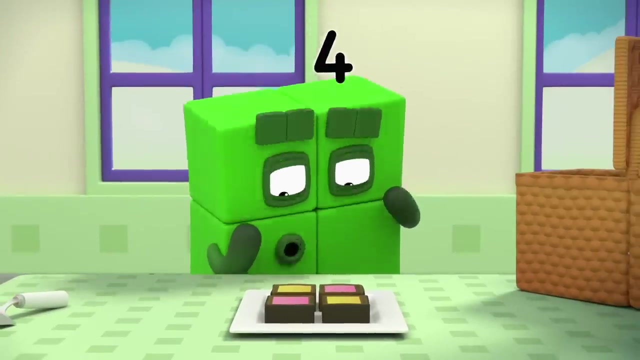 Square sandwiches, Square cheese on square crackers, Square apples, Square cake- Everything we need for a square meal Cake sounds good. Hmm, Pink or yellow, Pink, No, yellow, No pink, No yellow, Pink Yellow. Oh, I don't know. 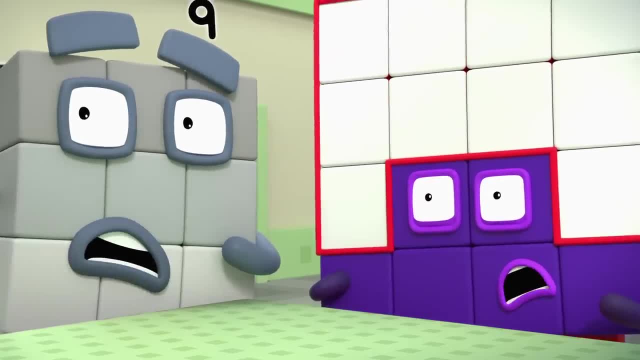 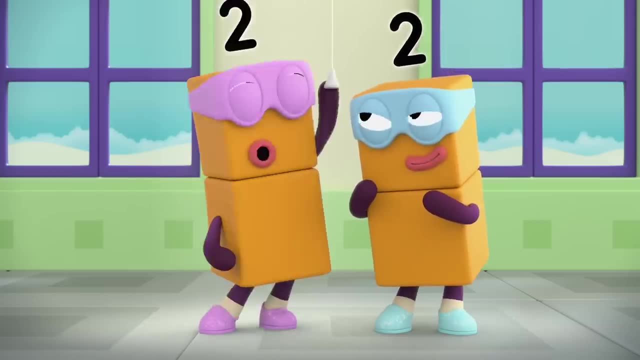 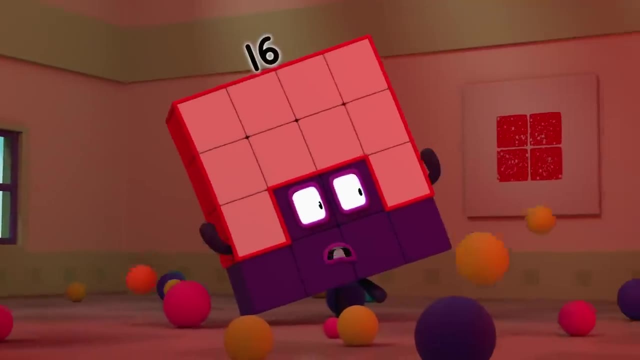 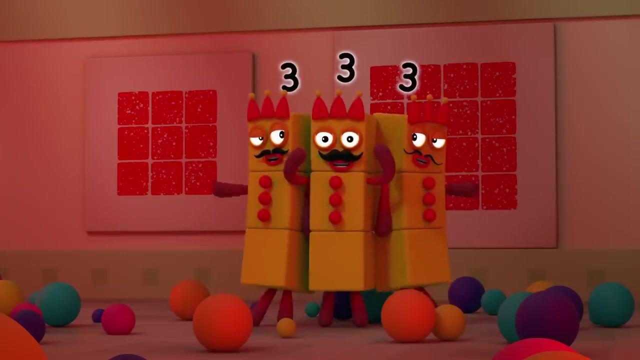 Oh no, That's terrible. twos. What's the first rule of Square Club? No round things, Oops, No round things. Don't panic. Don't panic. Pull yourself together Or not. We three are the three threes. 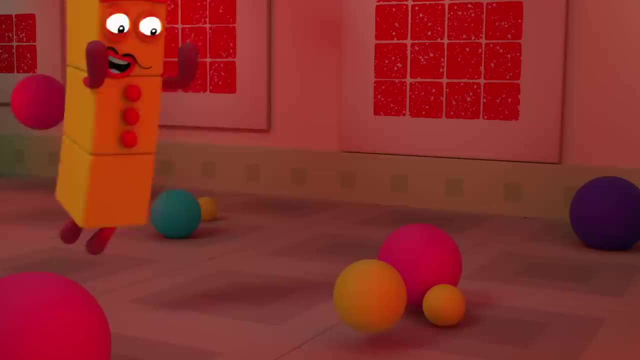 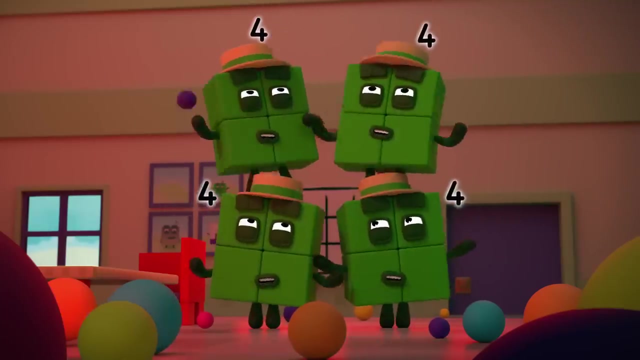 Drum roll please. Vroom, vroom, vroom, Vroom, vroom, vroom. Good idea, We are the one. two, three, four, four, fours. What could be more square than squares in a square? 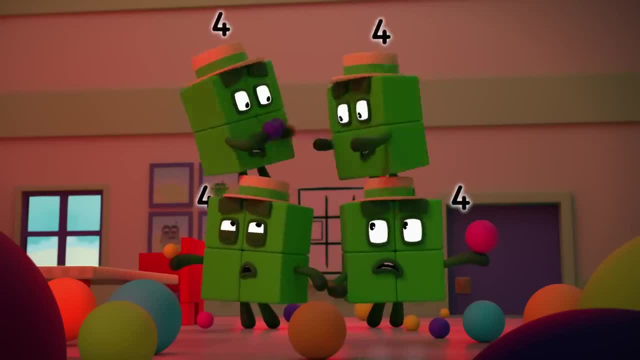 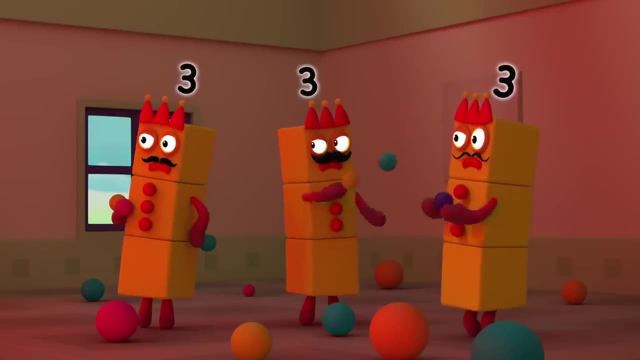 Hee, hee, hee, hee, Ahh, Don't give them to me. I don't want them, nor do I You have them. Don't just stand there juggling. Get rid of them, You can talk. Ha, ha, ha ha. 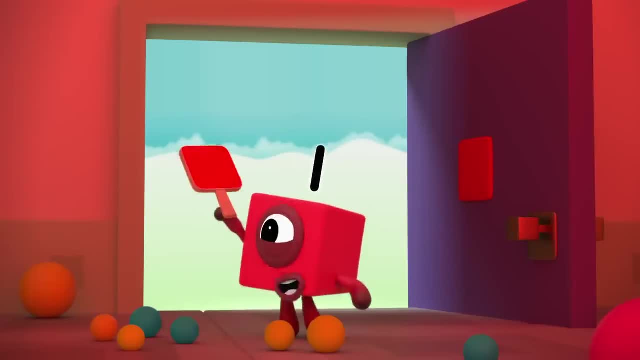 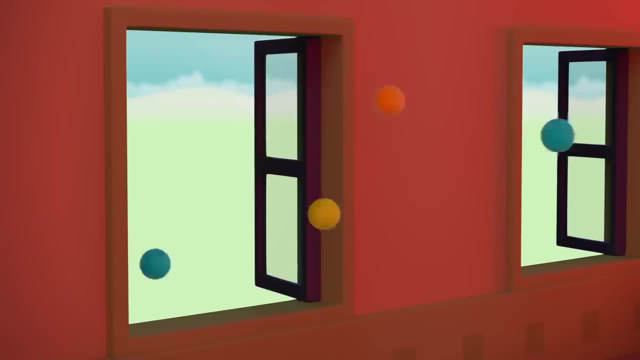 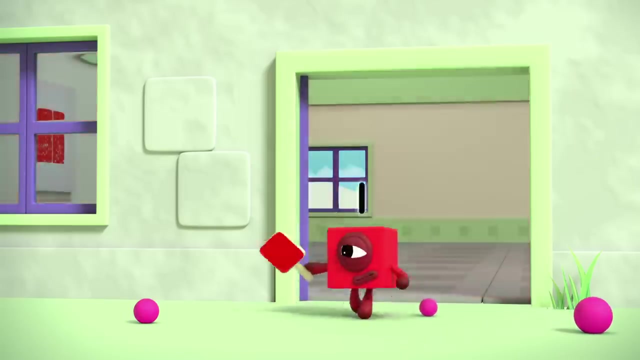 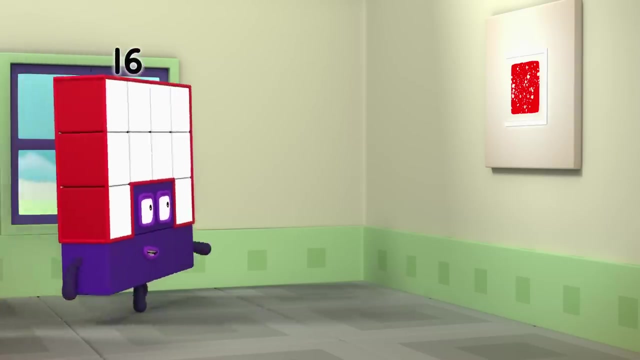 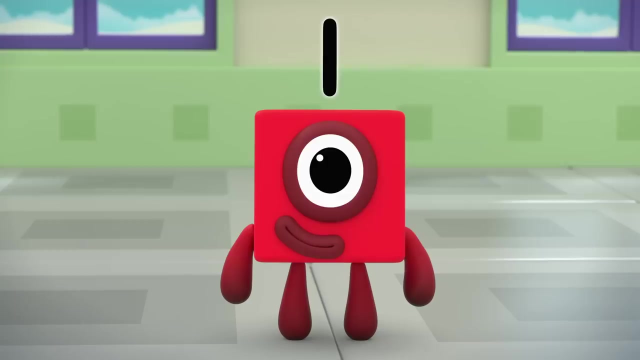 Leave this to The one, one, One, one, one one. four Duh There, All square again. Four sides all the same, Four corners all the same, One across by one down. One is a square number. 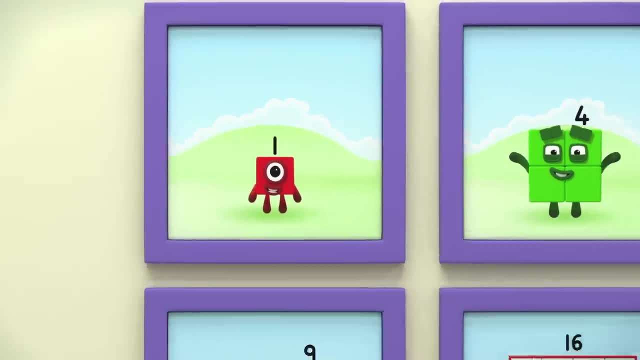 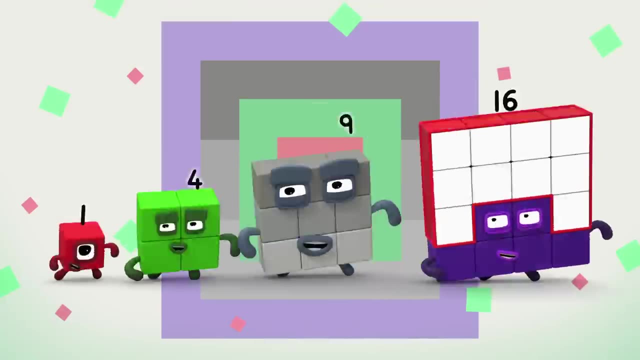 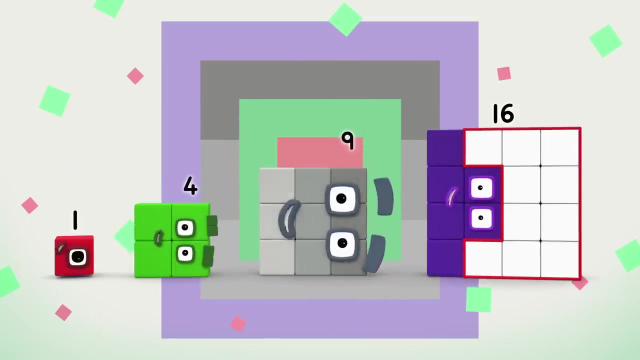 Nuh huh. Welcome to Square Club 1-1.. Even though we're different sizes, you can always recognize us. We're as tall as we are wide. we're the same dirt on each side. Four by four, Three by three. 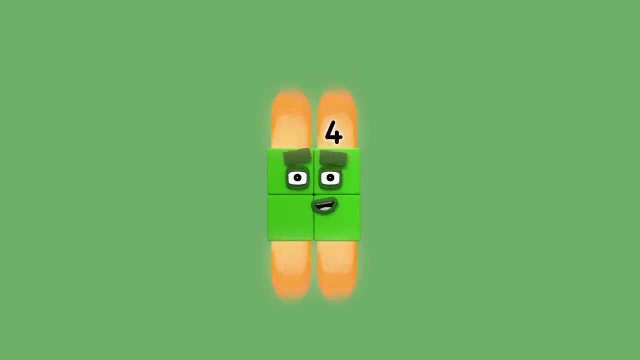 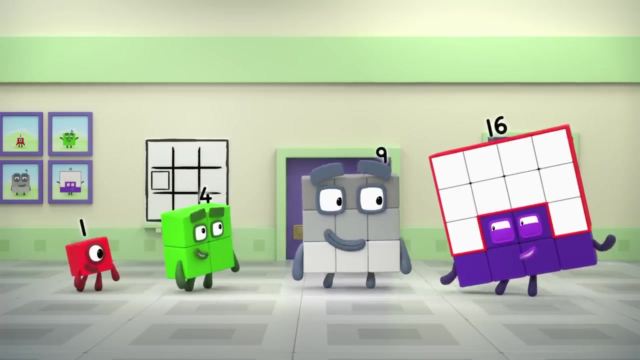 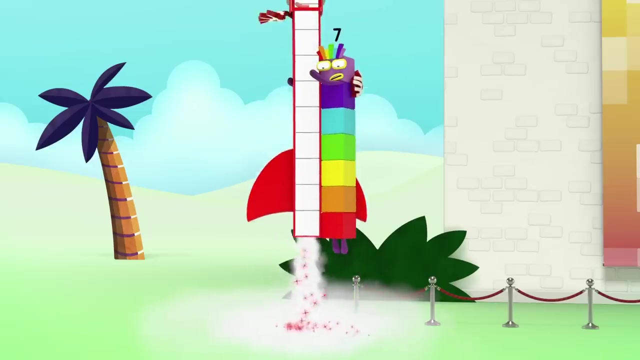 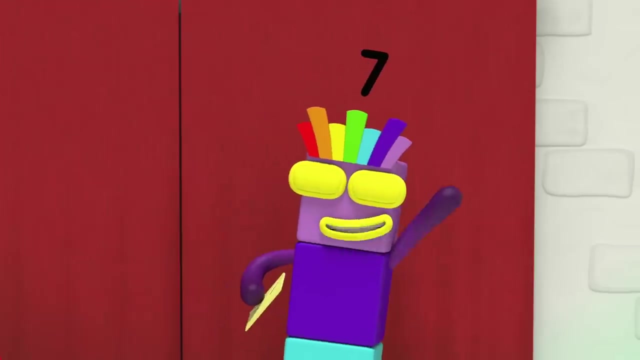 Two by two, One by one. Square Club Hooray, Hooray, Looks like we're back to square one. Thanks for the lift Ten. Are we in time? Yes, just about. That's lucky. I wouldn't miss the opening of Numberland's first art gallery for the world. 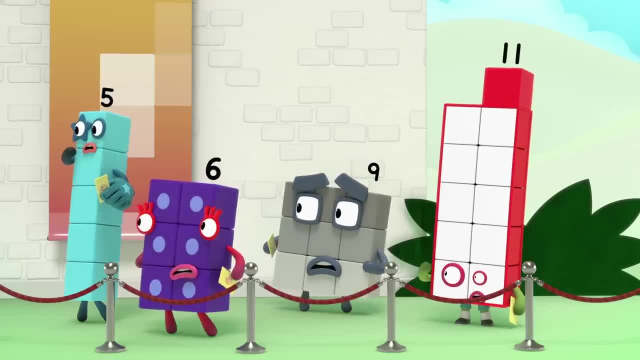 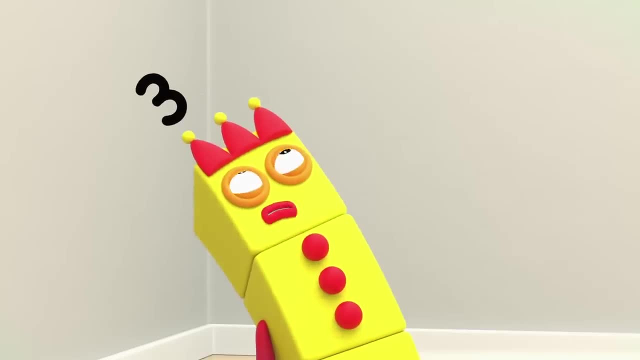 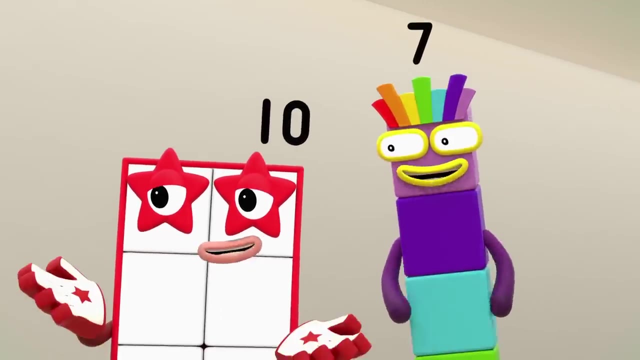 You and you Rock and roll. Oh, I like it, but where's the art? Oh, I spent so long making sparkly invitations I forgot to get any. Ooh, Can we help? I thought you'd never ask. 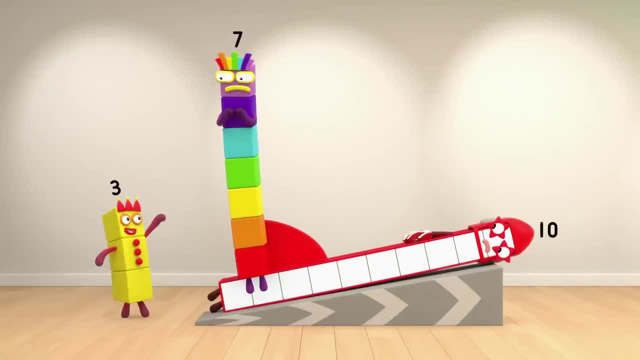 Are you sure you're a rocket? You're full of colours, Fly through the museum and make art. But Ten, nine, eight, seven, six, five, four, three, two, one, What? Ah, Whoa. 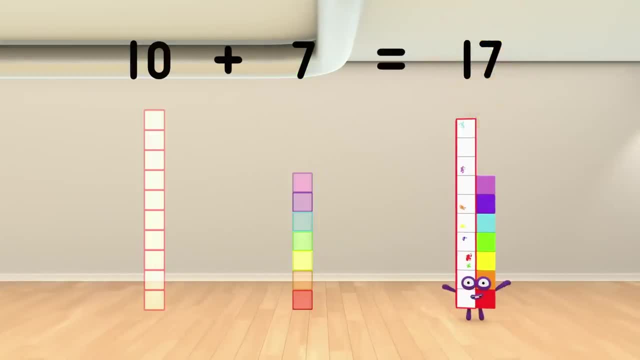 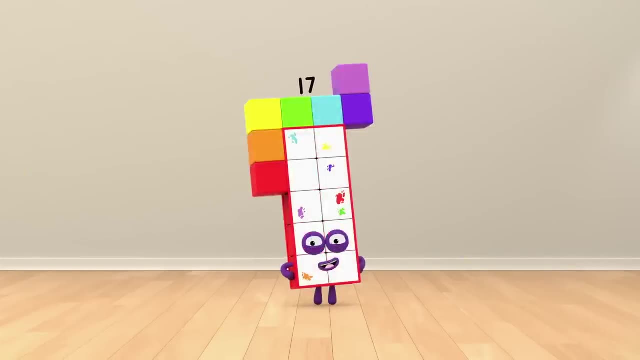 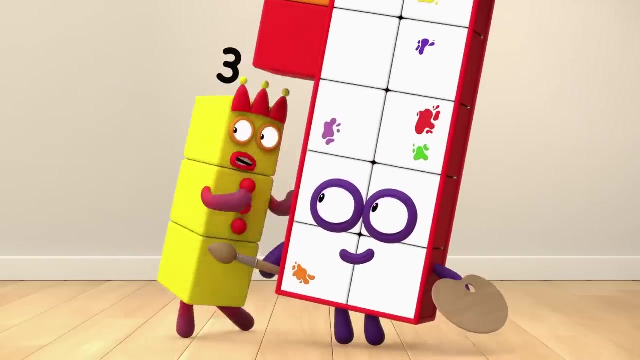 Ten plus seven equals 17.. Oh, now there's a surprise: I am 17, and I love to paint. They're coming in. Oh no, Go, go, go, Don't mind if I do. Some painters only paint portraits. 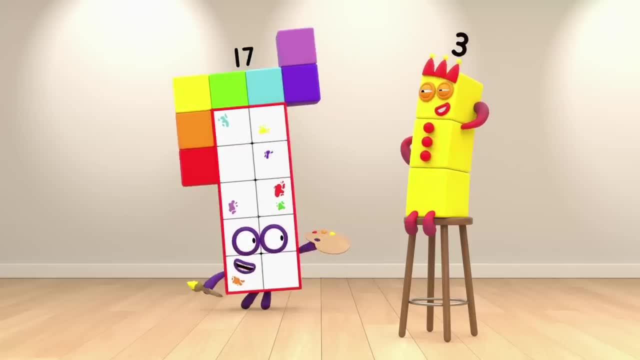 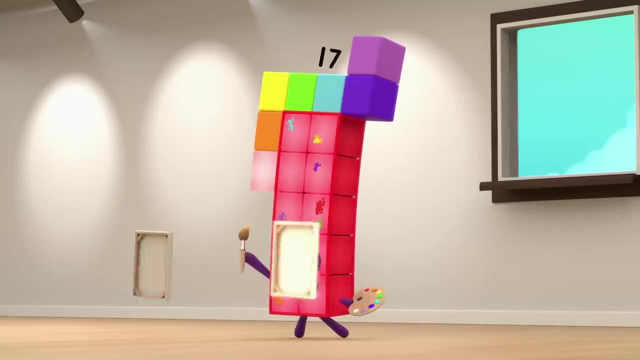 Majestic fancy rings. I can also paint portraits, but I paint 17.. One, two, three, four, five, six, seven, eight, nine, 10,, 11,, 12,, 13,, 14,, 15,, 16,, 17.. 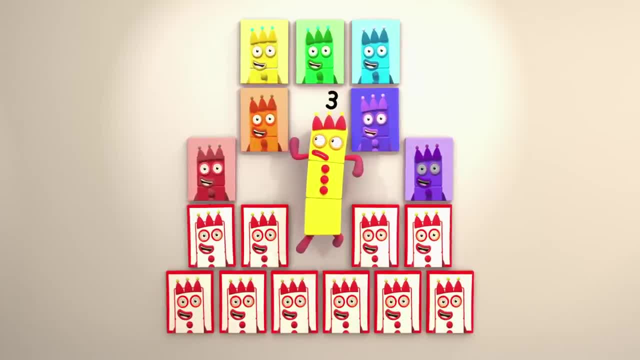 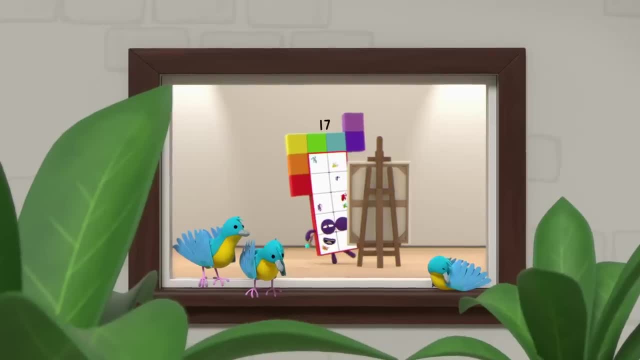 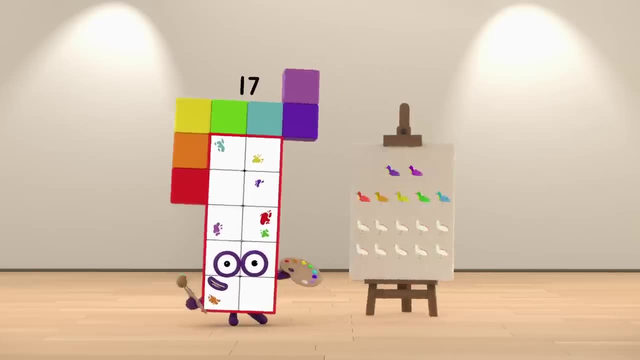 Hee-hee, Look at me. Ooh, No, Look at me. Hmm, Nice juxtaposition. Some painters like to paint bluebirds in a lovely nature scene. Why paint only a few birds when I paint 17?, Ten and seven? 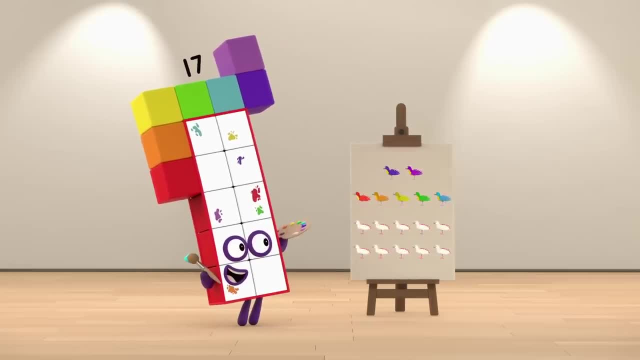 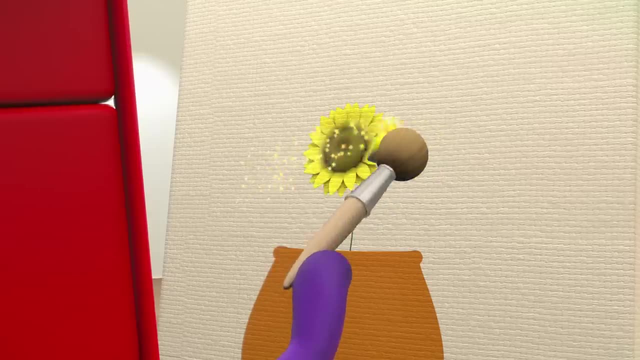 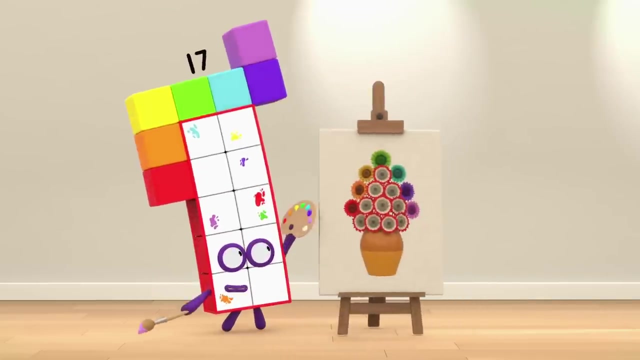 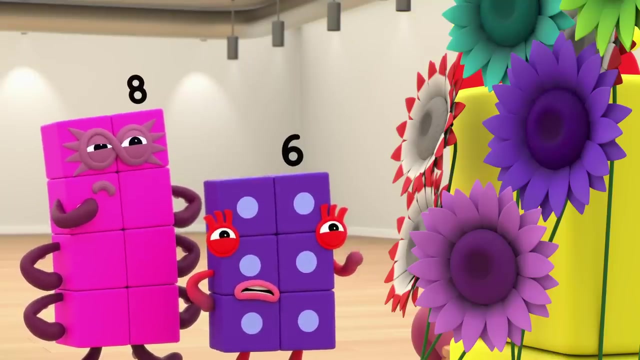 17. Ooh, Hey, Oh, Ooh, Nice juxtaposition. Some painters paint flowers. They look so sublime. I paint for hours. 17 of everything takes time. What? Hmm? Nice juxtaposition, Hmm, Hmm. 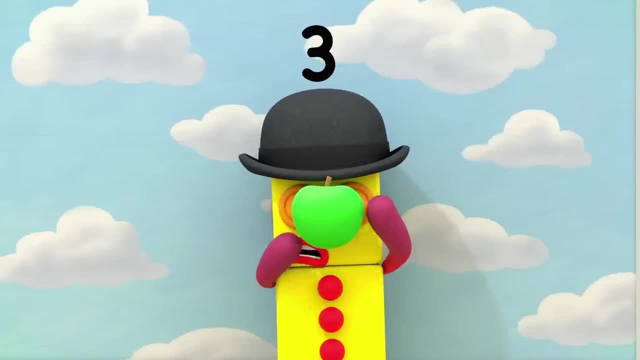 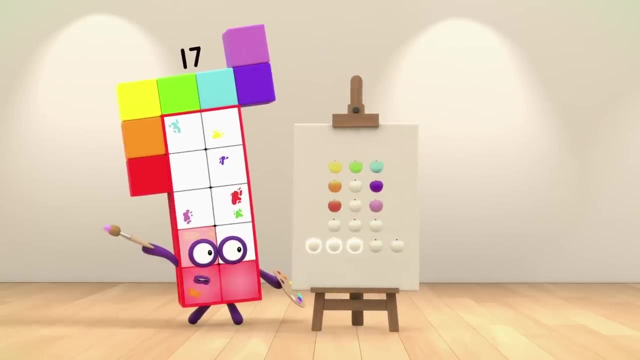 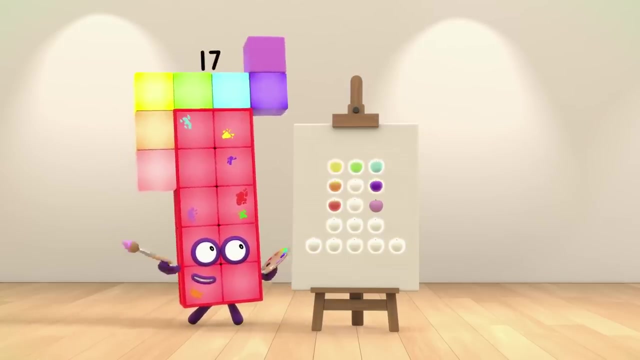 Hmm, Some painters like to paint apples in brilliant shades of green. I can also paint apples, but I paint 17.. One, two, three, four, five, six, seven, eight, nine, 10,, 11,, 12,, 13,, 14,, 15,, 16,, 17.. 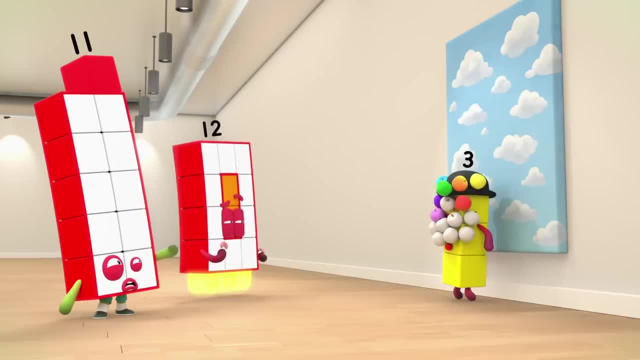 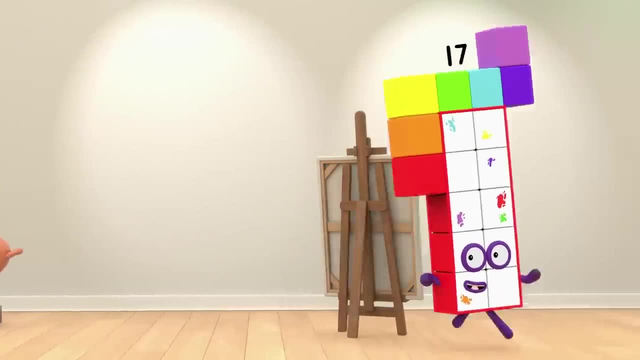 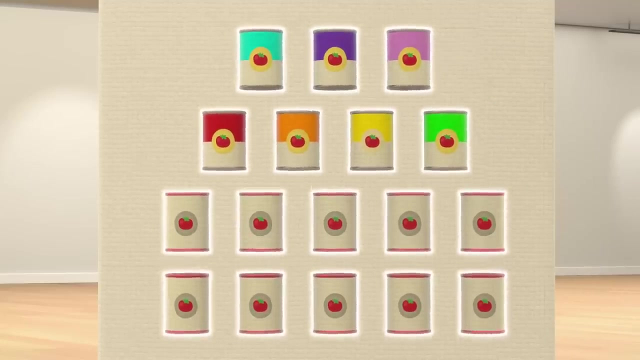 Hey, No, Get off, silly apple. Ah, Nice juxtaposition. Some painters like to paint soup cans. I like a whole tureen, So I paint plenty of soup cans. I paint 17.. Ten and seven, 17.. 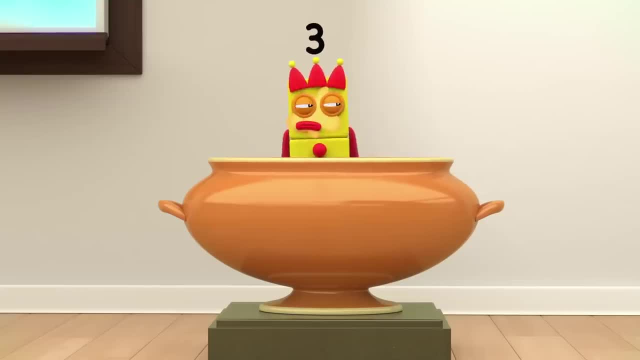 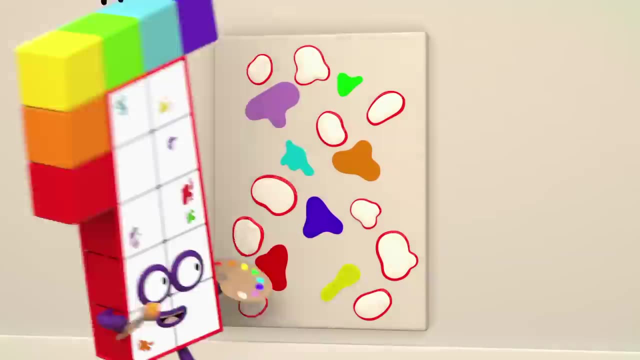 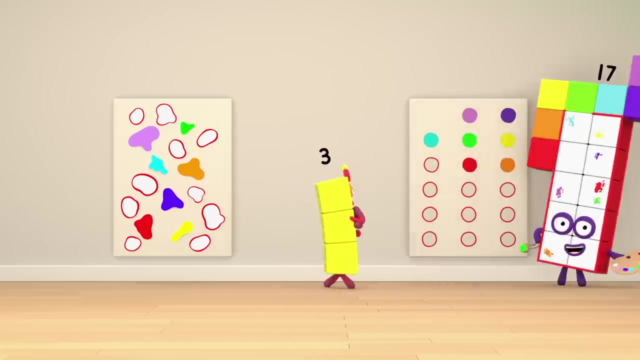 I'll eat soup. Hmm, Nice juxtaposition, Brrr. Ooh. Some painters paint splatters, Some painters paint dots. My number's what matters, 17 is lots and lots of spots. Ooh, Ooh, Ooh. 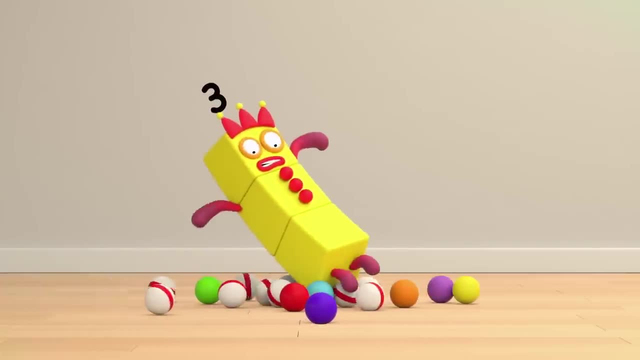 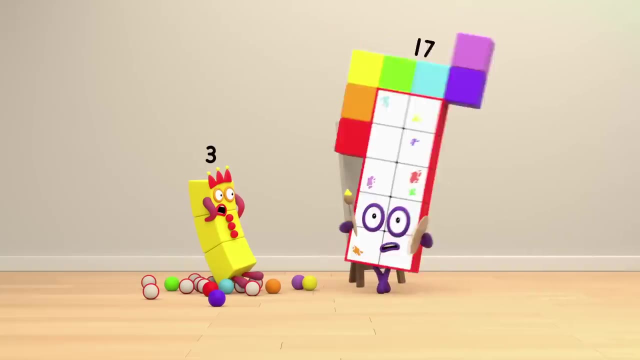 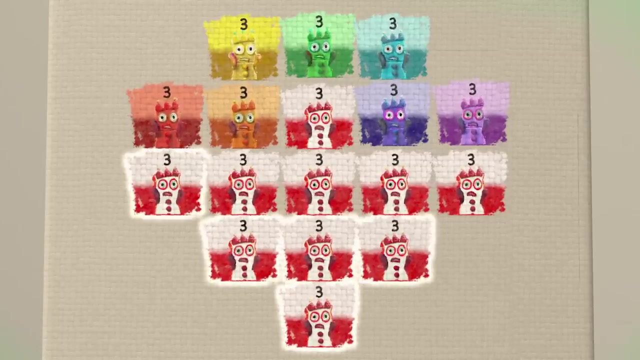 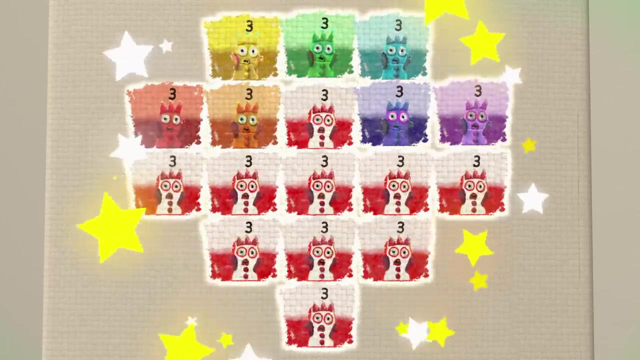 Nice juxtaposition. Ha Ha Ha. Hold that pose. Some painters like to paint faces that look like they might scream. I can also paint faces, but I paint 17.. One, two, three, four, five, six, seven, eight, nine, 10,, 11,, 12,, 13,, 14,, 15,, 16,, 17!. 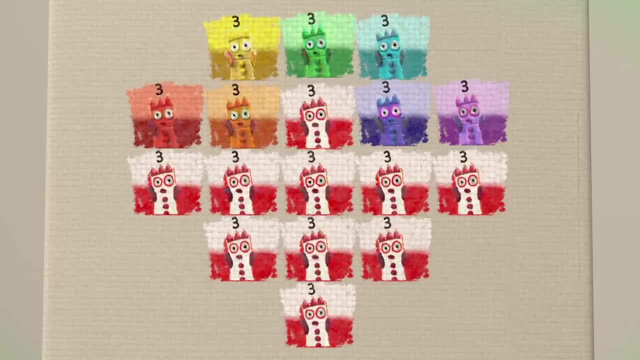 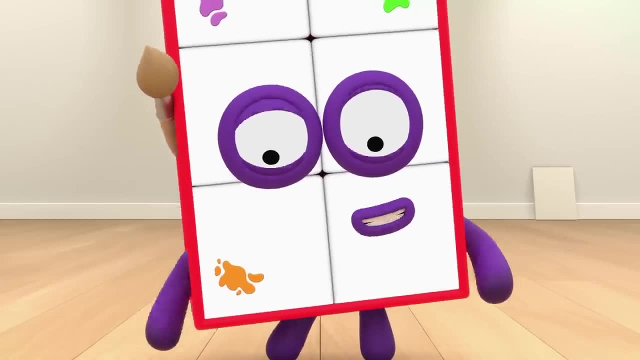 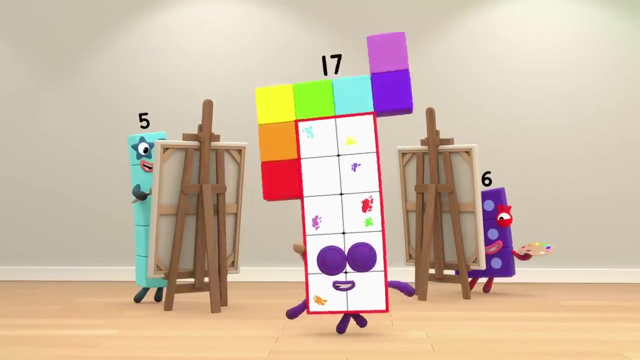 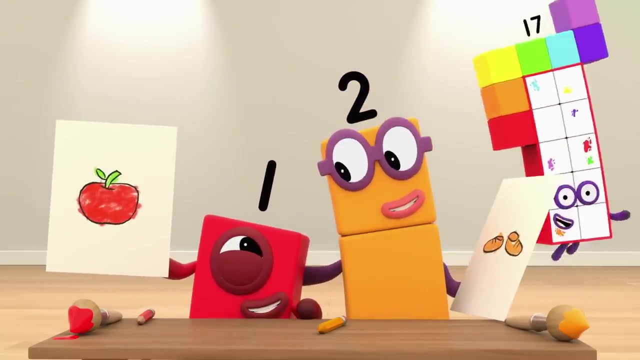 I scream, you scream, we all scream for ice cream, Ah, Yummy. Wait, I know what this gallery needs: Your art, Let your imagination play. Paint what you want, go your own way. A piece of paper's purpose is to be your picture one day. 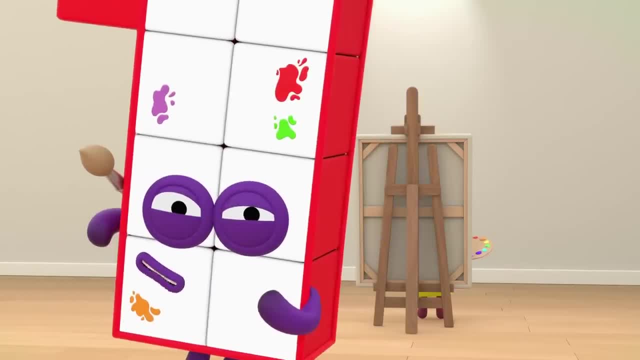 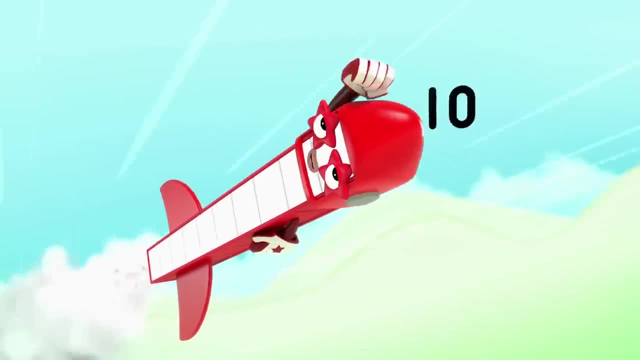 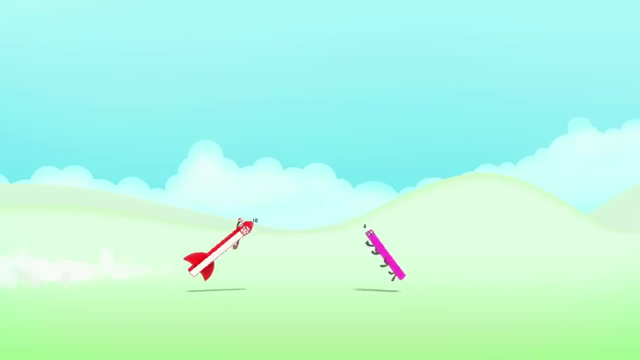 You could be an artist- the best there's ever been- But why paint only one of things when you could paint fast as a rocket Octo-speedy Too fast, Uh-oh. Ten Plus eight Equals, Whoa. 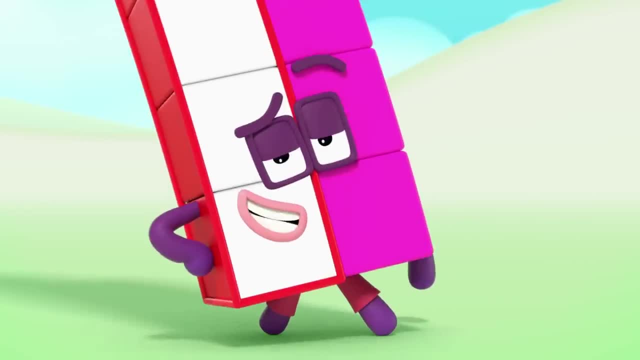 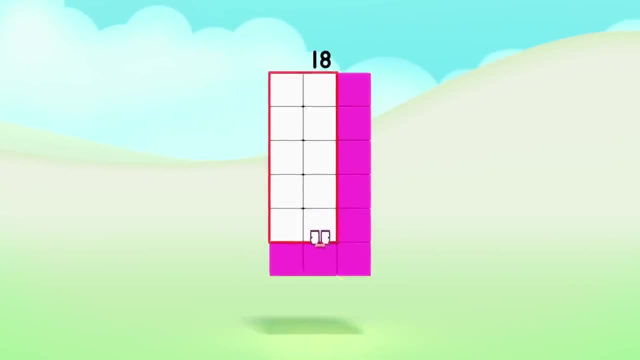 18! Refreshing Hey time to discover who I am Done, I am 18. And I'm a super-speedy Super-rectangle And I like to go fast. Yah Oh, so tall. Ooh, falling over competition. 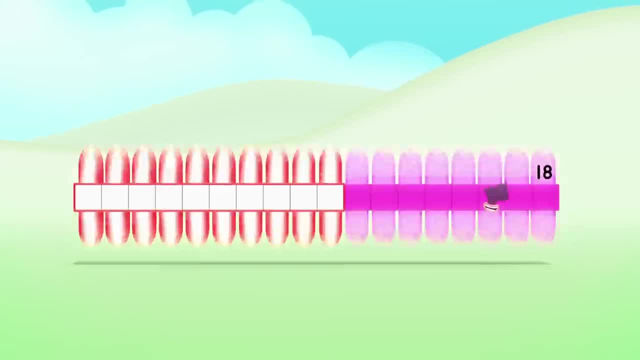 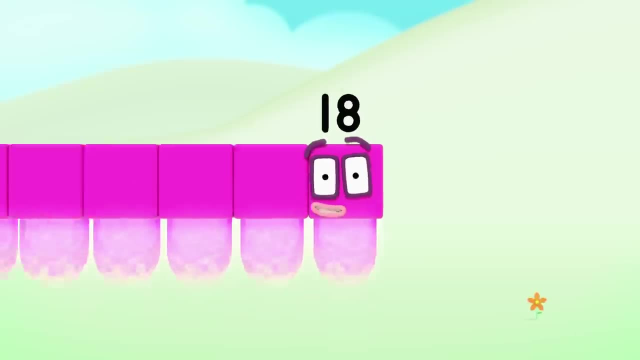 Ah Oof, I win Ah-ha 18 by one. One ray is all. I need One ray to build up speed. I start to glow and I go, go, Go. Whoa Ha-ha Ooh. 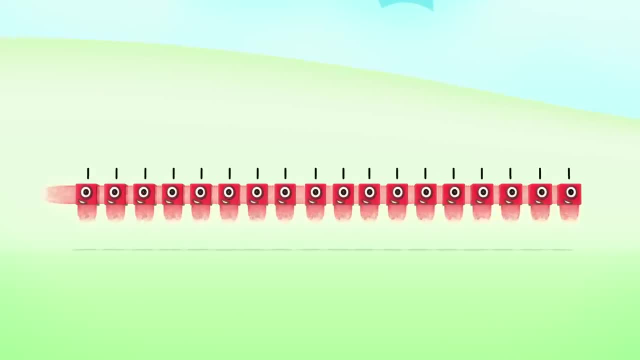 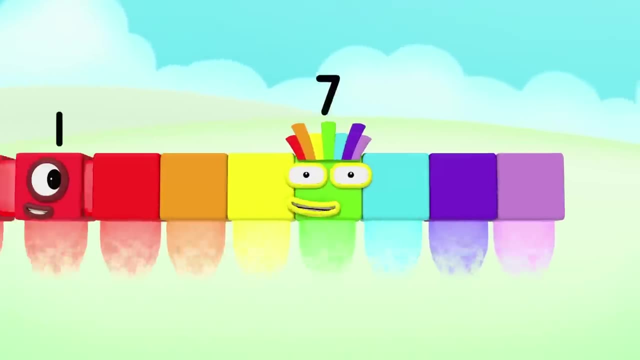 Ooh Ooh 18 once. this is fun Too fast. One, two, three, four, five, six, seven, eight, nine, ten, eleven, twelve, thirteen, fourteen, fifteen, sixteen, seventeen, eighteen. 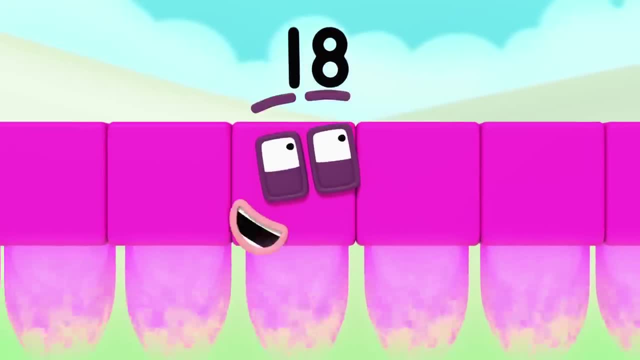 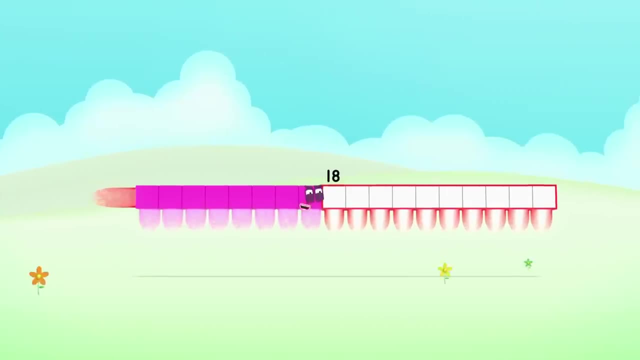 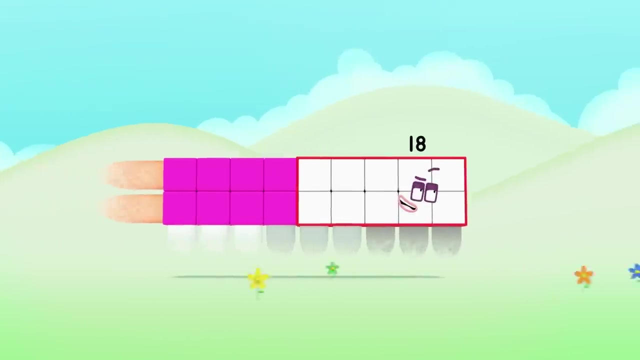 Ha. When it comes to acceleration, I'm the undisputed master. I'm the quickest in the nation. I change shape when I want to go faster. Switch Nine by two to race it away. I'm 18,. I'm a speed machine. I can set the world ablaze. 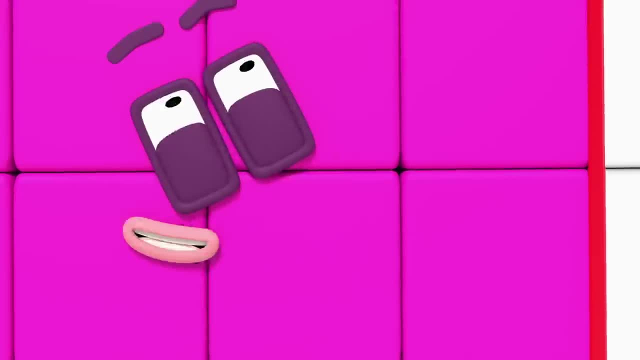 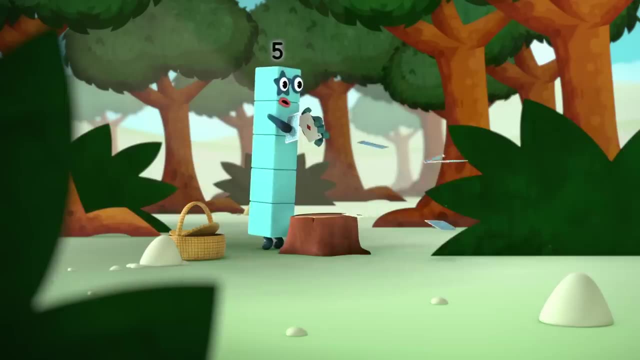 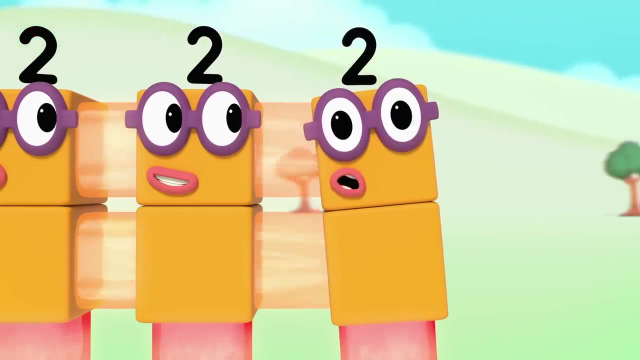 Watch me zoom with a sonic boom. I was born to ride the race. Wah-ha, Oh Oh, Nine twos, woo-hoo Ooh Ooh. Two, three, four, five, six, seven, eight, nine, ten, eleven, twelve, fourteen, fifteen, sixteen, eighteen. 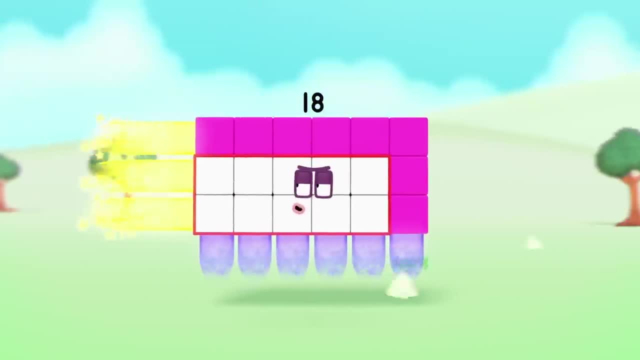 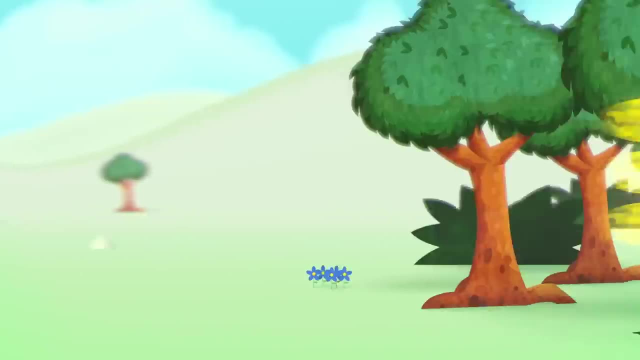 Brrrr Switch. Six by three. Three race are what I need. Three race and I build up speed, I start to glow and I go, go, go, Whoa, Whoa. Six, threes, yippee. 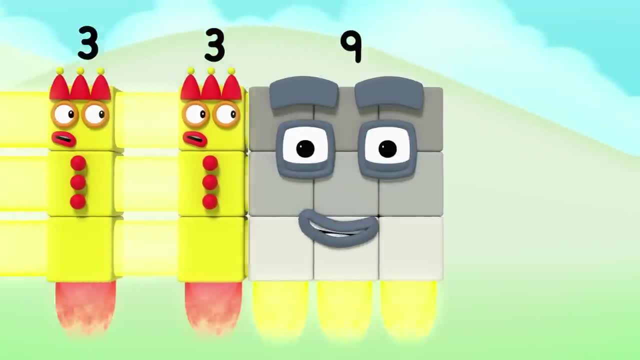 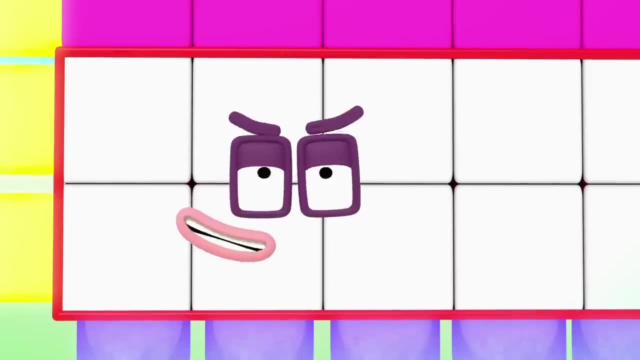 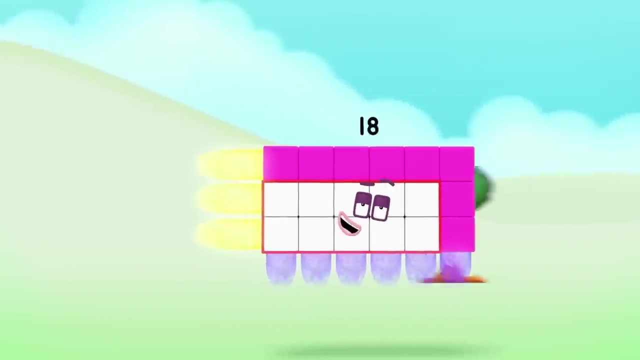 Too fast: Three, six, nine, twelve, fifteen, eighteen Cool times. When it comes to acceleration, I'm the undisputed master. I'm the quickest in the nation. I change shape when I want to go faster Turn. 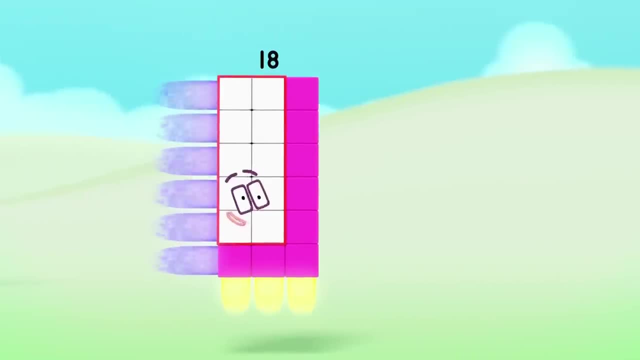 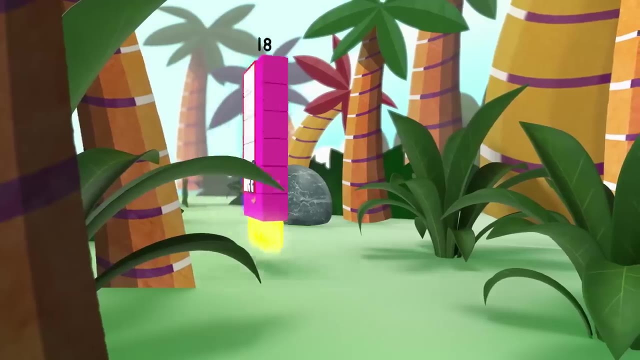 Three by six. Six race it away. One. I'm 18,, I'm a speed machine. I can set the world ablaze. Watch me zoom with a sonic boom. I was born to ride the race. Wah-ha, Woo-hoo. 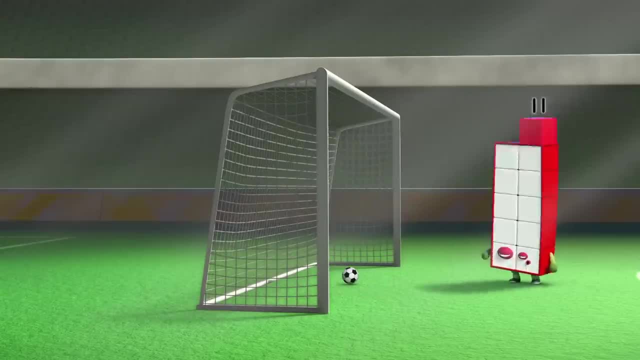 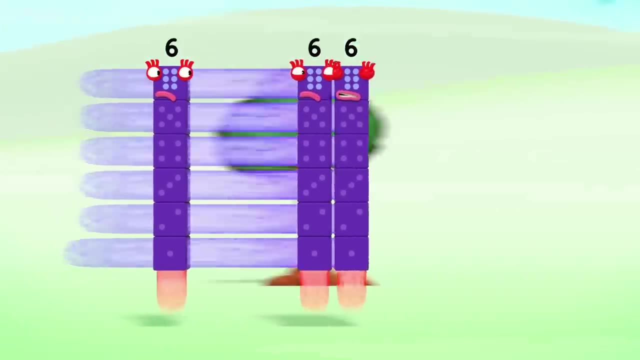 Woo-hoo, Woo-hoo, Whoa. Yeah, Three, sixes, let's remix this. We're coming past, we're going too fast. Yikes, Six, twelve, eighteen, Me again Switch Two by nine. 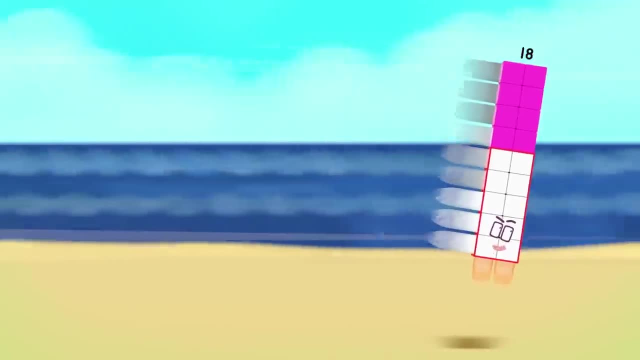 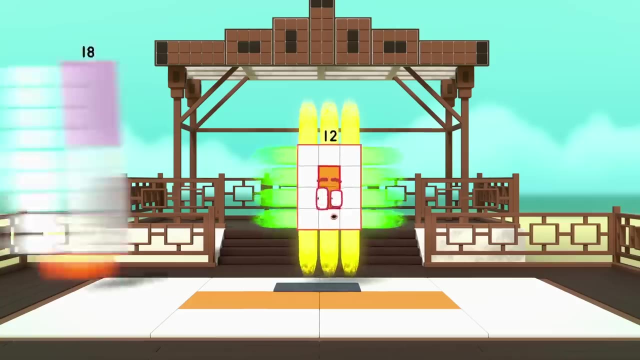 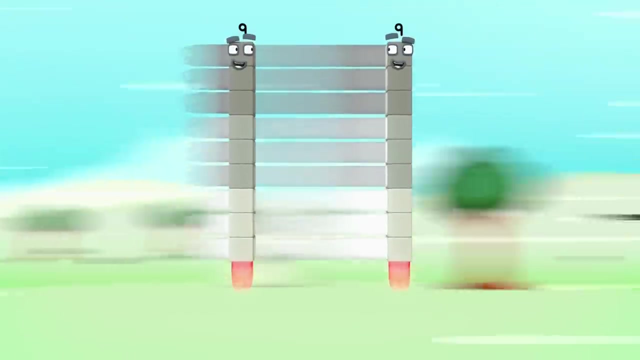 Nine race are what I need. Nine race and I build up speed, I start to glow and I go, go, go, Ah, Three by four, Whoa, Whoa-whoa-whoa, Whoa, Ah, Two, nines. 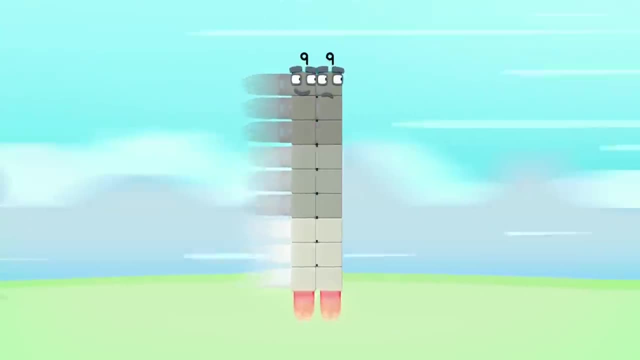 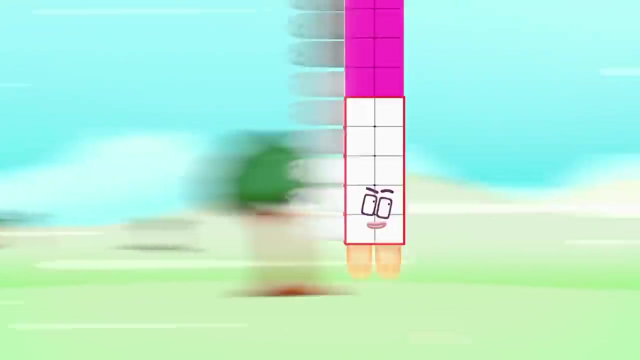 Parallel lines. Whoa-ho-ho, Nine, Eighteen, Did you miss me? When it comes to acceleration, I'm the undisputed master. I'm the quickest in the nation. I change shape when I want to go faster. 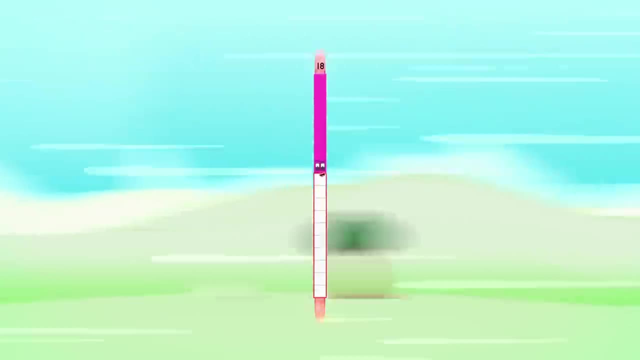 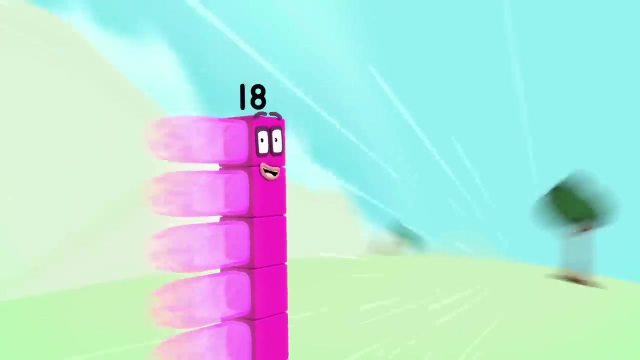 Ready for the big one? Switch One by eighteen. Eighteen, race it away. I'm so fast I'll be out of the gate Before you can lock it. I go at a rate no one can clock it. I'm ten and eight, I'm never late. 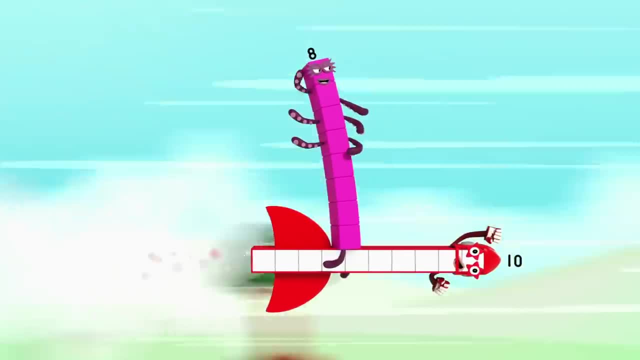 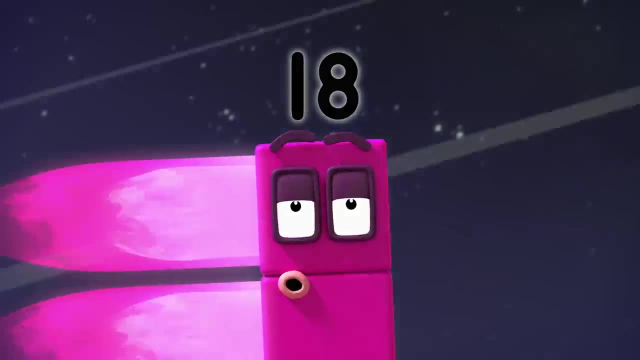 I'm Foxes, Locker and Rockets. Yee-haw, I'm eighteen. I'm a speed machine. I can set the world ablaze. Watch me zoom with a sonic boom. I was born to ride the rays Round the world. 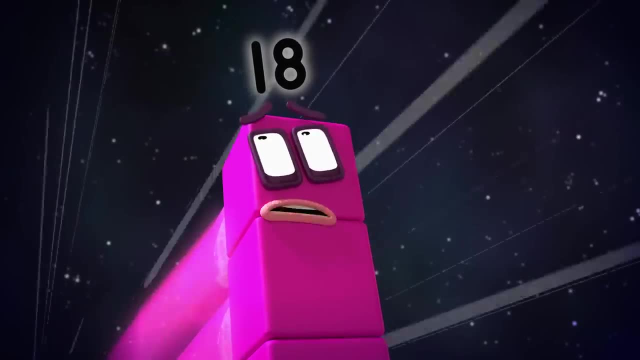 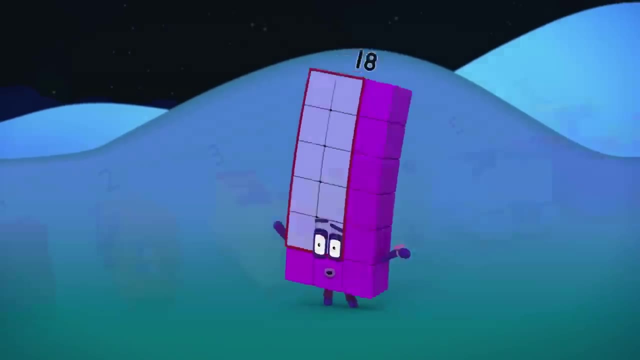 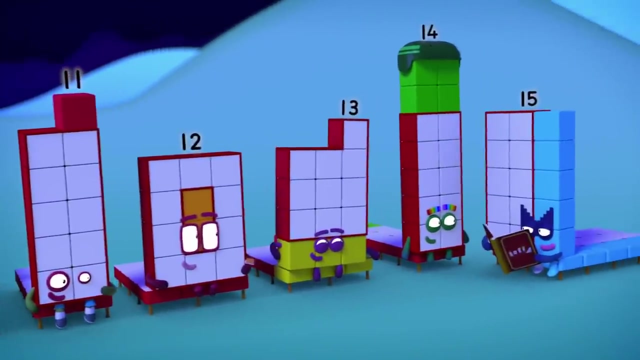 Whoa-whoa-whoa-whoa-whoa. Um, how do I stop this thing? Blam, Woo-hoo, Ooh, that's one way to do it. Blah. If you're sitting comfortably, then I'll begin. 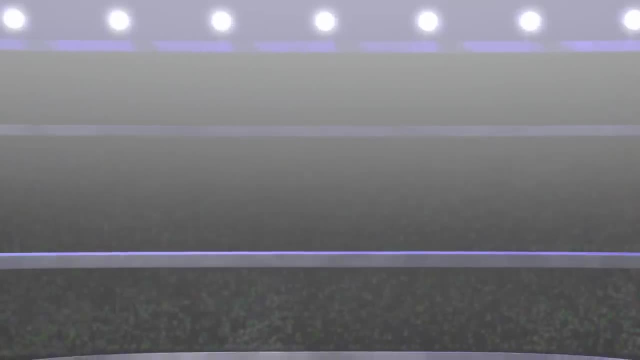 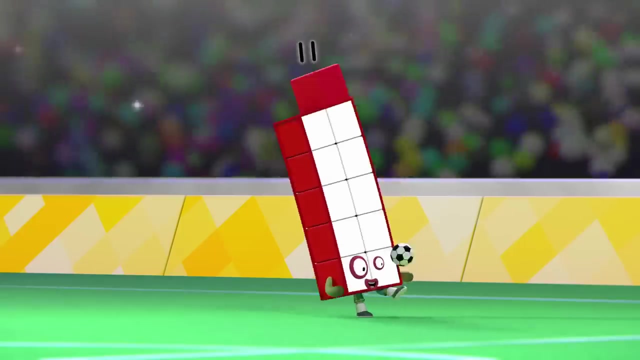 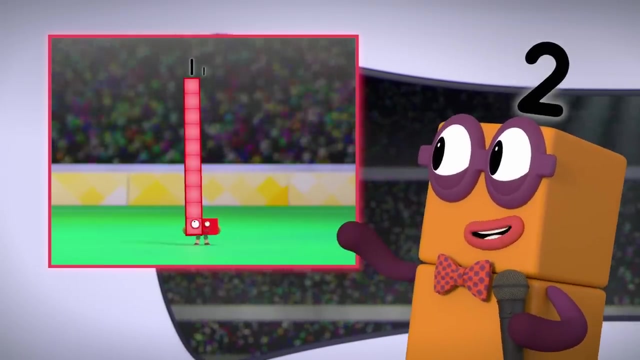 Chapter 11, Back of the Net. With time running out and the score tied at ten goals each, this free kick could decide it all. I am eleven and I love football. Her numbering's there, Standing for one ten-block and one block more. 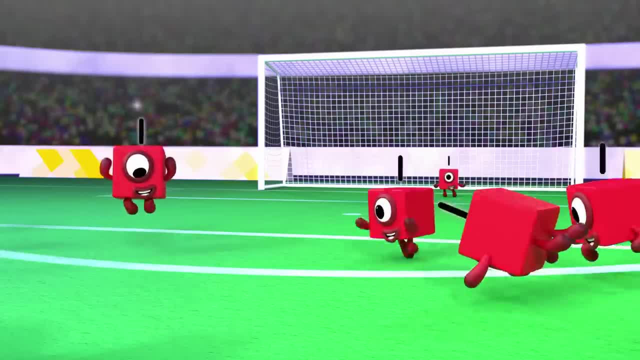 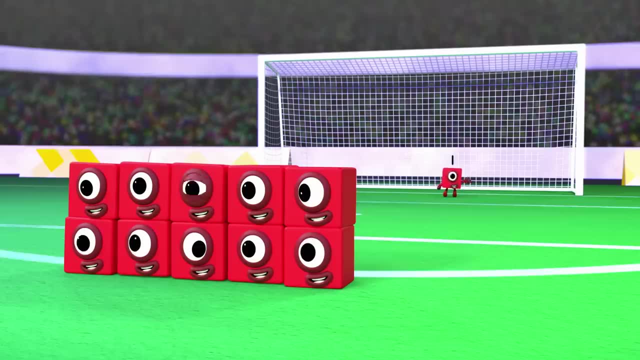 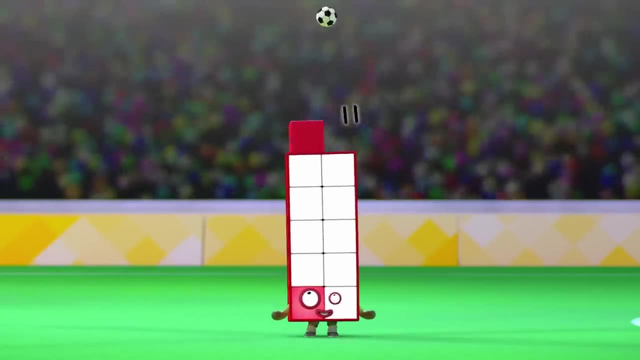 Ten and one making eleven. The defending team Wounds United get to make a wall. One, ten, Ten ones And one more in goal is eleven ones to beat. One, two, three, four, five, six, seven, eight, nine and ten. 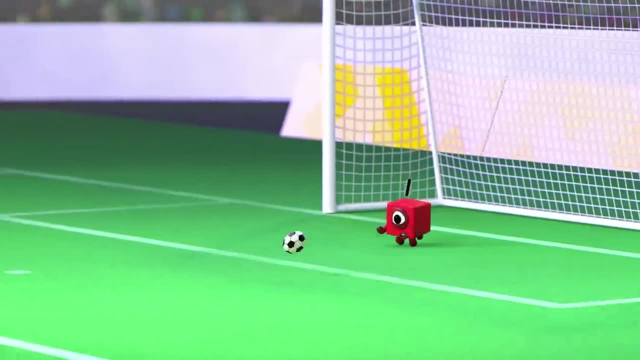 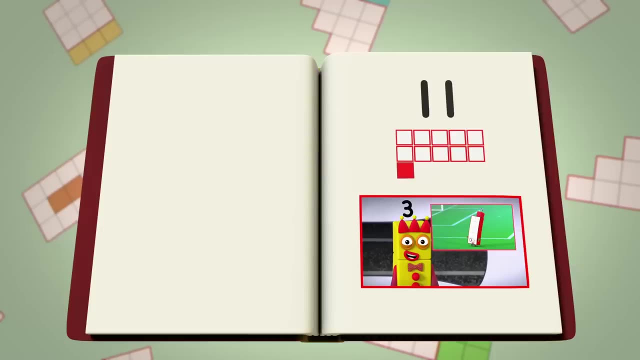 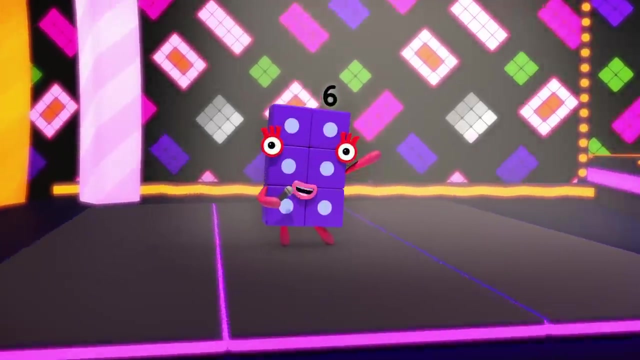 And one more is eleven. She shoots, She scores One, ten, One, one. There's only one: eleven. Chapter 12, Rectangle Rush. Yay, Welcome to Rectangle Rush. Let's see who's next to brave the crush, Yeah. 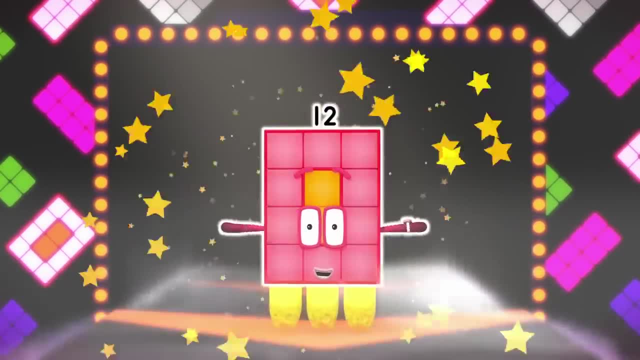 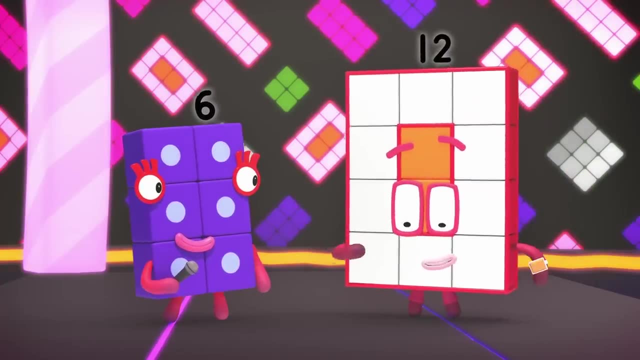 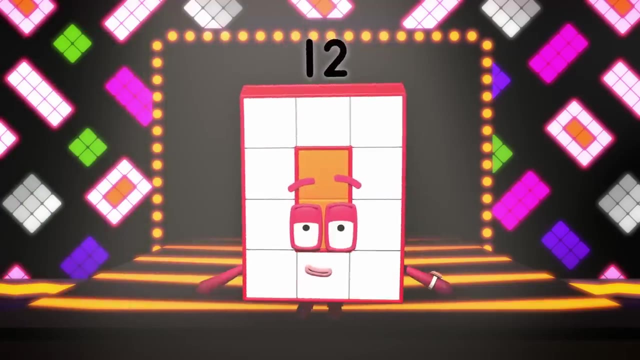 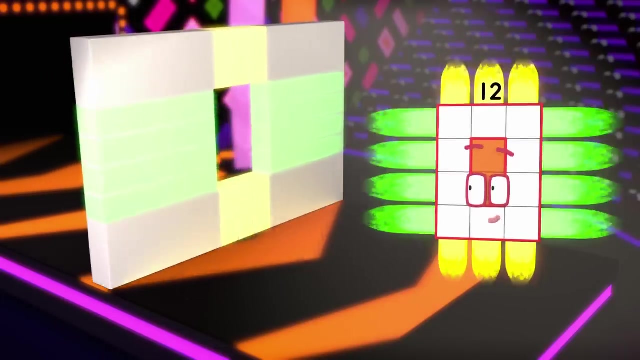 Woo-hoo, I am 12 and I am a super rectangle. Woo-hoo, That means I can make lots of different rectangles. Show us what you've got. Game on, I am 12.. I am ten and two And I am three. blocks by four blocks. 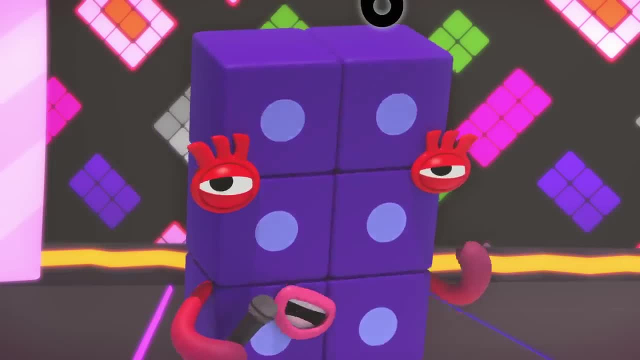 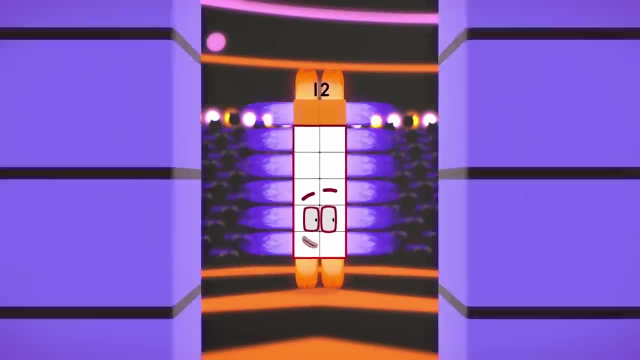 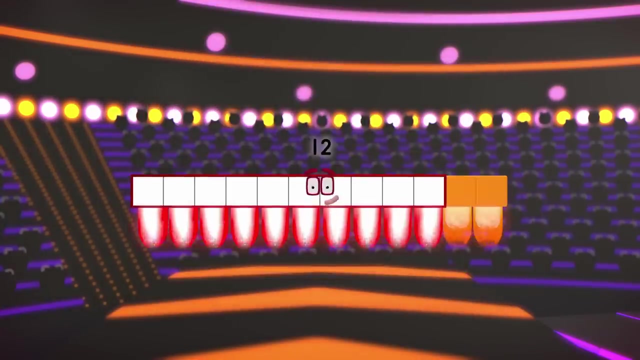 I am a rectangle, Ooh, Rectangle, raise Turn. I am four by three Switch. I am two by six Turn. I am six by two Turn. I am six by two Switch. I am 12 by one. 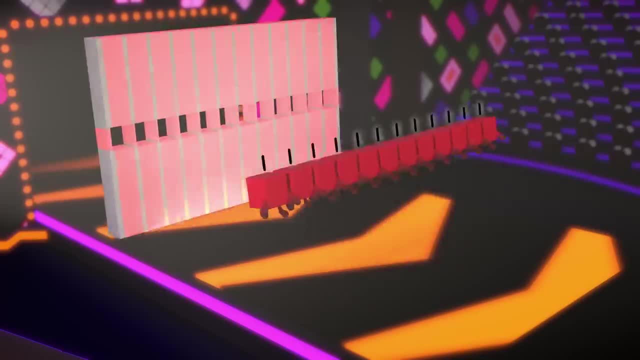 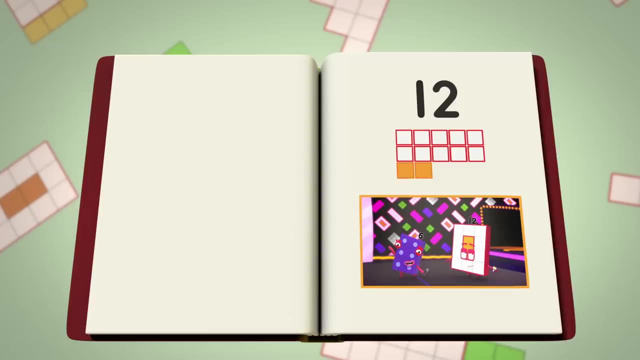 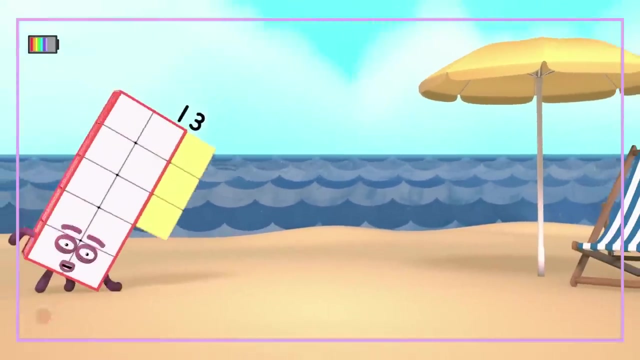 Switch. I am 12 by one, Which means I am also 12 blocks of one. Ha-ha-ha-ha-ha, Yay, Yay, Chapter 13.. Oops, Unlucky me Um ready one. 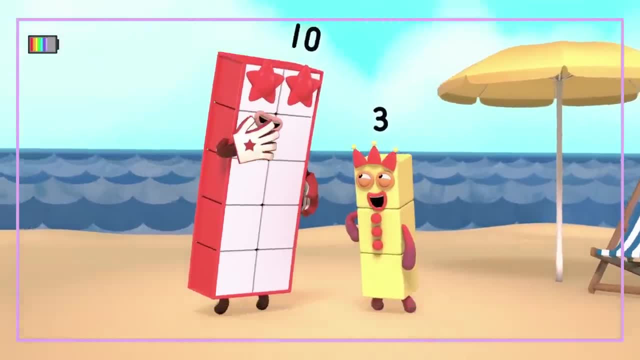 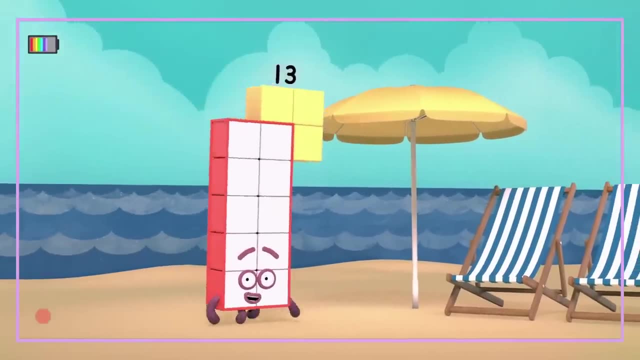 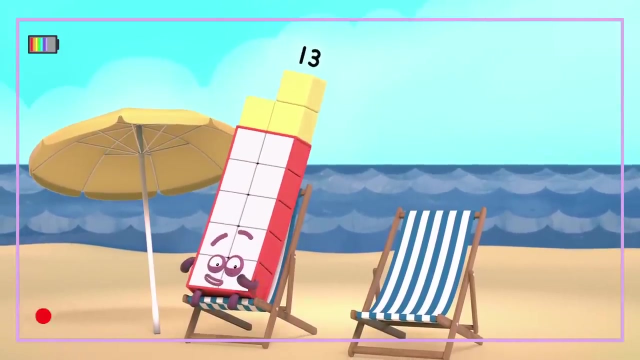 Ready 13!? Oh Oh, Cut. Oh sorry, My three falls off any time anyone says 13!. Ha-ha-ha, Cut Right Third time lucky. I'm ten and three. I am 13!. 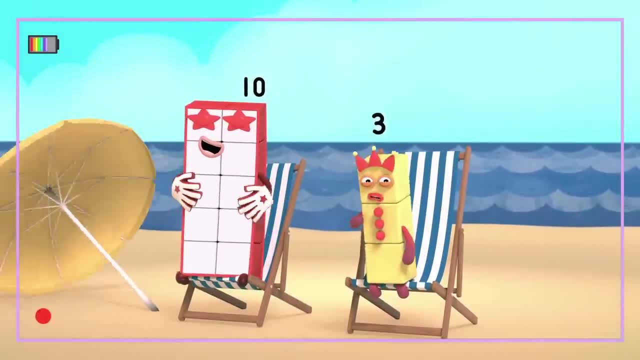 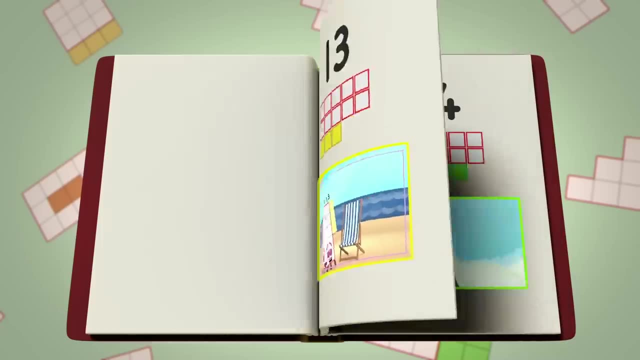 Ooh, Ha-ha-ha-ha. Ten and three Ha-ha-ha-ha, I'm lucky. Three Ha-ha-ha-ha Ooh. Chapter 14. Downhill all the way, dude. 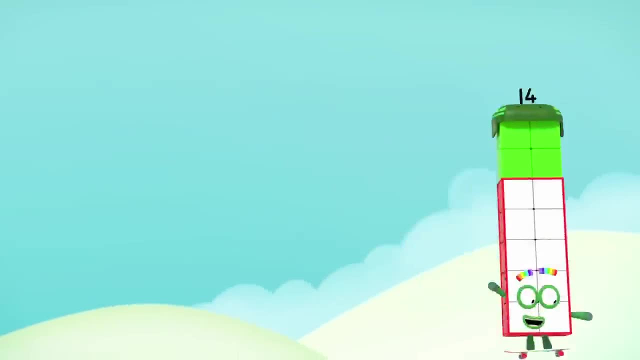 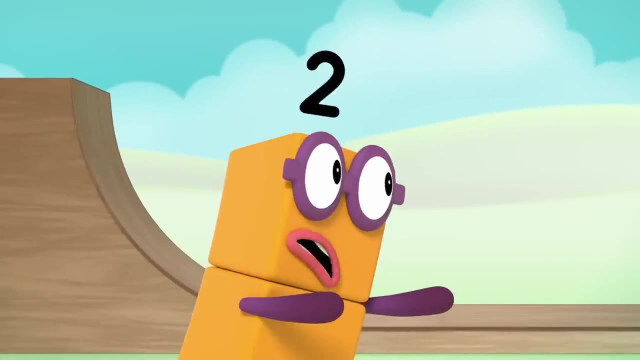 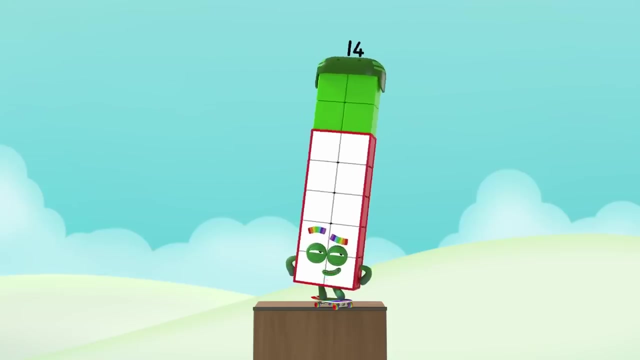 Whoa Hang ten Plus four. I'm extreme 14!. Check this out. Woo-hoo, 14!. Wait, Wait, The track splits in two. Worry not, bro, I'm 14!, I'm not just lucky. 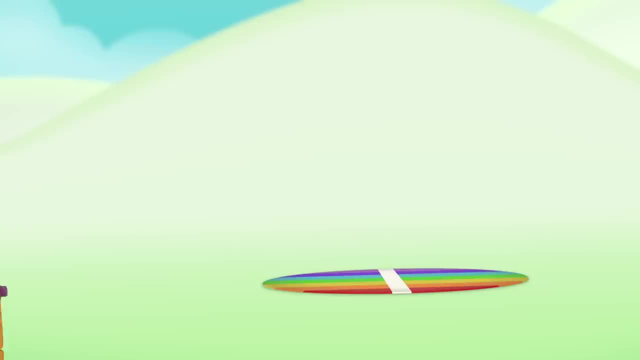 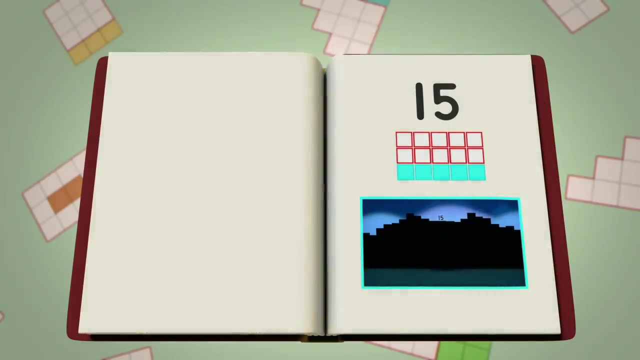 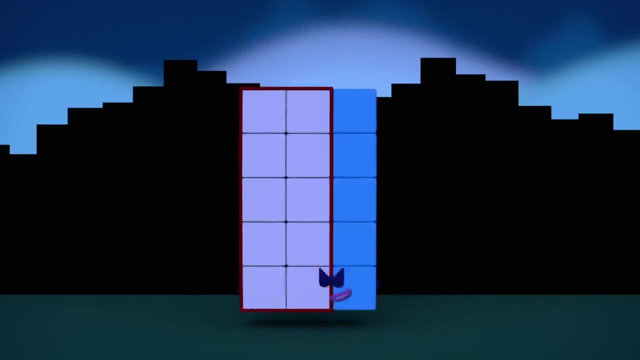 I'm double seven, Double lucky Woo-hoo. Hey, Tens, Chapter 15.. Night Mission: Hush-hush Agent 15. here You may know me as Ten And five, But on the quiet I'm also. 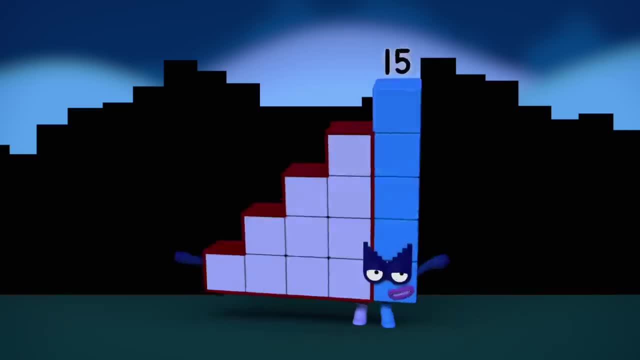 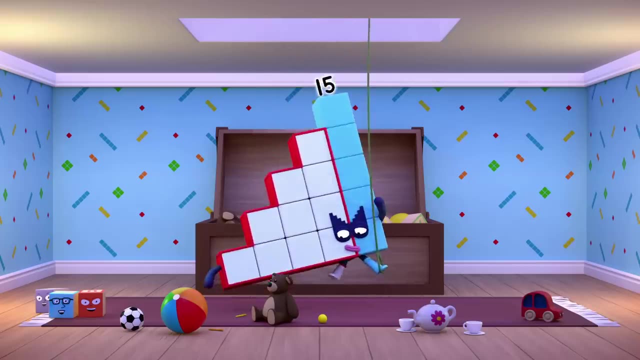 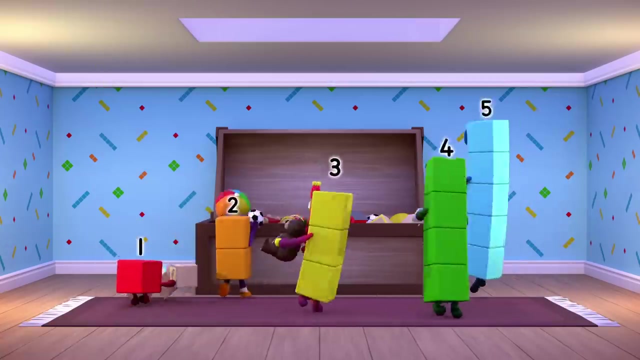 One plus two plus three plus four plus five. That's right, I'm Super Special Secret Step Squad, Super Special Secret Step Squad On a top-secret night-time mission, On a top-secret night-time mission. Step one: tidy, Step two: drink cocoa. 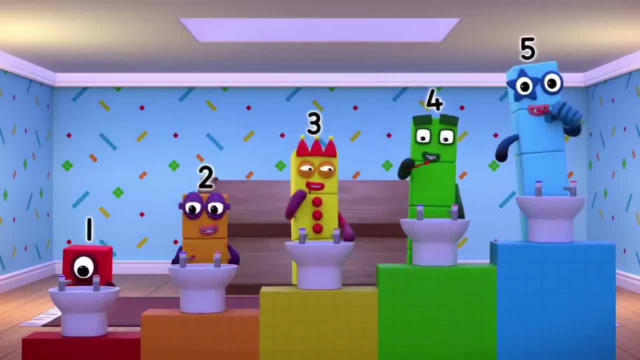 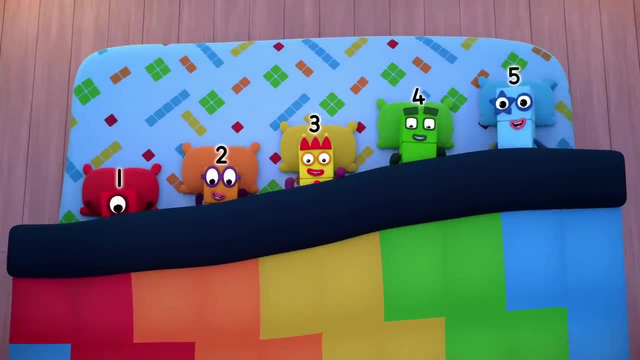 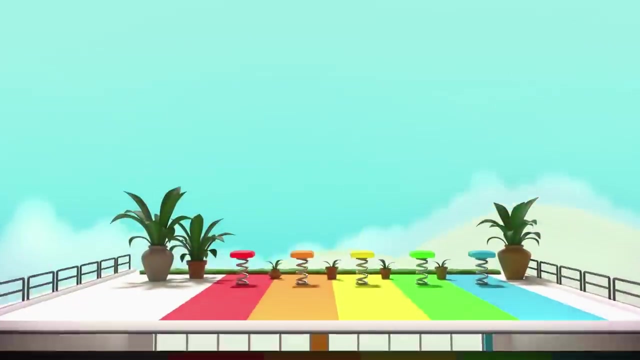 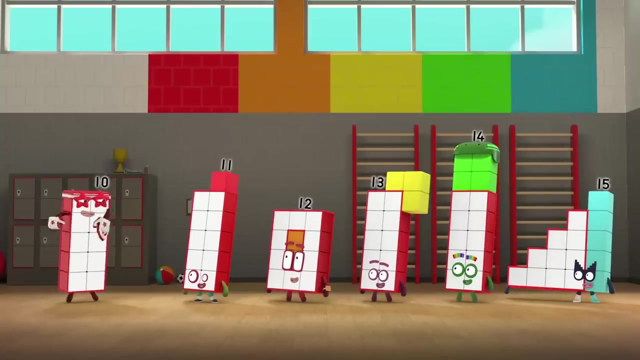 Mmm. Step three: brush our teeth. Step four: get on to the bed. Step five: read a nice bedtime story. Step five: read a nice bedtime story. Step six: pray What And six, It'll be alright. 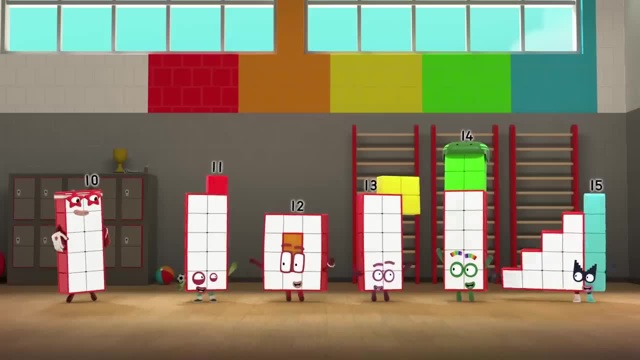 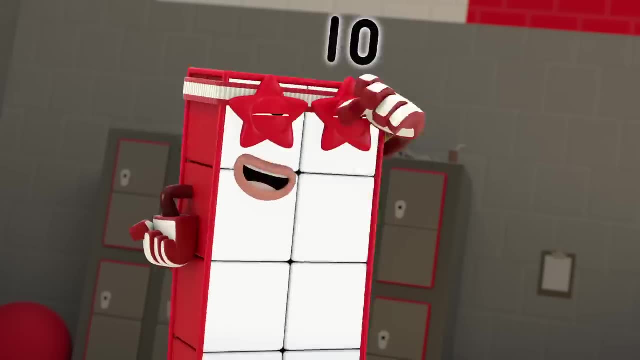 How's it going, guys? Go on, you guys. What an Bunnies. Bless, Bumblebee and surgical. Welcome to Ten's Place. All of you are bigger than me. Oh, That means each of you has a ten inside you. 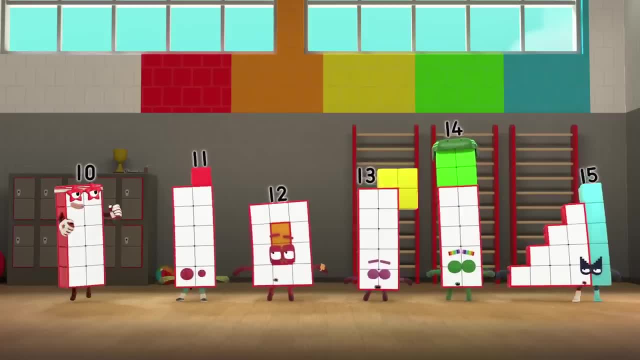 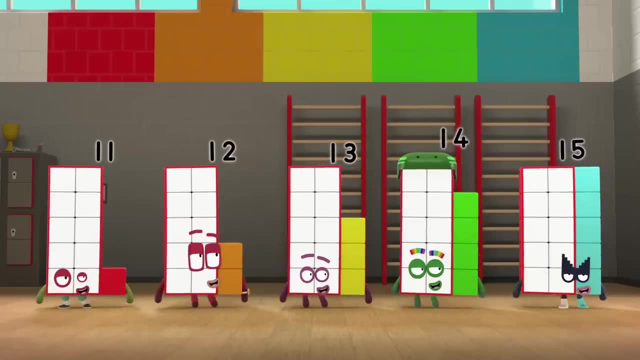 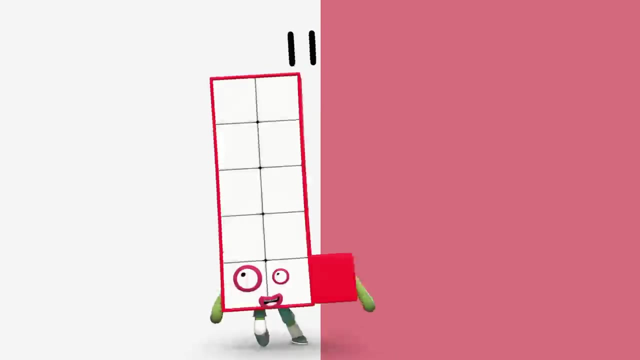 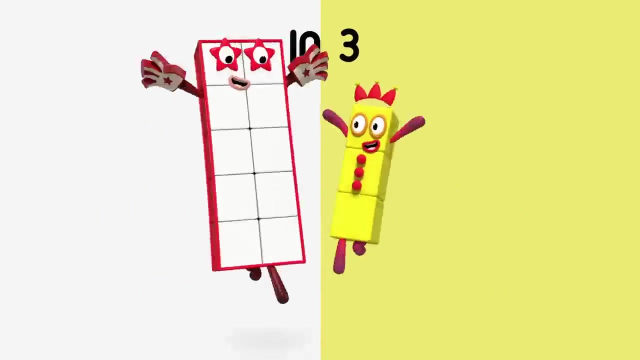 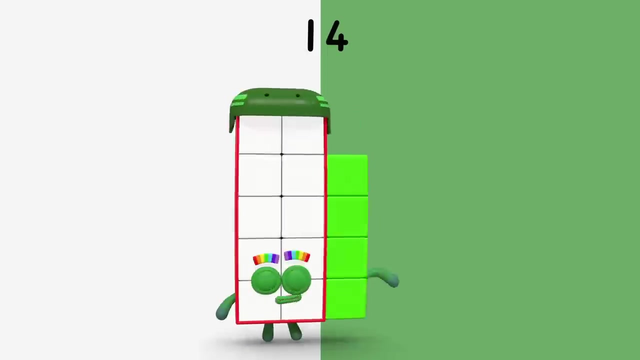 That's right Now give me some squats. Let me see you do the jump and bump. 10 plus 1 is 11. 10 plus 2 is 12, 10 plus 3 is 13. 10 plus 4 is 14. 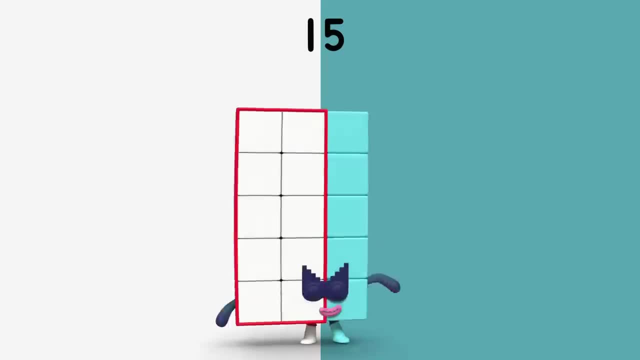 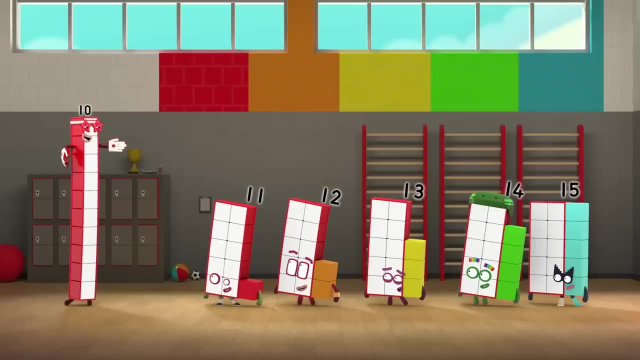 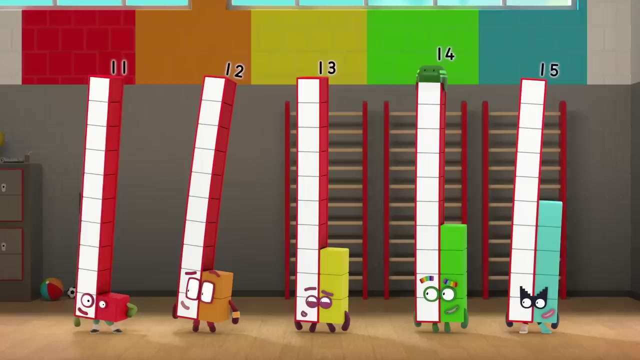 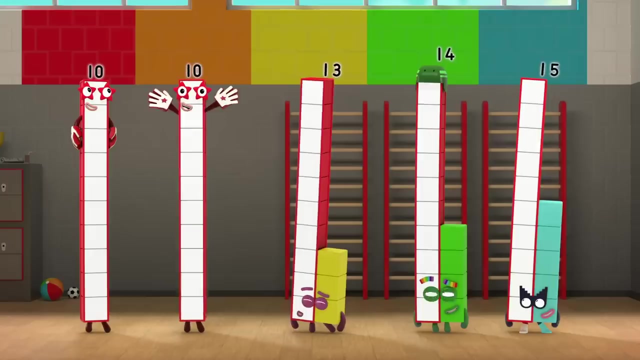 10 plus 5 is 15. Terrific, Now let's stretch our 10s. Nice and tall. Bling those ones high in the air. Take it away. 11 minus 1 is 10. 12 minus 10 is 10. 13 minus 3 is 10. 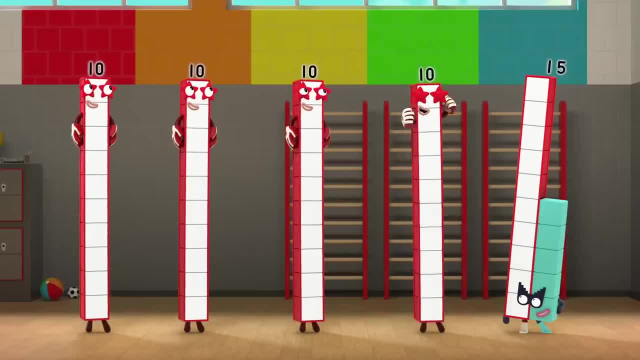 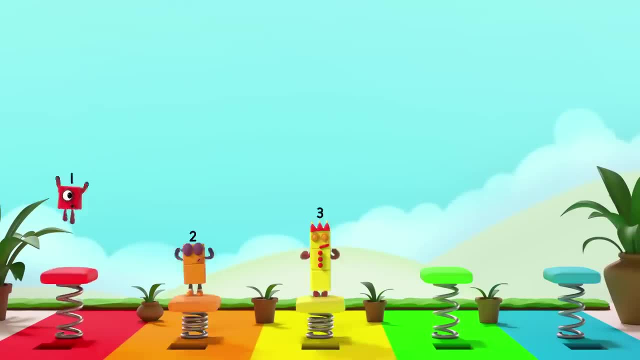 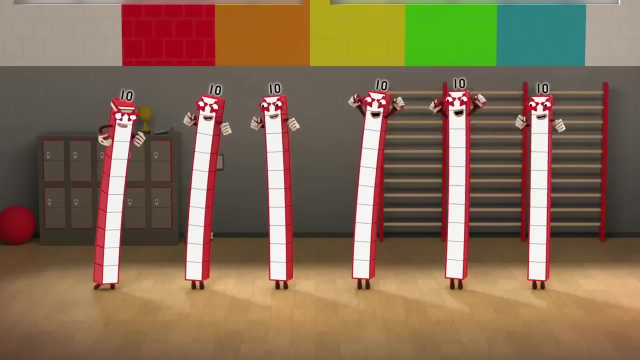 14 minus 4 is 10. 15 minus 5 is 10. 1, 2 ones, 3 ones, 4 ones, 5 ones. Ready, Let's work those 10s. Yeah, Tall slide 2-eyes. 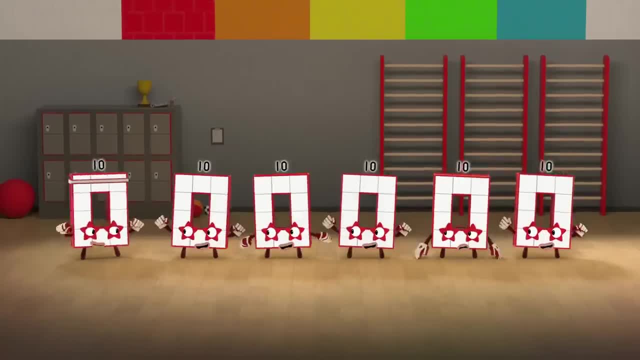 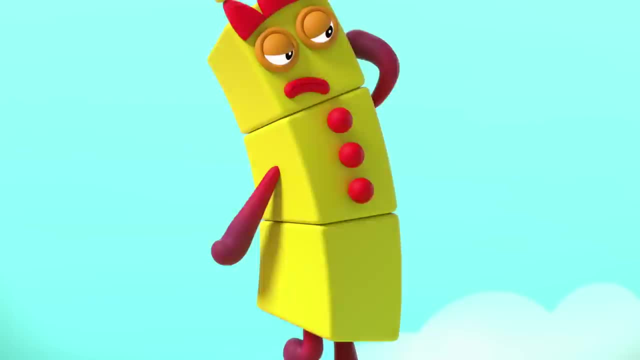 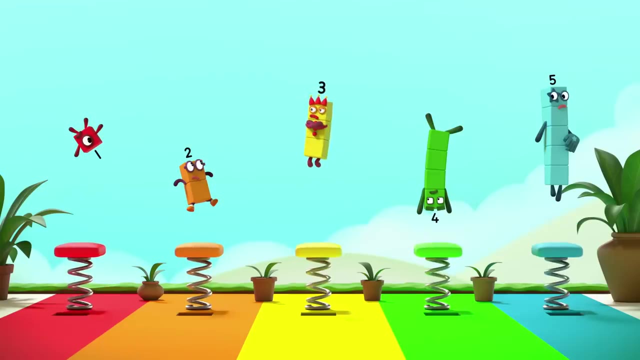 Slide and go low, Rectangle with a hole And freestyle: Yeah, Boing-boing, boing-boing, boing-boing, Stop, stop, stop. If this is 10s place, where are the 10s? Um, I say we make this floor 3s place. 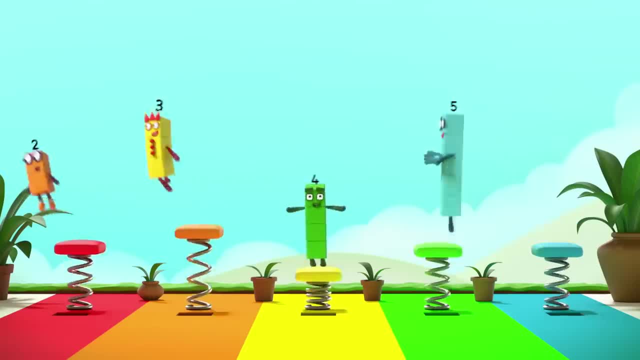 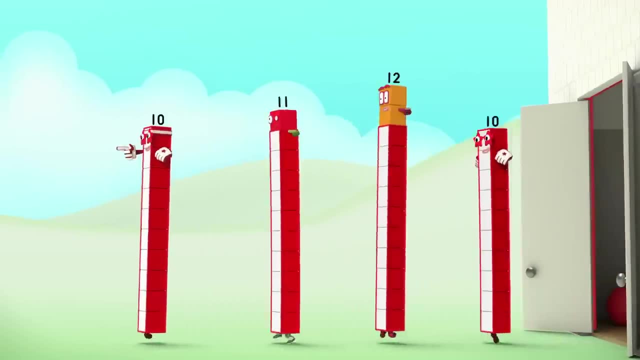 Everyone off Boing-boing, boing-boing, boing-boing, Boing, boing, boing, boing-boing, boing-boing. 10, 11, 12, 13, Wahoo, 14, 15. Welcome to. 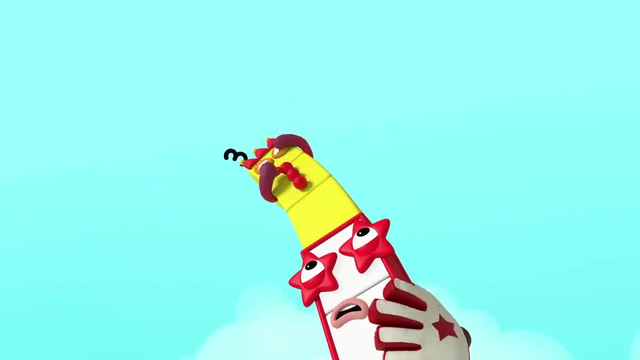 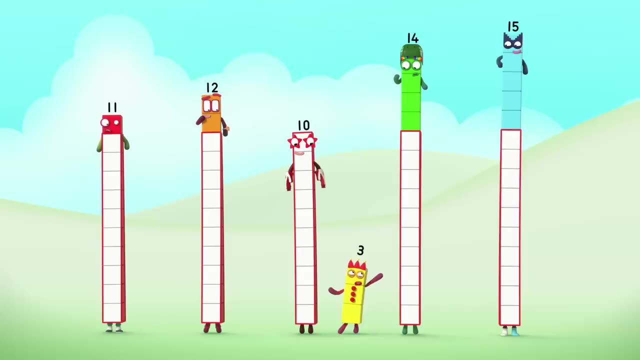 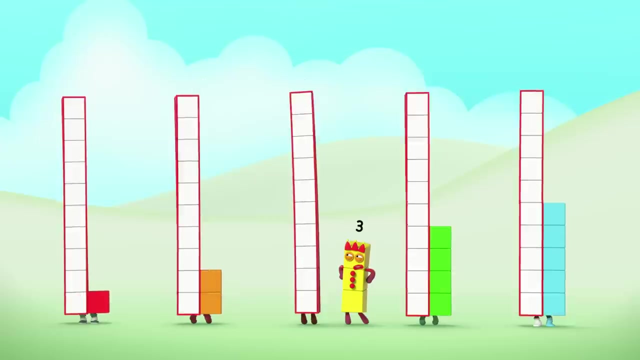 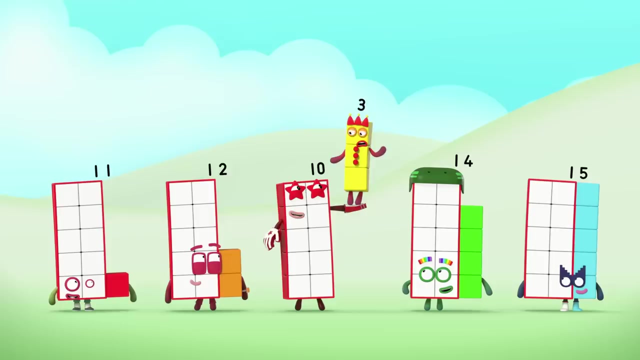 It's a bit high up here, put me down. All of you are bigger than me, So make yourselves shorter, Even shorter. Let's go. You've all got a three inside you. Well, except for thirteen. He already pinged the part into ten and me. 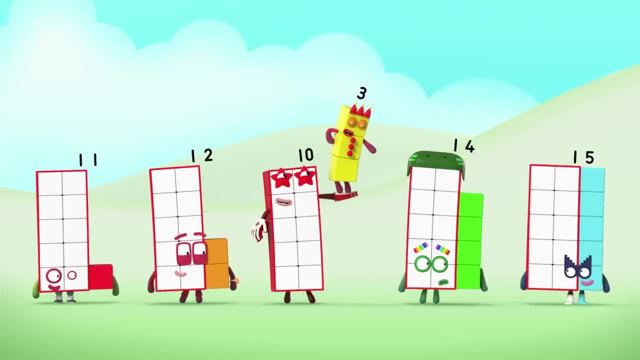 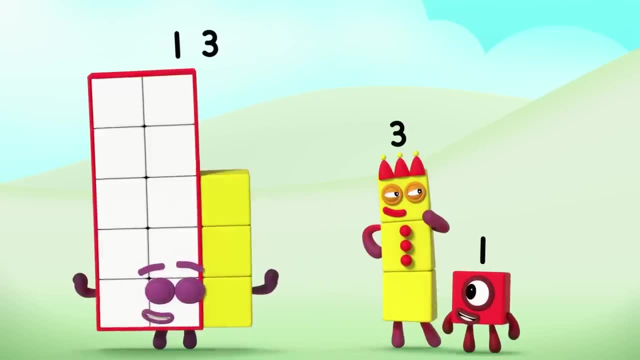 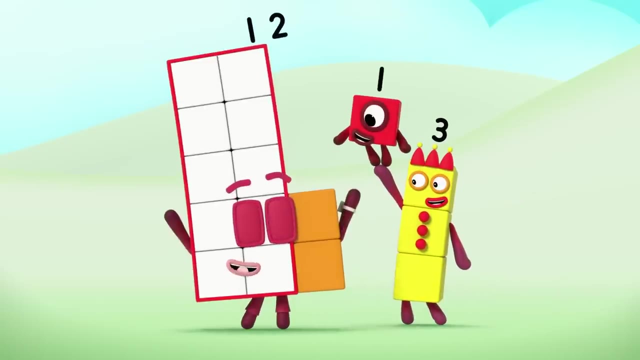 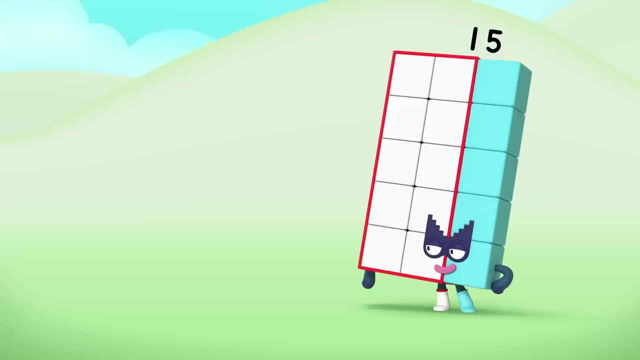 Fourteen, You're one more than thirteen. Extreme fourteen Minus one Equals thirteen. And for my next trick, twelve Plus one equals ten and three. Your turn fifteen. Let's say ten and five, but I want ten and three, And three is two less than five. 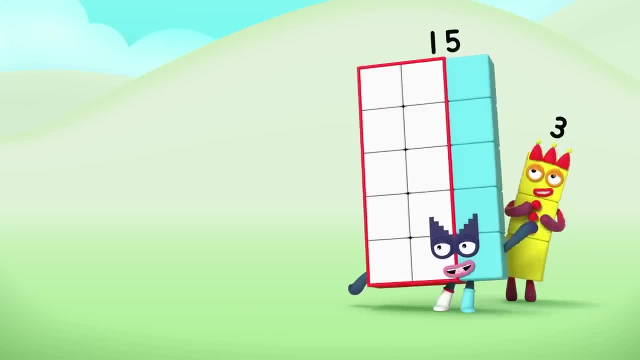 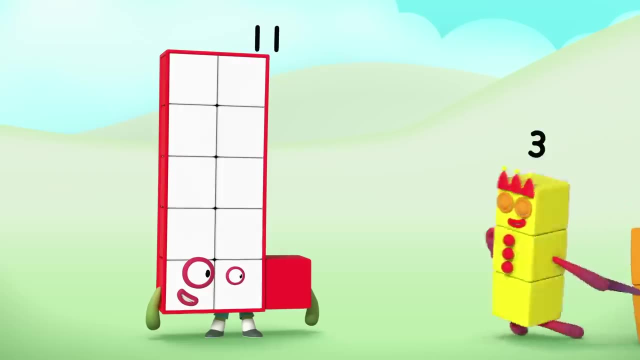 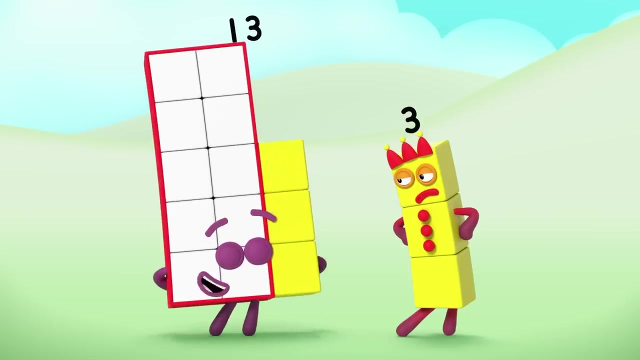 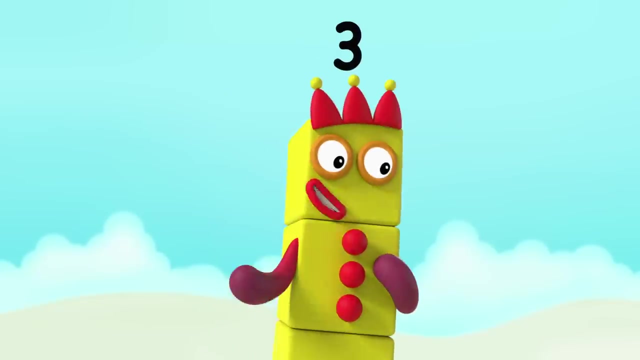 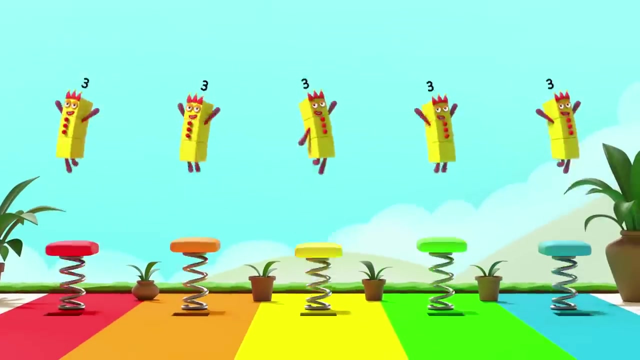 So let's pop off a two, Ten and five Minus two Equals ten and three. Ten and one Plus two Equals Three. Only joking: ten and three. There now, everybody stand tall When I say: go, go, go, my lovely thirteen, Welcome to Three's Place. 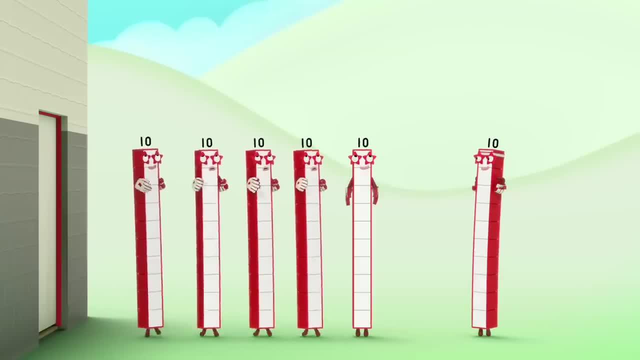 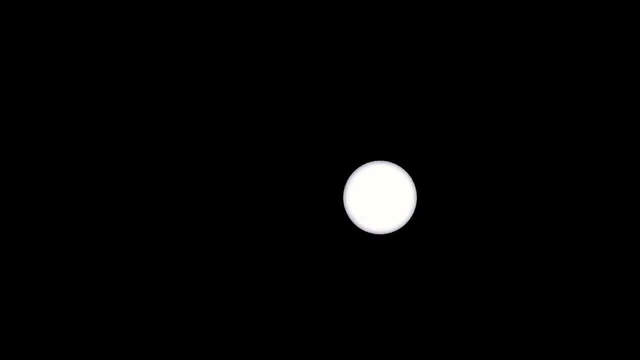 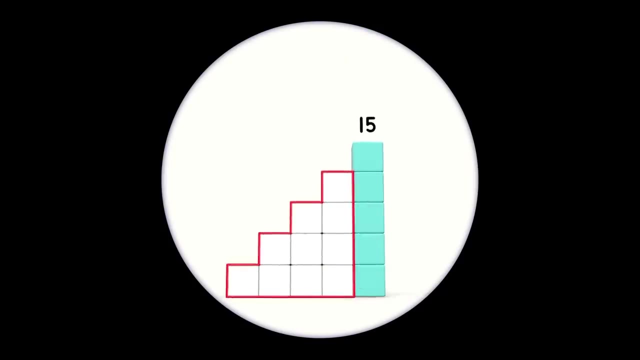 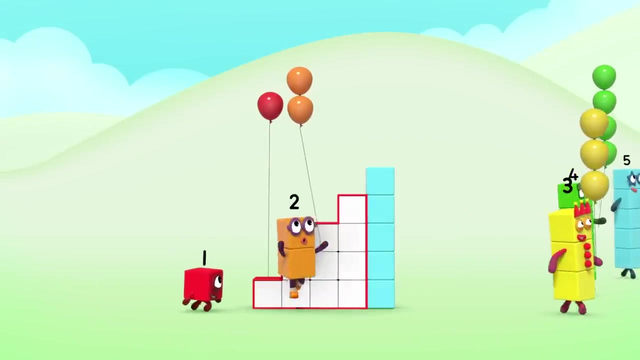 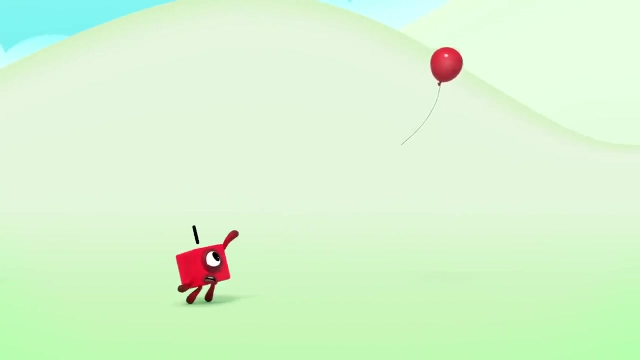 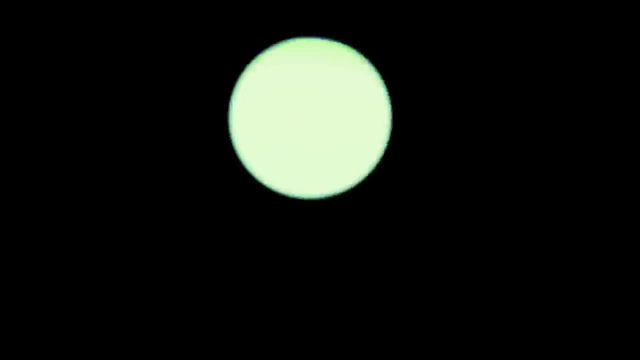 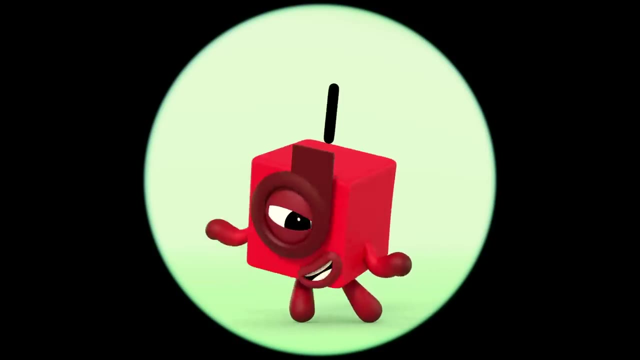 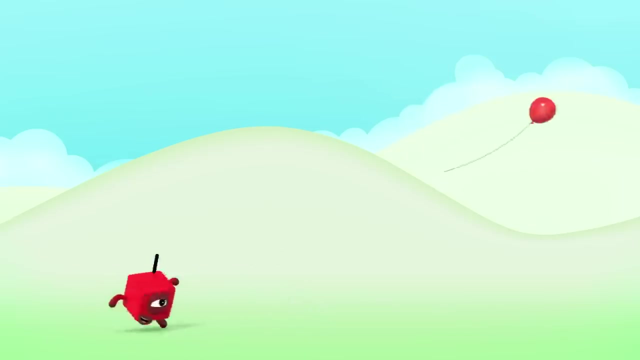 The super special secret, Step Squad is here. Oh me, A Step Squad, all by myself. I'll give it a go Step one. Okay, go Step one. My plan is working perfectly. Push, push-. One Plus two Equals Three. Ec Google three, One, two, three, Three escaped balloons. If only Step Squad were here. 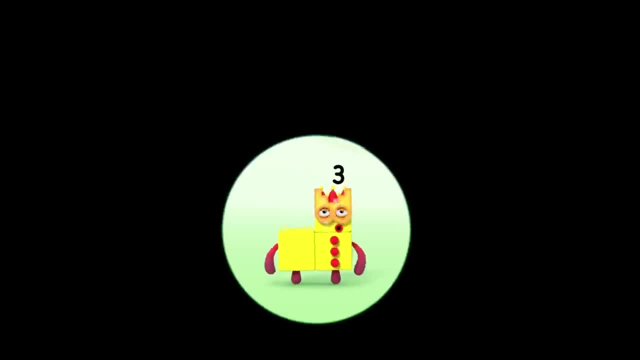 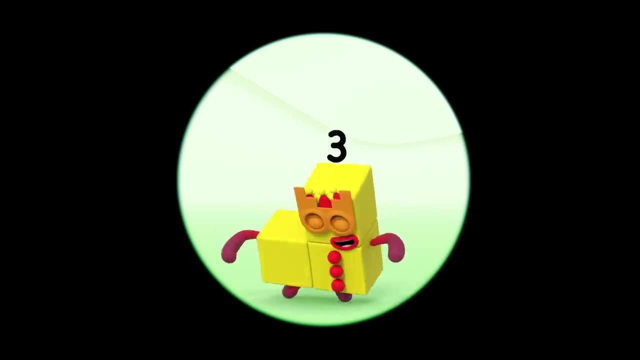 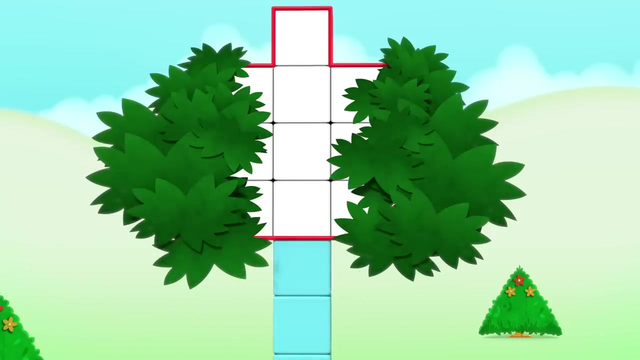 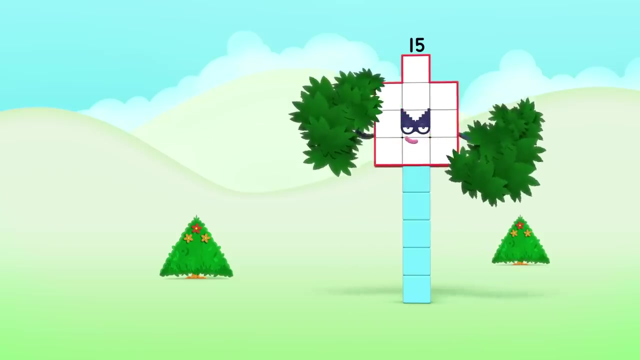 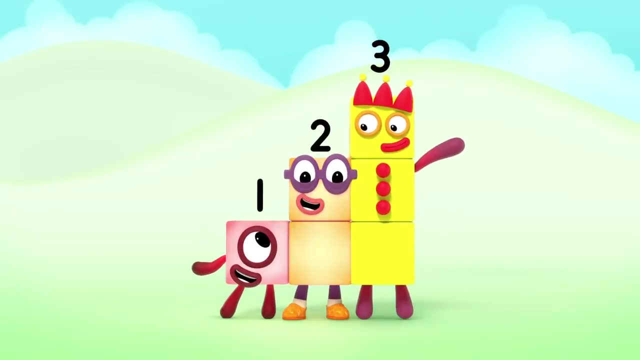 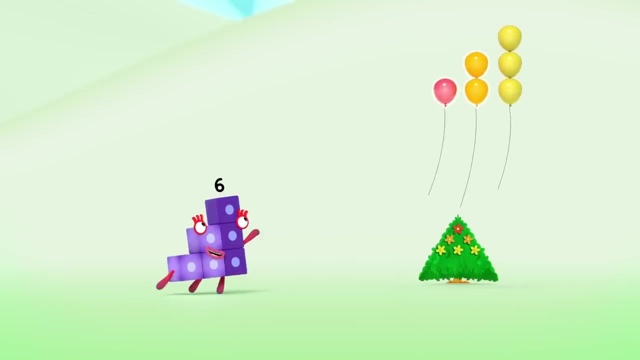 The super special, secret Step Squad is here. Look at me, I'm step shaped too. Maybe I can be a Step Squad. Step one, chase, Step two, peddling hard, Hush, hush The count. One plus two plus three equals six. One, two, three, four, five. 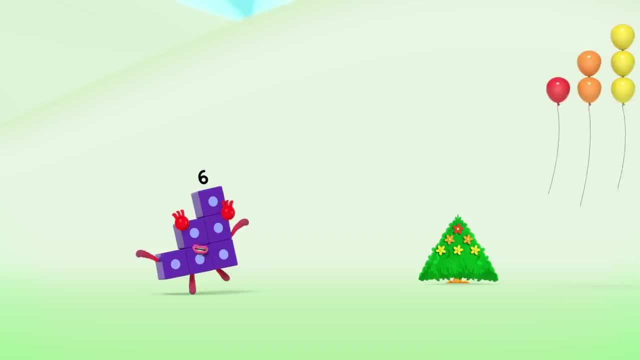 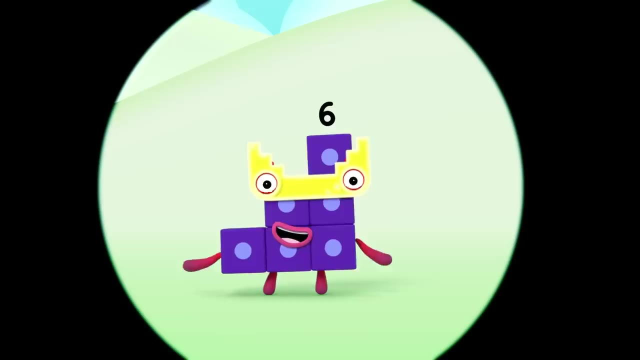 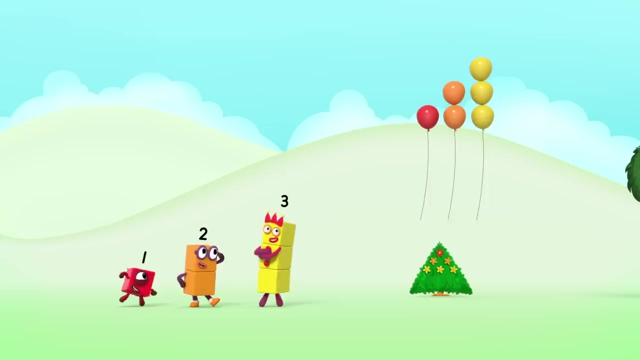 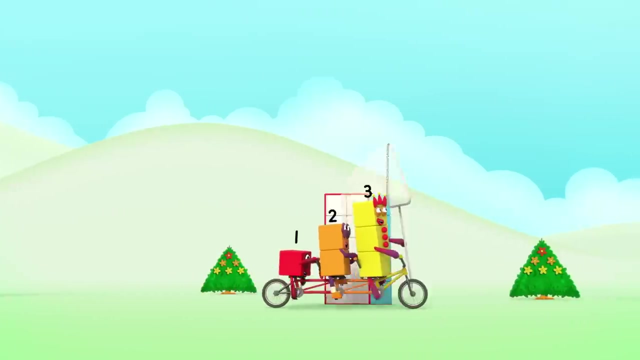 six, Six balloons have now been freed. I know exactly who we need. The super special secret Step Squad is here. Look. Step one chase. That must be true. I can be a Step Squad too. Step one chase. Step two, peddling hard. Step three with a net: Hush, hush. 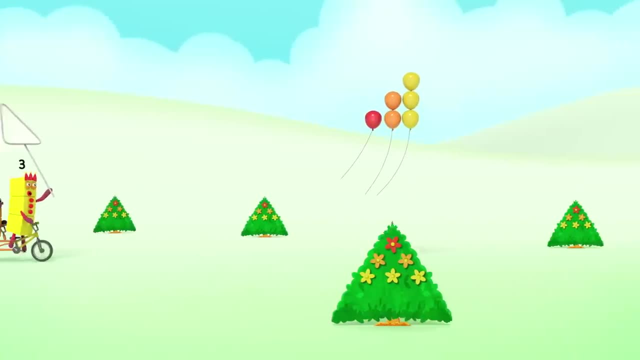 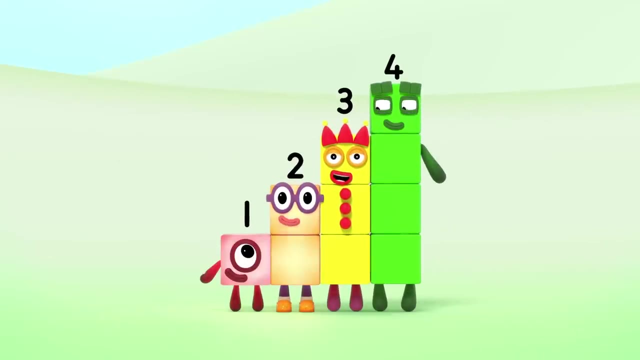 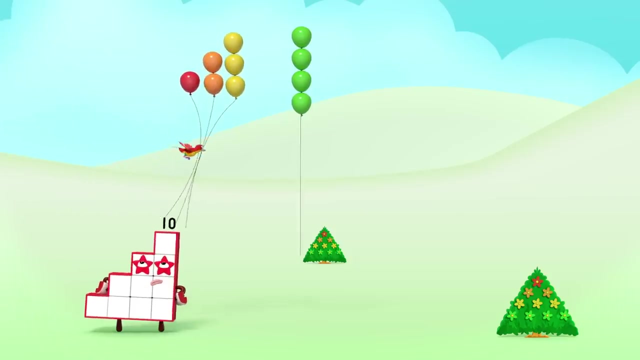 Hey, Whoa, One plus two Plus three Plus four equals six. This is okay, There I'm faster, Yep. Where to now To blow up the hill? You naughty bird, You bring those one, two, three, four, five, six, seven, eight, nine, ten, ten balloons back. 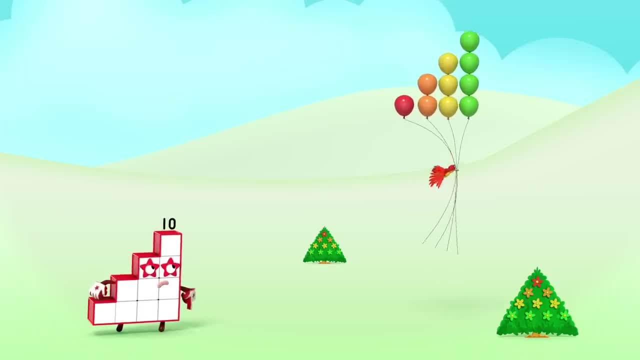 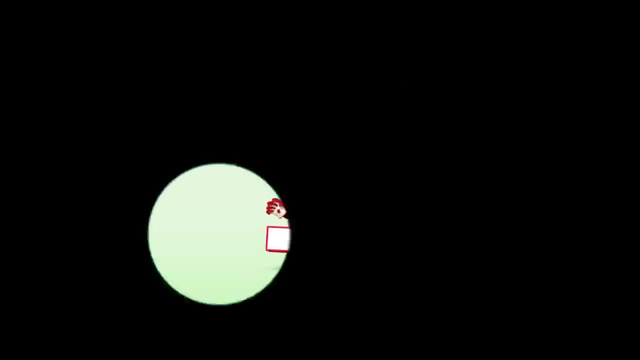 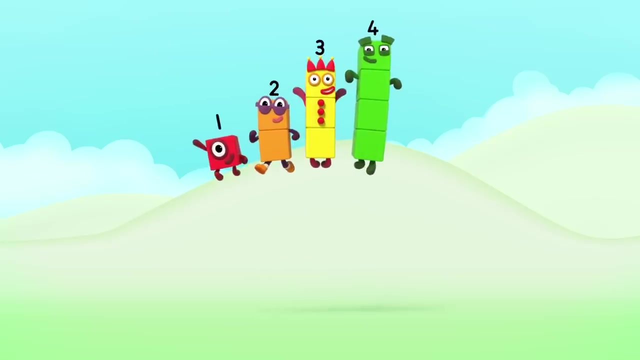 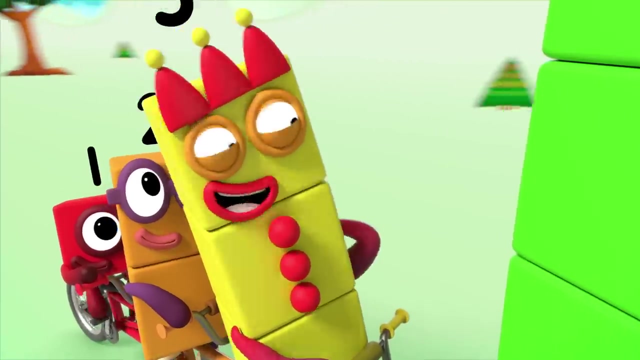 I need Step Squad. The super special secret Step Squad is here. Can it be? Yes, it can. I'm a Step Squad too. Step one: chase. Step two: peddling hard. Step three with a net. Step four: press the square button. 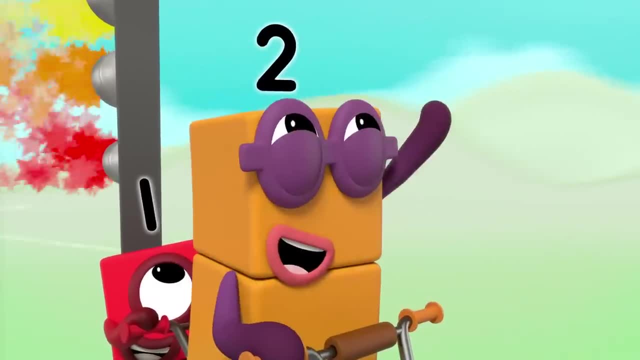 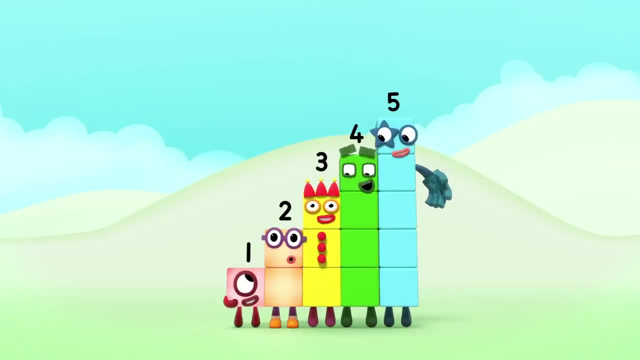 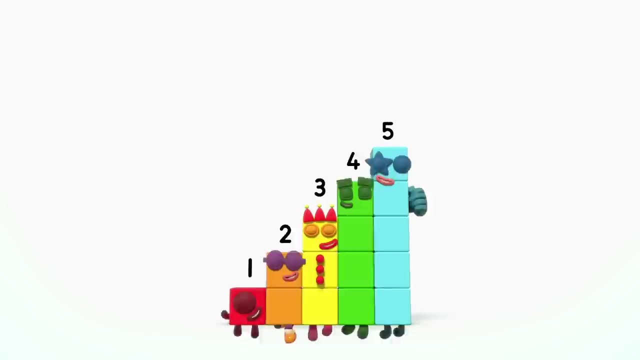 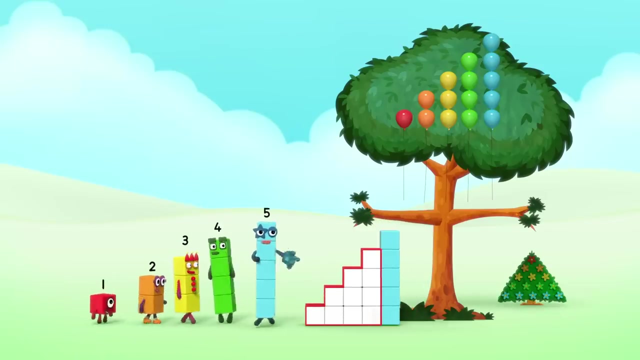 Grab them. One Plus two Plus three Plus four Plus five: Equals One Plus two Plus three: Equals Fifteen. The super special secret Step Squad is here. Step Squad off the steps, Step Squad down the steps. 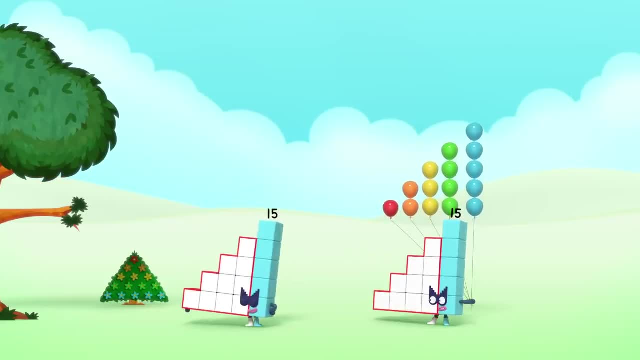 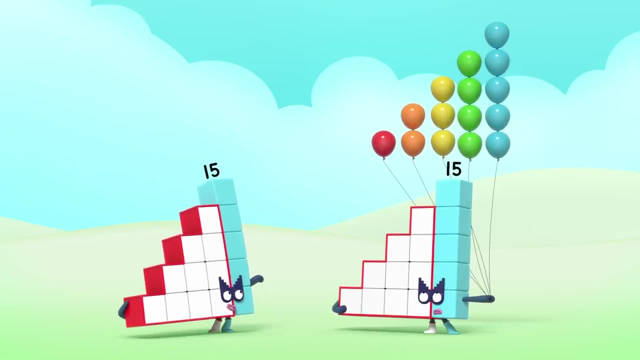 Agent 15.. Does this make me a double agent? You passed my test with flying colors: Good: Orange, yellow, green and blue. Well done all of you, All of us, All of you. Step Squads Fifteen. 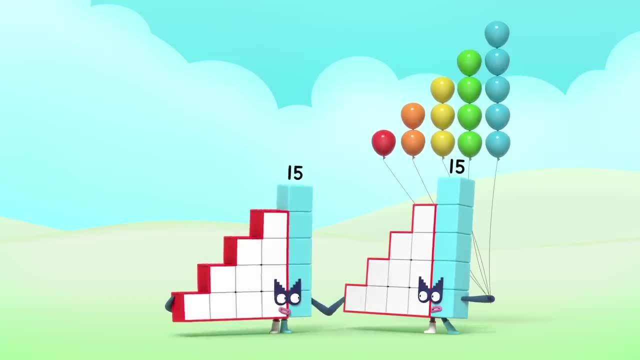 You're a Step Squad. Oh And ten, You're a Step Squad too. One, two, three and four. Six: You're a Step Squad. One, two and three And three: You're a Step Squad. 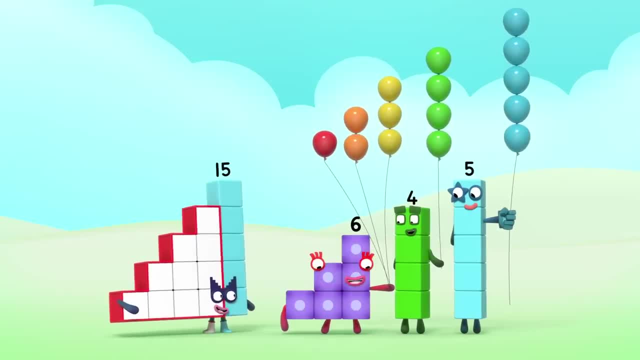 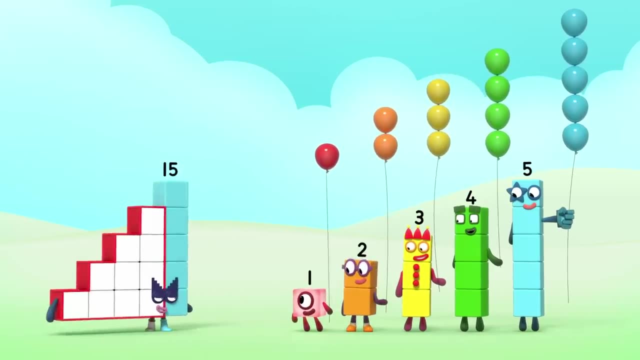 One plus two And one. You fit the pattern. So you're a Step Squad as well. One, Two, Three, Four, Five, Six And ten. You're a Step Squad. One plus two And twelve. One. 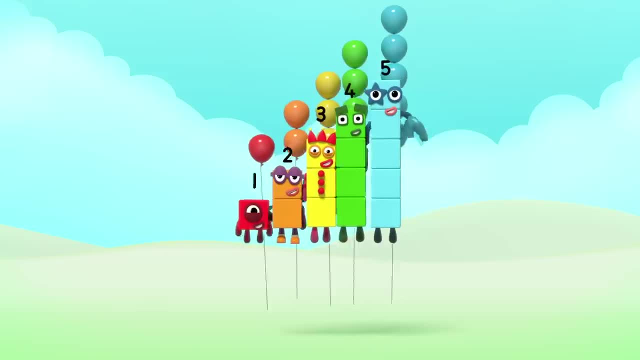 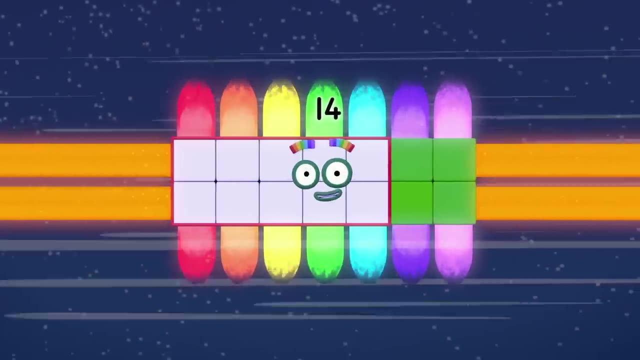 Three, Six, Ten, Fifteen Step Squads Ready for action. Two by seven. Extreme Three, Six, Nine, Twelve, Fifteen, Eighteen makes the scene. You think this is fast? Follow me for some real speed. 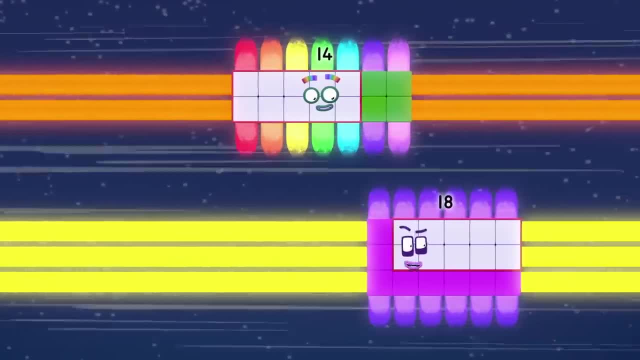 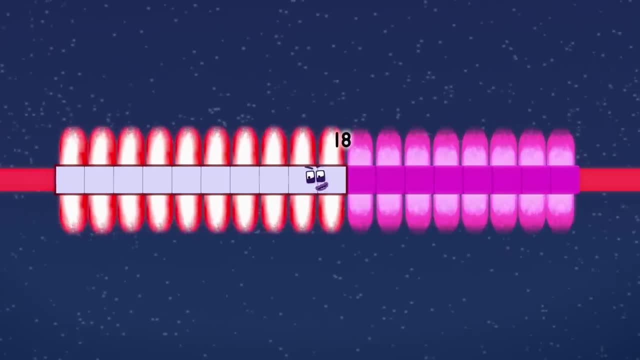 You're a Step Squad. You're a Step Squad. You're a Step Squad. I'm up for the nine. And too close. You're too fast enough to loop the loop. Go, go, go. Let's do it again. 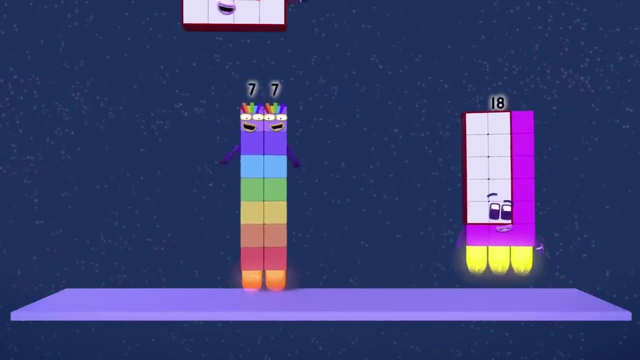 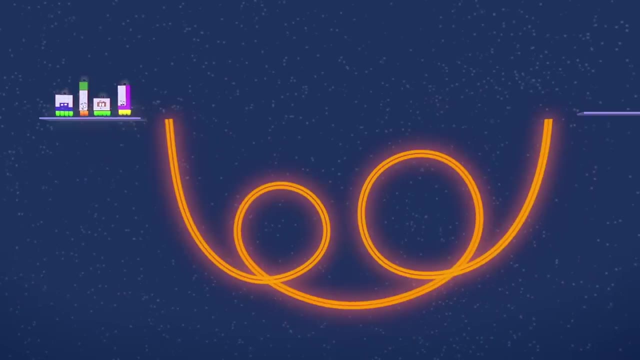 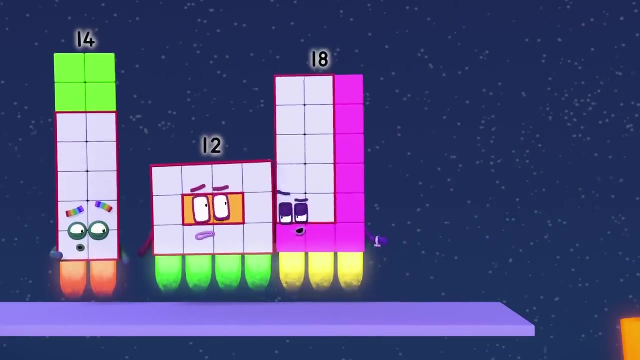 Anyone can ride that thing. Check this out: The Double Looper has a two-ray mateys So you can only ride it if you can make a rectangle that's two blocks wide, Like this, Two by nine. Two rays and away. 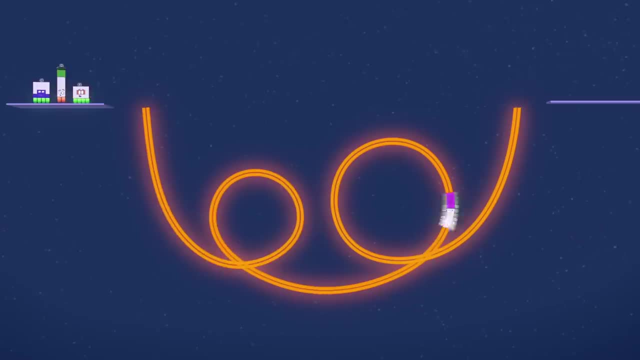 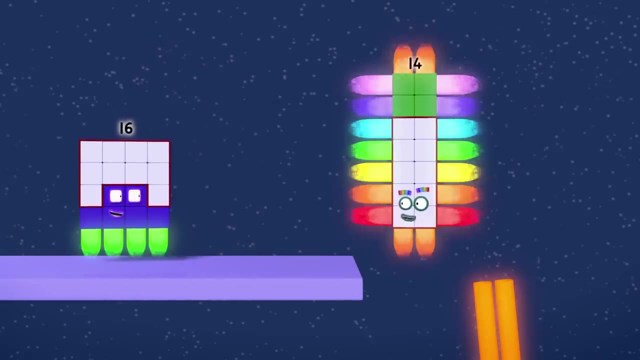 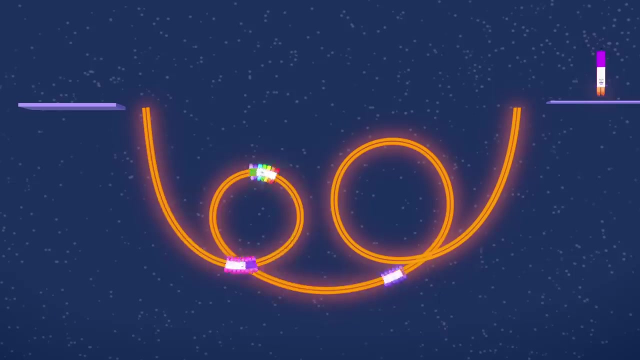 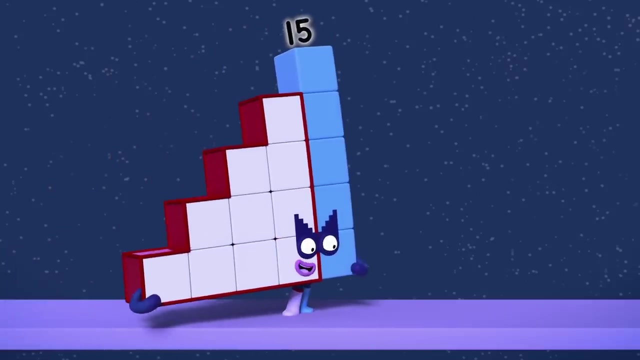 One, two, three, Five, six, Five, seven, Two, Woo-hoo Land. Two by six, One, Two by seven, Double, lucky Double seven. Two by eight. Hooray, That does look like fun. 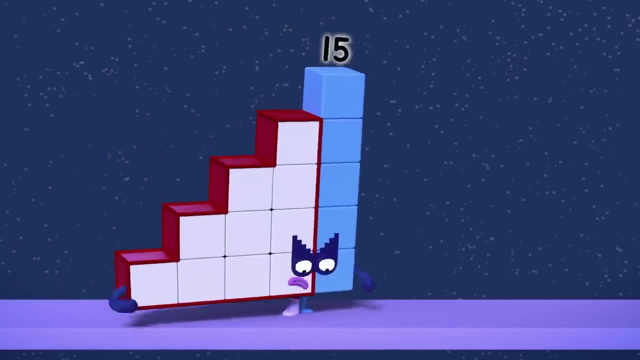 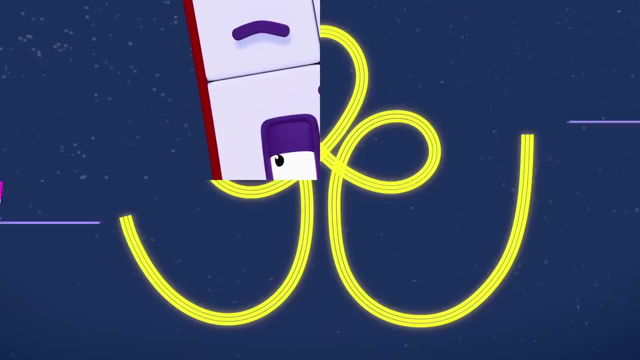 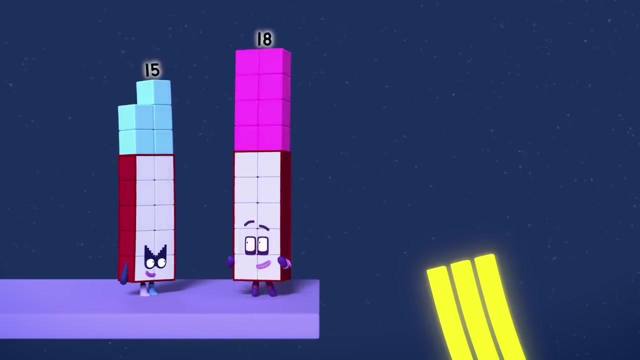 But odd numbers like me can't make a rectangle two blocks wide. See, Don't let that slow you down 15.. This next one could be made for you, A triple looper with three rays. So you need to make a rectangle that's three blocks wide. 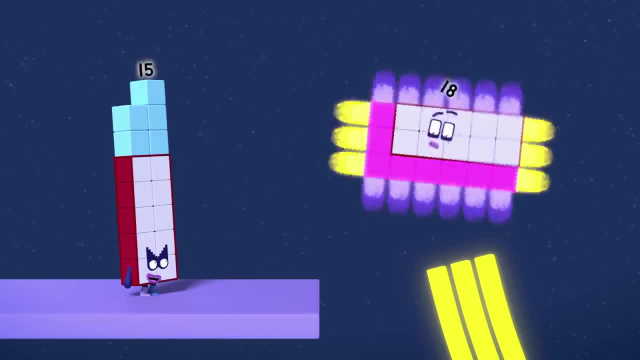 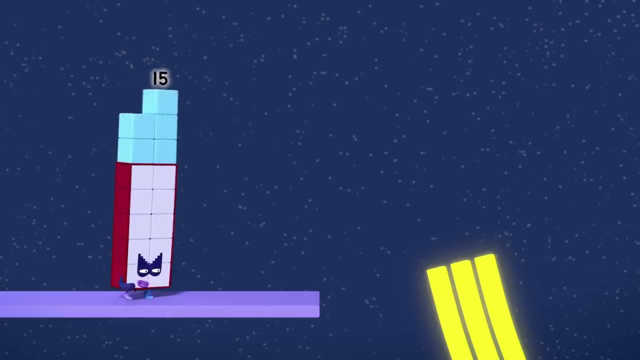 Like this: Three by six. Three rays and away. Three by six: Woo-hoo Land again, Now that I can do Three by five: Ha-ha-ha-ha-ha-ha-ha, Three by five. 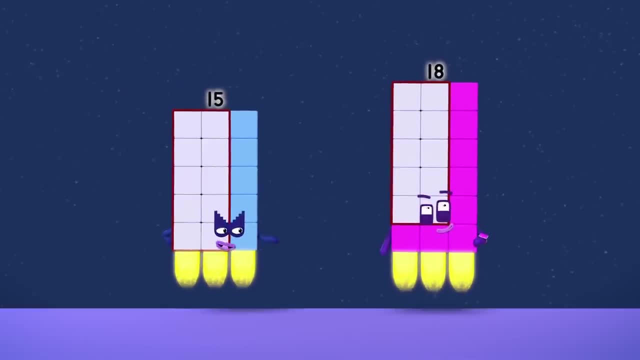 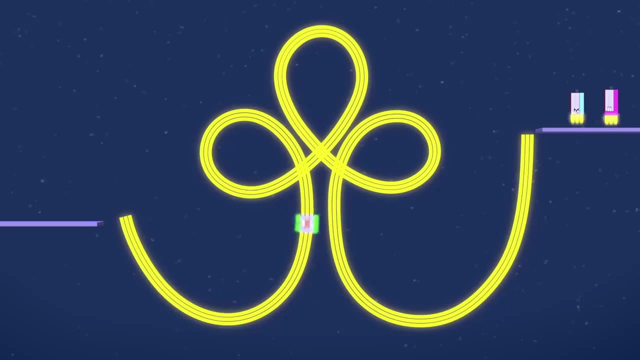 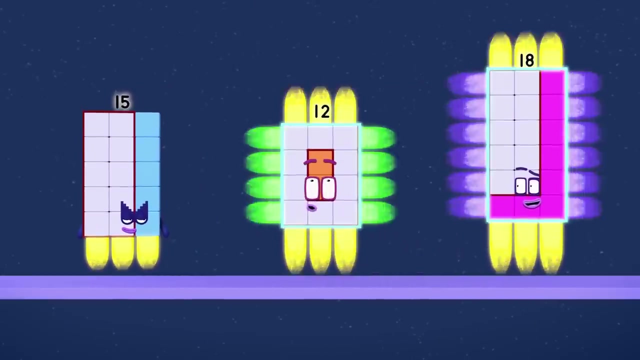 Woo-hoo, Amazing. You're built for speed 18.. You can ride loopers and double loopers and triple loopers Three by four. That's because my brother and I are both super rectangles, Which means we can make lots of different rectangles. 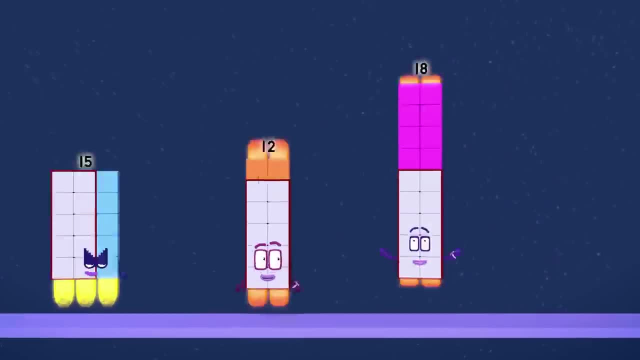 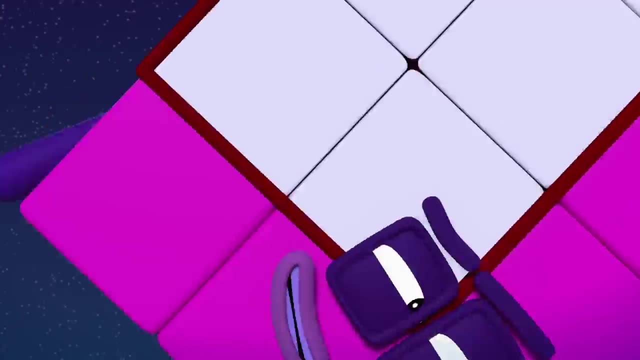 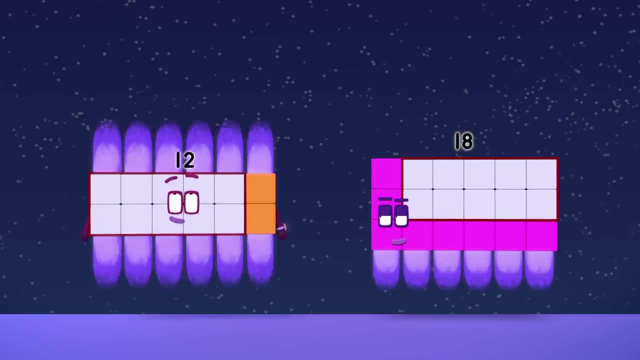 So we can make one rays And two rays And three rays, And that's not all. We can both make six rays, Six by three. Well, yes, that's true, Six by two. But why do we need six rays? 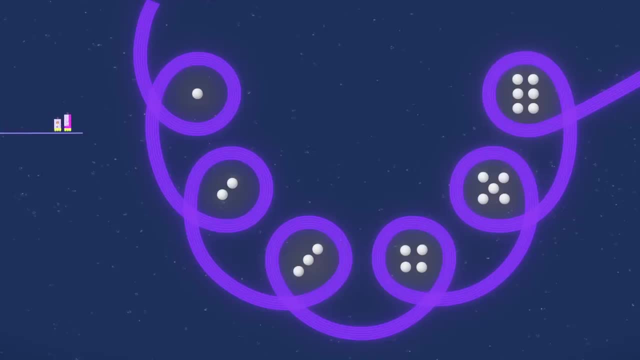 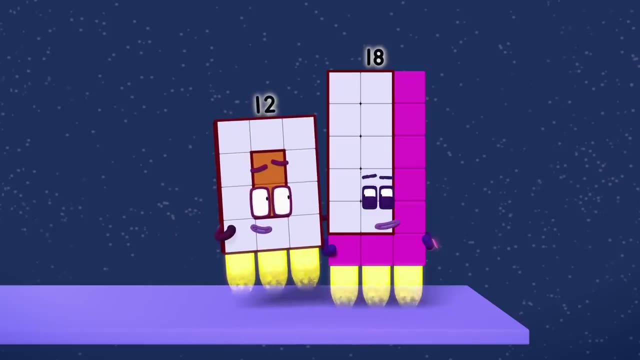 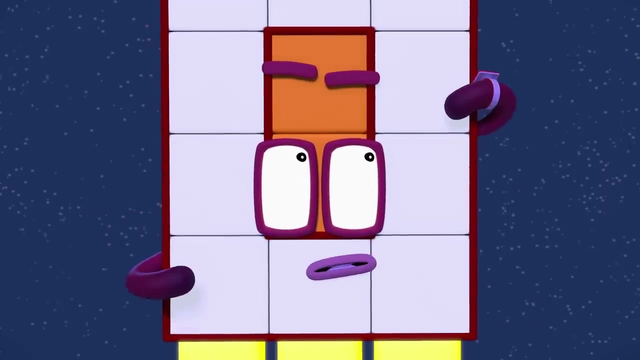 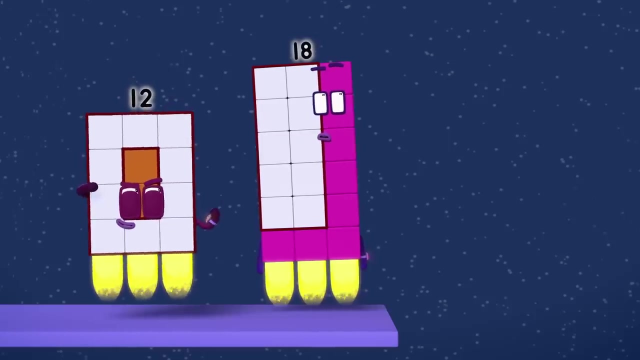 Unless There's a six looper. Oh no, How do we get up there? Relax, Let me handle this. I am 12.. I am a super rectangle Master of the rays. Oh wait, Can you do that again? 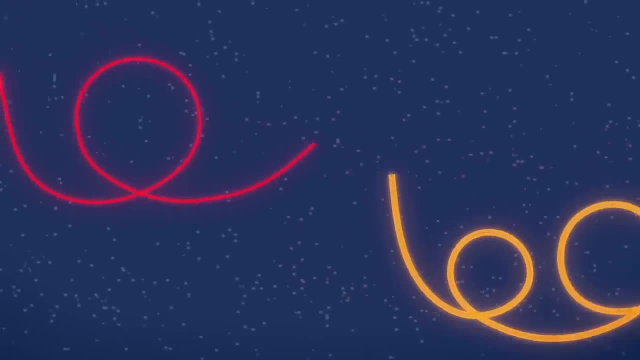 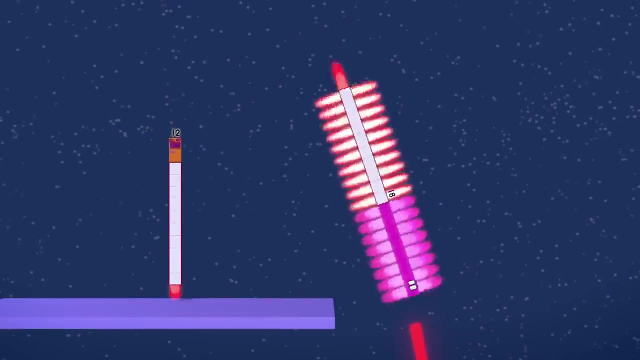 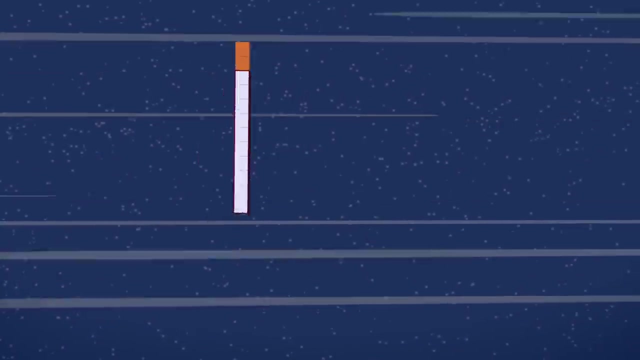 Behold The super duper looper. Go, go, go go. Switch One by 18!, 18!, 18!. One by 12!. Wow, Nice, Woo-hoo. Two by nine. Switch Two by six. 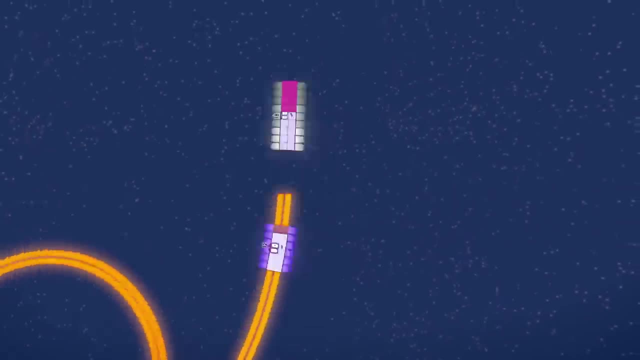 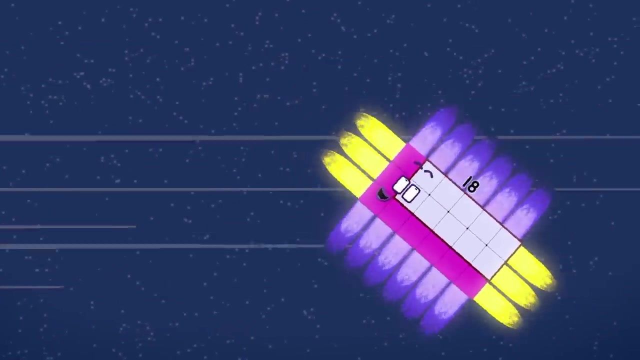 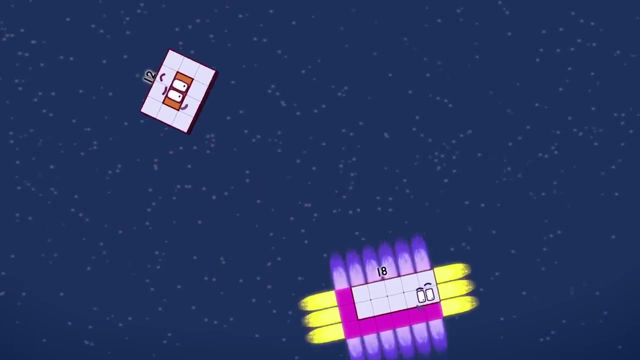 Ah, Ah, Yeah, Yeah, Switch. Three by four, Fast work, sis Race on Three by six. Woo-hoo, Yeah, Woo Woo, Nice Woo-hoo. Six by three, See ya Switch. 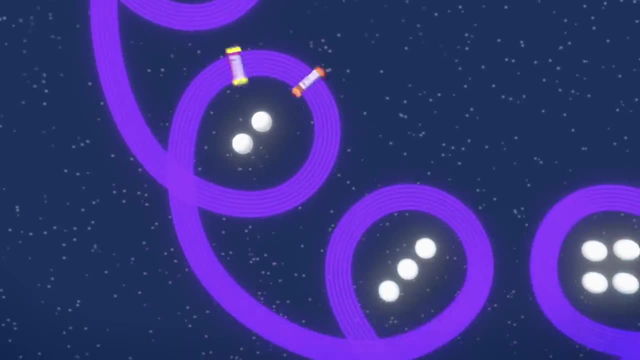 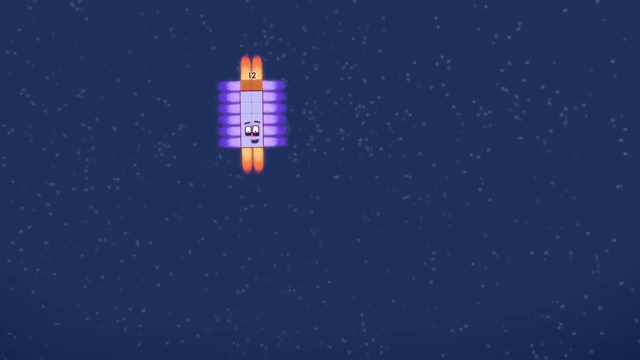 Six by two: Woo-hoo, Whoa, Woo, Woo-hoo, Woo-hoo, Woo-hoo, Whoa, Woo-hoo. Oh, Who's that? That's you. That's fast enough for me, But not me. 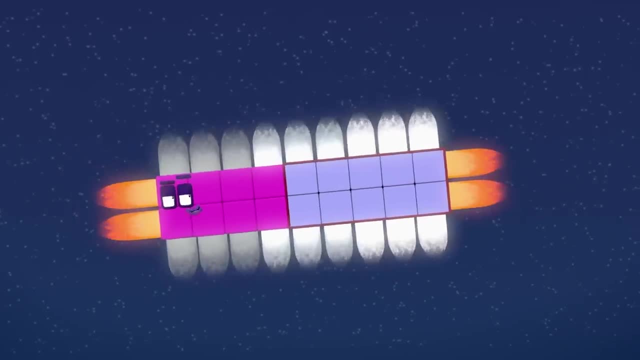 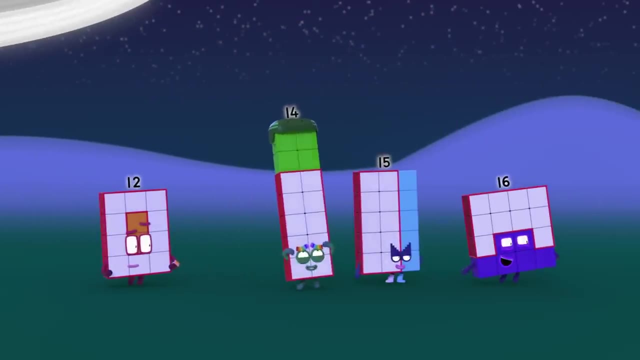 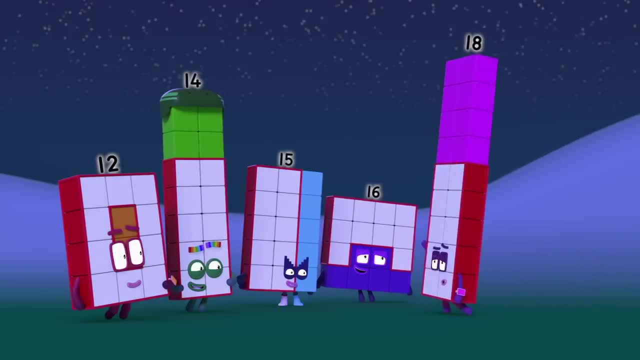 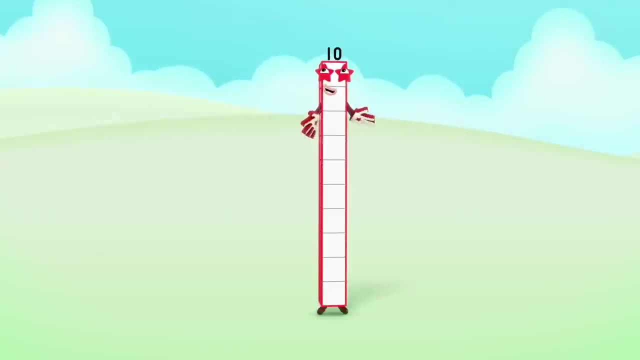 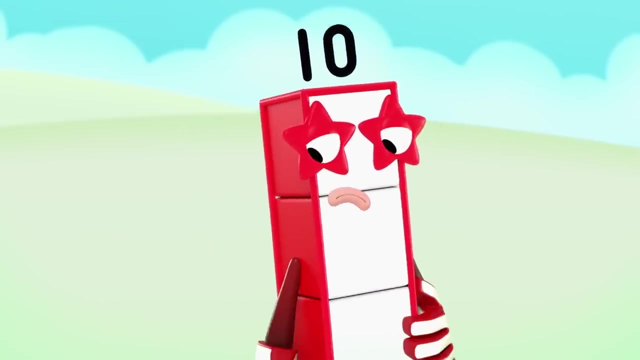 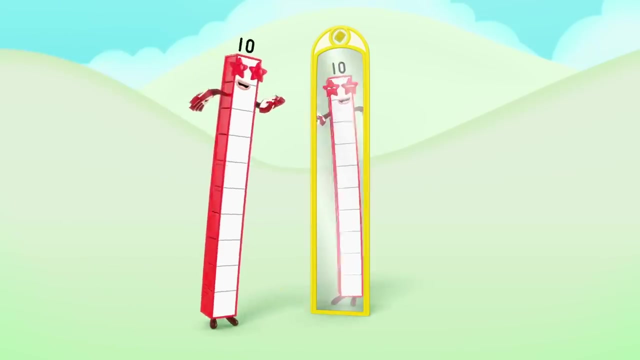 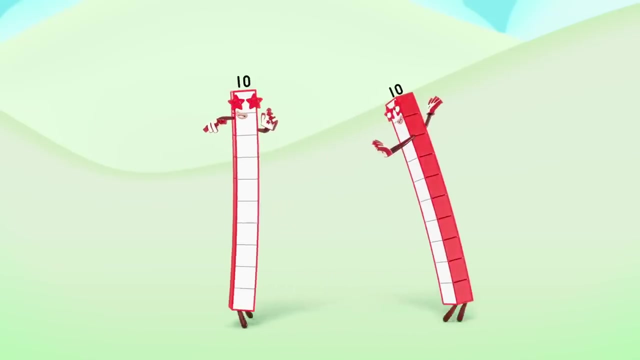 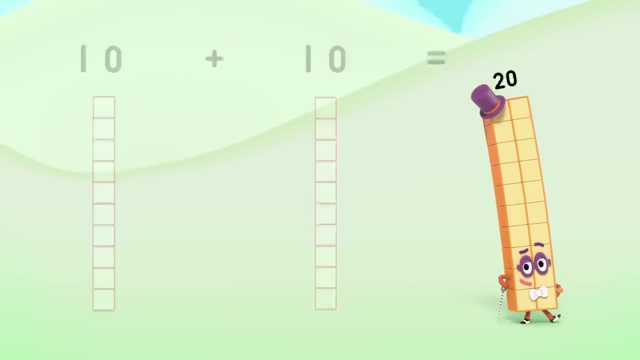 That was refreshing. and now to do something else really fast, Have a lie down. Who wants to dance with me? I Know someone who wants to dance Me. Shall, we dance cha-cha-cha. 10 plus 10 equals 20. Hello, Hello, Did somebody say. 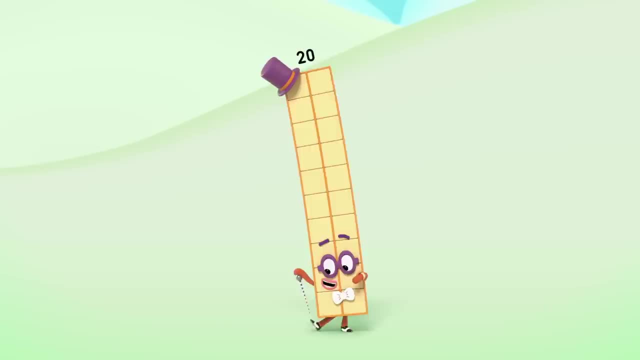 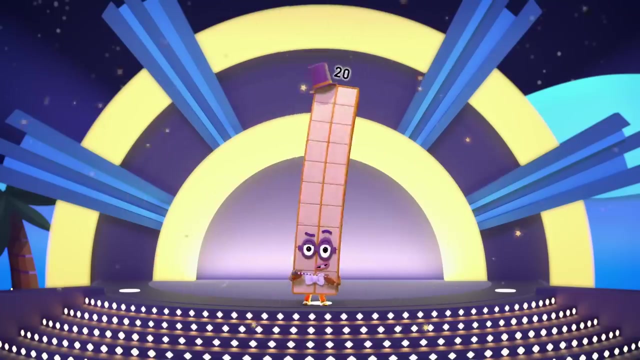 Don't. I've got the shoes tap. I've got the cane tap. I've got the tip top top, hat, tap, tap, tap. Are you ready for the big dance number? That's me, I am 20 and I love to dance With plenty of moves to my name. 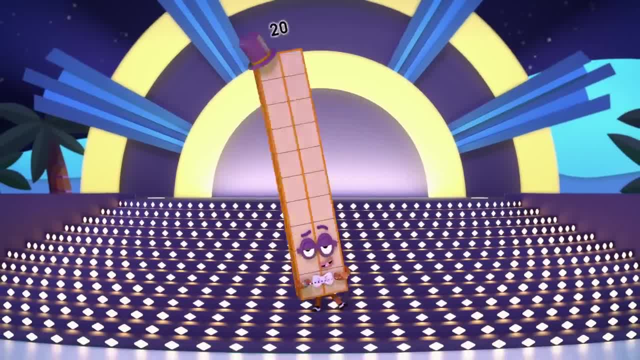 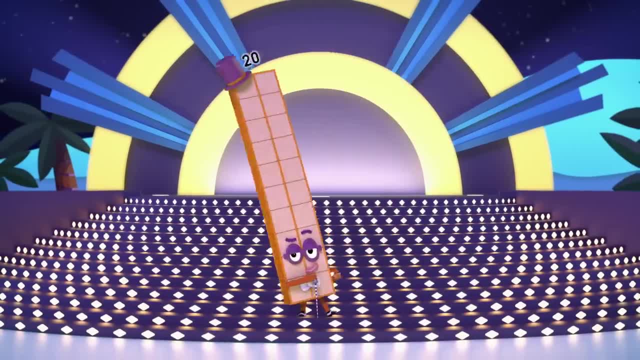 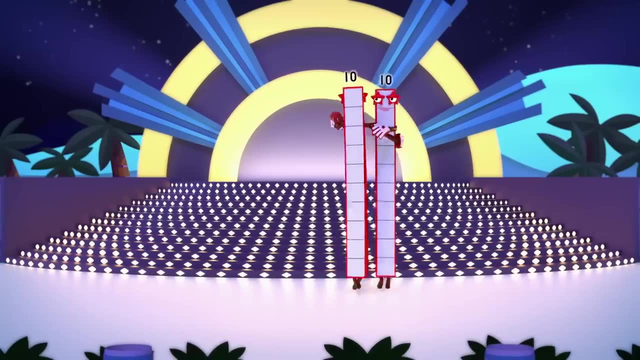 I'm tall and I'm slender. I'm graceful and tender. I swear, as I do the Fandango To tend, nothing more as I take to the floor and dance to the two tens tango: 1, 2, 3, 4, 5, 6, 7, 8, 9, 10. 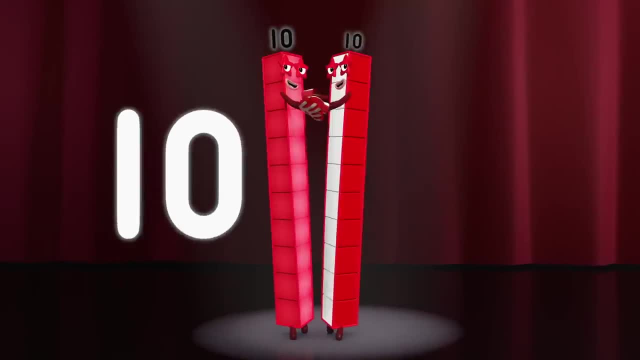 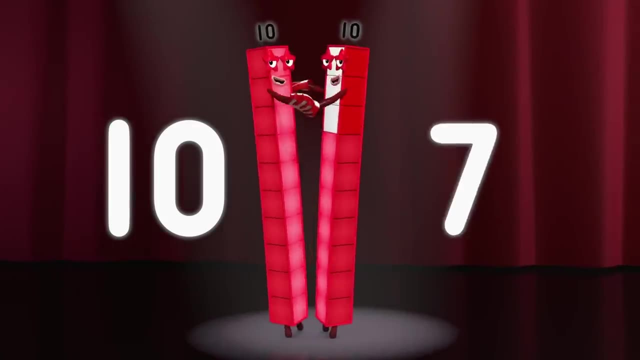 1, 2, 3, 4, 5, 6, 7, 8, 9, 10. Drop to the floor and go round again. 1, 2, 3, 4, 5, 6, 7, 8, 9, 10, 2 friends, 2 tens make 20. 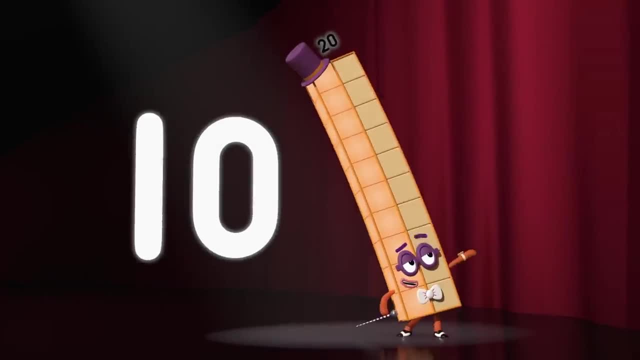 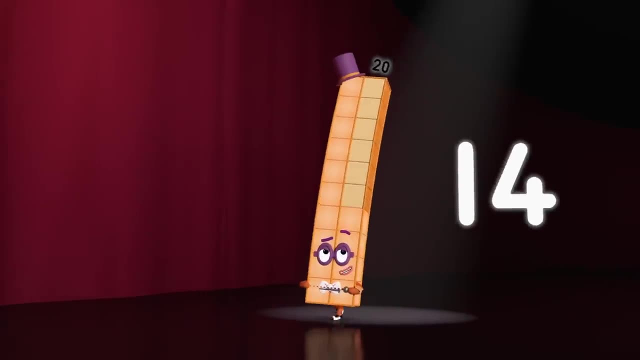 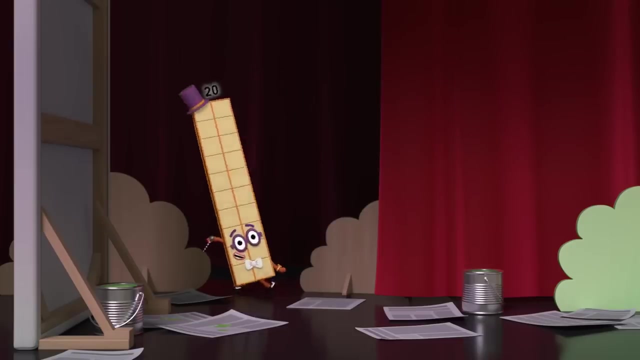 1, 2, 3, 4, 5, 6, 7, 8, 9, 10, halfway to 20, Go round again: 11, 12, 13, 14, 15, then 16, 17, 18, 19, 20. My two says I'm made of two tens and 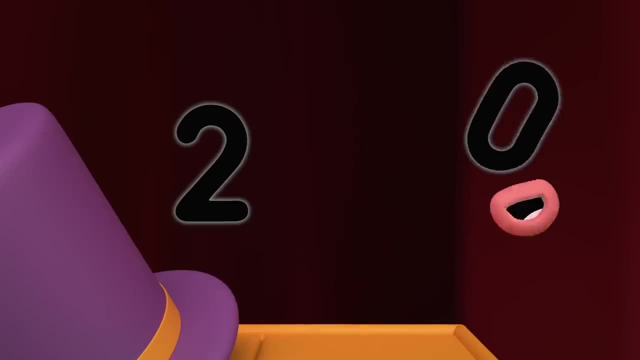 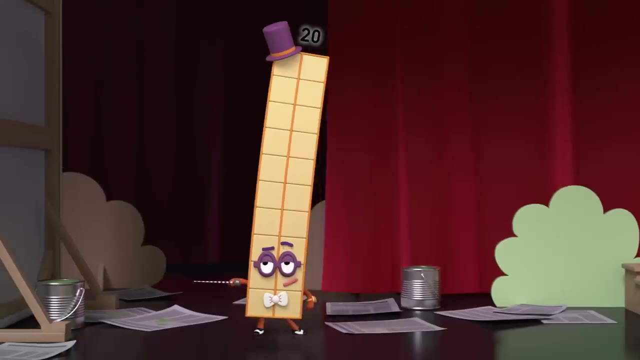 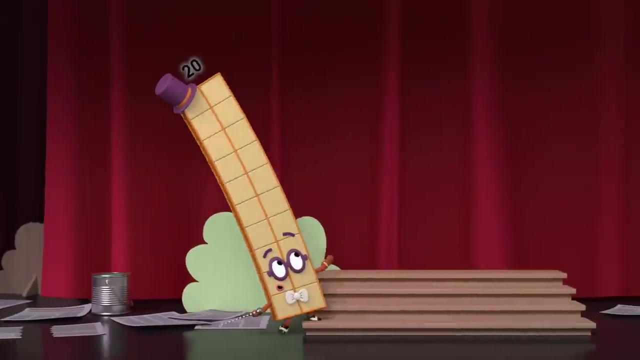 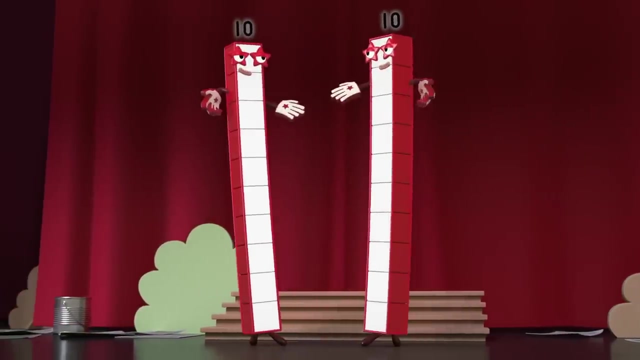 Who says I need any more. That's how I'm created. I'm perfectly weighted to move to the beat of a mambo And then writes on cue: I can split into two and dance to the two tens. tango 1, 2, 3, 4, 5, 6, 7, 8, 9, 10. 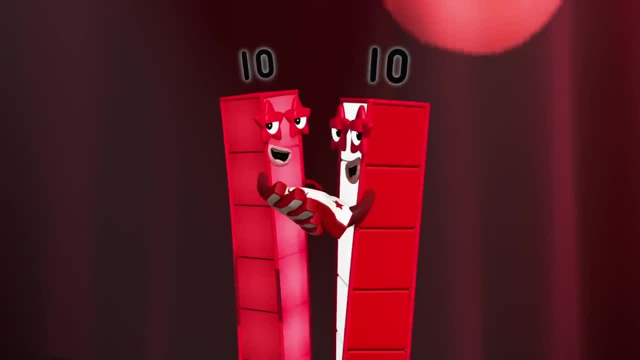 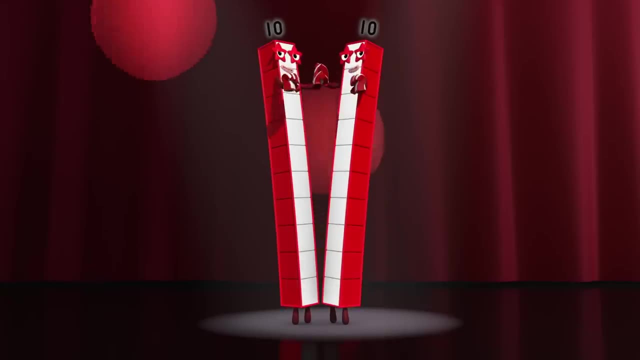 Drop to the floor and go round again. 1, 2, 3, 4, 5, 6, 7, 8, 9, 10. 2 friends 2 tens make 20. 2 friends, 2 tens make 20. 1, 2, 3, 4, 5, 6, 7, 8, 9, 10. 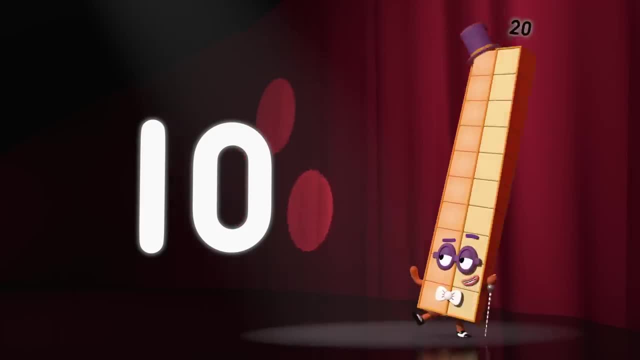 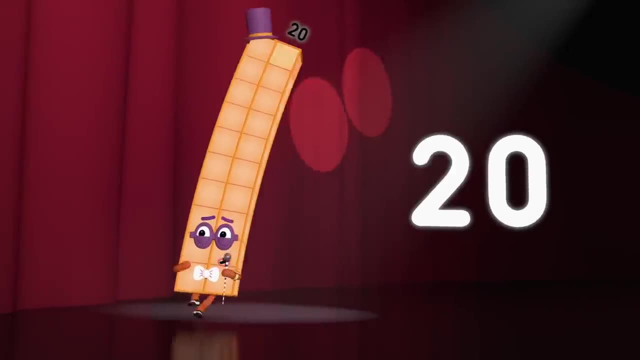 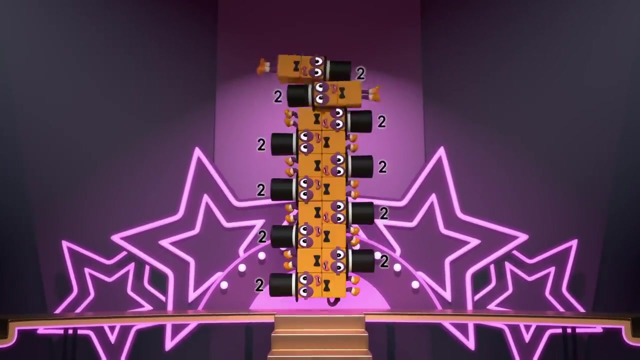 Halfway to 20, Go round again: 11, 12, 13, 14, 15, then 16, 17, 18, 19, 20. I have some more friends I'd like to meet. It's a ten seas, hot sea shuffle, Ten of us teasing a row. 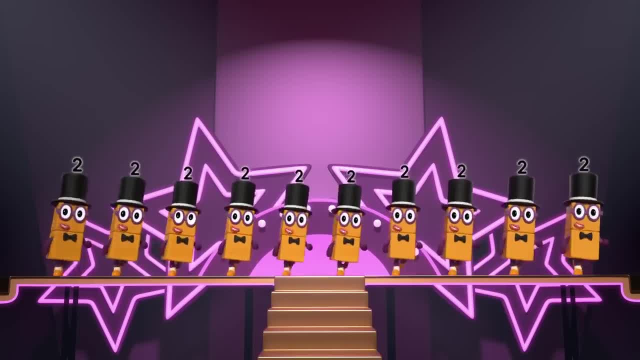 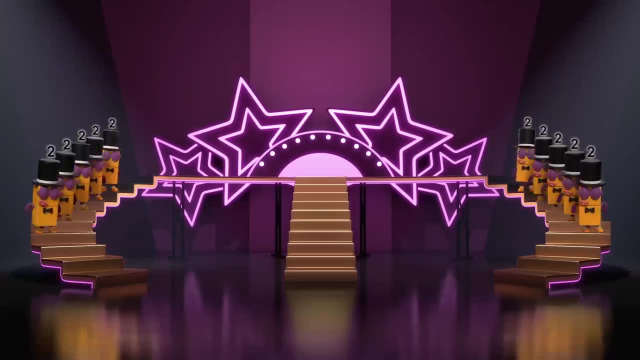 It's the Tentoo's Hot Shoe Shuffle. welcome to the Tentoo's Hot Shoe Show. We can shuffle to the beat, so we shuffle our feet. people say your shuffling sure looks sweet. It's the Tentoo's Hot Shoe Shuffle. ten of us, two's in a row. 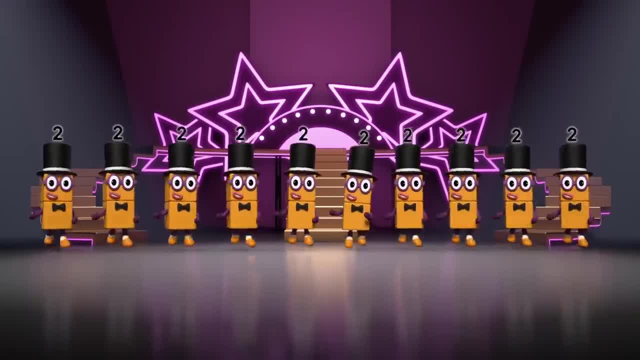 It's the Tentoo's Hot Shoe Shuffle five wide. for now it's time to go. 1, 2, 4,, 6,, 8,, 10,, 12,, 14,, 16,, 18,, 20!. 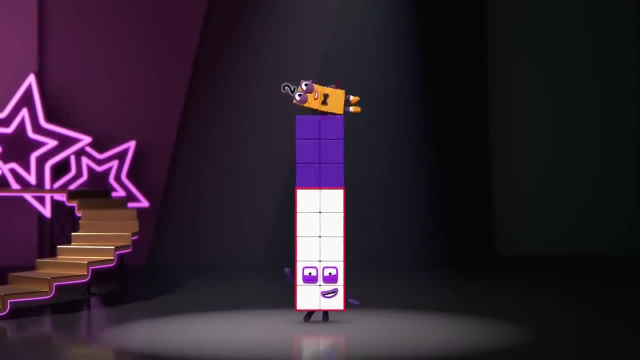 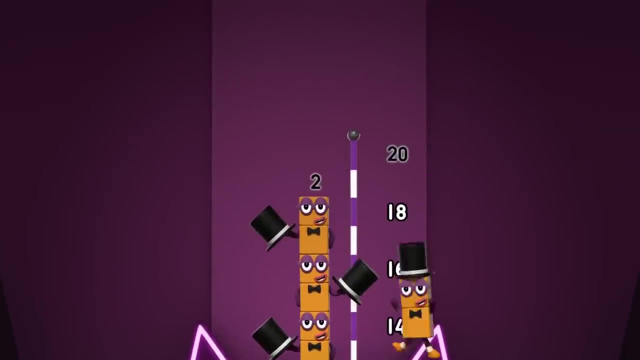 1,, 2,, 4,, 6,, 8,, 10,, 12,, 14,, 16,, 18,, 20!. 1,, 2,, 4,, 6,, 8,, 10,, 12,, 14,, 16,, 18,, 20!. 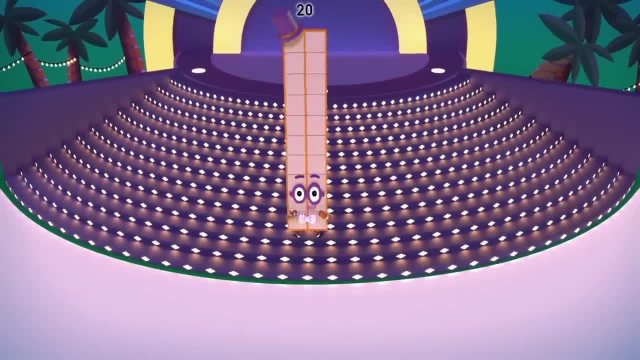 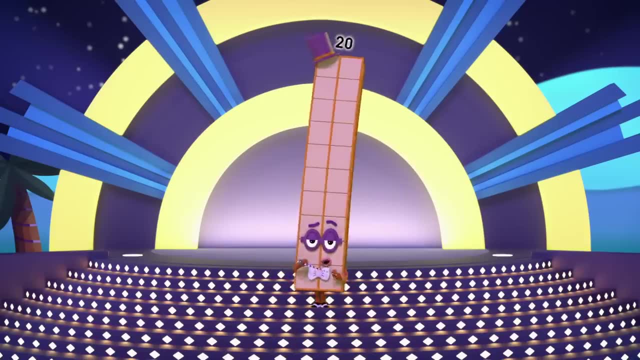 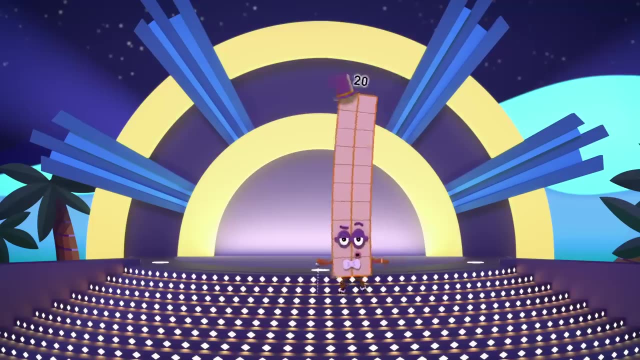 I'm 20 and I love to dance, with plenty of moves to my name. I'm tall and I'm slender. I'm graceful and tender. I sway as I do the Fandango To Tent, nothing more, as I take to the floor and dance to the Juten's Tango. 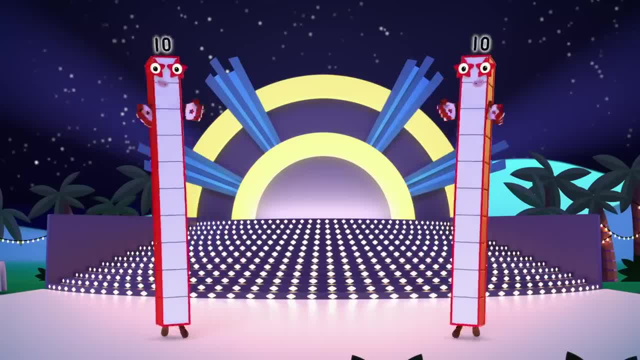 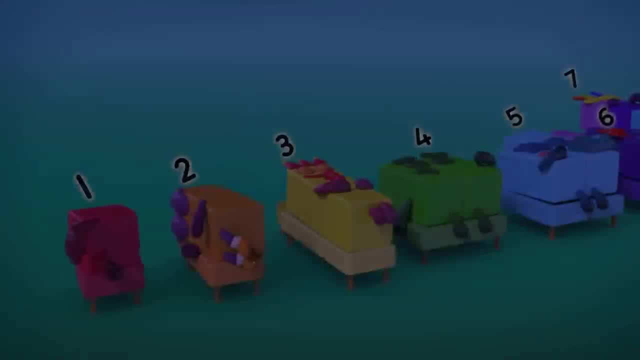 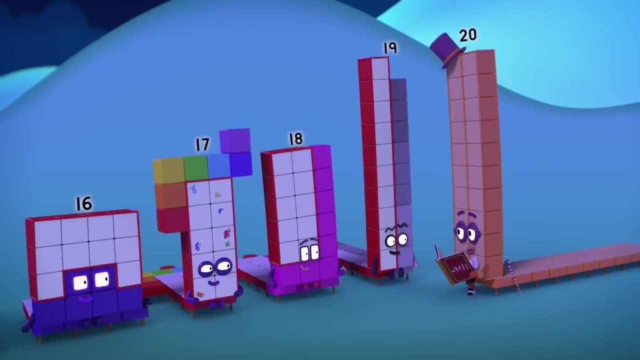 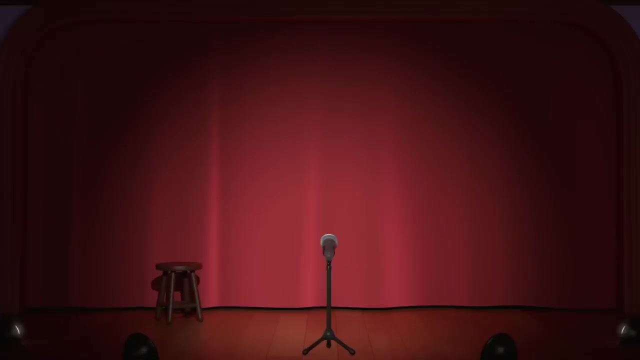 To Tent nothing more, as we take to the floor and dance to the Juten's Tango. If you're sitting comfortably, then I'll begin Chapter 16, A Six Walks Into A Ten. Ow. Now it's time to introduce you to an act who will amuse you. 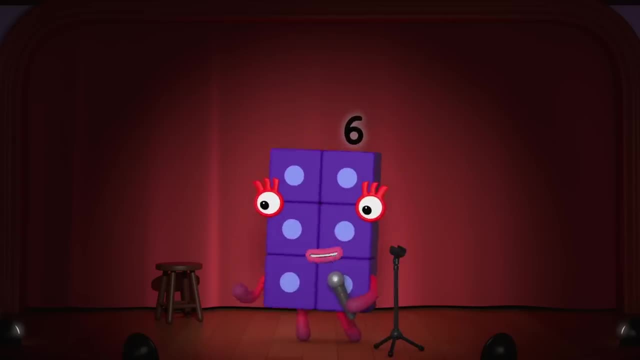 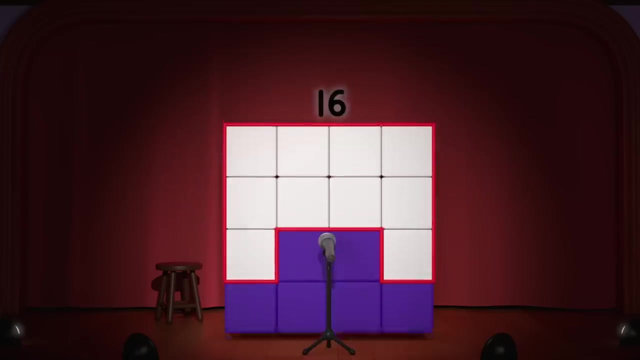 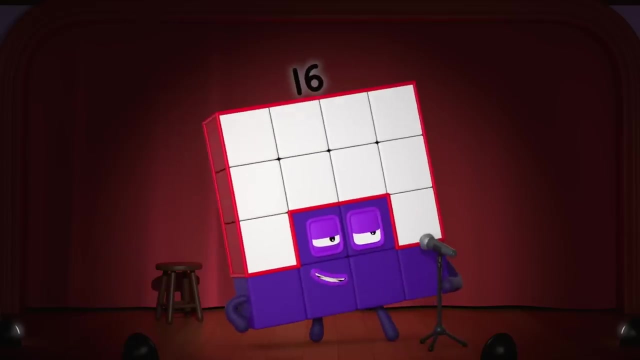 She knows how to make a scene. give it up now for Sixteen. Um, hi Tent, there's Sixteen. Right here, I'm Sixteen. let's get this party started. It's nice to be here and here and here and here. 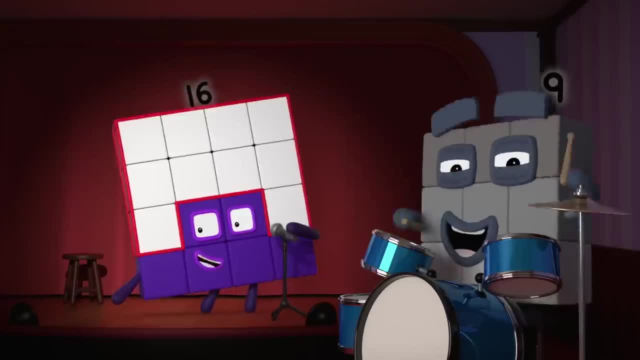 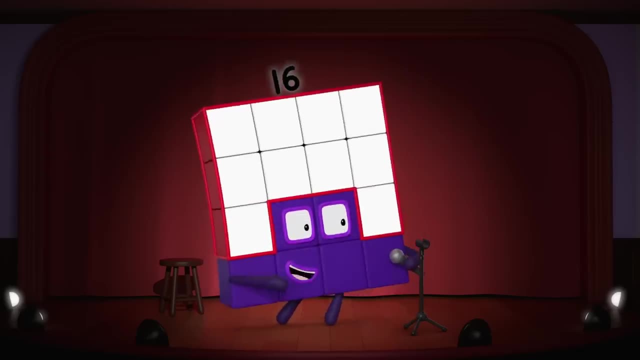 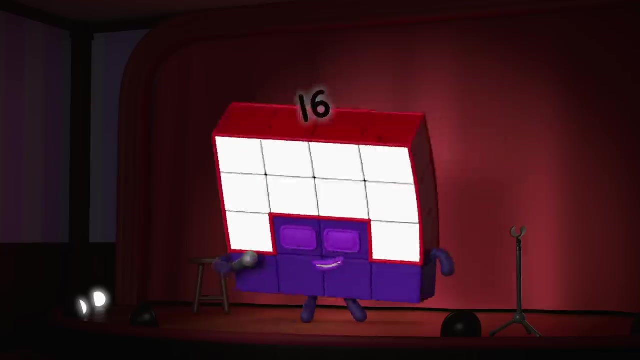 Look at that: I'm a square turning round. Hey, you know what Nine's favourite story is? Goldilocks and the Three Squares Squares. And if you're after a square deal, here I am. I'm a square. 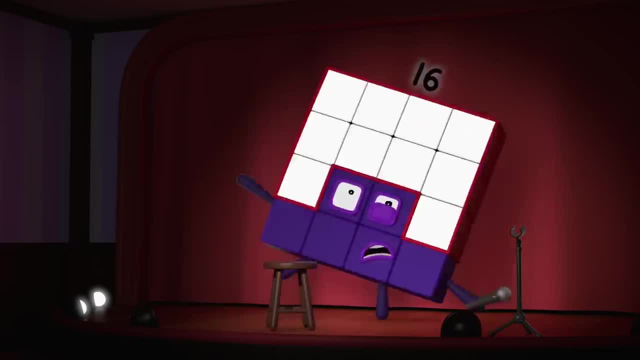 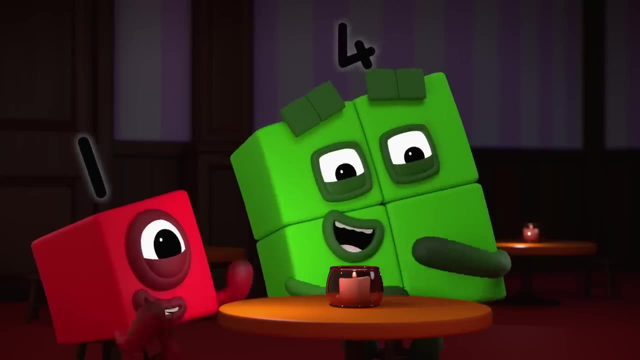 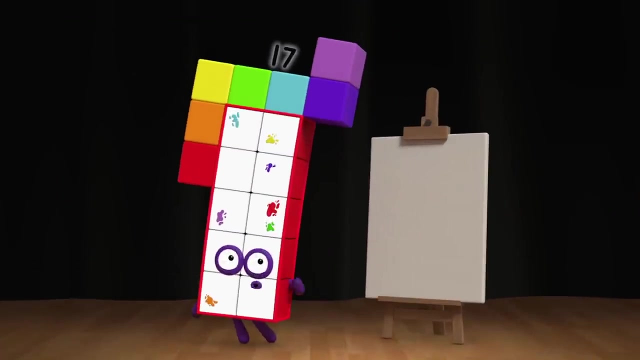 Made of squares, With a a square in the middle. Chapter 17,. Portrait of the Artist in His Prime. How do Seventeen here Today, I'm going to show you how to paint a self-portrait. Here goes. 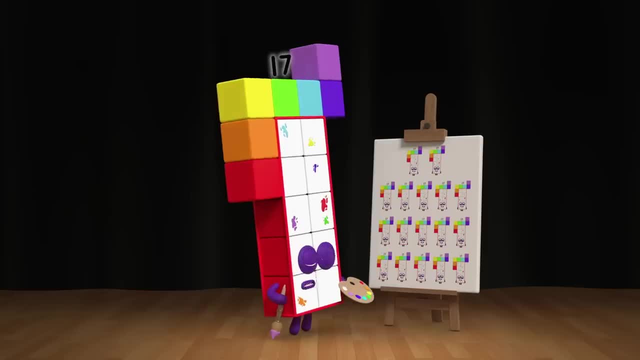 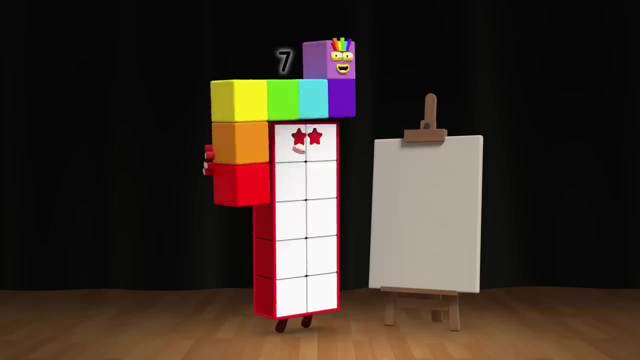 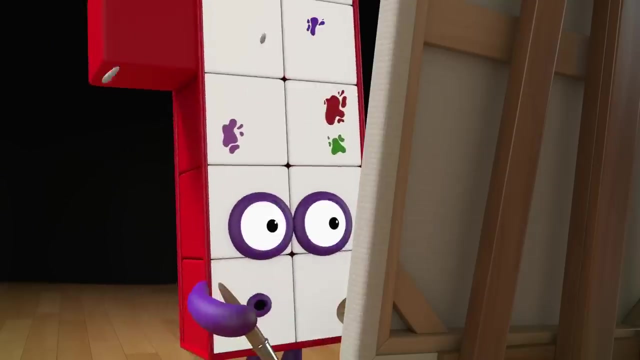 Oh, deary me. that's seventeen self-portraits. Let's try again. I'm ten and seven. So if I paint ten and then seven, Oh, seventeen of each, Oh, I'm never going to get this right. 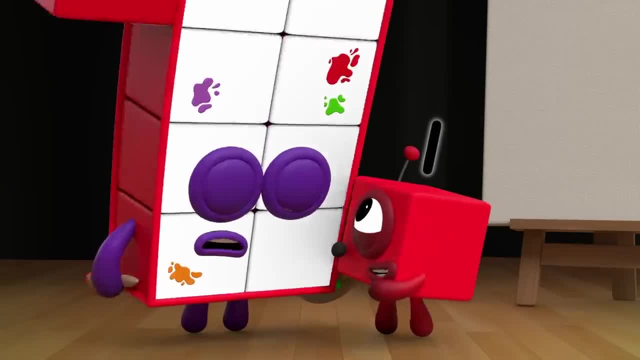 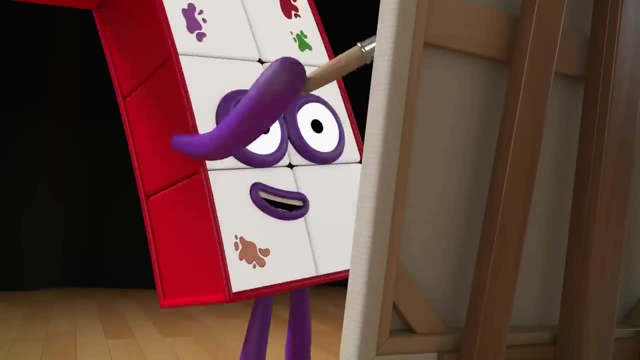 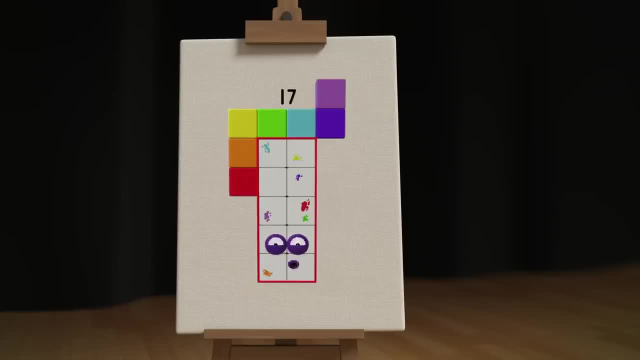 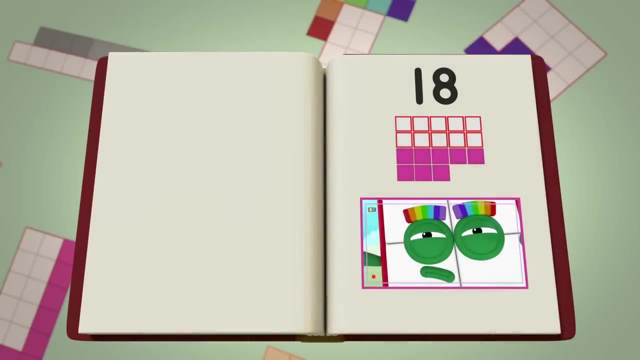 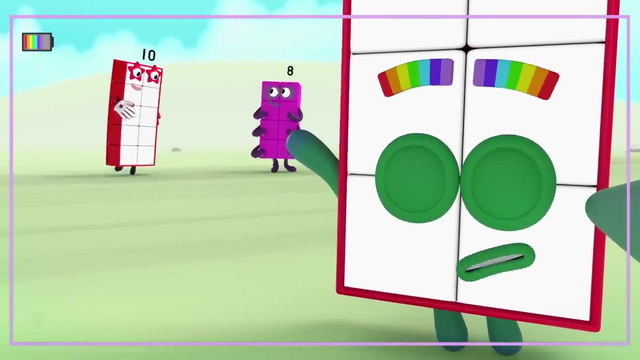 Seventeen ones, Which makes one seventeen Pretty as a picture. Chapter 18, Full Speed Ahead. Extreme Fourteen here Reporting live on a cool attempt to be the fastest number ever. Rocket ten ready to fire Two, four, six, eight. 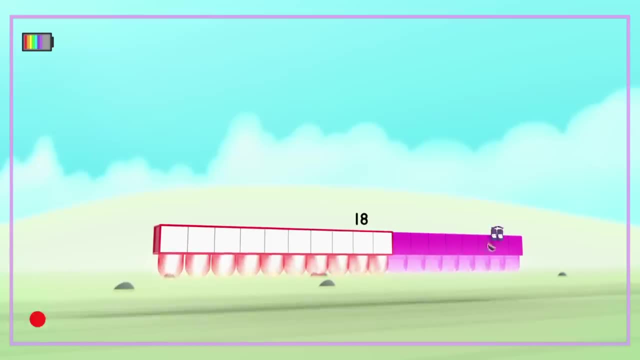 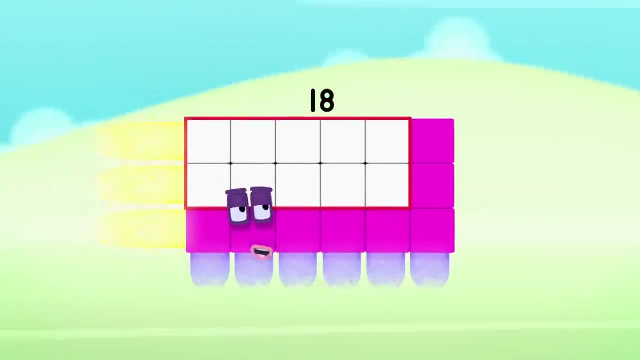 Super speedy, don't be late Speed. Somebody say speed Eighteen, Speed Machine, One ray and away. Wanna see me go faster? Two rays and away. Three rays and away. Six rays and away, Nine rays and away. 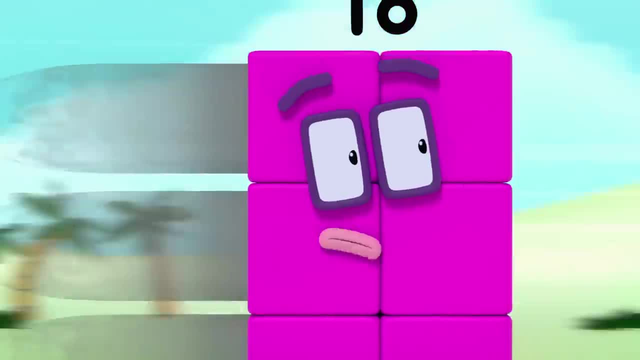 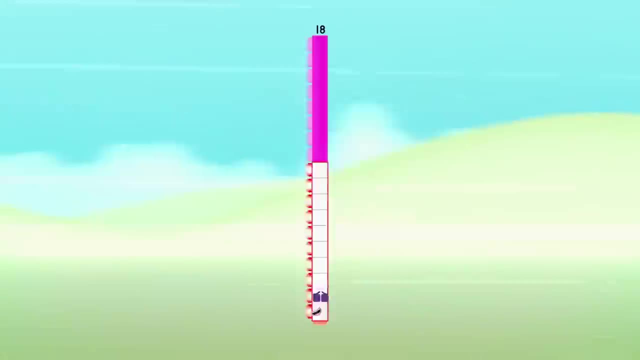 Super Sonic. Eighteen, Eighteen, Good call, compadre. Eighteen rays and away Go dude, Look out Tunnel. Uh-oh, Now that was a speedy escape. Phew, Chapter 19, Full Speed Ahead. 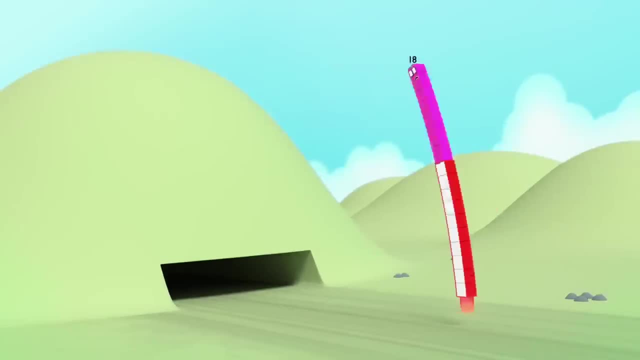 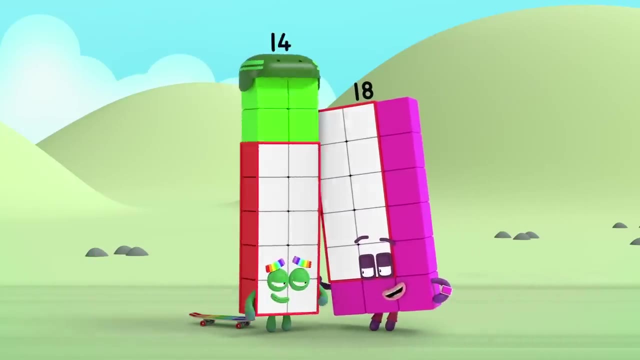 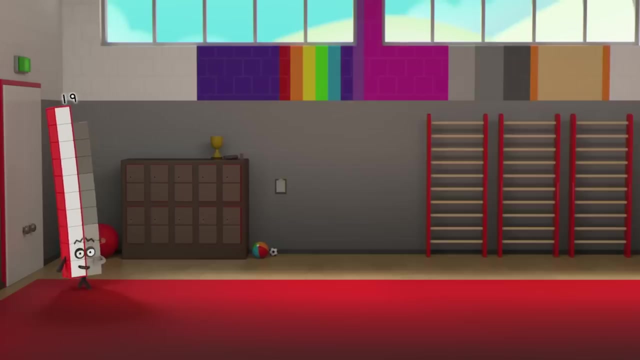 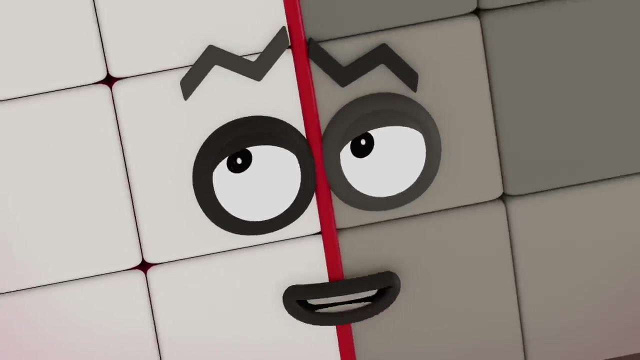 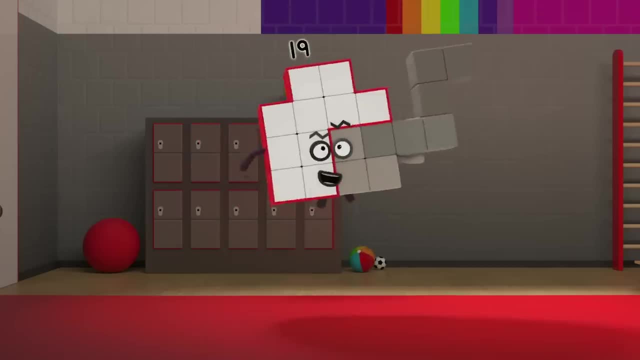 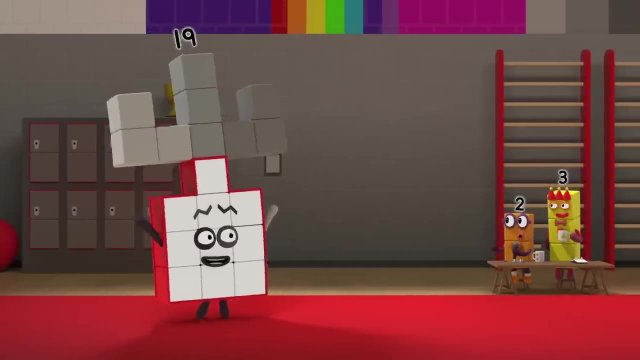 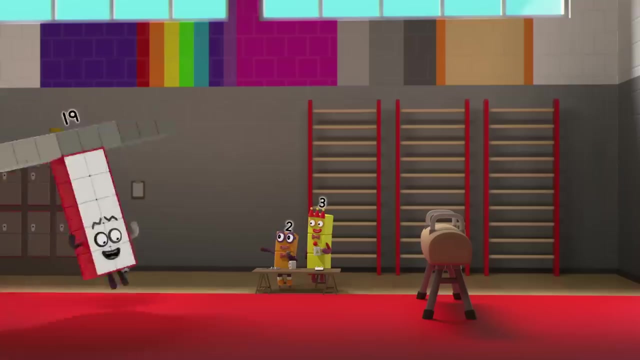 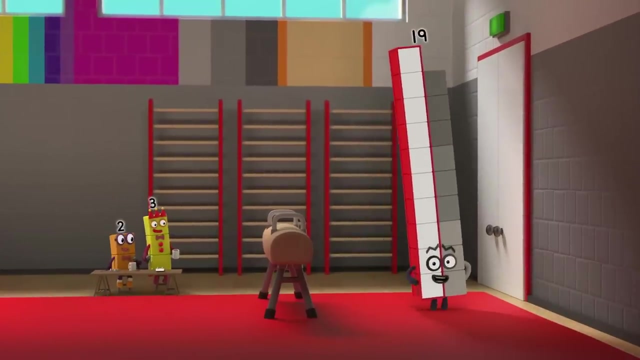 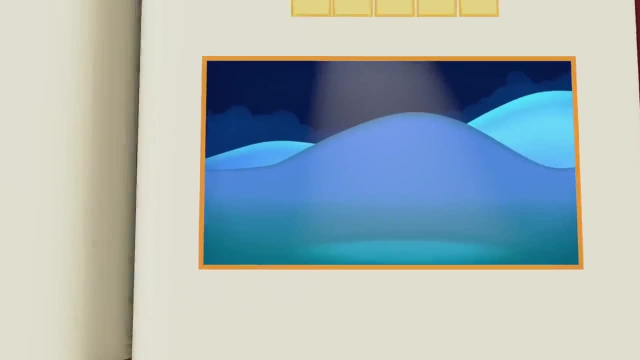 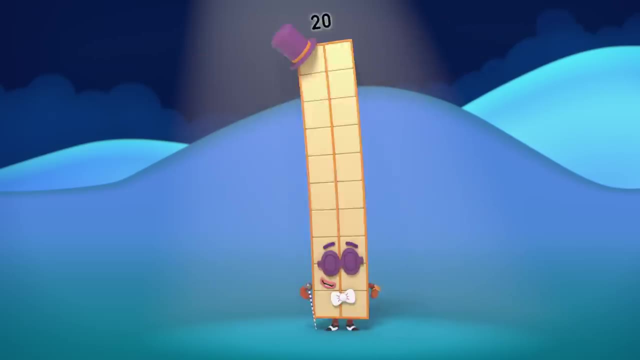 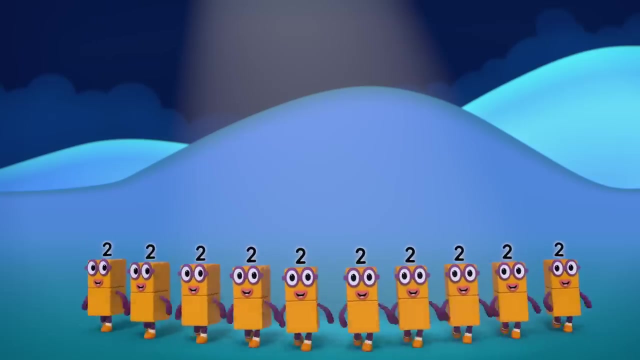 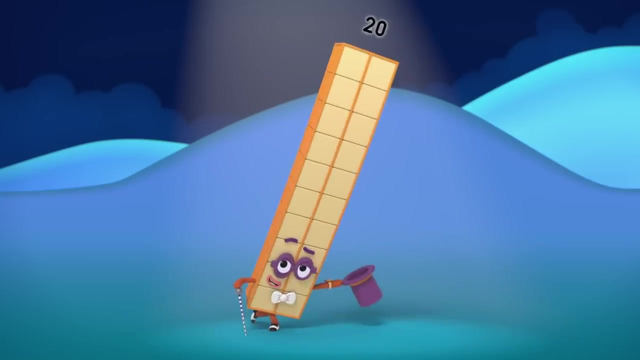 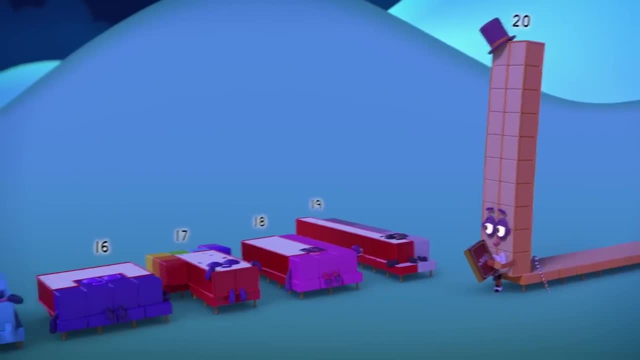 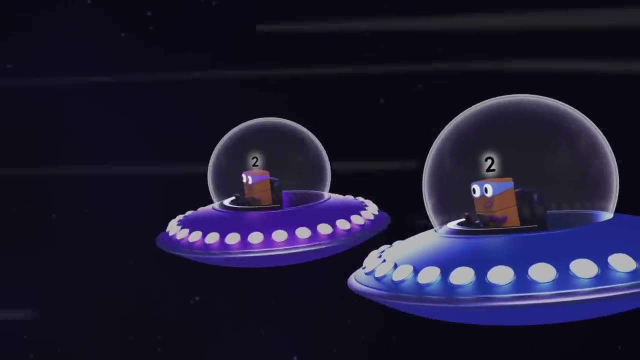 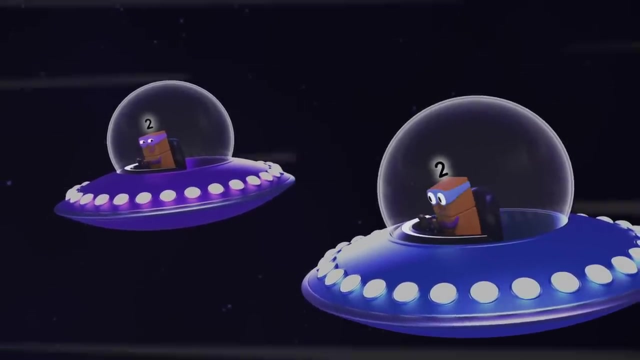 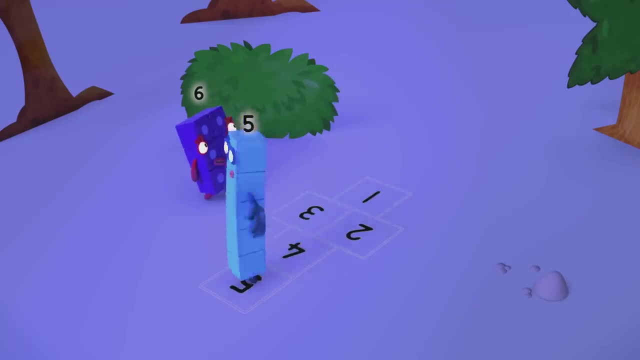 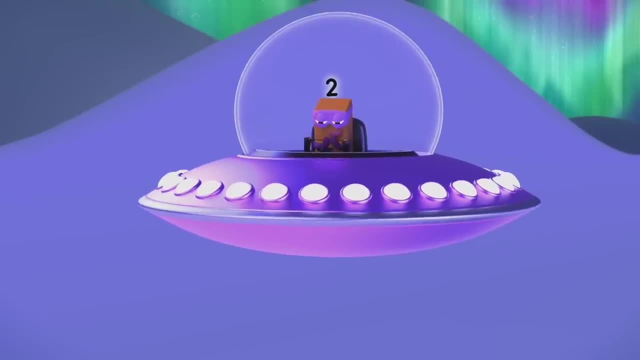 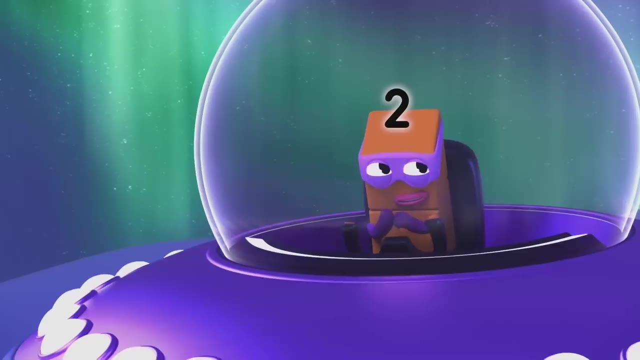 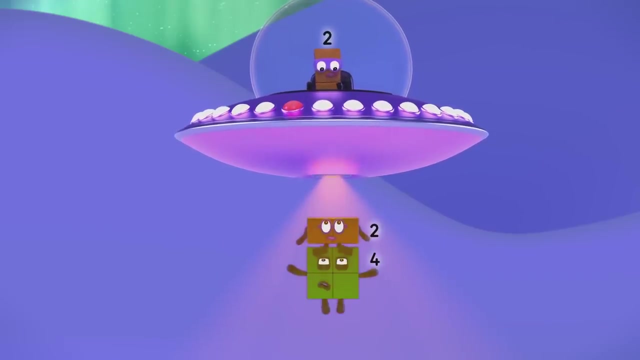 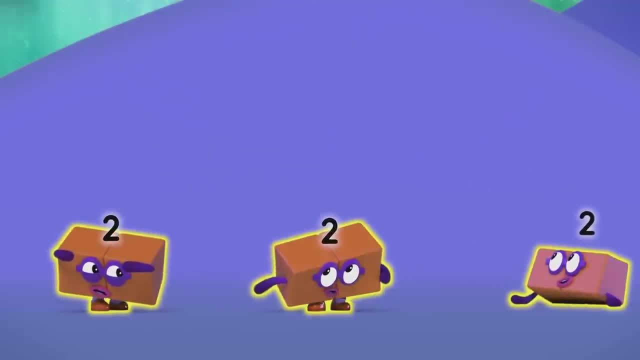 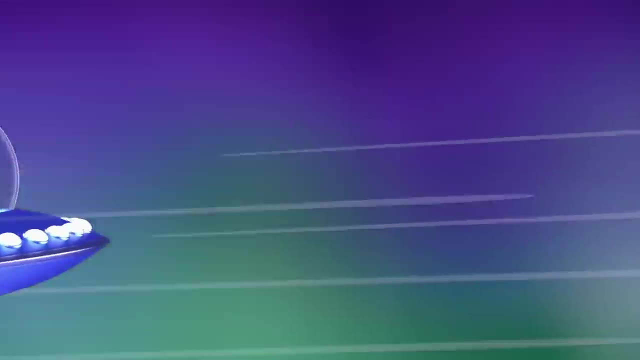 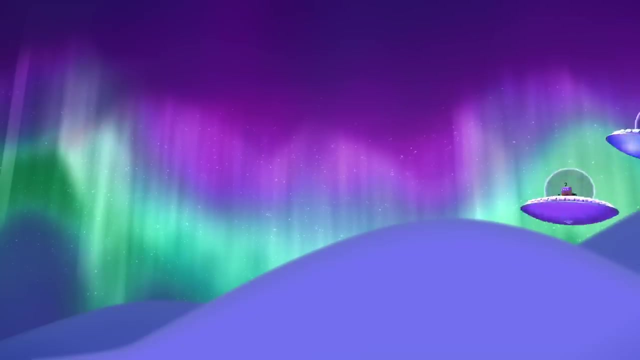 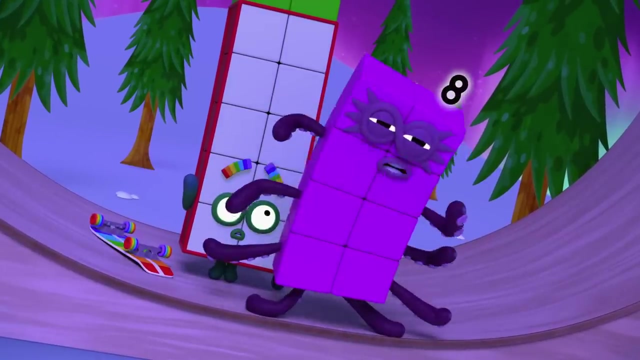 Speed Speed. Oh, happy, Terrible Tuesday. everyone, Of course, should that be every two Whoo-hoo, Whoa. Target acquired Never fail Fourteen. I've dealt with the Terrible Twos before. Off to block shield. 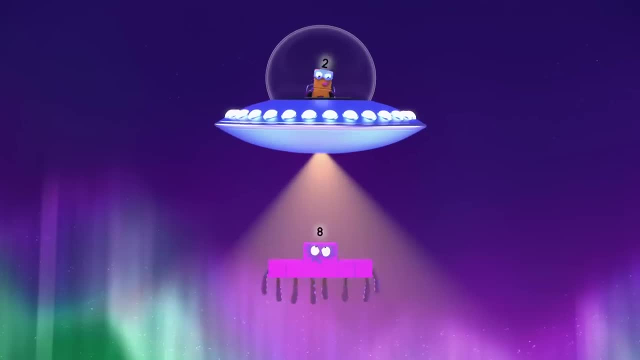 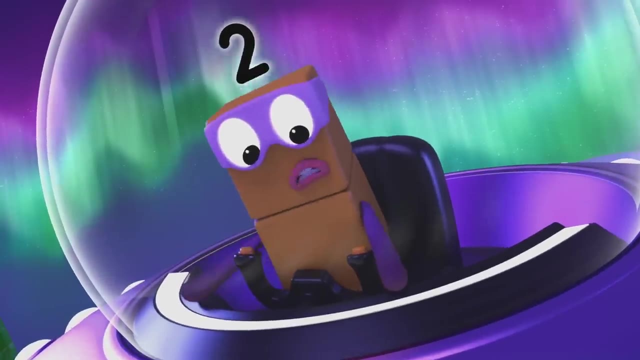 One, two, three, four, five, six, seven, eight. Yikes, One, two, three, four. hey, There are four twos in eight. You're in the lead, Amigo, but not for long. 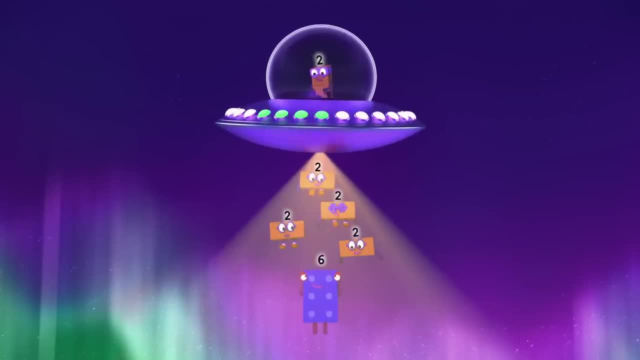 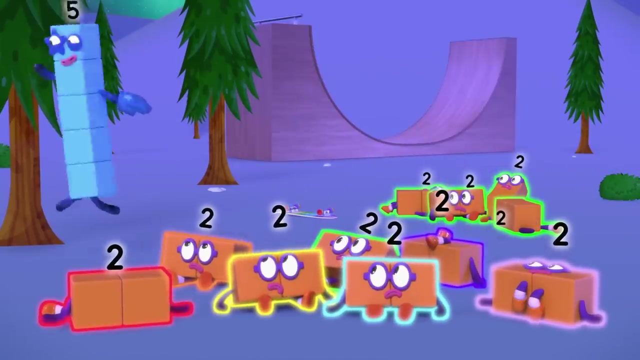 Whoa One, two, three, four, five, six, seven. Oh pretty, There are seven twos in 14.. Beat that, Whoa. Excuse me, I need to land a hand. Whoa Hold still. 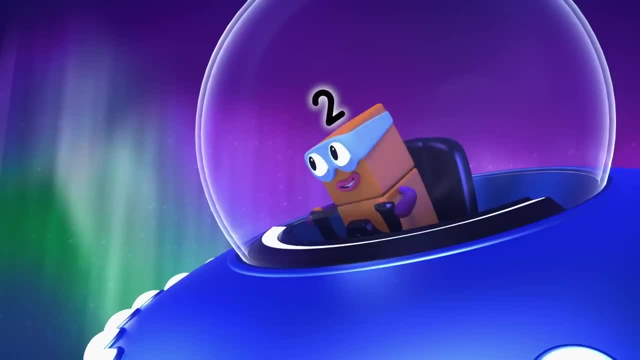 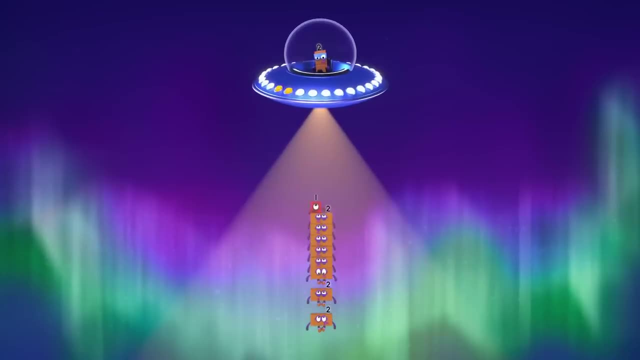 Seventeen is greater than 14, so this should put me back in the lead. Hey, Whoa, Hey. Remainder alert, Remainder alert. There are eight twos in 17 and one left over. Remainder one, No. 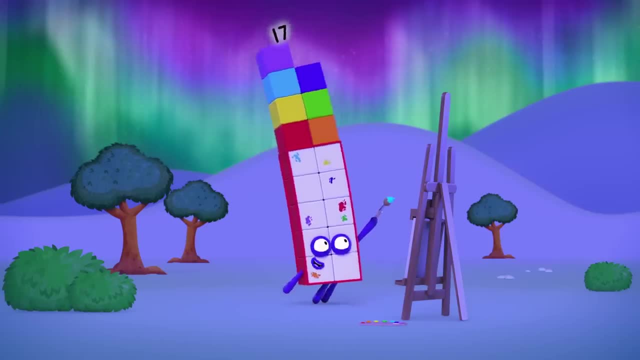 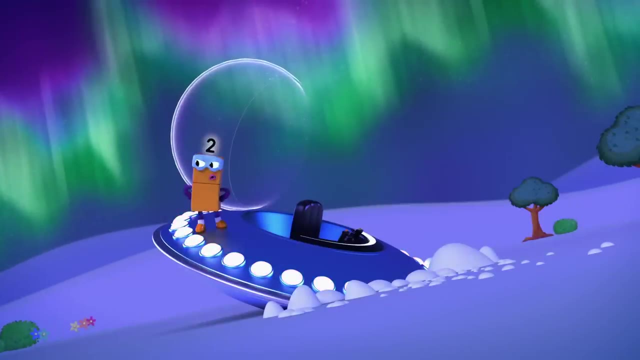 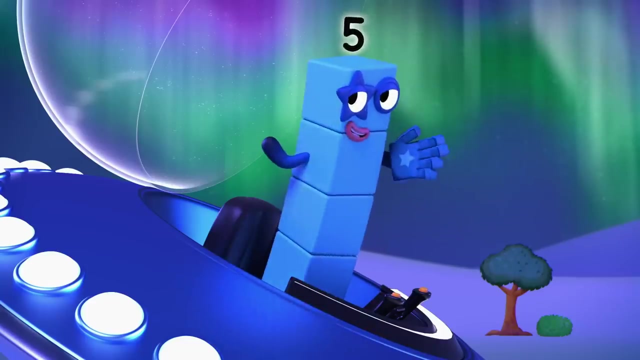 Ten experience: I must paint it. Whoa, Whoa, Whoa, Whoa, Whoa. Oh Uh, where's that reset switch? Ah-ha, Oh, You've got to hand it to me, Whee. 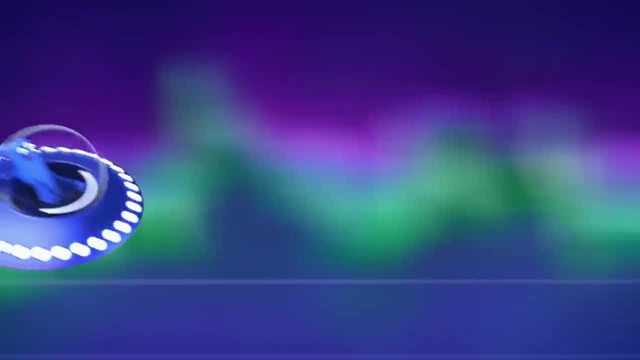 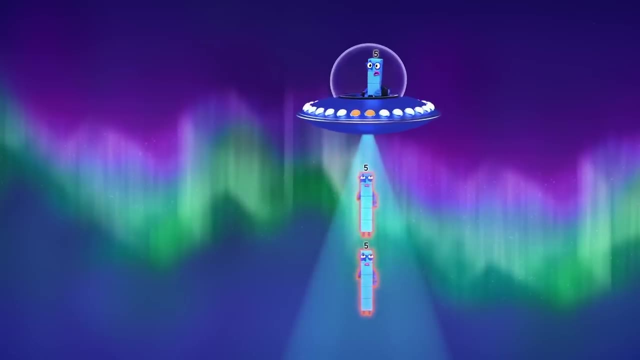 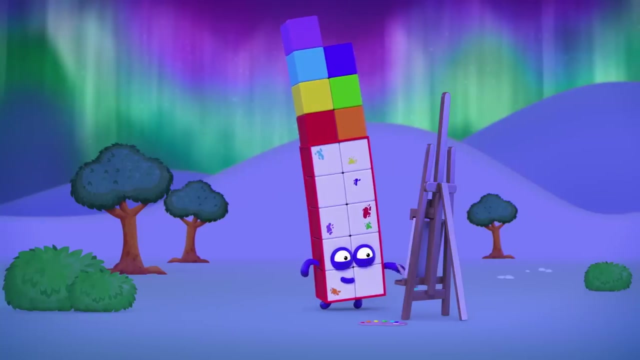 Hey Factor beam reset. Divide into fives. Ha, You can't catch me, Whee, Oh, Oops, I've divided ten into two fives. Huh, Huh, Huh, Huh, Huh, Huh. 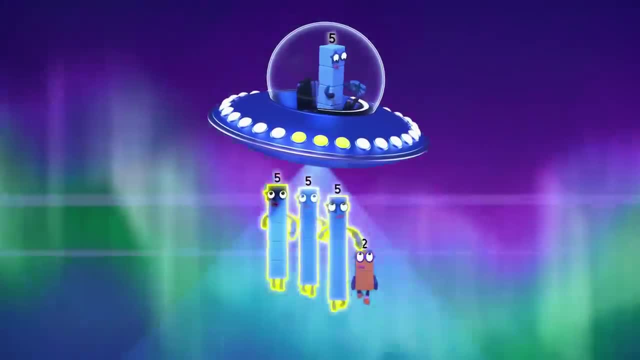 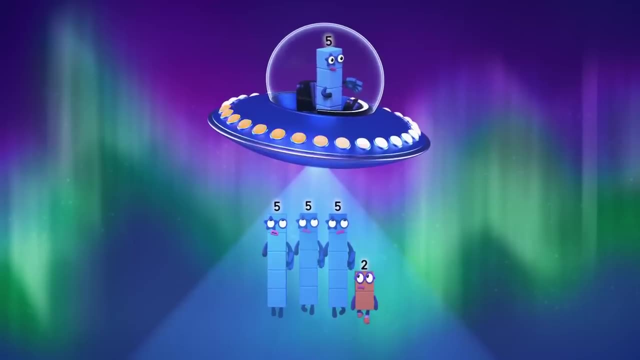 Huh, Sorry, Learn a driver. Remainder alert. Remainder alert. There are three fives in 17 and two left over. Remainder two. Whee, I think I've got the hang of it now. The twos factor beam divides you into twos. 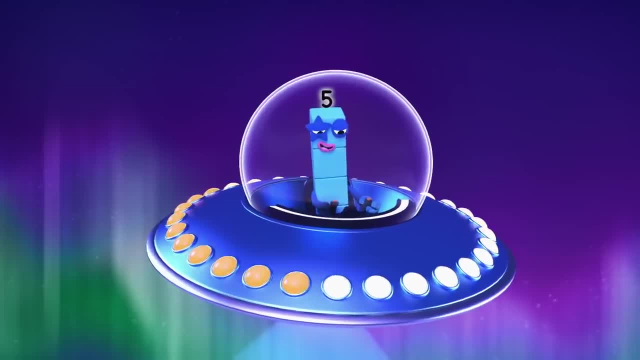 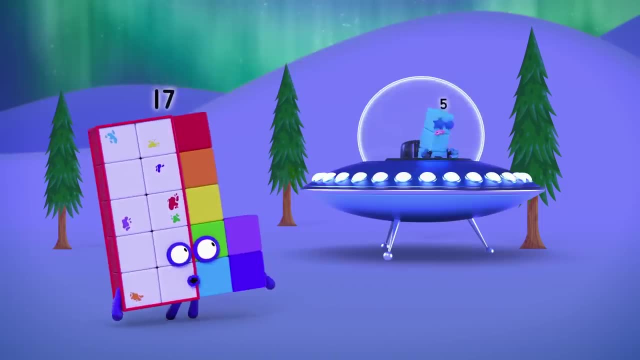 and my factor beam divides you into fives, But only if there are no blocks left over. Whoa, Whoa, Whoa, Whoa. What, What can I say? There's just no dividing some people, Ha-ha. 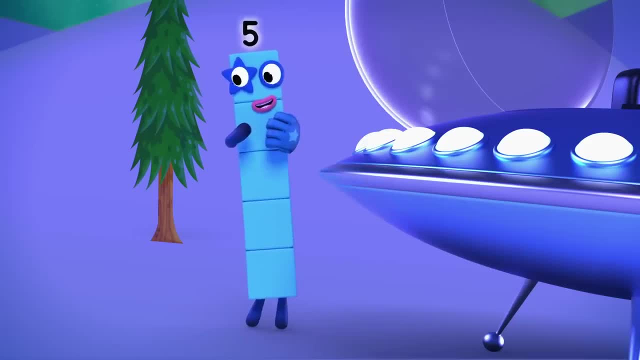 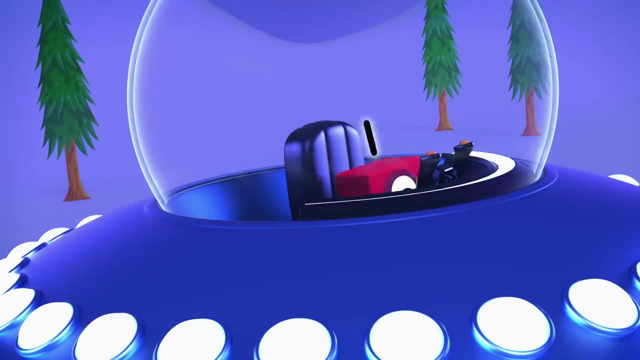 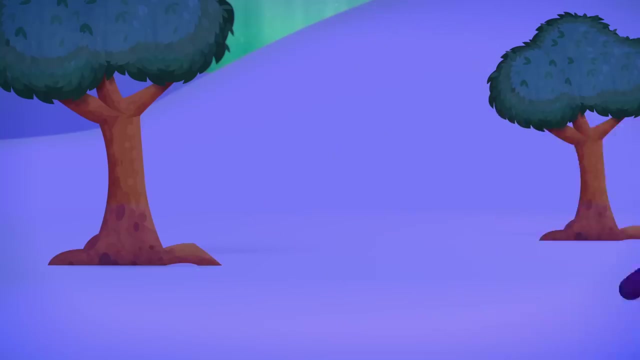 I know how to stop the terrible twos And I know who can stop them. Mission accepted: Factor beam reset. Divide into ones. Uh-oh, Uh-oh, Ah, Uh-oh. How many ones in two? Two, of course. 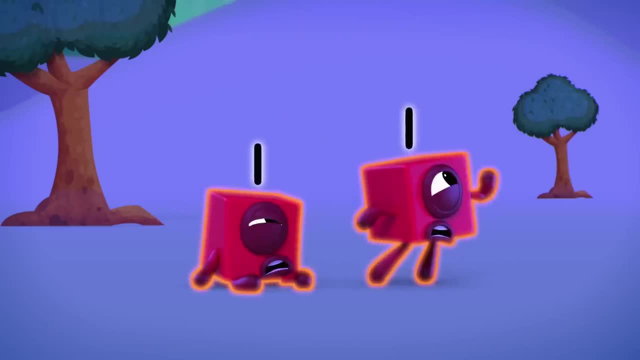 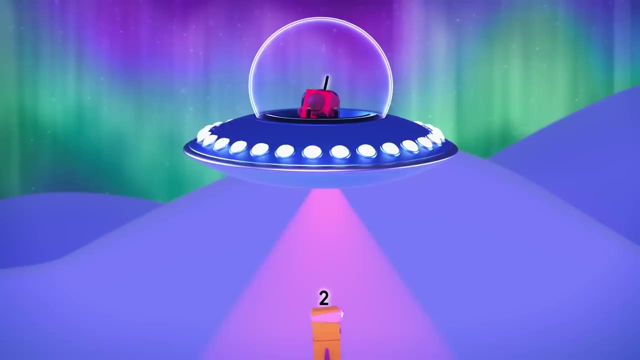 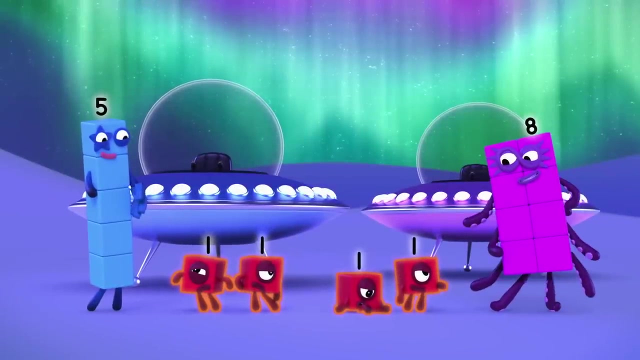 Ah, Double, Bah, Ha-ha-ha-ha, Whoa, Ha-ha-ha-ha, Oh, Oh, Whoa. Never any remainders when you split into ones Bah, Well, well, Aren't you the naughty ones? 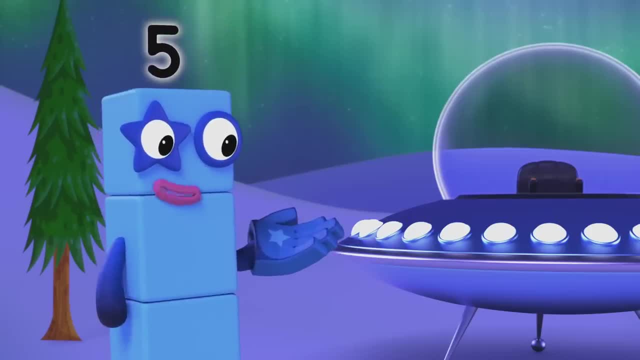 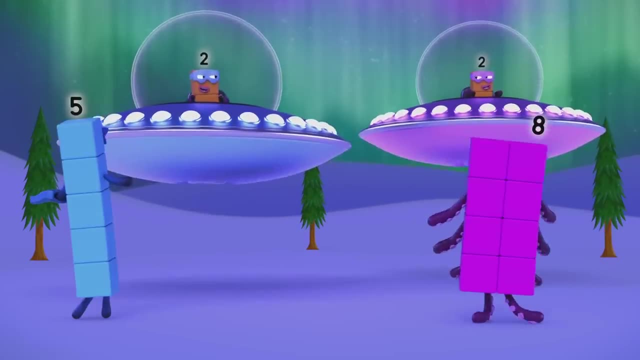 Ha-ha-ha, Don't worry, The factor beam wears off in time. Well, I don't think we'll be having any more trouble from Wait, Where have they gone? Ha-ha-ha-ha, Watch the skies. 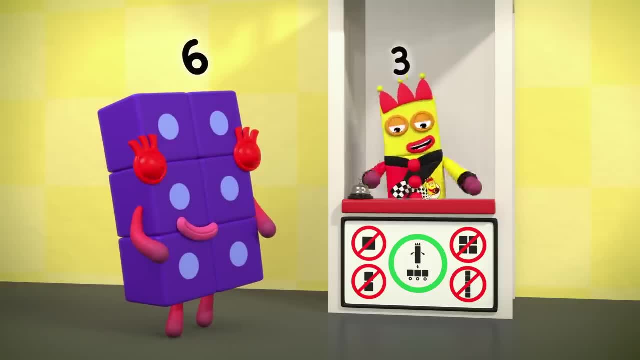 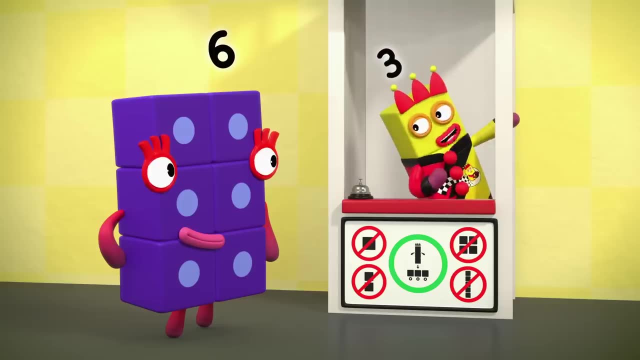 Welcome to my divide-and-drive go-kart track. How many karts do you need? What do you mean? how many? Isn't one enough? No, no, no, Only threes can fit into my go-karts, so you'll need to divide into threes before you can drive. 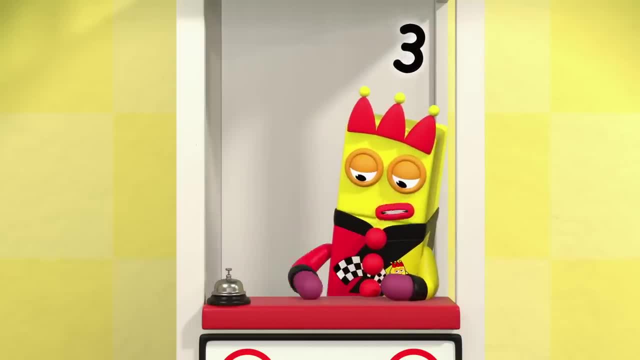 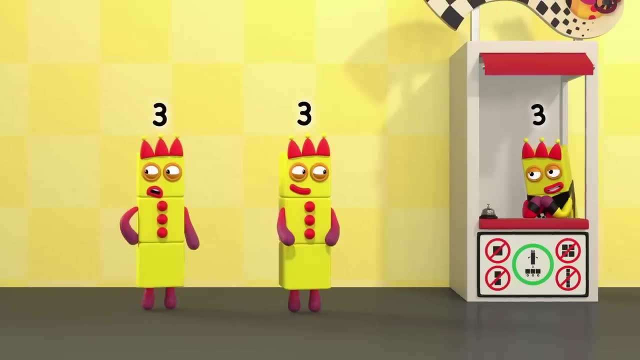 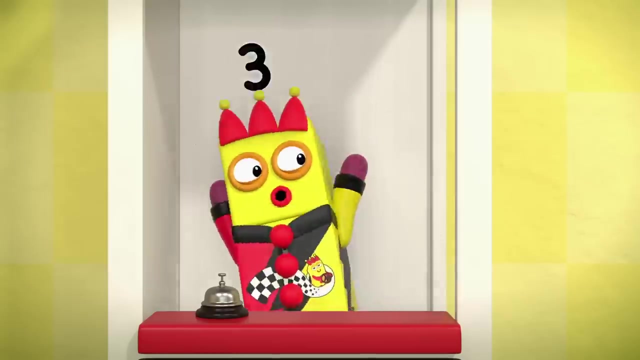 Divide and drive, take off three and we'll see what's left. Six minus three equals three. There you go. There are two threes in six, so you need two karts. Off you go, Ha-ha-ha-ha. 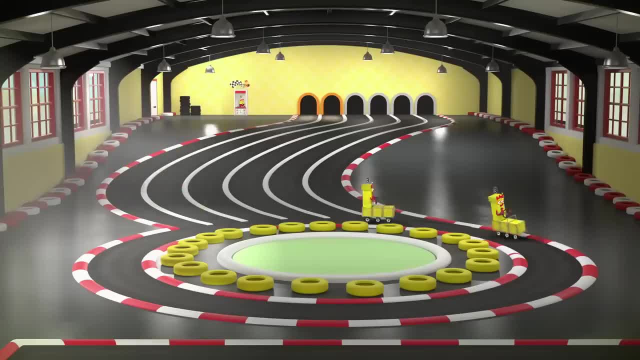 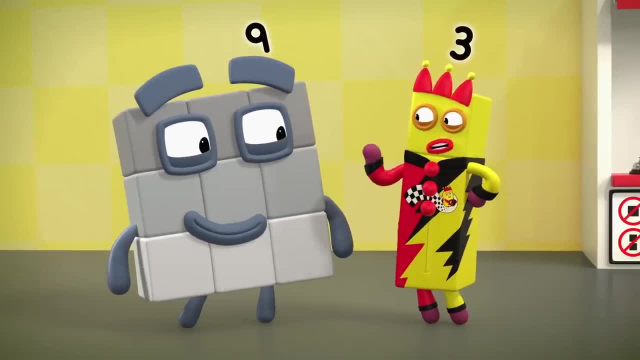 Ha-ha-ha-ha, Whee, Ha-ha-ha-ha. Yikes, Lots of customers. Nine: How many karts do you need? How many threes in nine? Huh, Leave it to me. I'm good with threes. 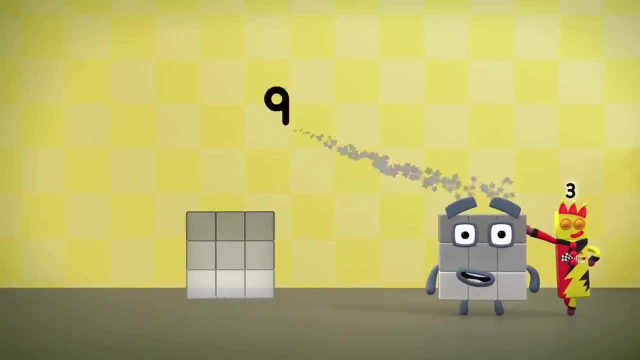 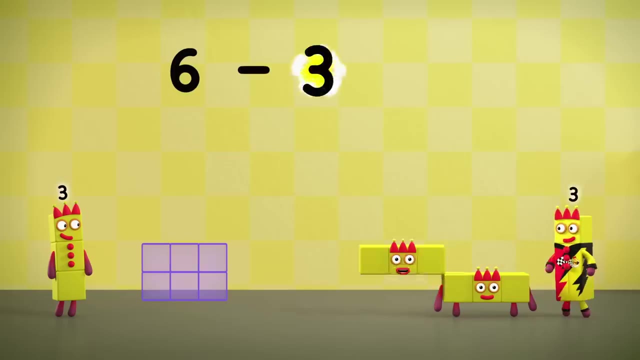 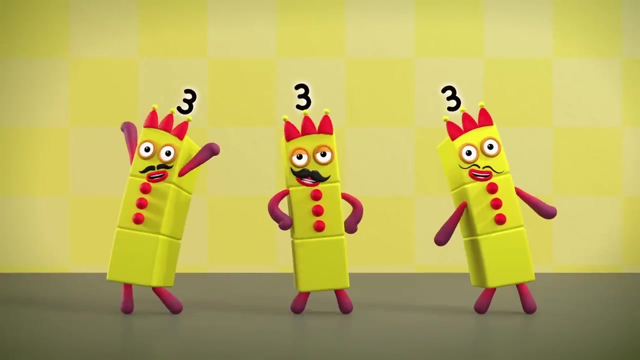 Let's take a three off: Nine Minus three equals six, And again: Six Minus three equals three. Hey, One, two, three, The three threes. Yes, yes, yes, Oh, can you please move faster? 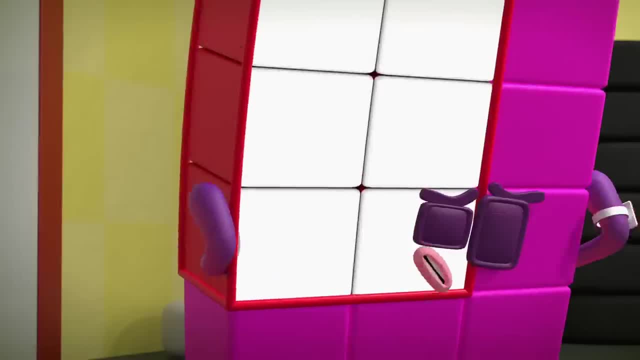 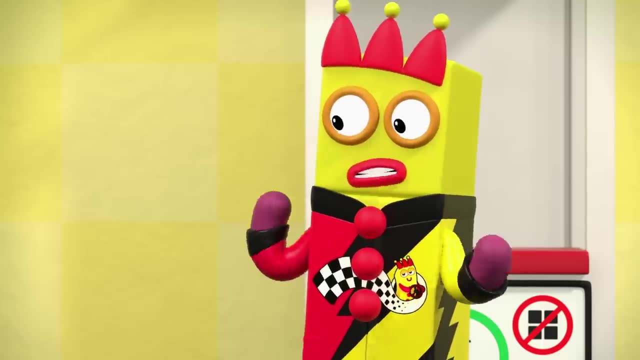 Some of us can't wait to go-go-go-kart. Hey, hey, hey, I'm going as fast as I can. you know, Subtracting threes one by one is a slow business. I mean, if you know a faster way of dividing into threes. 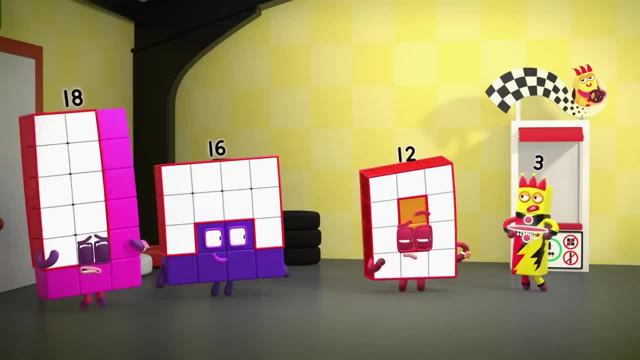 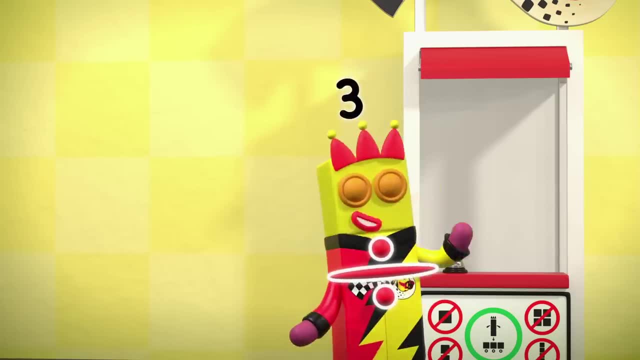 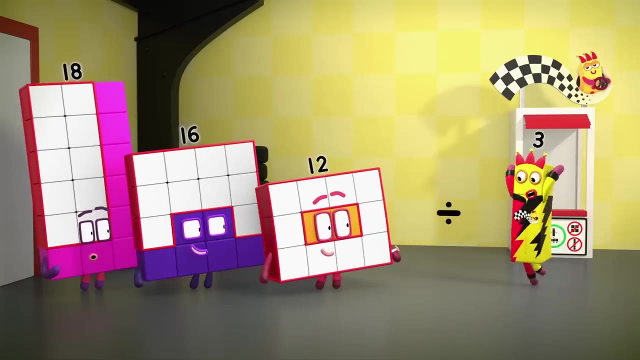 you tell me Turn Mm-hmm. Oh, I know, Juggling helps me think: Oh, It's time. Oh, Oh, It's a sign, A new sign. Maybe this can help me divide you up faster. 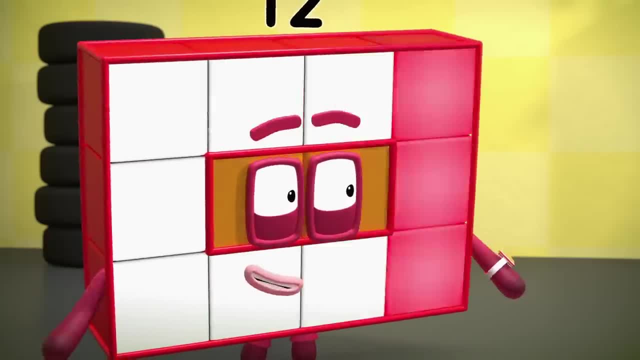 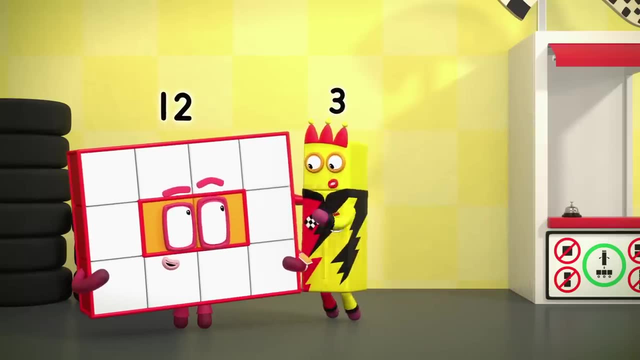 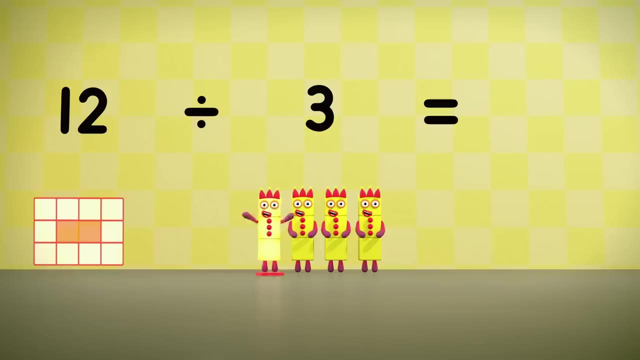 Let's see. Look, can't you see? I'm keen to try something new. Instead of taking threes away over and over, let's divide you into threes all at once. Twelve divided into threes equals One, two, three, four. 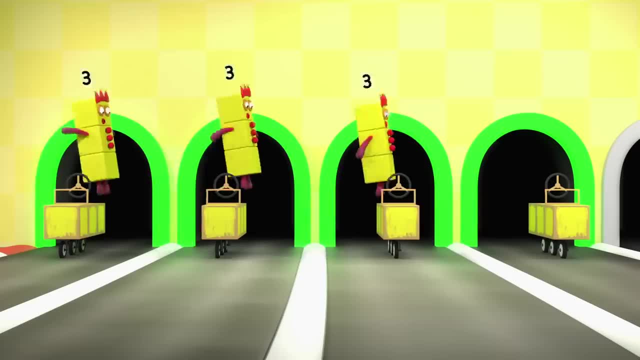 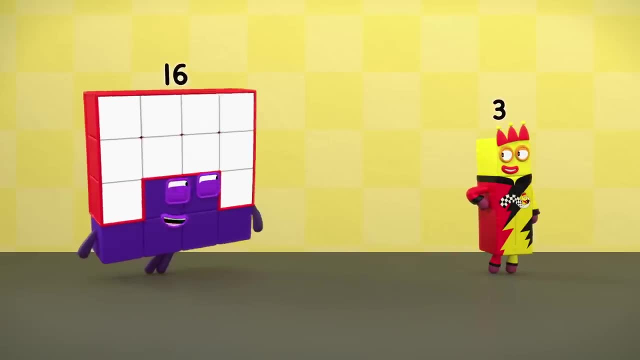 There are four, threes in twelve. Woo-hoo, Whee, Whee. Oh, I can divide anyone like this, Anyone. you say Why I'm anyone Give it a go. Sixteen, No, no, no. 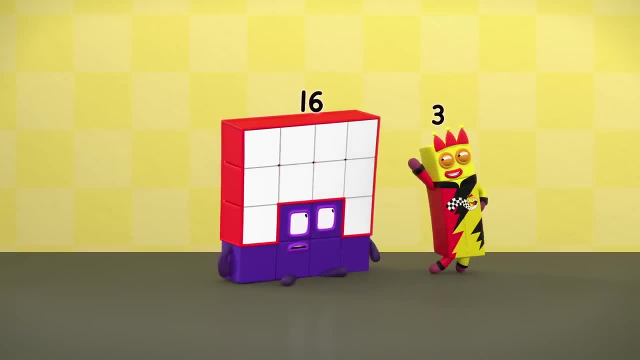 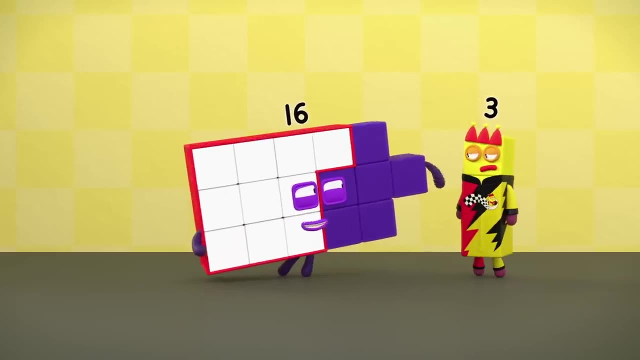 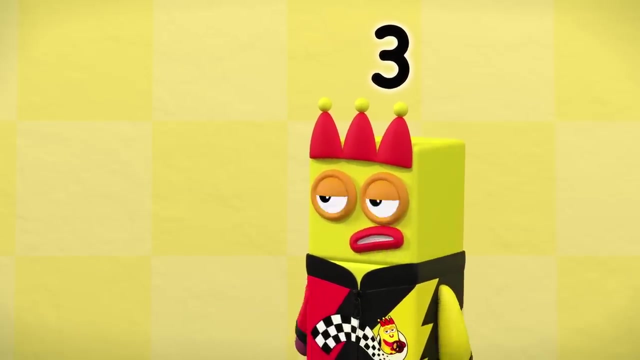 You need to make a rectangle that's three blocks high, like twelve did. Nope, not going to happen. Got this one block remaining on the end. I guess I can. I can't divide you into threes without leaving some of your blocks behind. 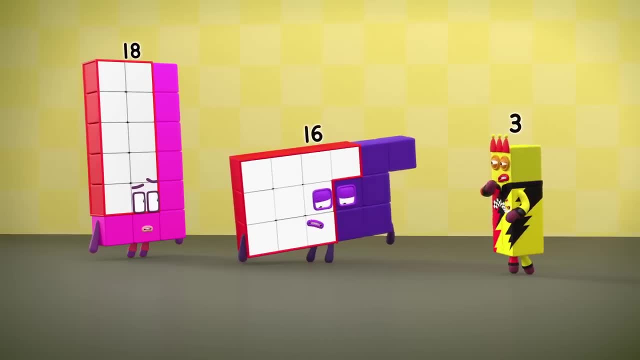 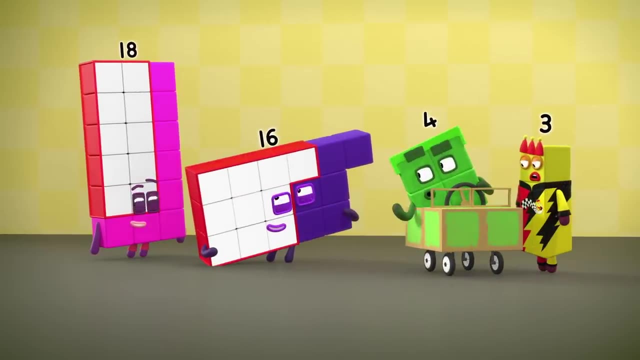 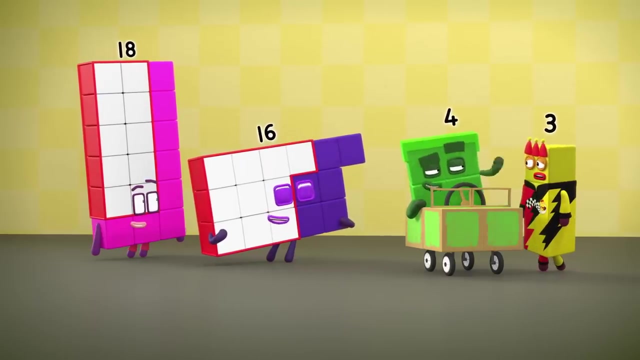 Sorry, sixteen, but you won't fit in my go-karts. Oh, Excuse me. coming through, Who wants to go on my go-kart track for four-wheel drivers? Ooh, can I try? Sorry, three, only fours can drive my karts. 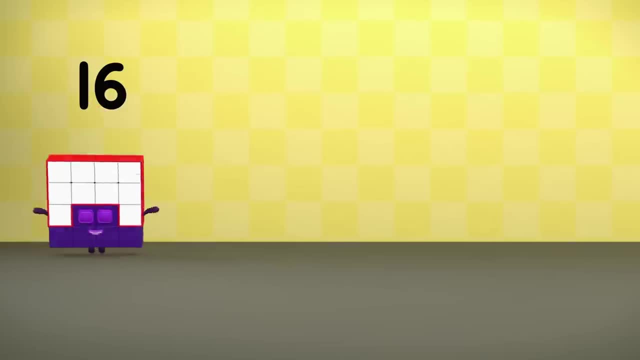 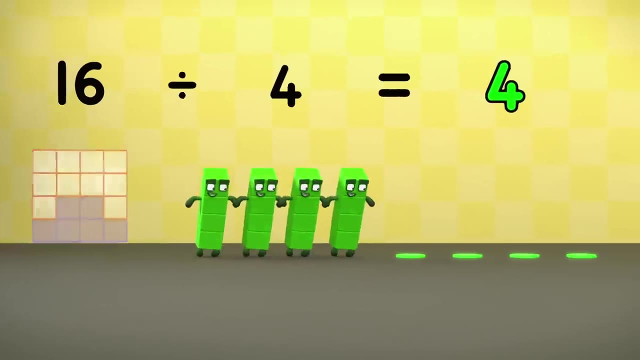 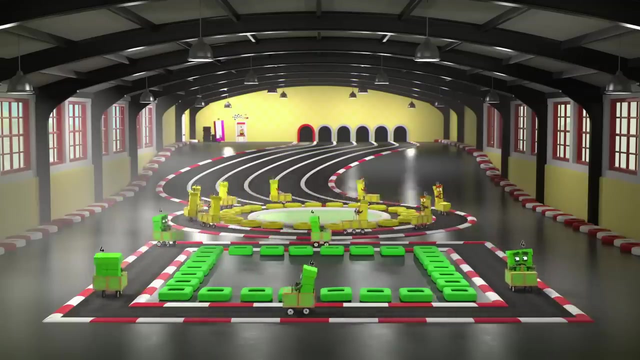 Oh, maybe I can. Sixteen divided into fours: One, two, three, four, The four fours. Ooh yeah, Ha-ha-ha-ha-ha, Woo-hoo, Literally unable to wait a moment longer. 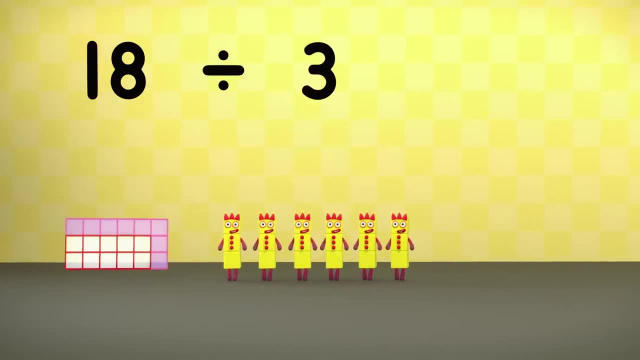 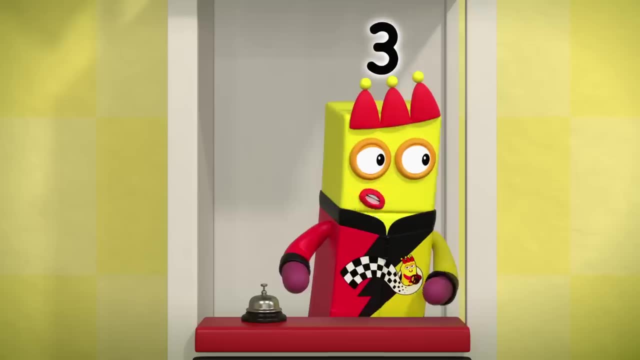 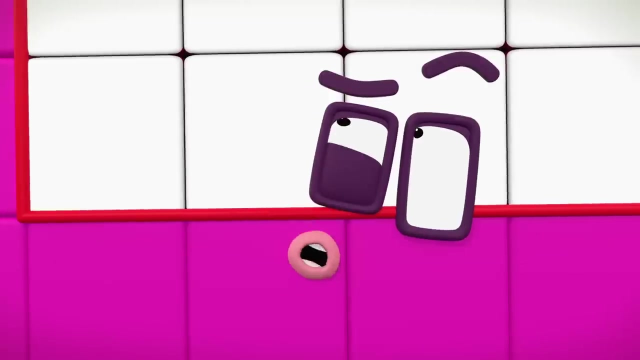 Eighteen Divided into threes equals One, two, three, four, five, six. All right, yeah, Six times three, Three equals Eighteen. What do you know? Division is the opposite of multiplication. Here I go again. 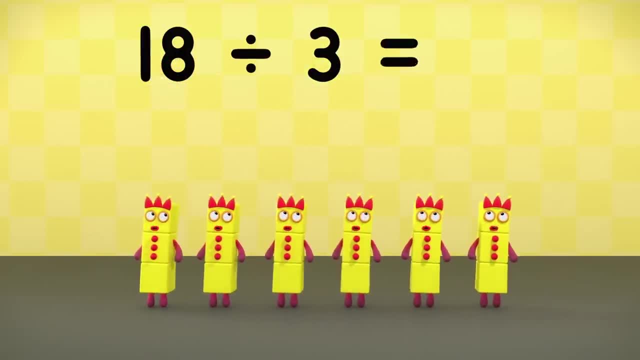 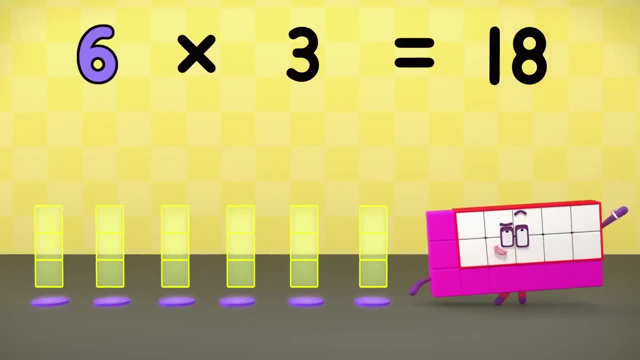 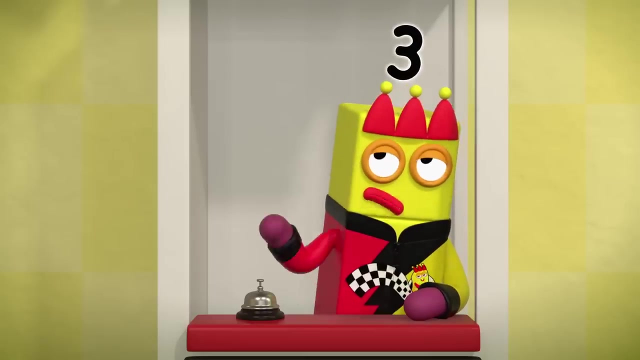 Eighteen Divided into threes equals Six. Six times three equals Eighteen. I could do this all day, So I will. Eighteen Divided into threes equals. Some rulers are just born to show off. Six times three equals. 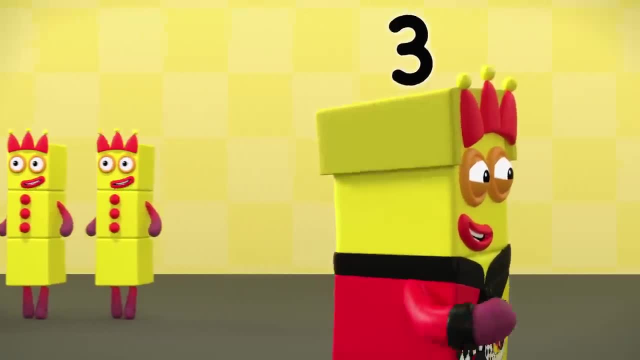 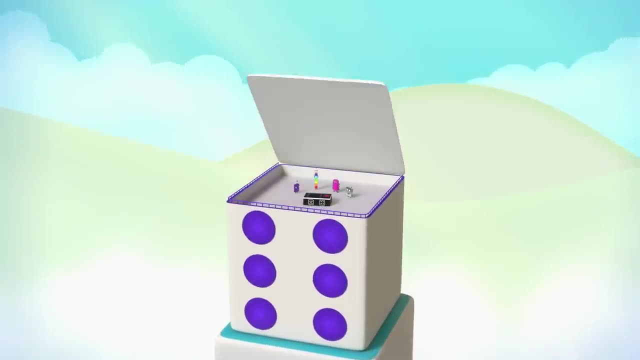 Eighteen Divided into threes equals. Look at me. Ha-ha-ha-ha-ha-ha, Ha-ha-ha-ha-ha-ha, Ha-ha-ha-ha-ha-ha, Thank you for coming to play my big new game. 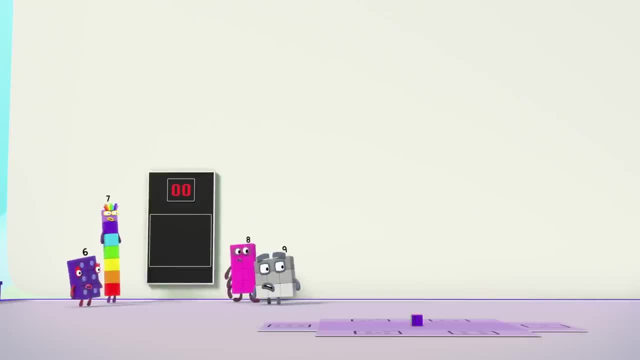 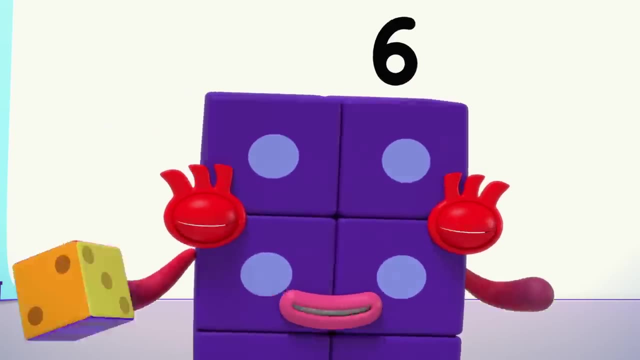 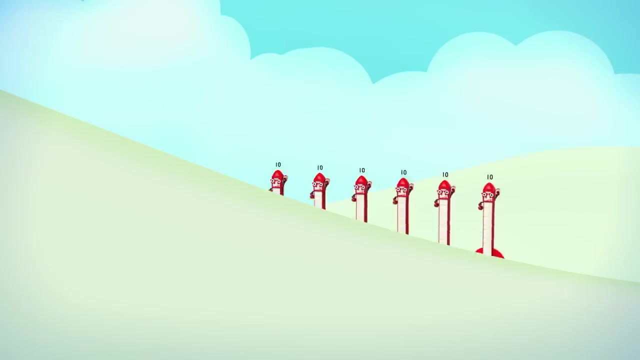 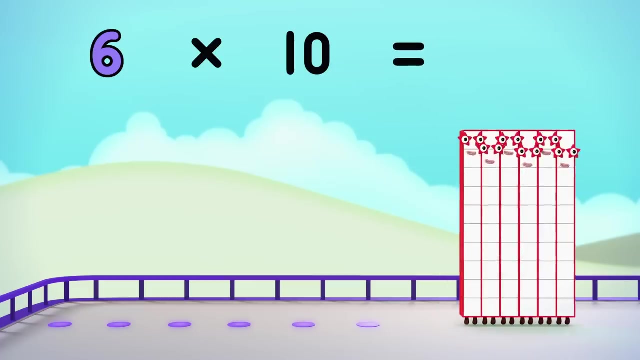 Ha-ha, Huh, I'll roll the dice to start my friends. This game is called How Many Tens? Hmm, Six, Ooh. Six times ten equals Sixty. I am Sixty here to play with Sixty Spots. Hip, Hip Hooray. 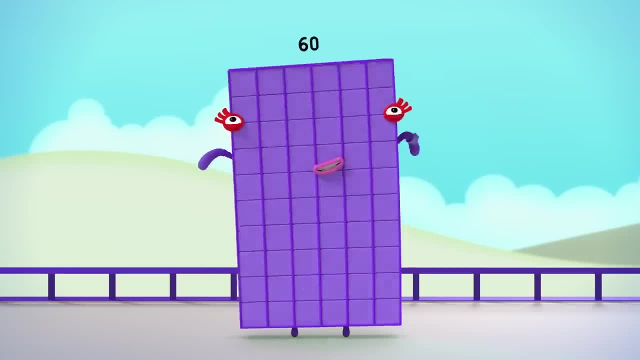 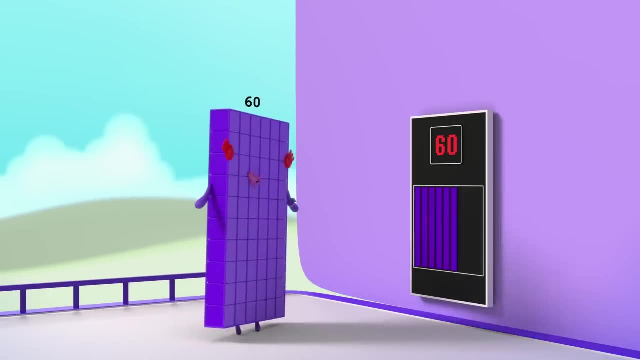 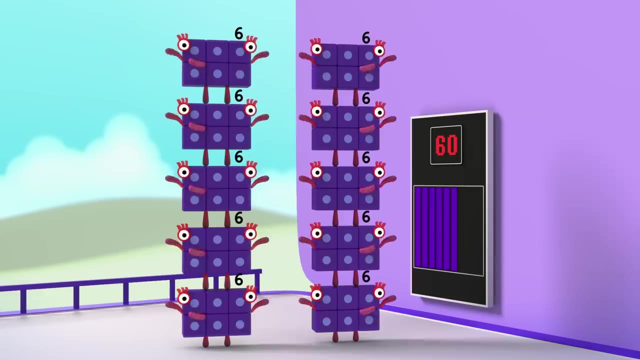 Wow, Ho-ho-ho-ho, Sixty. I am Sixty. here to play with Sixty Spots, Hip, Hip, Hooray. Six, lots of ten is a new high score. I'm six, tens or Ten sixes. 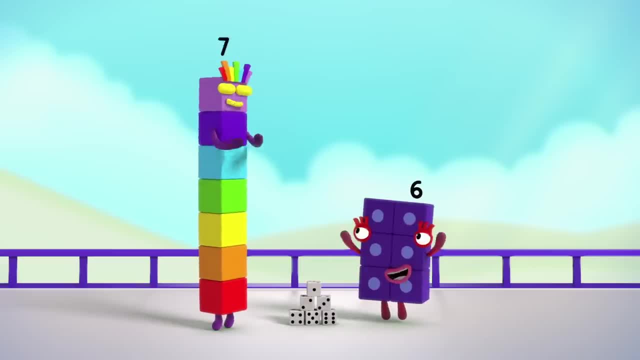 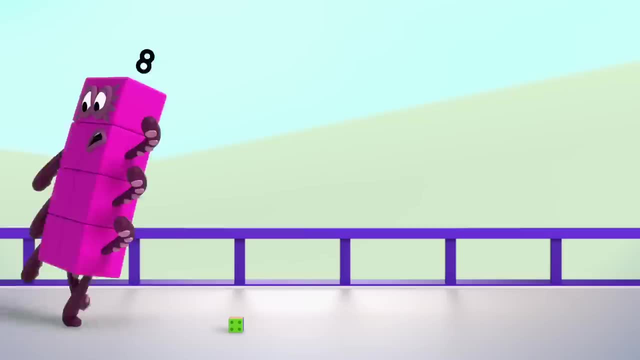 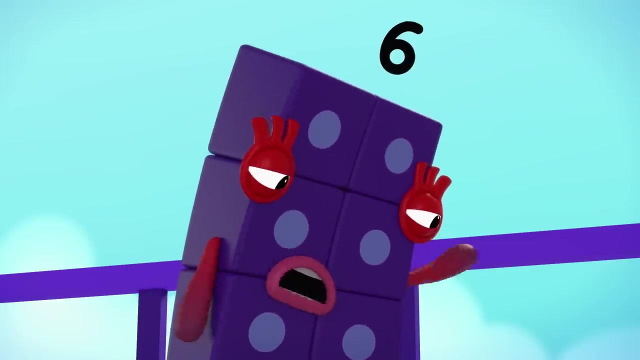 Game on: Yeah, Hee-hee, Ha-ha. Come on Nine, we can Ha-ha-ha-ha-ha, Uh-oh, Oh, Oh. no, The special game dice. Huh, I don't see that dice again. 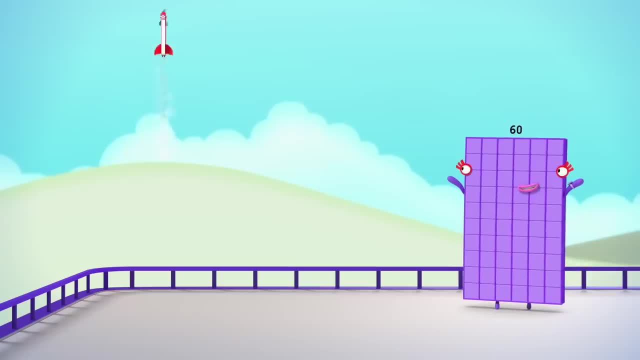 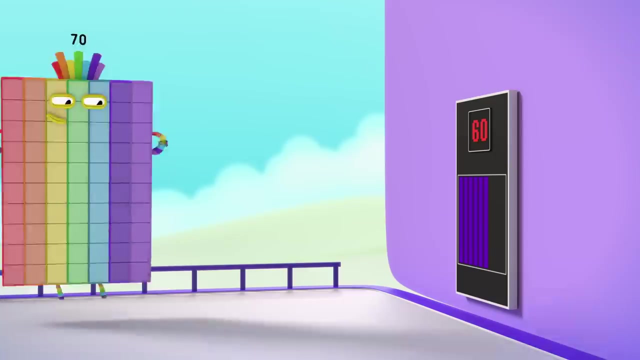 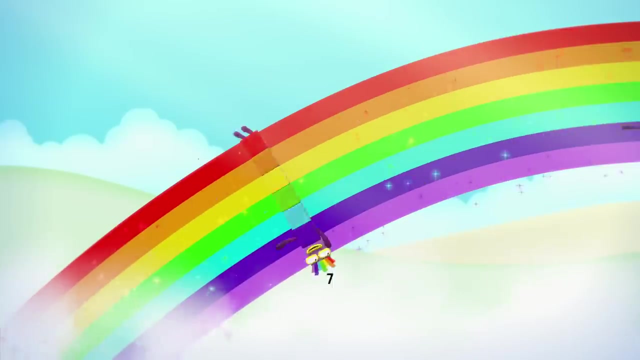 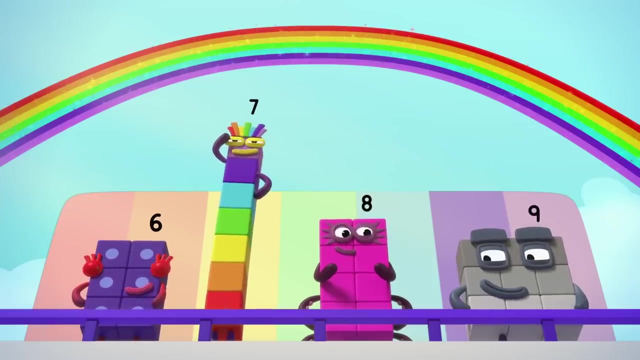 This calls for another ten. Seven times ten equals Seventy. I am Seventy. you lucky numbers. As luck would have it, I'm seven tens, so I'm also Ten sevens. The Rainbow Connection- Ooh, I see it, It's way over there. 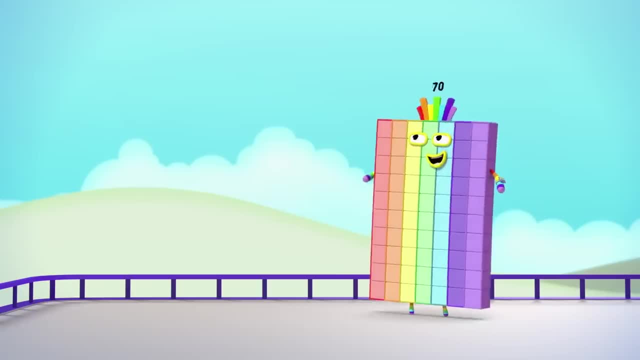 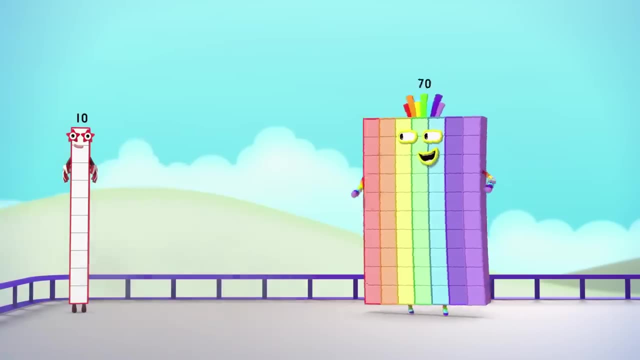 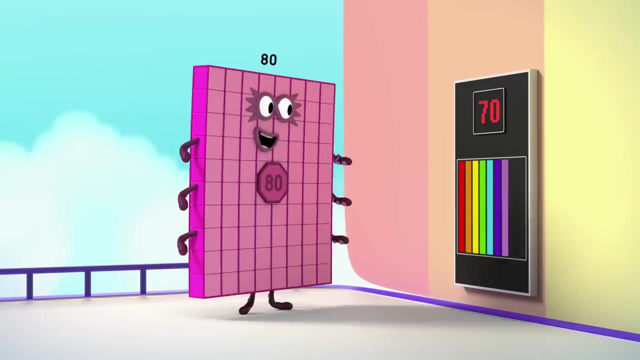 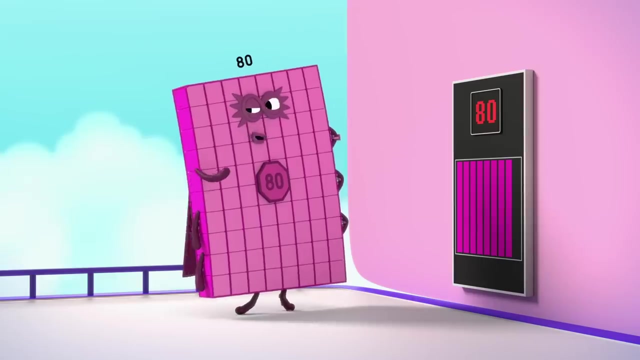 But how can we get it back again? Luck is in the air tonight. Here comes another ten. Eight times ten equals Eighty. I am Eighty. Super Octoblock to the rescue. Oh, Oh, Secretly, I'm eight tens. 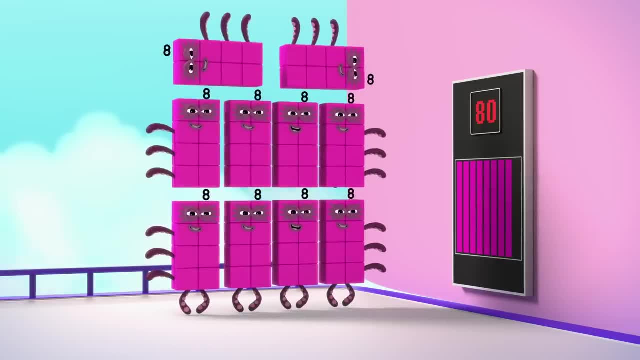 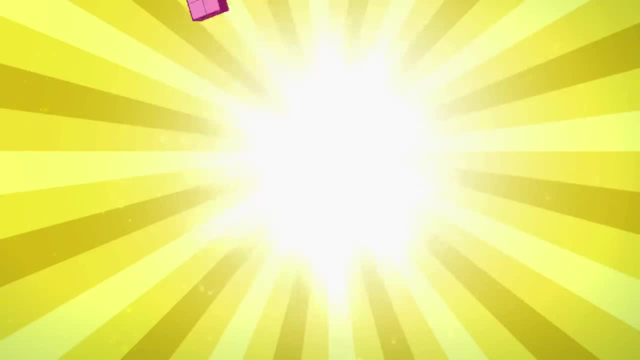 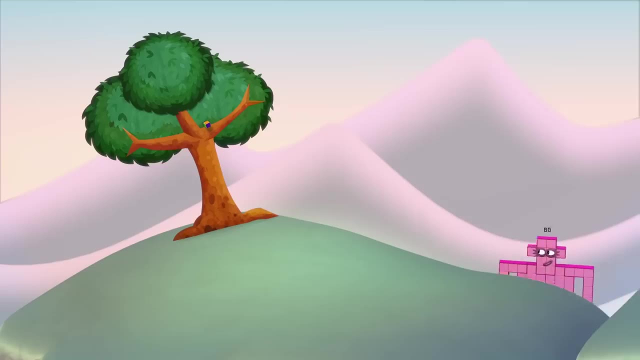 But this is a job for Ten eights Octoblocks. assemble Roboctoblock forward. Oh, Ha-ha, Ha-ha, Ha-ha, Ha-ha, Ha-ha, Mmm. Ha-ha. 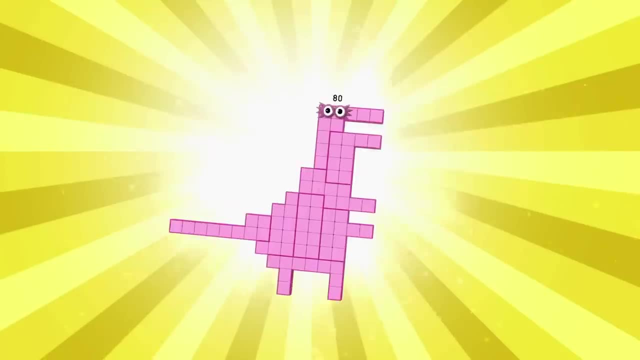 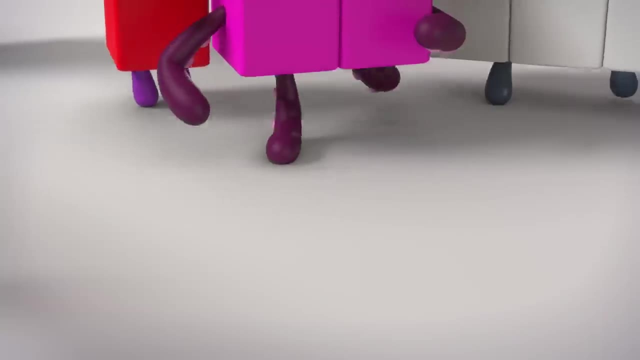 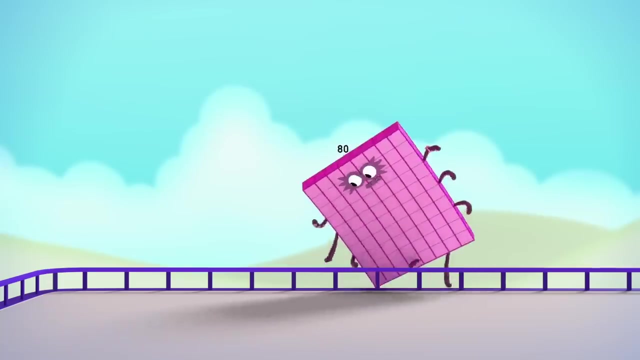 Mmm. Ha-ha-ha, Ha-ha, Ha-ha, Ha-ha, Din-octoblock smash. Ha Whoa Eighty's the biggest hero of all. Oh, there's always someone bigger. 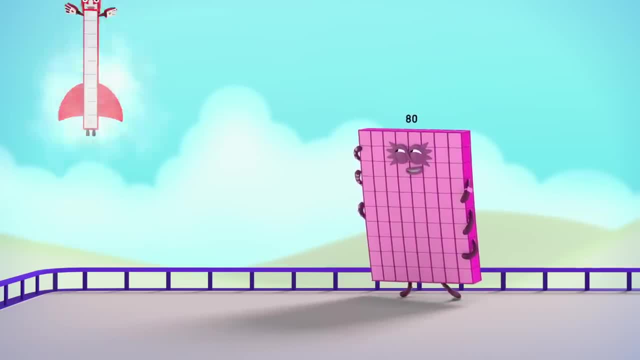 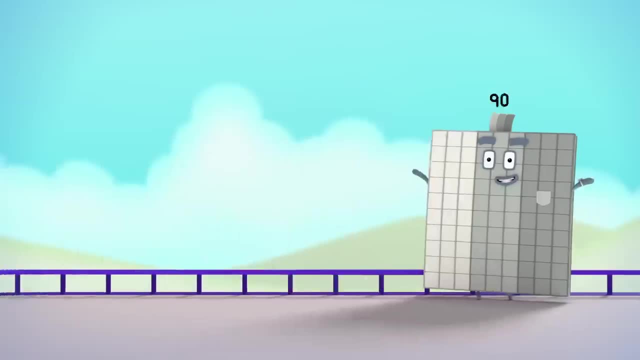 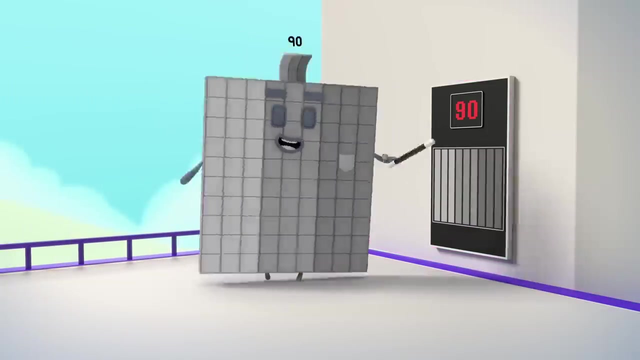 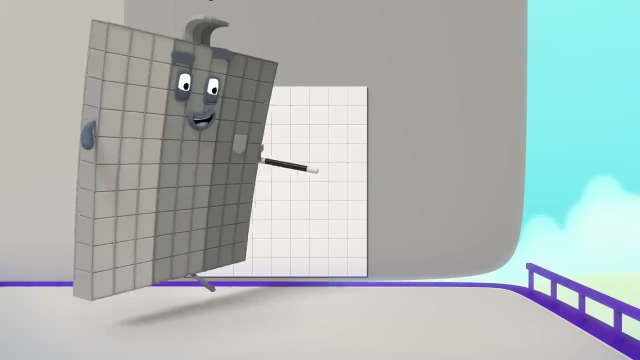 Look Up in the sky, It's Another ten. Nine times ten equals Ninety. I am 90!. You won't believe your eyes. Are you a square or not? I can't tell. This grid is ten blocks by ten blocks. 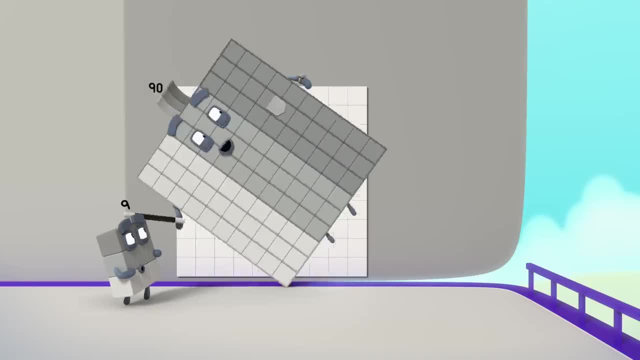 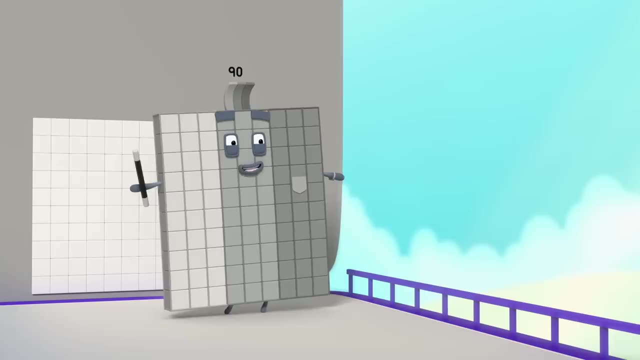 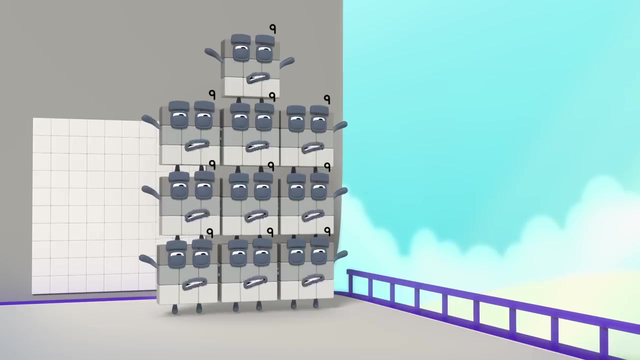 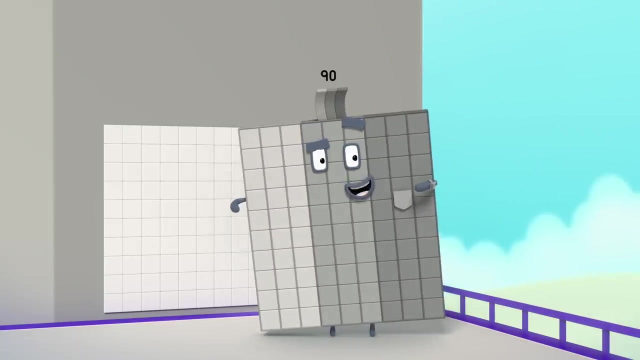 But I am one column short or one row. Either way I'm not all square. And now a vanishing trick. Ten lines: Now you see us, Now you don't. And what have we got here? Ten Twenty. 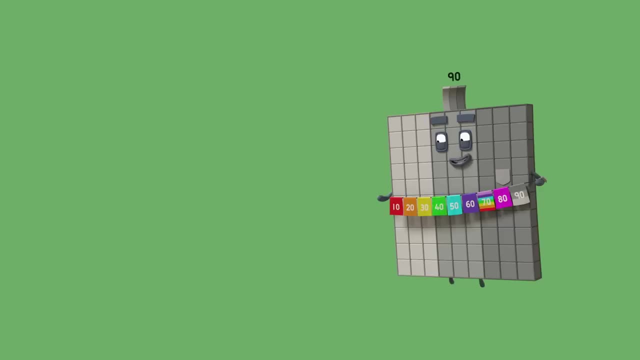 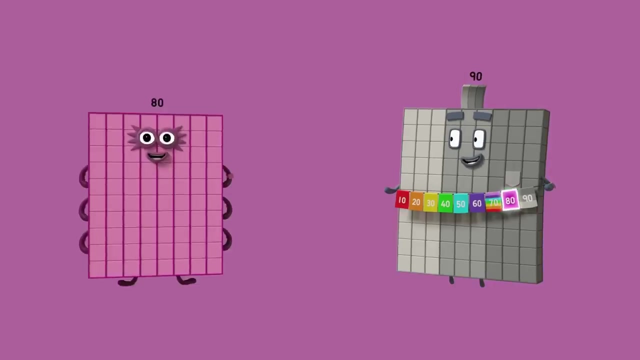 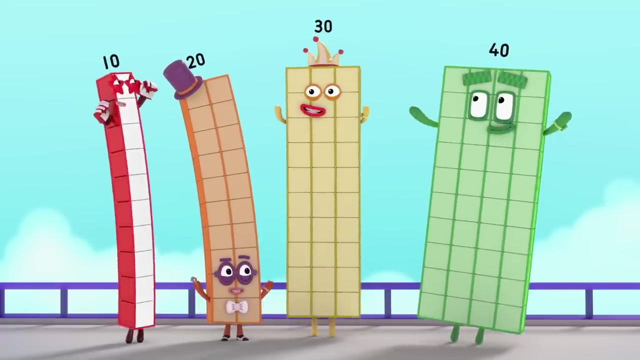 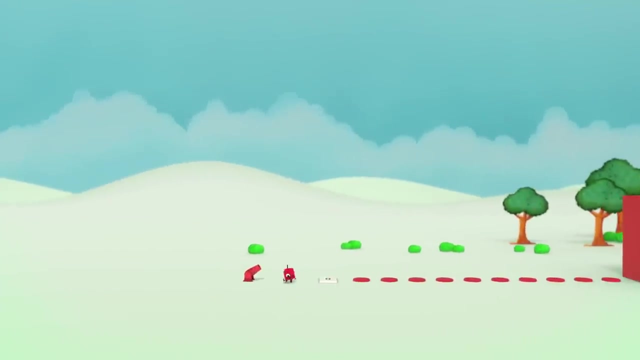 Thirty, Forty, Fifty, Sixty, Seventy, Eighty And Ninety. Ninety's got the highest score, but I wonder, Hello one, What are you up to? Hello zero, Today's the big one. 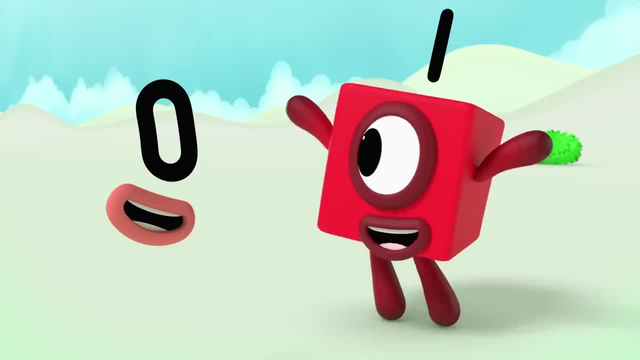 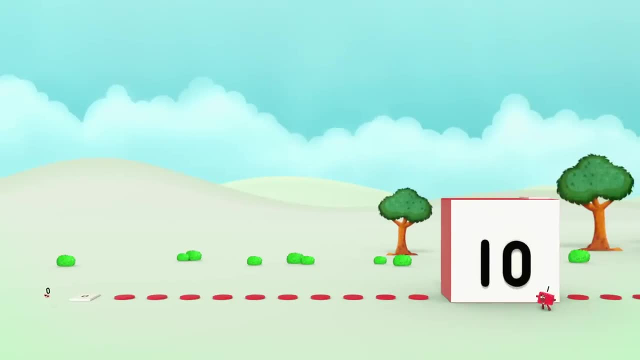 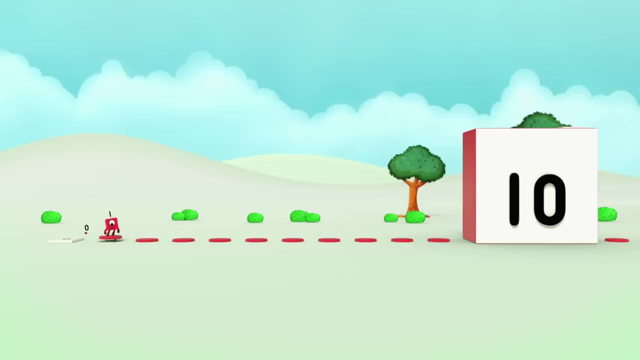 I'm going to count higher than I've ever counted before. Ooh, I've got ten fantastic flippers like this one, Ten tall towers like that one And ten, lots of ten springy springs. Whee, That looks fun. Can I have a go? 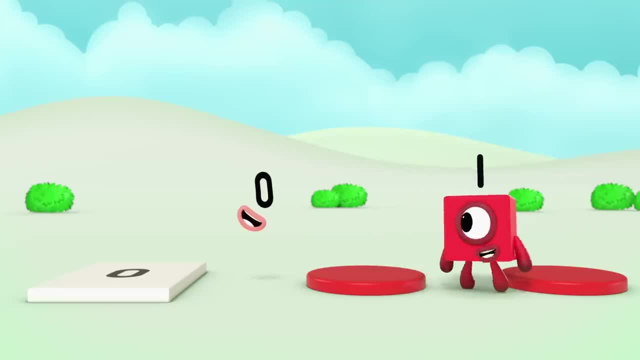 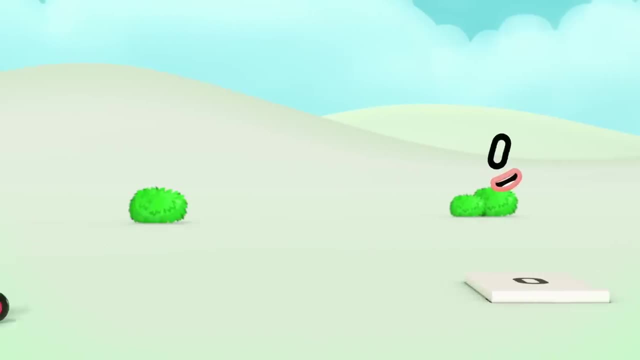 I was counting on it. There's a flipper here with your number on. Then let's go for it. Great, But we need to go fast so we reach the last tower in time to catch this. Ha, Zero, Ha. 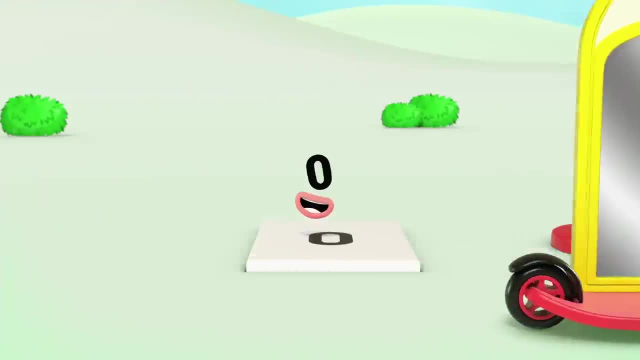 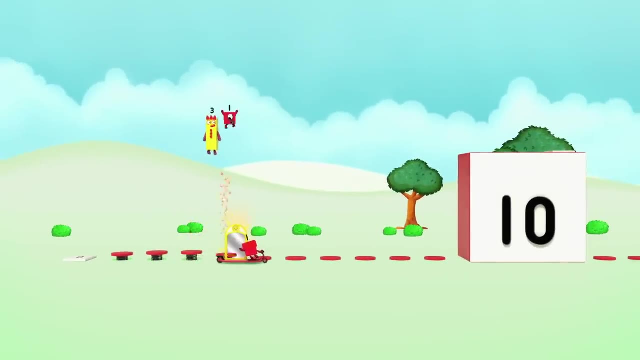 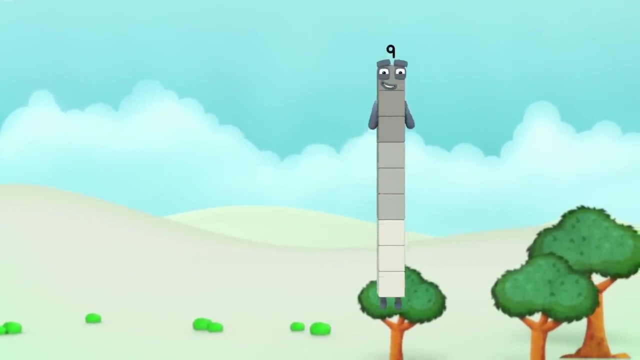 One, Two, Three, Four, Five, Six, Seven, Eight, Nine, Ten Coming in for landing. Keep going, Every second counts And clear for launch: Eleven, Two, Three, Four, Five, Six, Seven. 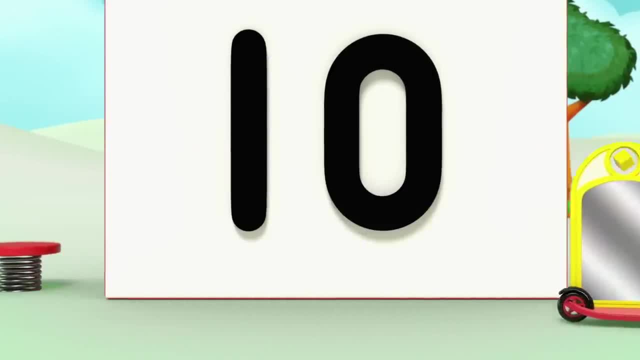 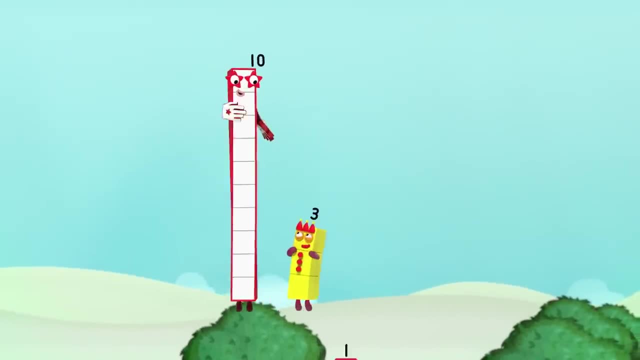 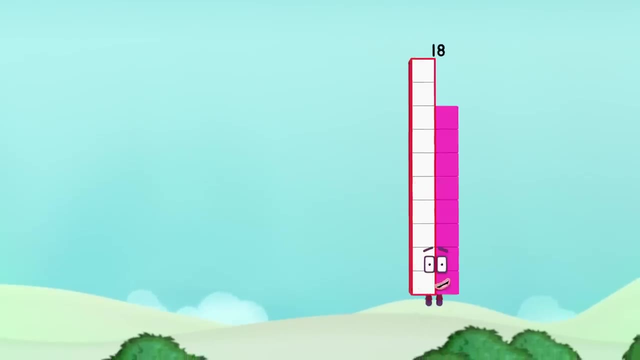 Eight, Nine, Ten Coming in for landing. Keep going, Every second counts. Eleven, Twelve, Thirteen, Fourteen, Fifteen, Sixteen, Seventeen, Eighteen, Nineteen, Twenty. We're going to make so many new friends today. 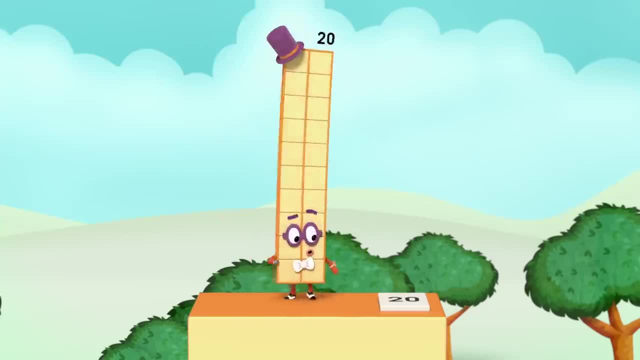 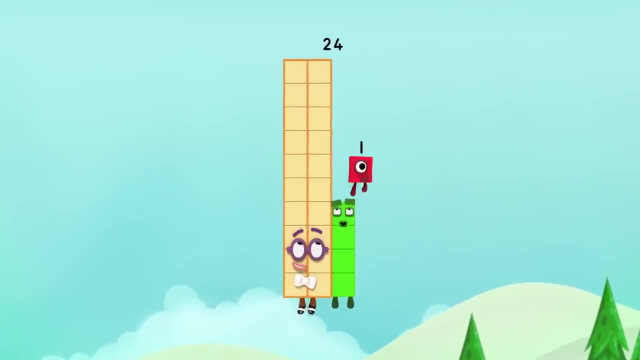 Whee. Twenty-one, Twenty-two, Twenty-three, Twenty-four, Twenty-five, Twenty-six, Twenty-seven, Twenty-eight, Twenty-nine, Twenty-nine, Twenty-eight, Twenty-nine, Twenty- stör perch Twenty-nine, Twenty-eight. 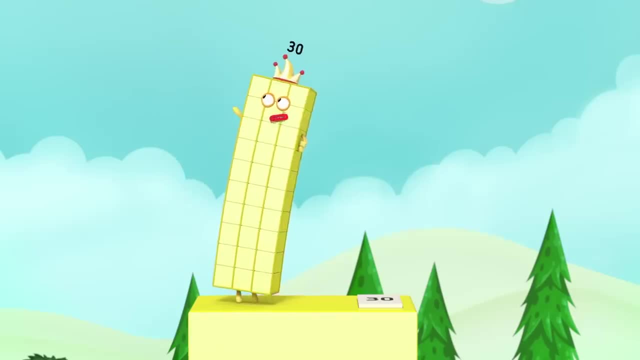 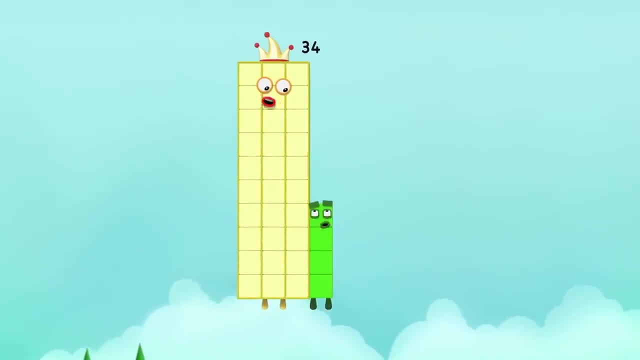 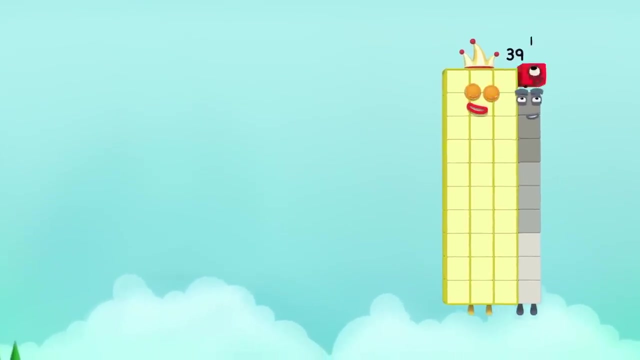 Twenty-nine, Thirty- Excellent acrobatics. everybody On with the show. Thirty-one, Thirty-two, Thirty-three, Thirty-four, Thirty-five, Thirty-six, Thirty-seven, Thirty-eight, Thirty-nine, Forty, Ooh, I like the flipper. It's rectangular. 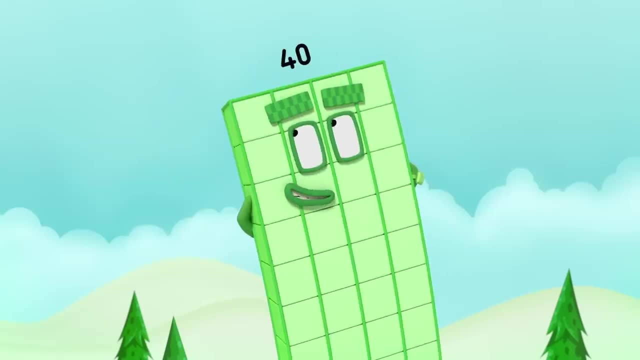 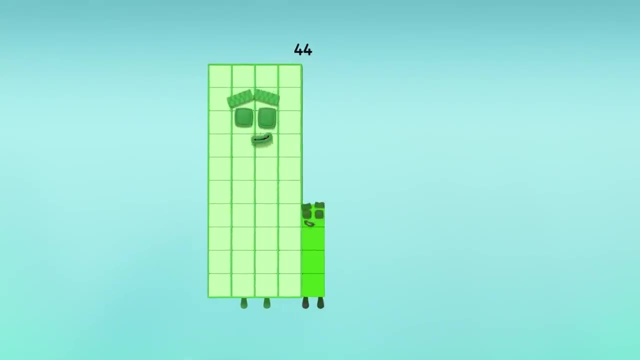 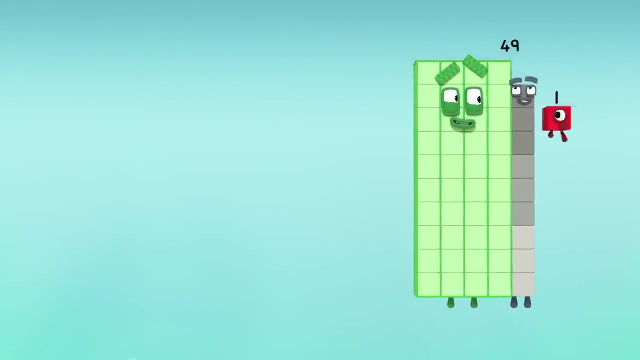 Stay focused. We can do this, Sorry, Ahem. Oh. Forty-one, Forty-two, Forty-three, Forty-four, Forty-five, Forty-six, Forty-seven, Forty-eight, Forty-nine, Fifty, We're halfway there, Ooh. 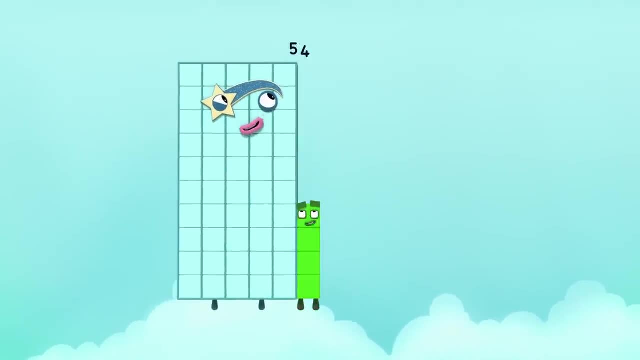 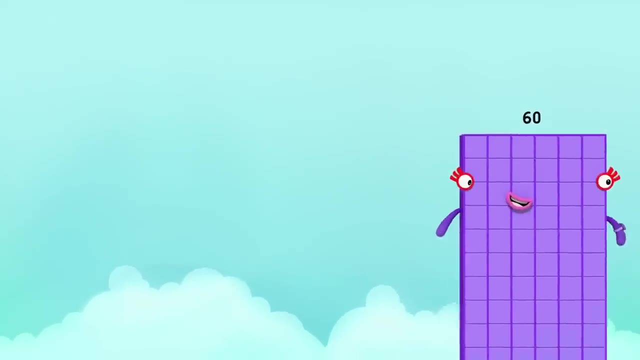 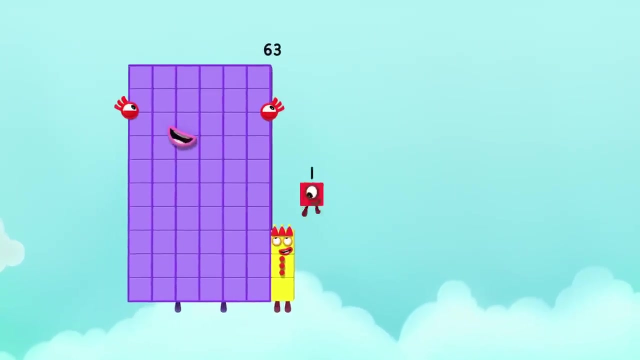 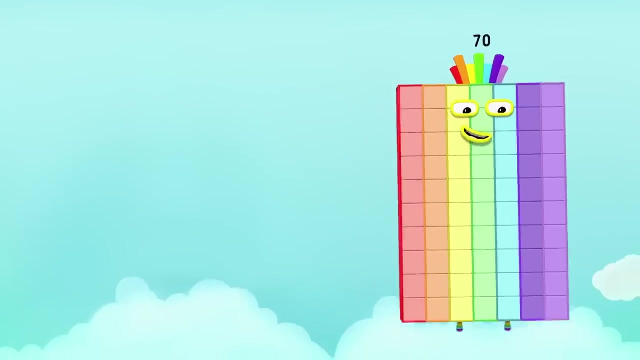 Fifty-one, Fifty-two, Fifty-three, Fifty-four, Fifty-five, Fifty-six, Fifty-seven, Fifty-eight, Fifty-nine, Sixty. Racing through the sky, this high roller's gonna fly. Sixty-one, sixty-two, sixty-three, sixty-four, sixty-five, sixty-six, sixty-seven, sixty-eight, sixty-nine, seventy. 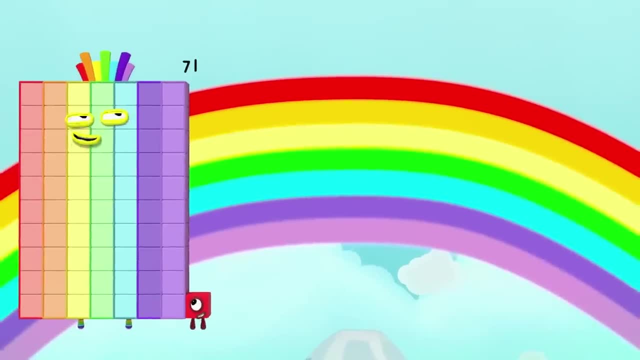 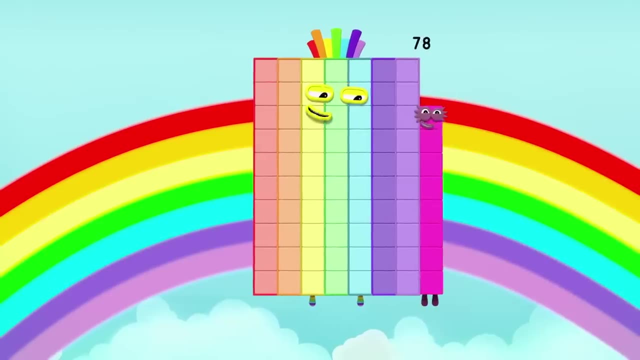 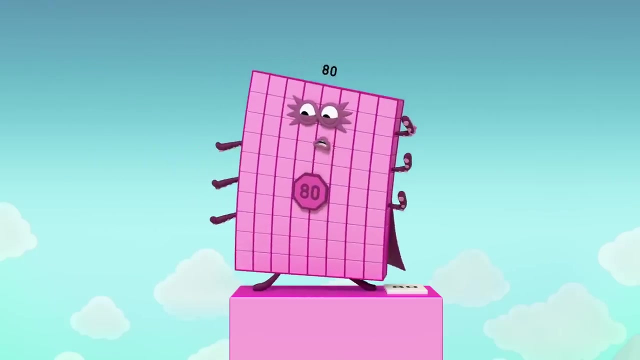 We're going over the rainbow. Seventy-one, seventy-two, seventy-three, seventy-four, seventy-five, seventy-six, seventy-seven, seventy-eight, seventy-nine, eighty. I don't like the look of those clouds. There's no time to stop. 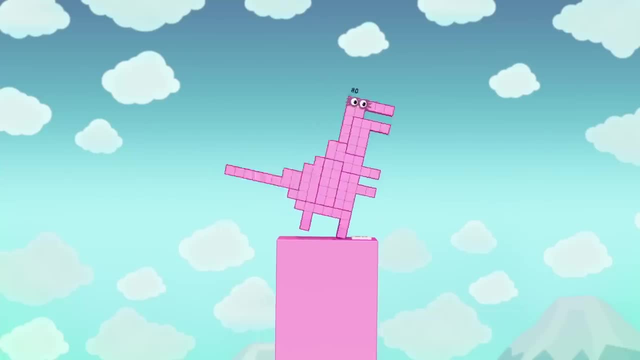 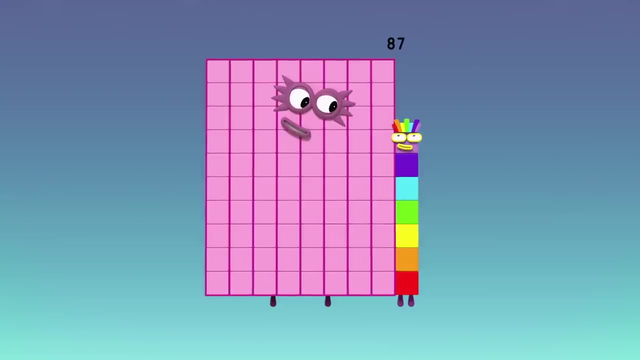 Octoblocks assemble Dinoctoblock roar, Roar Up, up and away. Eighty-one, eighty-two, eighty-three, eighty-four, eighty-five, eighty-six, eighty-seven, eighty-eight, eighty-nine, ninety. 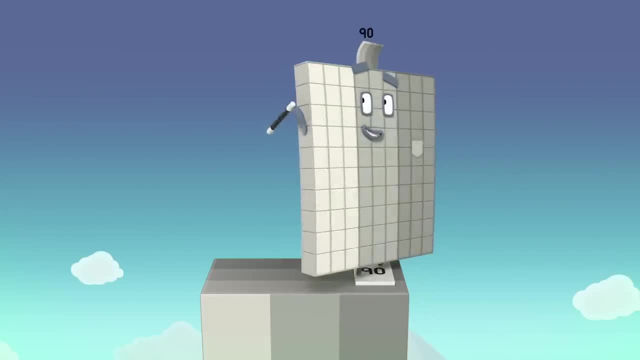 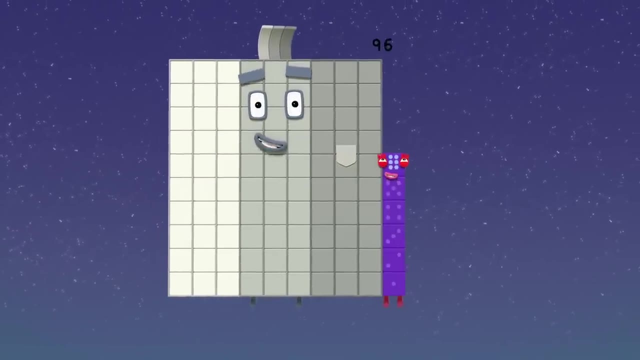 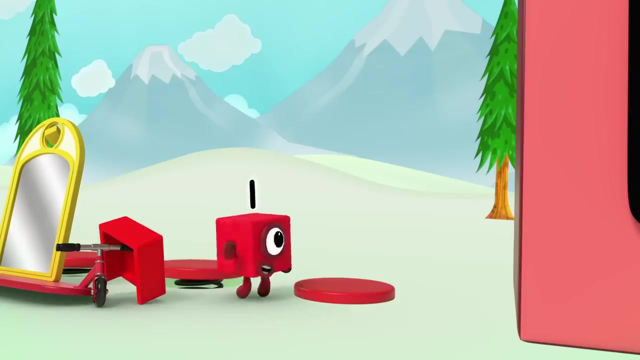 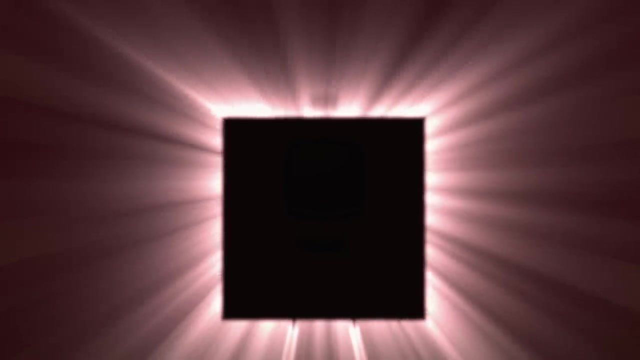 Nearly there. with no time to spare, This should do the trick. Ninety-one, ninety-two, ninety-three, ninety-four, ninety-five, ninety-six, ninety-seven, ninety-eight, ninety-nine, And one more is free, One hundred. 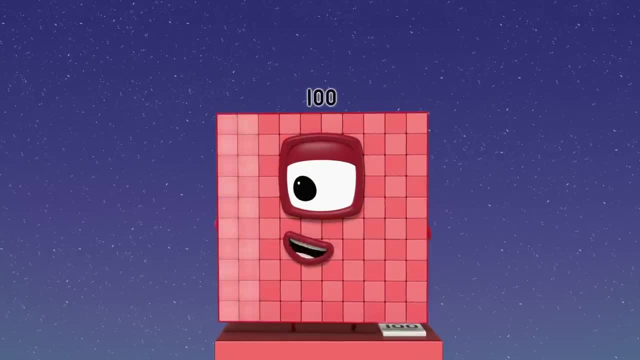 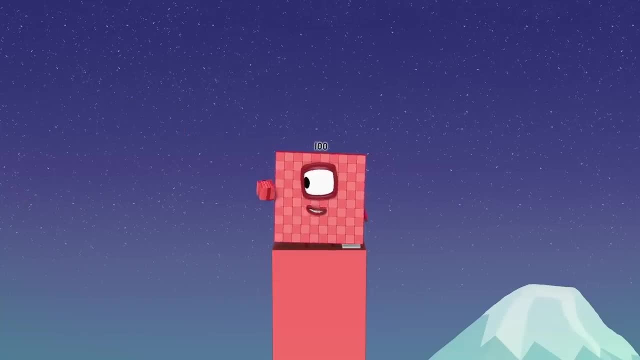 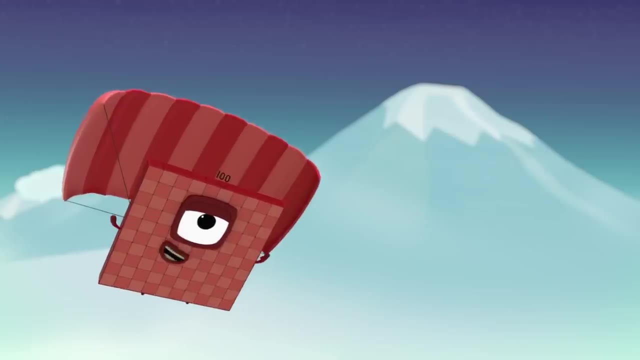 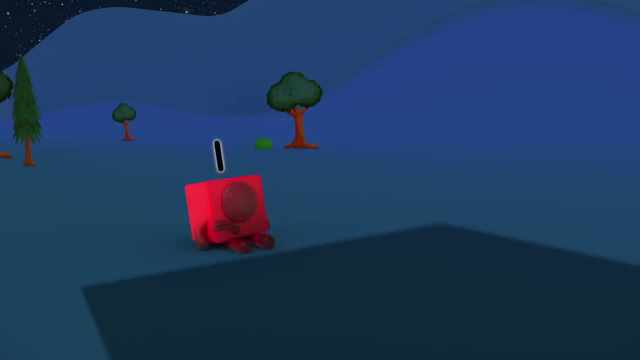 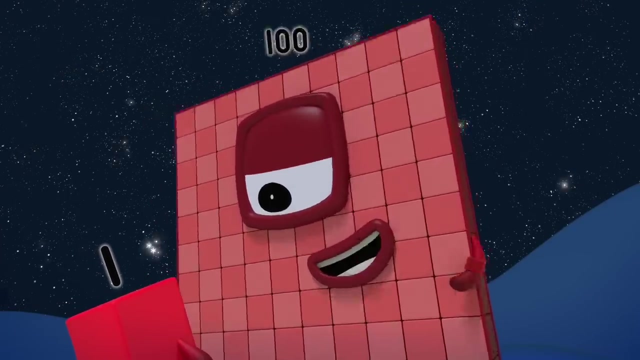 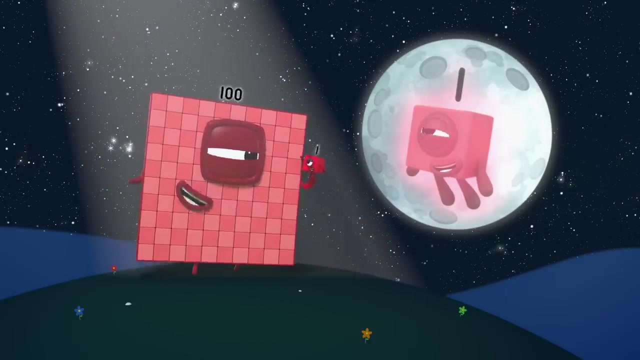 You're here, One hundred, Hello one, You're so big. Yes, little one, I'm a big number, But I wouldn't be here at all If it weren't for you. Look how far we've come. Remember, when there was only one? 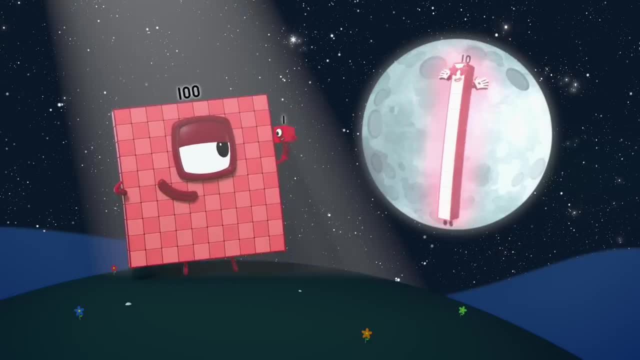 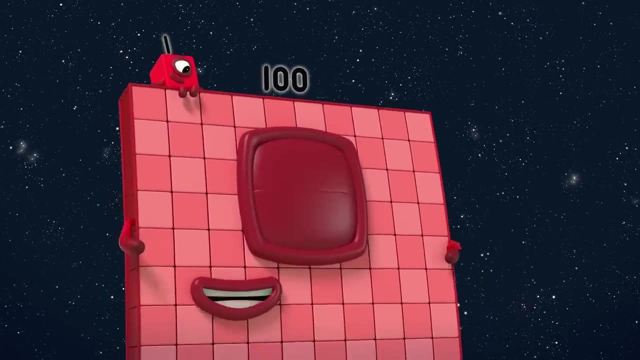 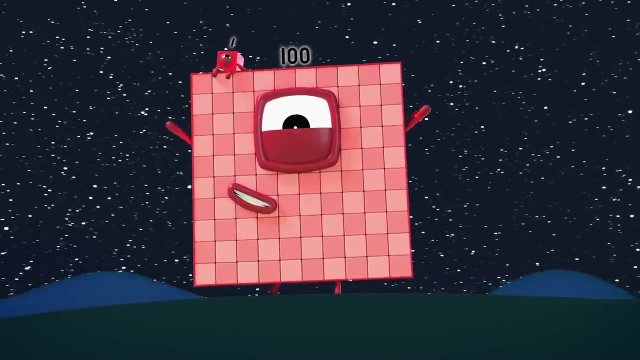 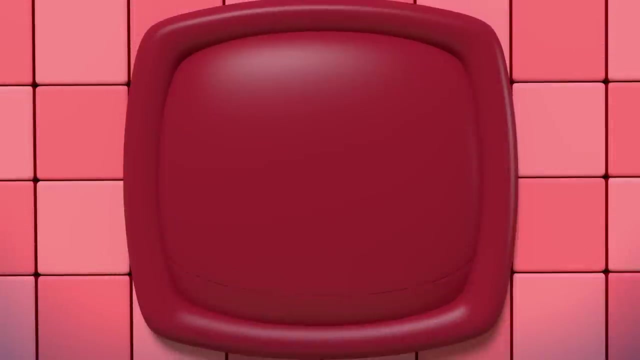 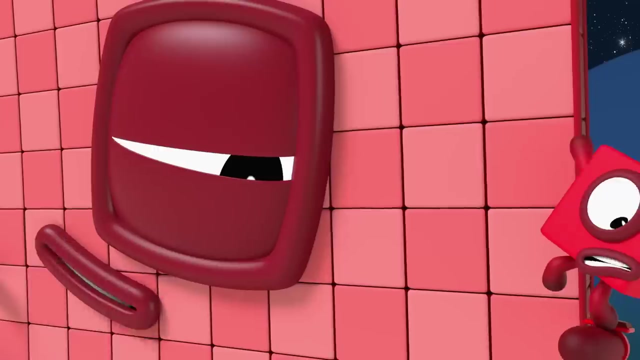 Then ten ones made one ten. We're the one and the zero. Now we've reached a new place, A place of possibilities, A new friend, a new face And a brand new kind of hero. I'm big, I'm really really, really big. I'm gigantic. 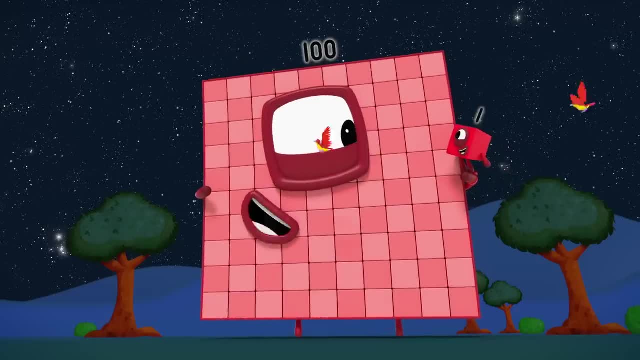 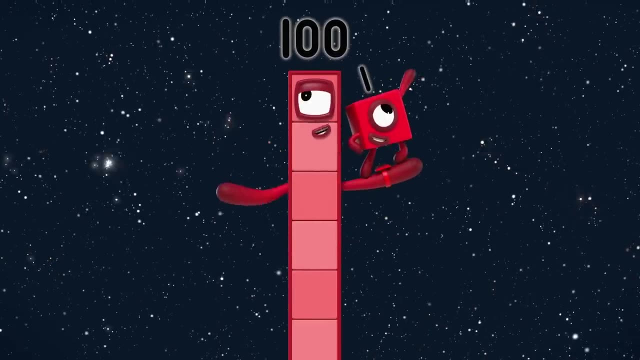 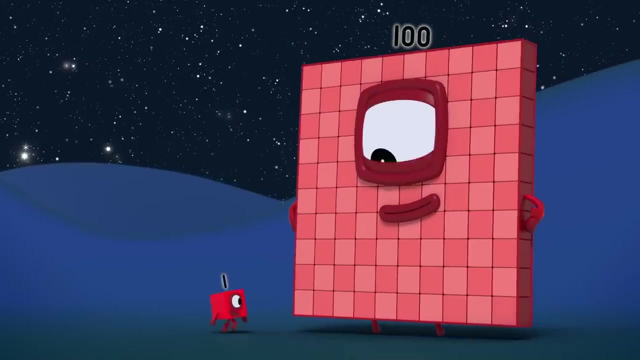 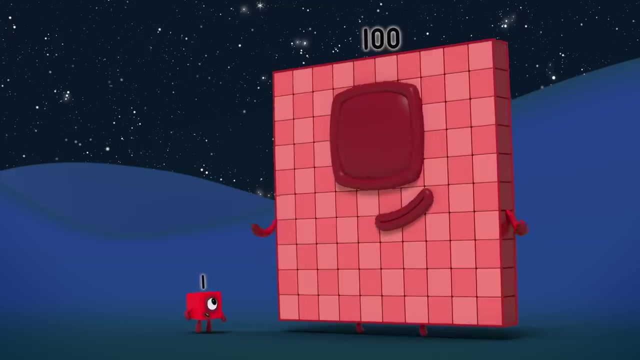 Did I mention I was big? I'm taller than the tallest tree. No one here Is as tall as me, Cause I'm big, I'm really very big, I'm so big. You'll need a quicker way to count. If you count ten tens, One ten at a time. 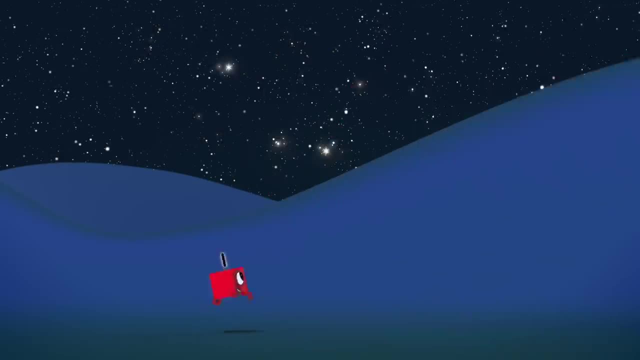 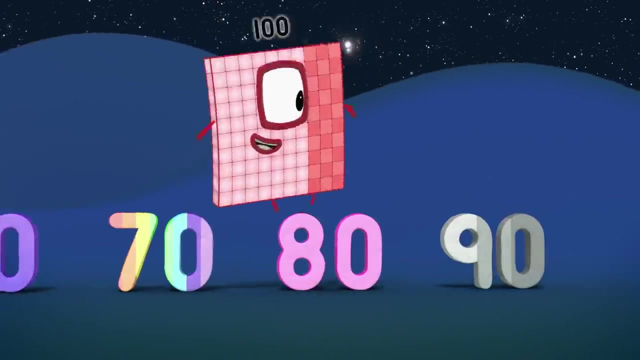 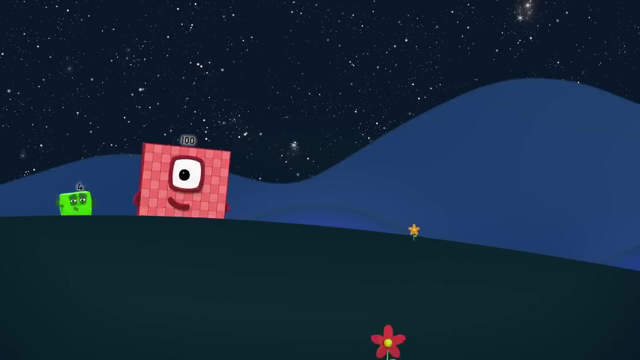 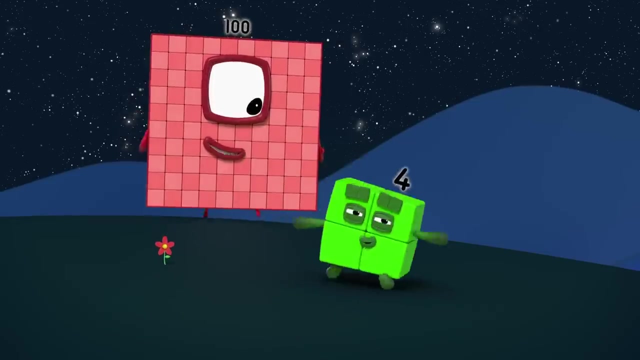 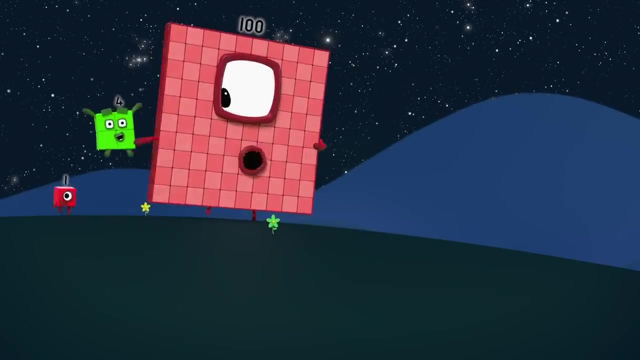 You'll reach the right amount. Ten, twenty, thirty, forty, fifty, Sixty, seventy, eighty, Ninety, one hundred. She's square. I'm ten by ten. That makes me square. She's impressive. Now I've noticed that she's square One. four, nine, sixteen, twenty-five. 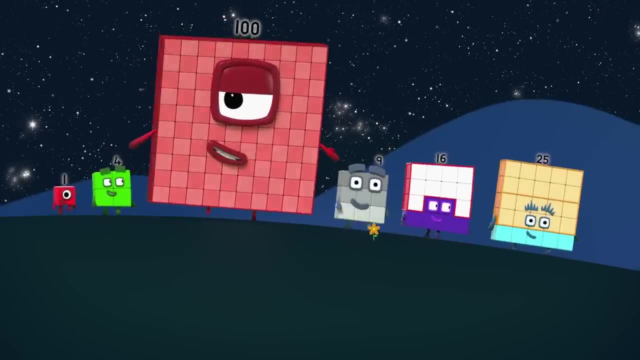 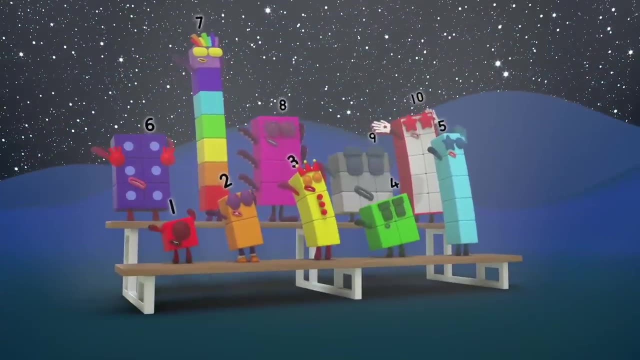 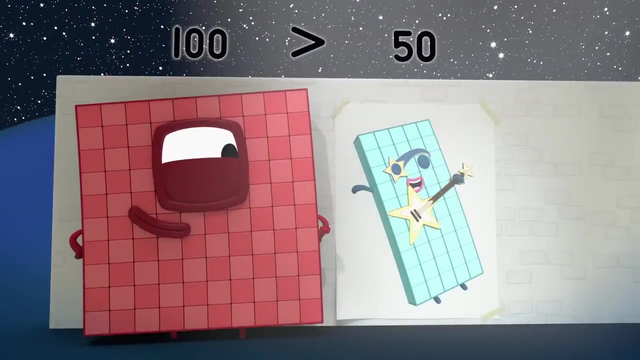 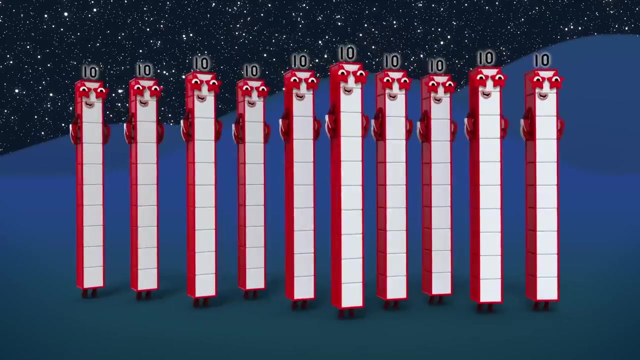 You'll know when all the squares arrive, Cause I'm square, I'm one big man, Big, massive square. She's great. You can't help being quite impressed. She's the greatest, She's greater than the rest. She's ten times ten, as you can see, A hundred times the size of me. 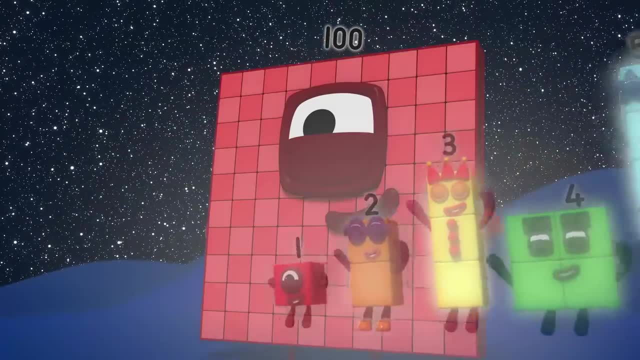 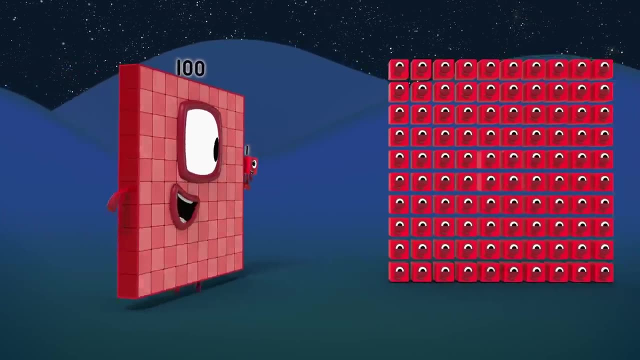 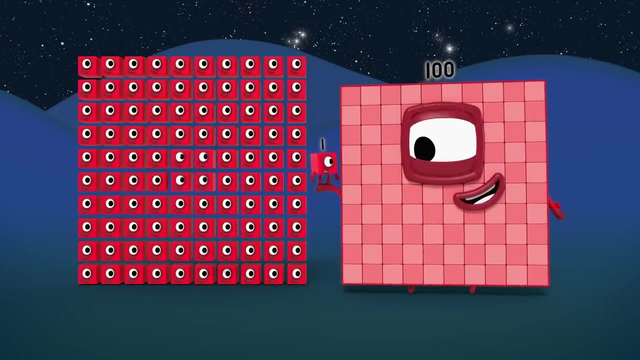 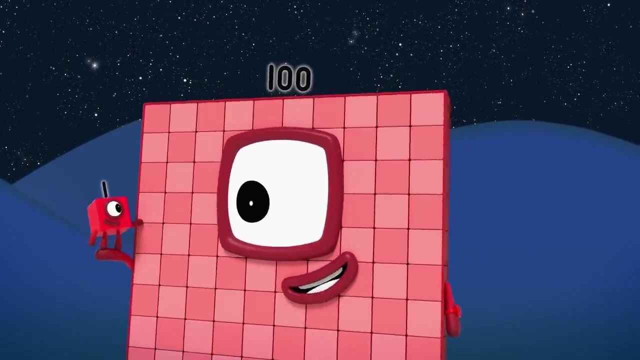 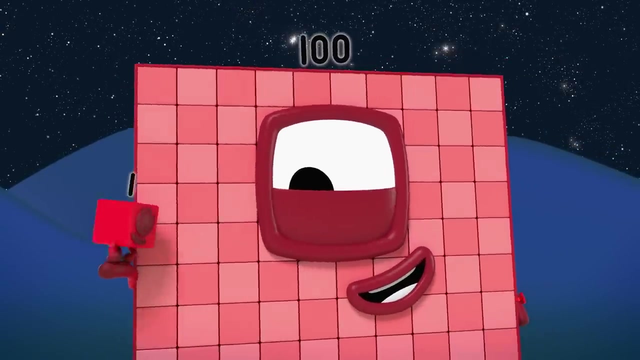 She's great, We all think she's the best, But I'm still one of you, I'm one with you. It takes a hundred ones to make one me. I won't make fun of you. I'm not done with you Inside. I'm just like anyone. you'll see.